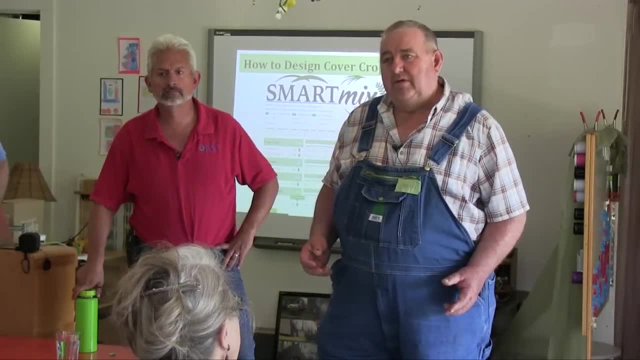 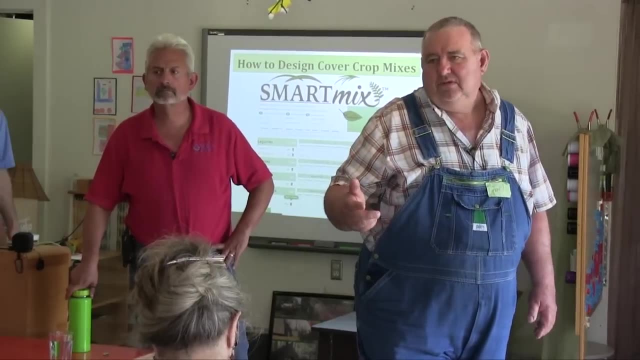 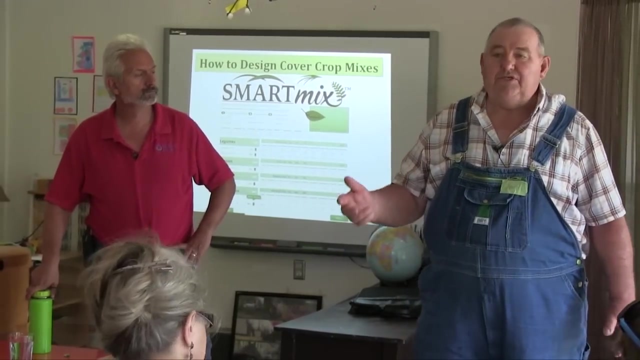 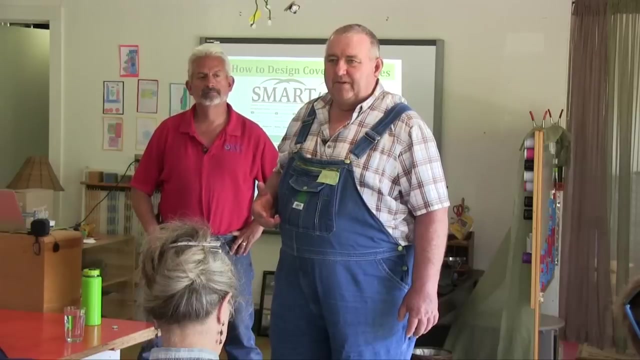 weather climates, we'll get success with something you know. And brassica is a reddish, a turnip, kale, mustard rape canola. What else did I miss? That's pretty much it. And there are deep-rooted plants that tend, when they die, to fumigate the soil And when they die, and 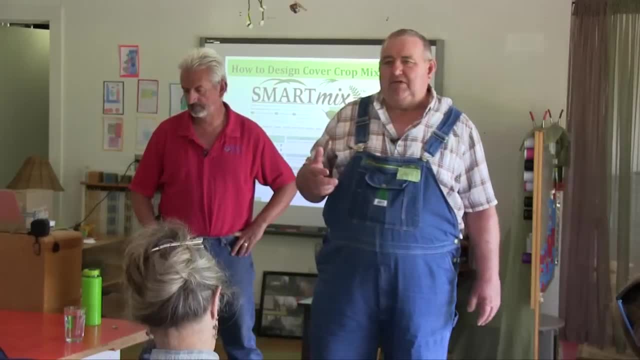 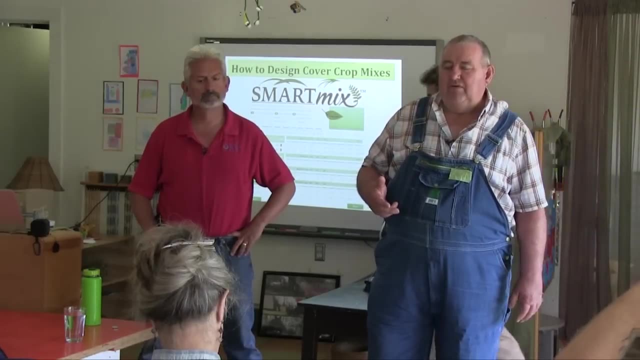 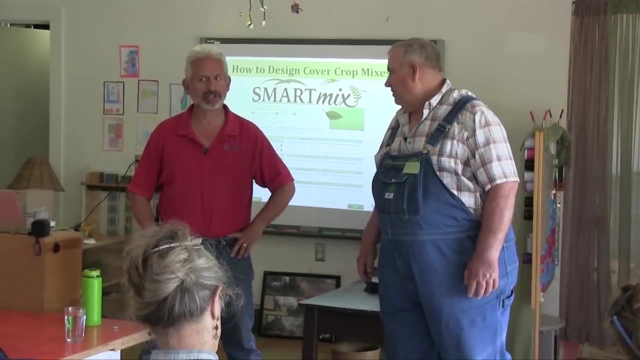 fumigate the soil, they usually take out the harmful cyst nematodes that's in the soil, like soybean cyst nematode, corn cyst nematode. It will actually terminate them and not hurt the beneficial cysts. So there's a good book You ready, Because we're throwing a bunch of stuff at you. Here's: 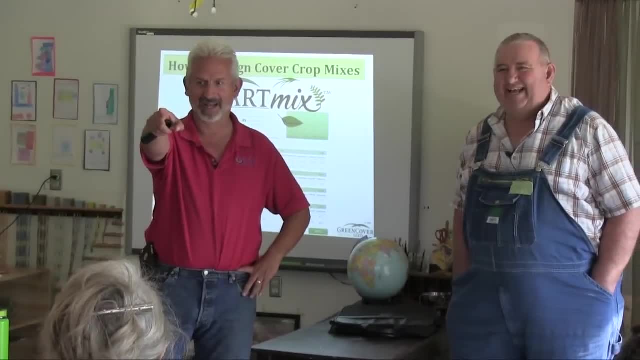 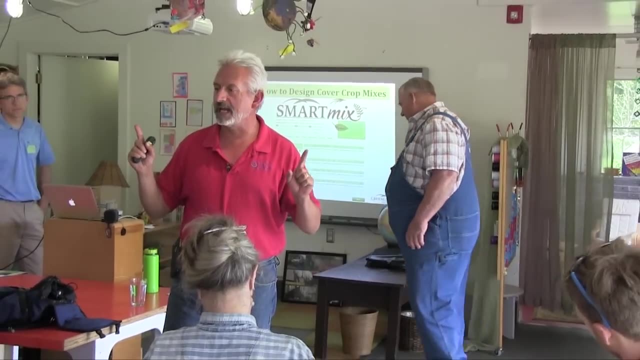 a book you can get for free. Oh, I saw him wake up now. I was like, hey, You said free. Okay, Go to SARE's website, S-A-R-E Sustainable Agriculture. I don't remember What's the you remember? 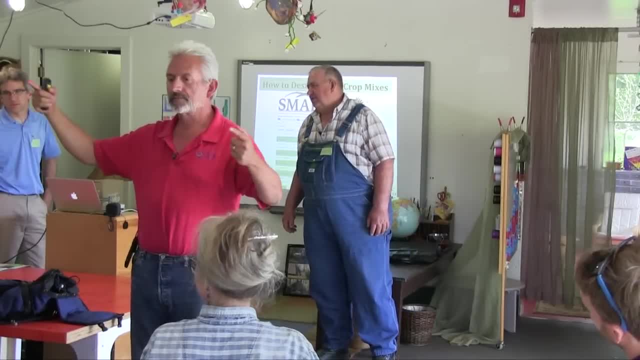 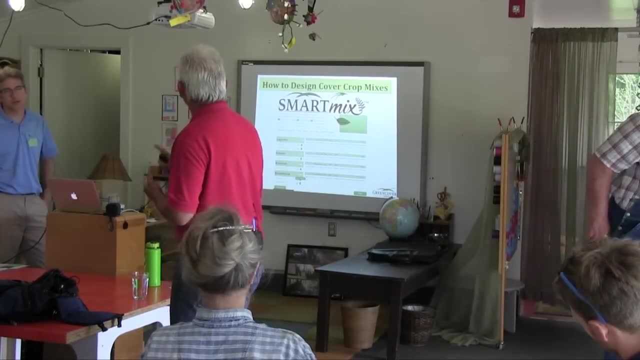 S-A-R-E Sustainable Agricultural Research and Education. Okay, there's Research and Education, Thank you. There's a PDF file called there's Growing Cover Crops- Growing Cover Crops- profitable Free book. Now you can buy the printed version: $20,. 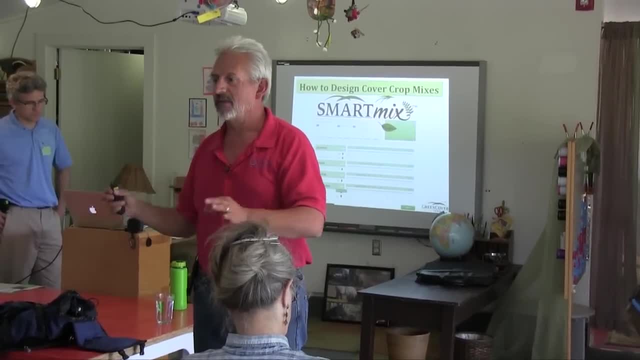 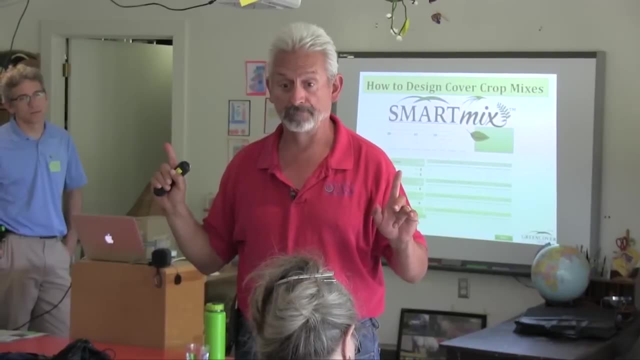 and it tells you all what all these cover crops do. That's a great book. That's a great book to buy for $20, and you can get the PDF. You got a printer. you can download it for free. Okay, I put it on my iPhone because you can read PDF and I go. 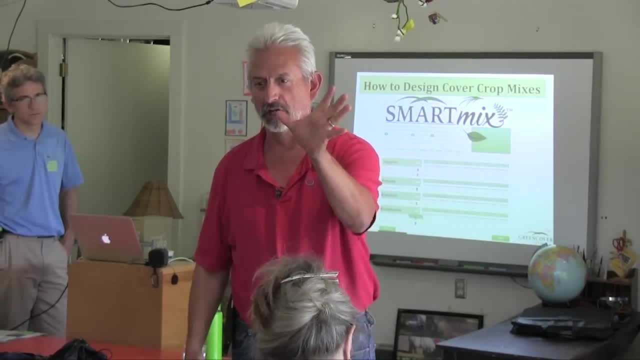 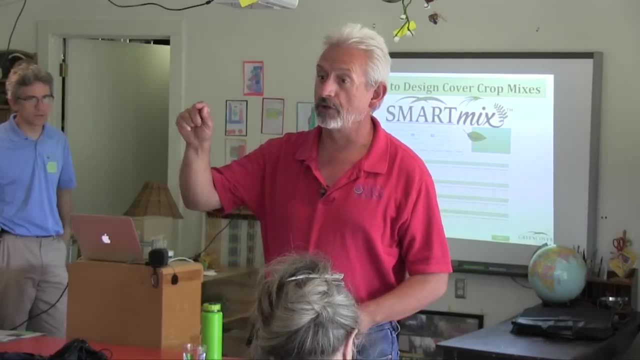 now I don't have to write any printed. I got my mother of a load iPhone. That's why look at this, that's why I got the big honking screen So I can sit there, and there's also another web for your app there that you need. 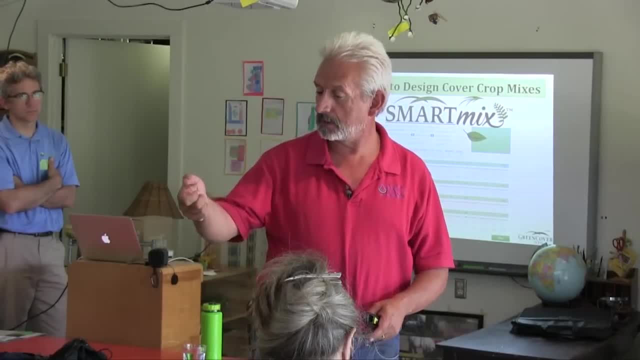 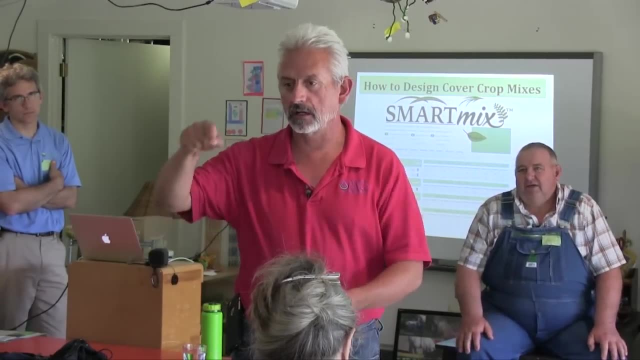 to get. It's called SoilWeb. You can. actually it's called SoilWeb, isn't it SoilWeb? Yeah, it's SoilWeb. Anywhere you stand, you click on there, it'll pick up that point and it'll tell you your soil type, all the other things on that particular field, It's. 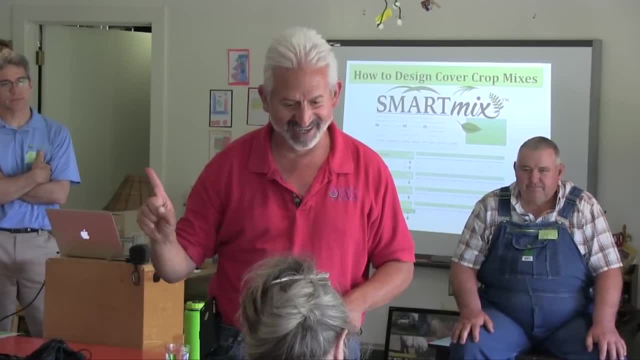 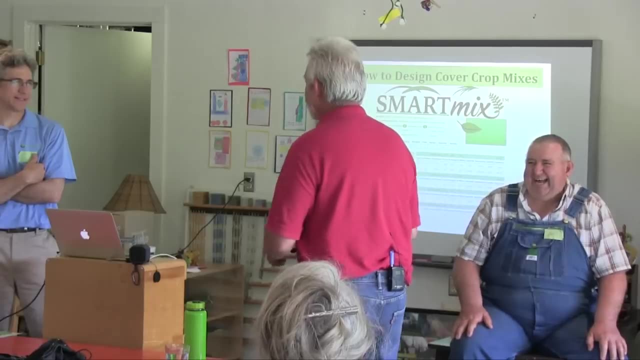 called SoilWeb. It's a free app, Oh cool. Oh yeah, Isn't it cool. This also makes dinner and it's got a phaser, It's all. Does it vacuum? Well, I just, yeah, I tell my daughter vacuum, I call her vacuum. yeah, Here's. 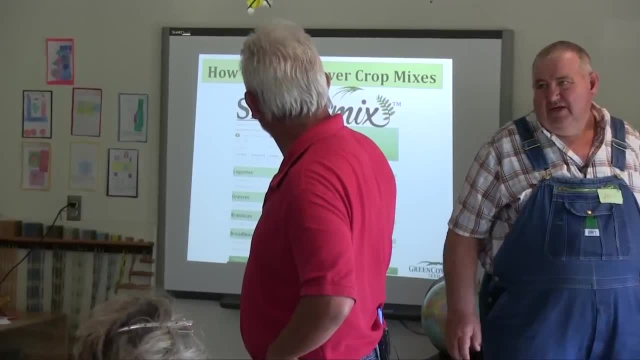 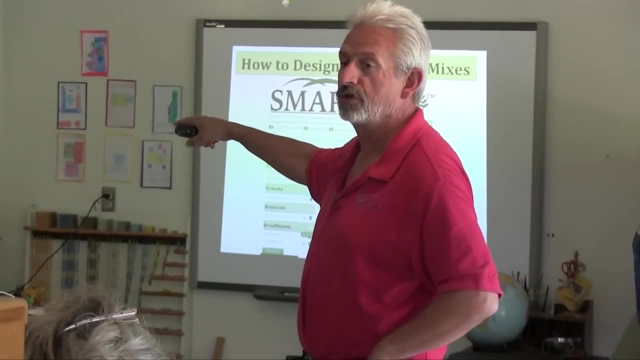 the thing you want to write down. Jay's got one. It's called SmartMix Green Cover Crop Seed Calculator- Really good, so you can design your own mixes And Jay's going to show you one. Are you going to give that and put it? 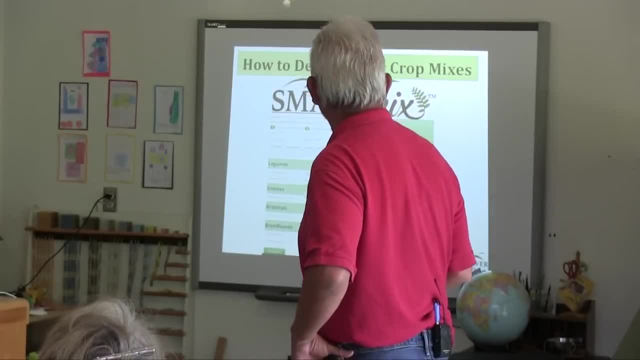 on your website. eventually, Eventually, And Jay's designing one, Show you another one Now. Periodic table, Periodic table, Yeah, and he's got. there's going to be another one We're going to do you have a picture of that one? 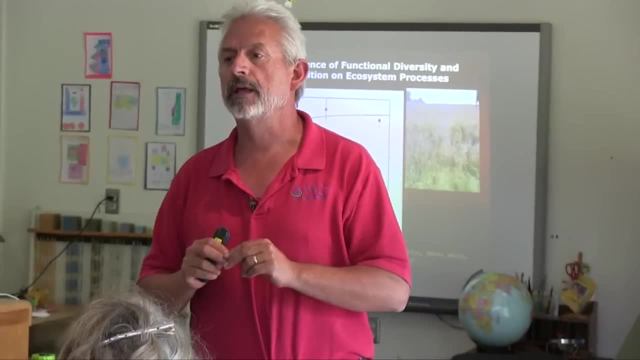 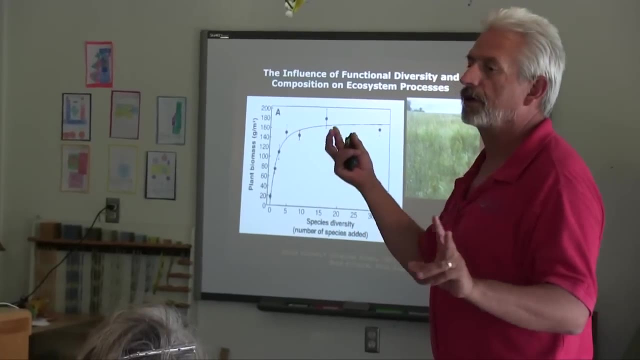 I do. Okay, There's another one called type Cover Crop Periodic Table. It shows you all the cool covers and that You'll find that online. All right Now, for some of you that are real geeky like me, there's a great work by Dr David. 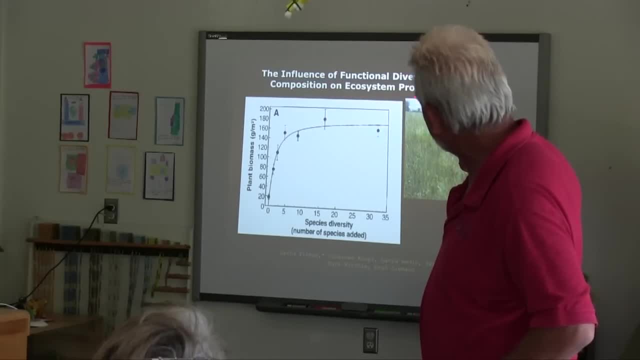 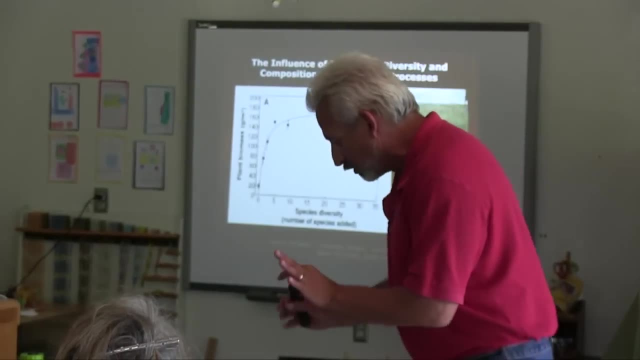 Tillman called The Influence of Functional Diversity and Incomposition on Ecosystem Processes. They did some prairies. Remember I told you prairies in our forest are our template. They had graduate students going through each of those prairie plots and picking out which. 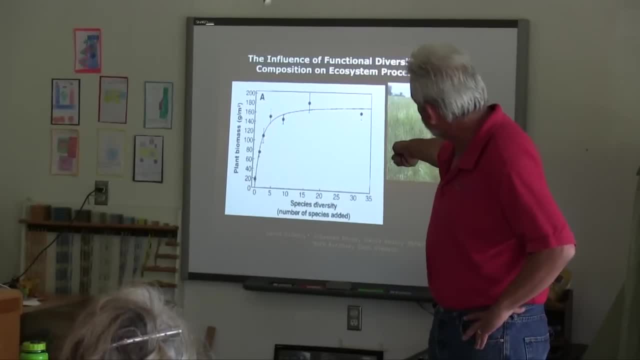 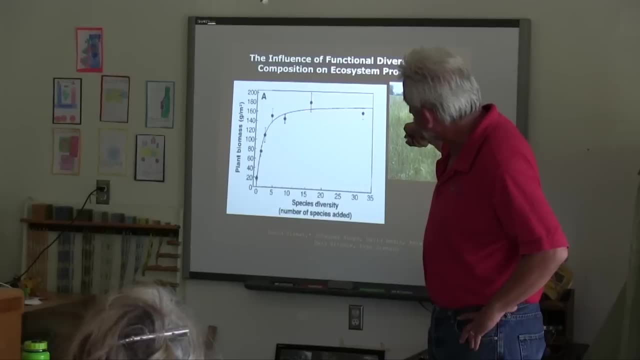 of the functional groups. Here's interesting. Look at the species, Look at plant biomass. Look at here: From five to 15 million- Wow, From five to 15 species. you put in the mix in the prairies, the biomass went up. 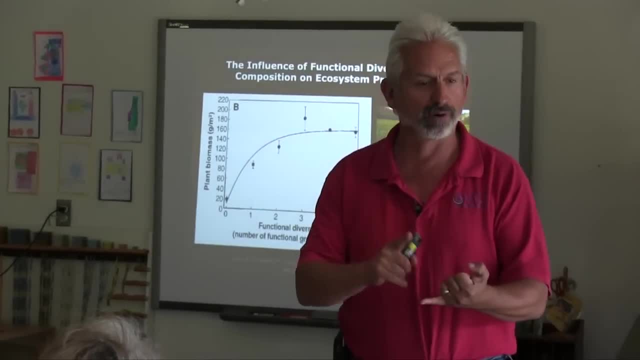 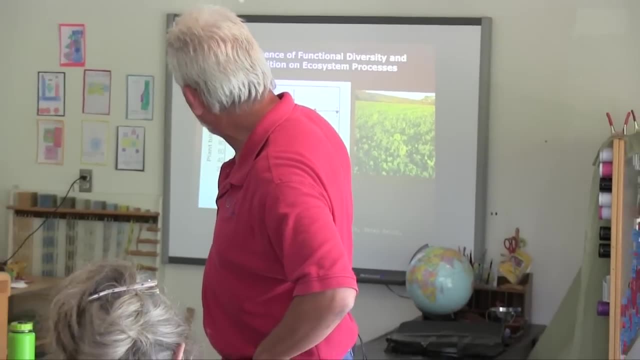 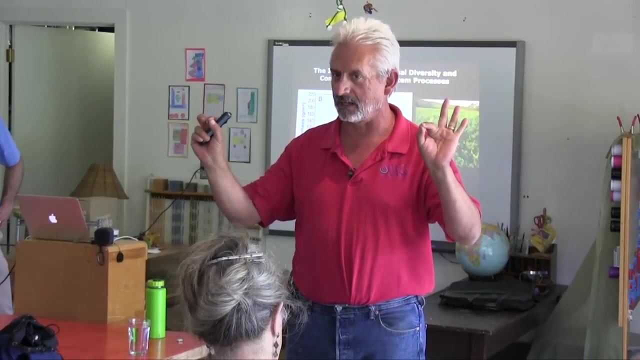 Look at the functional groups. Functional groups is broadleaf legumes, The more I like to have at least three functional groups in my eight-way mix. Now David said something very precious to you. I hope you guys caught on to it. Folks, if I go out there and do, 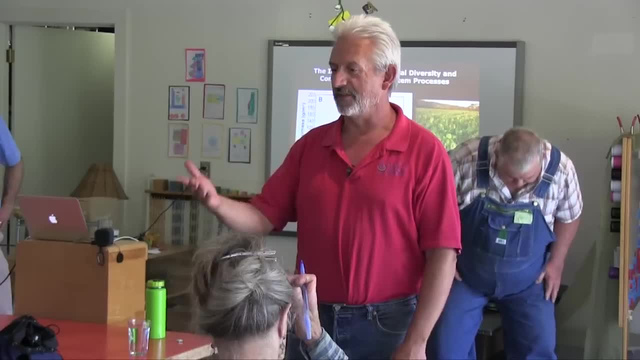 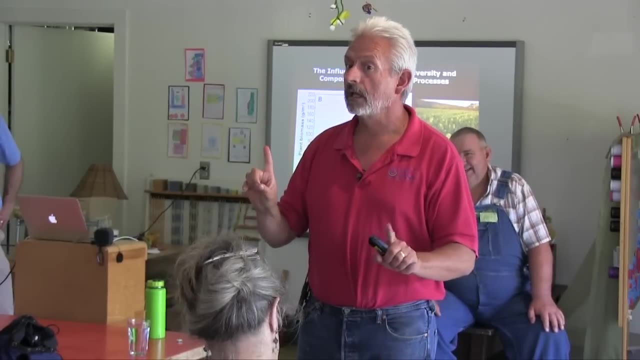 a monoculture cover crop. let's say, I throw wheat, Nothing comes up. David, How would you feel about that? Sucked, Sucked, huh. Yes, You're ticked. This is why I love seven, five, eight mixes. Something will grow under. 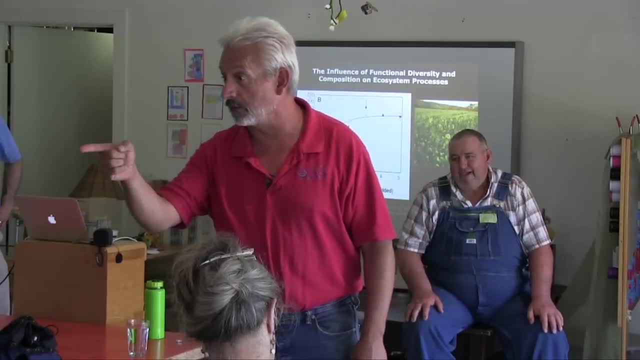 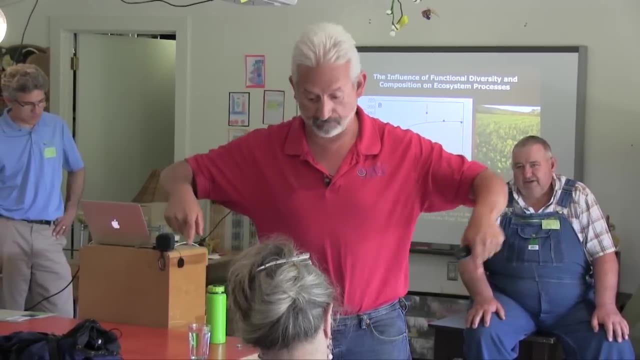 that condition, Even only three comes out of the eight. you're not so angry, are you? What does nature do? Does nature put all her eggs in a basket? in one? Some of these prairies in a square acre can have hundreds of species. That's called redundancy, Redundancy, Redundancy. 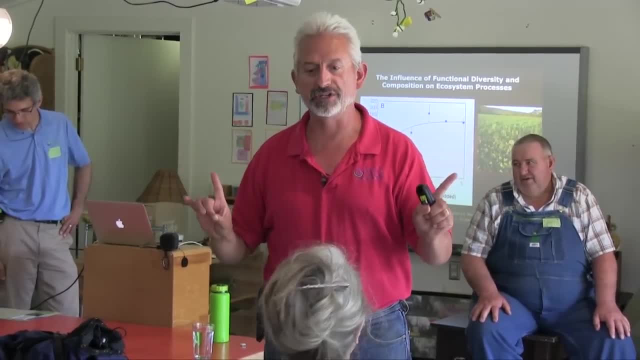 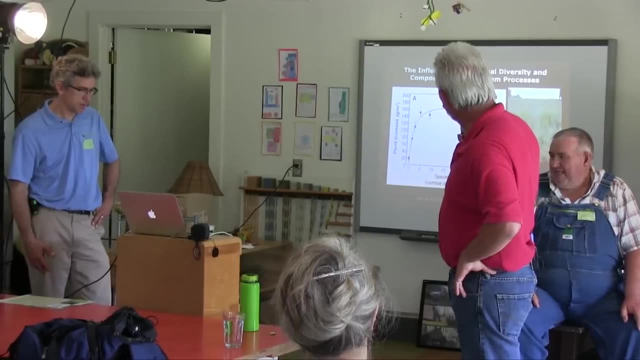 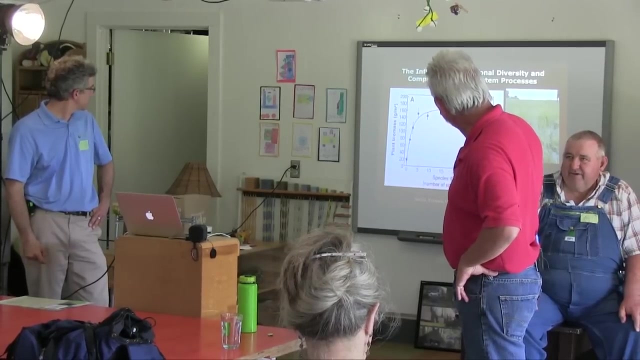 Redundancy, Redundancy, Redundancy, Redundancy seed builds resilience, diversity, okay. so when we design these mixes, i want to see anywhere from. look at the biomass from 5, 8 to 15. once you hit below 15, it starts to plateau. now, okay. 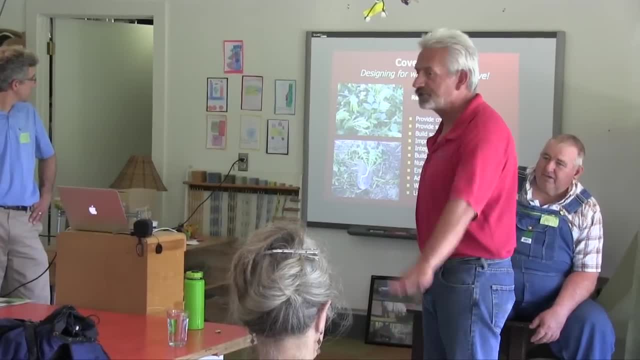 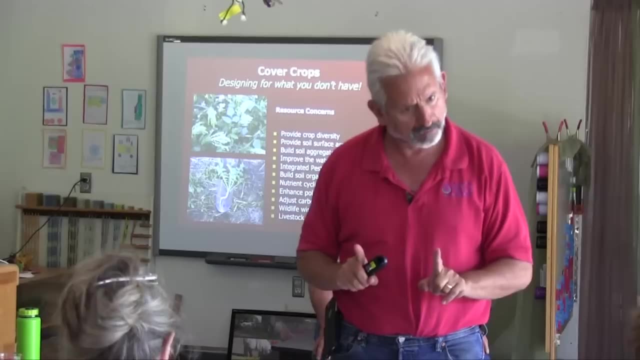 and the cost of seed. what do we want? so the first thing i'm going to ask you guys: what do you want to do on your farm? what is your goal? you don't throw cover crop seed. to throw cover crop seed it's the seeds expensive. what are your goals? first thing in my, out of my mouth: 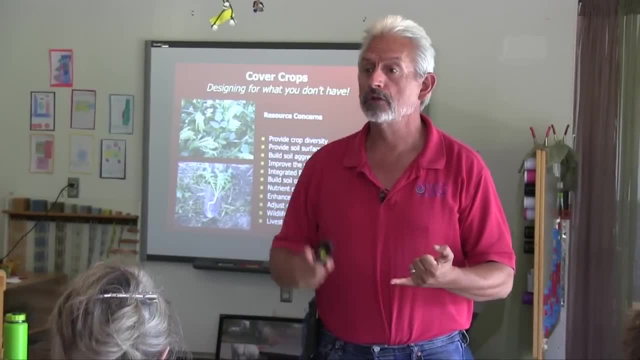 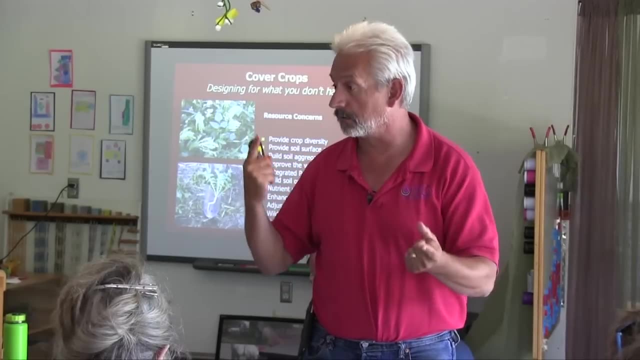 what do you want to do? do you want to graze it? do you want to build organic matter? do you want to suppress weeds? that's the first things are going to come out of my mouth. i want pollinators, i'm going to graze, so then we design a mix accordingly. so the first thing i look at is the 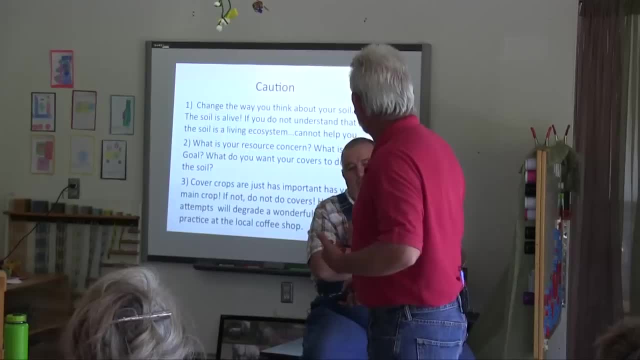 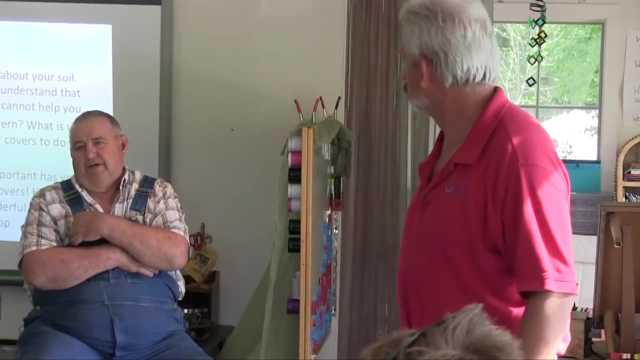 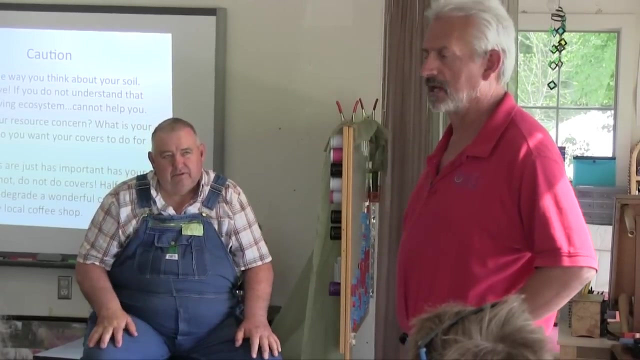 crop that's going to go the following year, okay, or you might also look and see. do you want to improve the drainage? yeah, you know, you don't use a shallow rooted plant as a cover to improve the drainage. if you've got drainage problems, use a deep rooted plant- and here's my cautionary statements, and then we're going to design one. 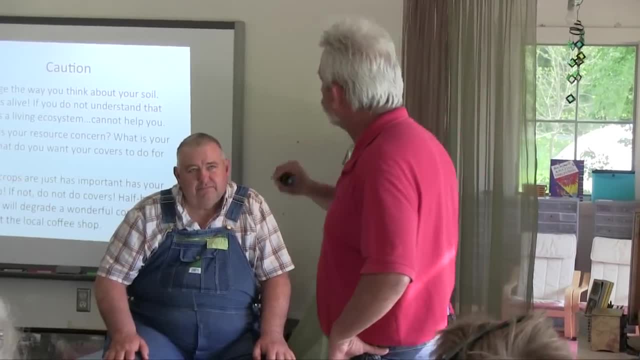 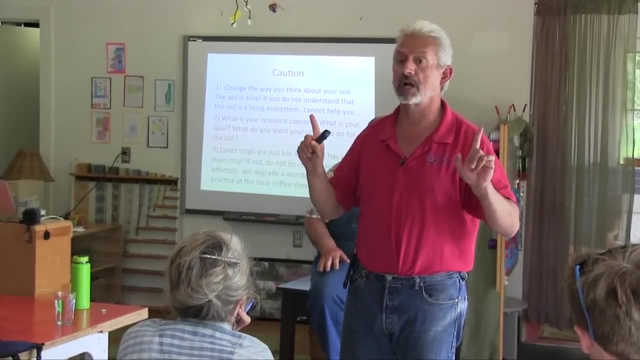 because i gotta place these cautionary statements. here's the first thing you got to understand: soil's alive. you don't understand. i can't even help you. okay, it's an ecosystem. can't even talk to you. you think it's a growing medium. cautionary statement number two: what is your resource? 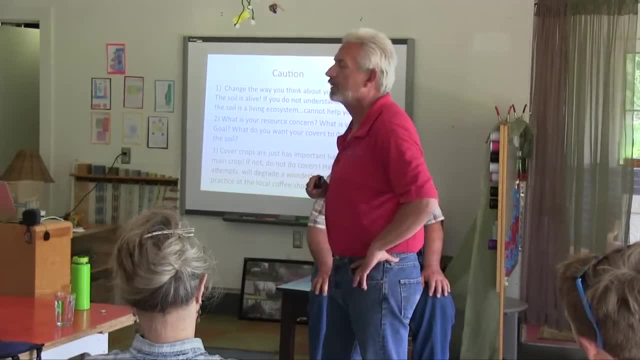 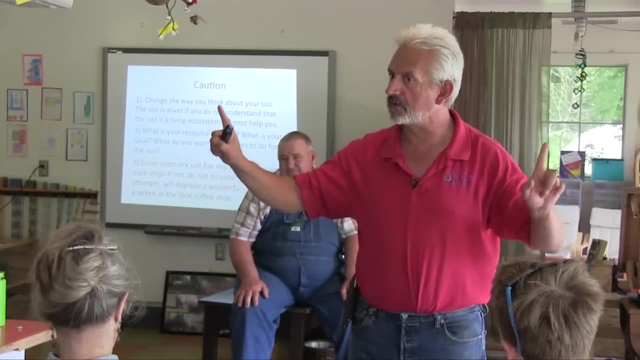 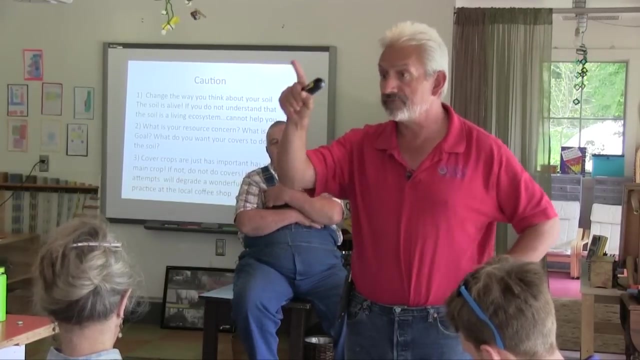 what's your goal. cover crops are just as important as your main crop. if your cover crops are not as important as your crop, can't help you. your cover crops are not optional. they got to be as important as your tomatoes, as everything else. you got to put that commitment. if you're not committed, i don't want you doing cover crops. you know. 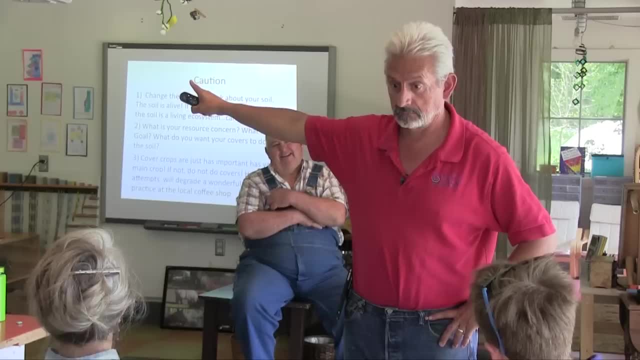 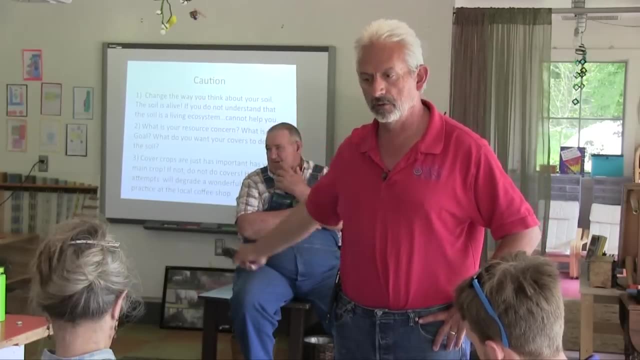 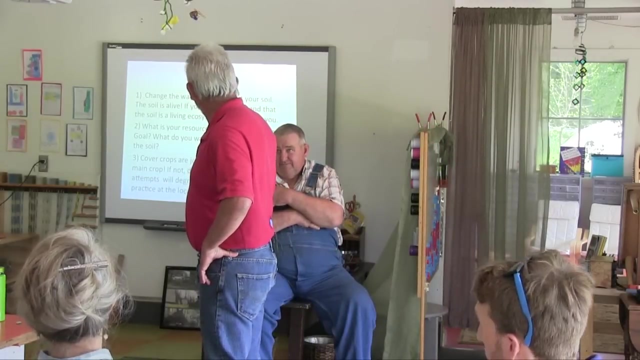 why you're going to go to the coffee shop and you're going to blast it and you're going to condemn it. don't do that. i rather you continue to buy the compost, your compost teas, and continue to do what you do. that's how i get. when it comes to the cover crops, don't do any half-hearted attempts. yes, sir. 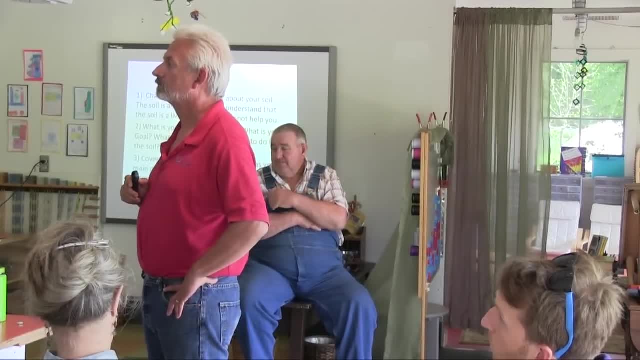 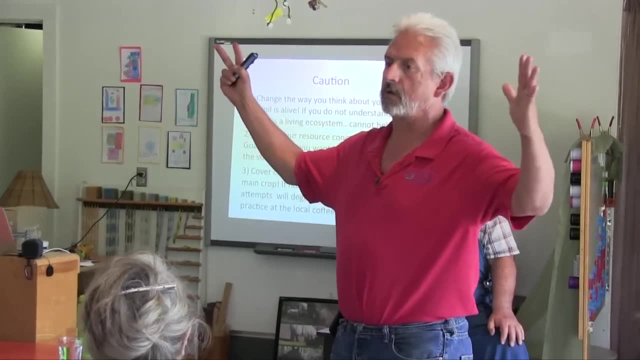 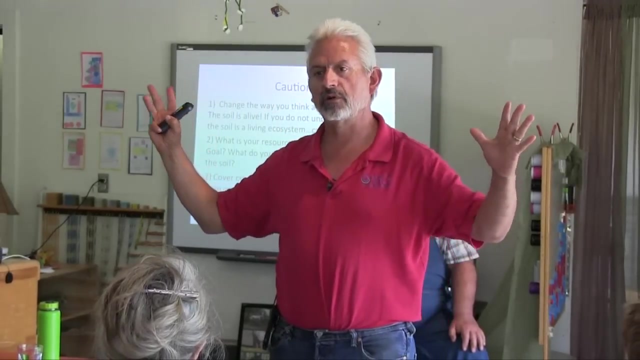 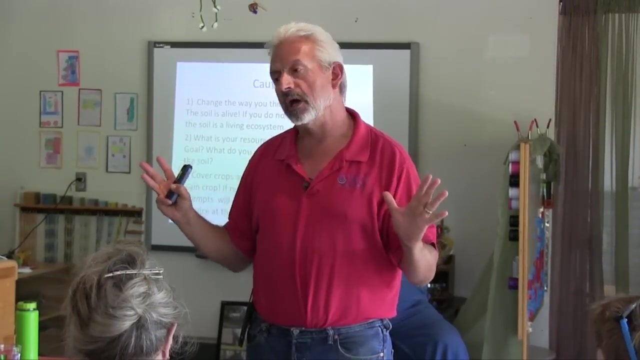 absolutely, and sometimes what i'll do is, if i got sweet corn dave's starting to cut his varieties of his crops down. give yourself some room. sometimes we're growing 120 day corn where we should be growing 100 day corn. give yourself room. that top hören't have enough yard packaging and that kind of stuff. but if you guys put 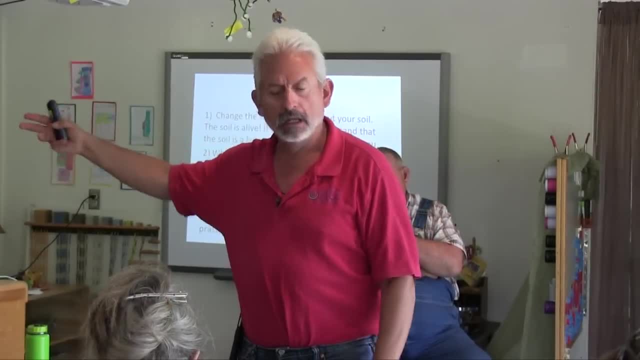 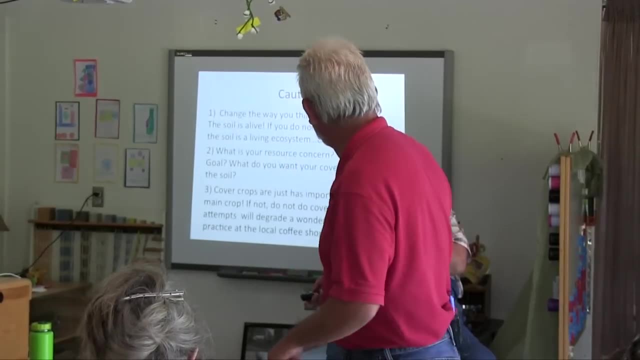 into your há持á hobby garden right here, with your own local Italyob Adventures. most of all, what we do is we back ourselves into a corner and then you don't have space. you don't have space for climbing the front and you don't have space for the back cut. 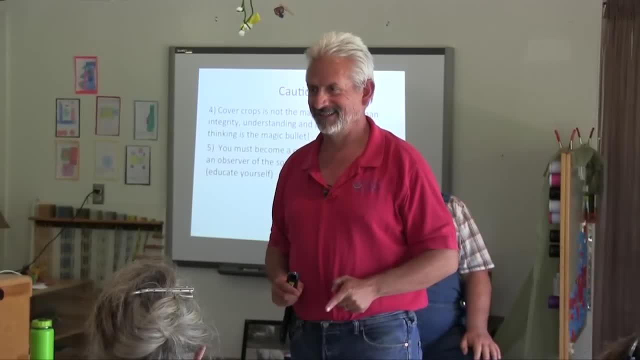 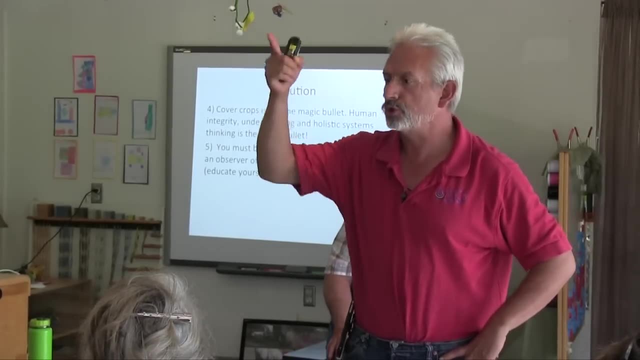 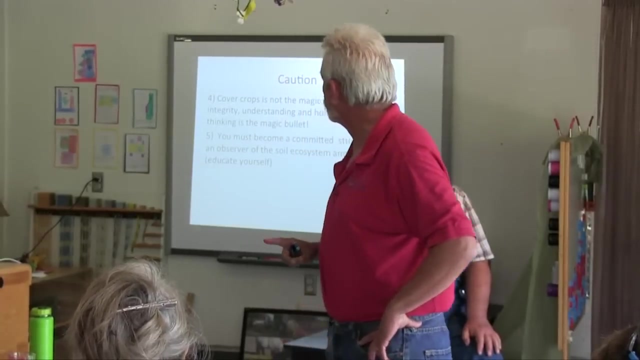 down your variety sizes day length. give you time for your cover crop. you don't want bare ground. going into the season, cover crops is tool. they're never the goal. understanding is the goal. okay, be a committed student. if you're not committed again, I'll say it again: don't. 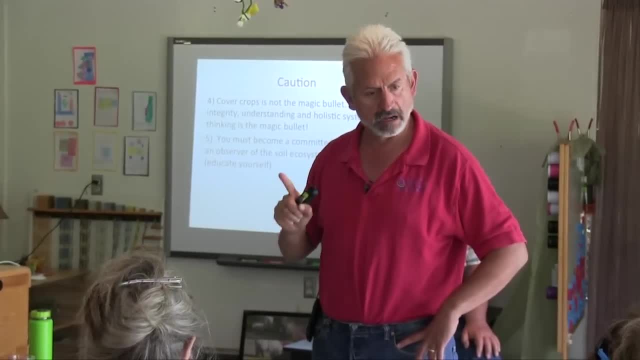 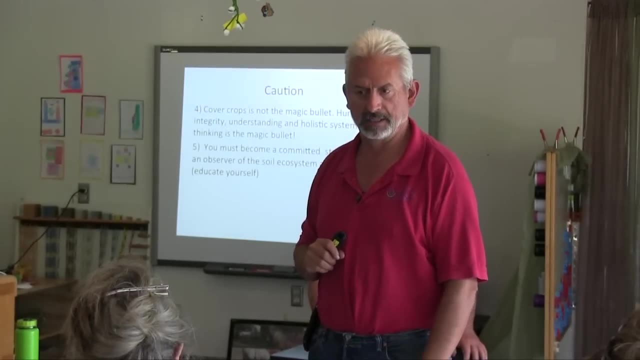 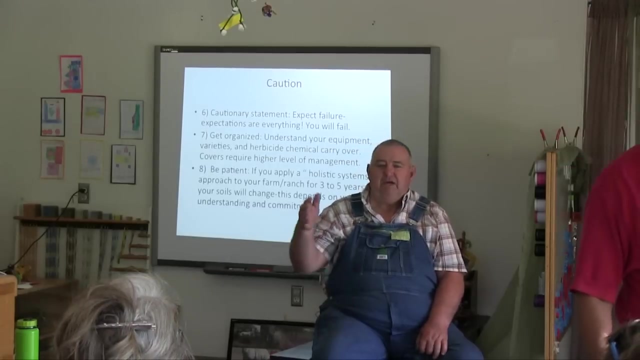 do this. you're just gonna blast it. you got to be a student. I'm taking you to a higher level of management. cover crops require more management. great to find a mentor. yes, oh, great to find a mentor. you know could be your neighbor, it could be me, it could be Gabe Brown, whatever phone and use the phone and find out. 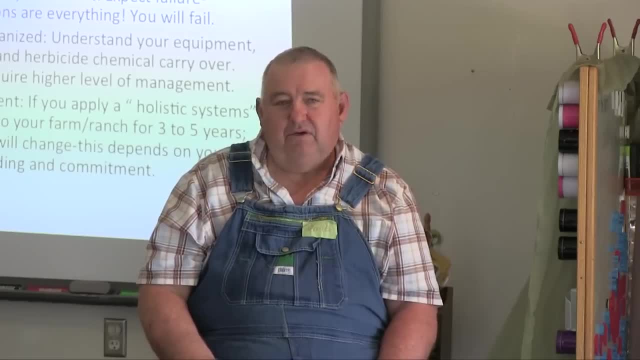 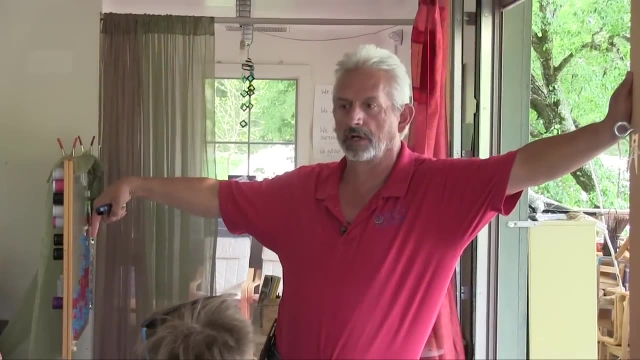 where, where you want to be and who you want to be with. and you know it's neat to start a little group in the county. this place, right here, is a beacon. yes, right here's where's the school we're gonna learn. here's what? another number. 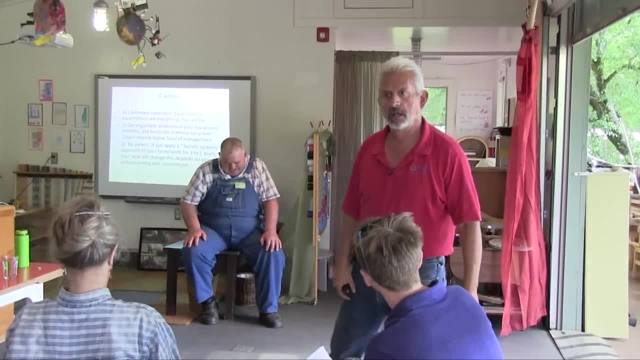 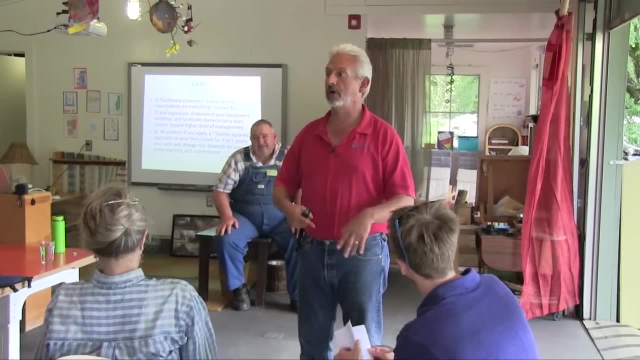 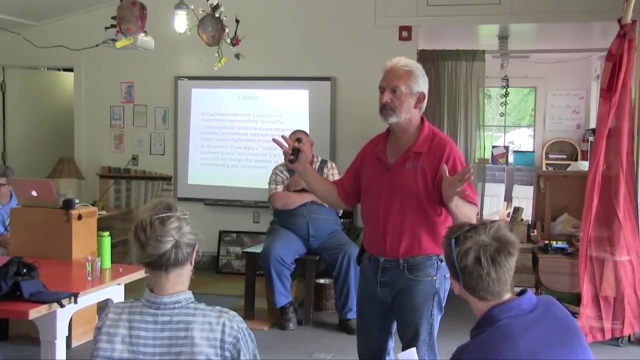 six expect failure. my goodness, you farm expectations are everything. some of you got there, well, raise and raise and something like that, and then you're gonna have to go out there and you're gonna. Dave and Jay says the magic bullet is covers. no, I want you to expect failure. 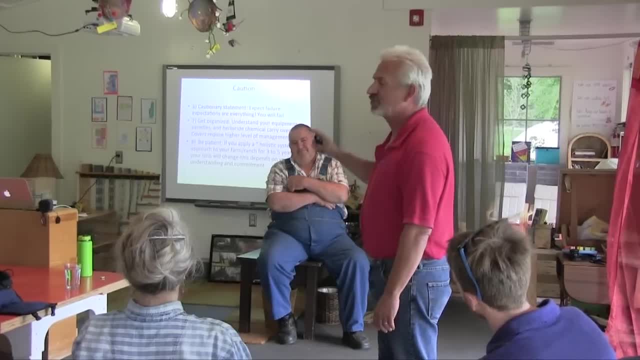 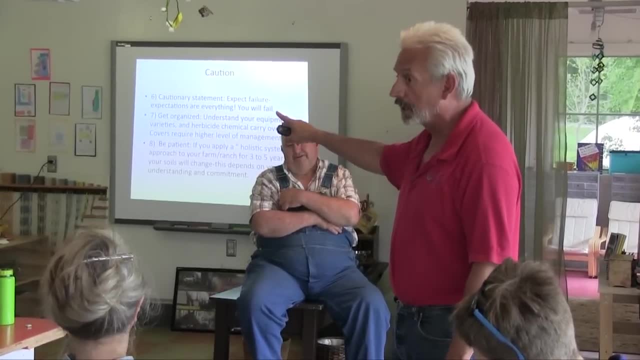 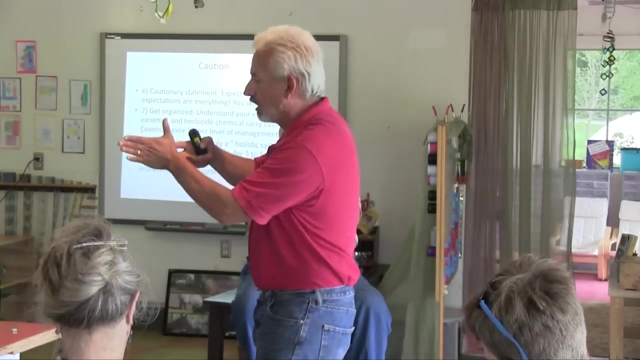 you're going to fail, aren't you? David? number seven: get organized, be very organized. this man, these two are very organized. I've been in their operation. they got the planner ready. they they got the no-till drill ready. as they're harvesting soybean, they got the no-till plan, are coming right behind them. you. 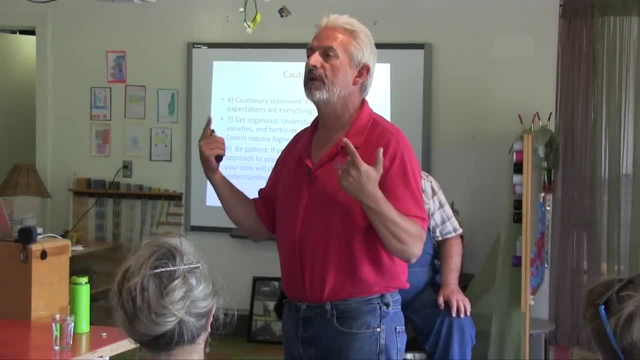 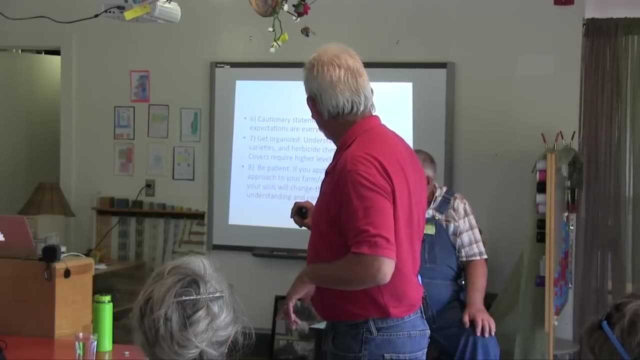 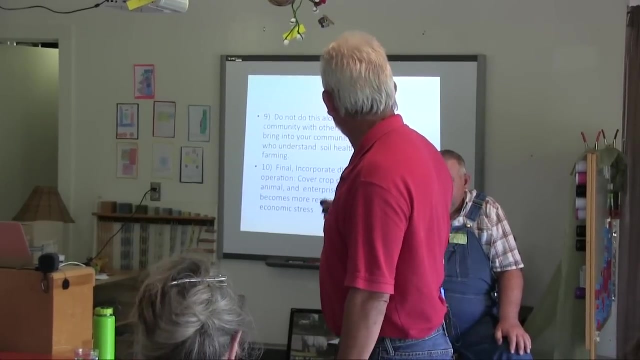 got to have everything planned in the system. a lot of times we fail. it's our mindset and we're disorganized and we're not planning way ahead. okay, get organized requires management. be patient, give us two or three years and we'll change the system around. do not do. 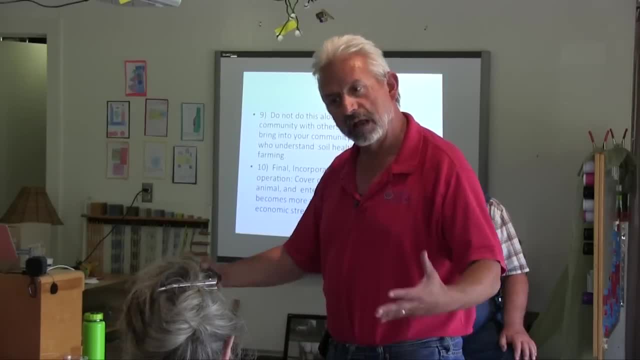 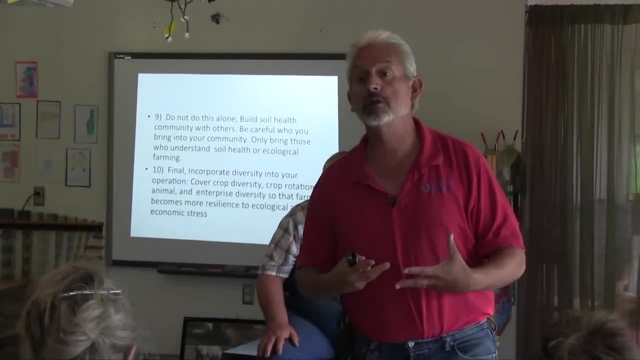 this alone. don't do this alone. you got mentors: help each other. like Dave said, we've got community. do this together. we know what we starting to do in Kansas when we start doing this. so health, we have breakfast together. well, Pat, what we'll do is some of our district. 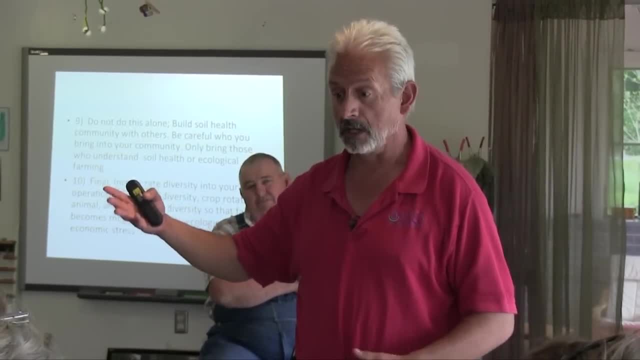 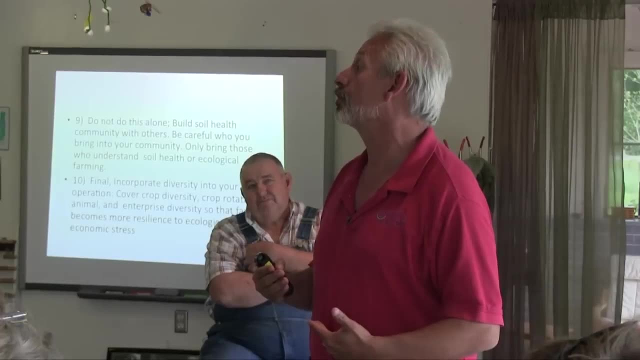 conservationist, get with our farmers and they'll have breakfast, soil health meeting and they'll talk about: okay, how can we be do better, how can we have the breakfast in North Dakota? you know, what they'll do is shop talks. we'll go and we'll talk and in the winter we'll have shop talks where we'll talk about how we 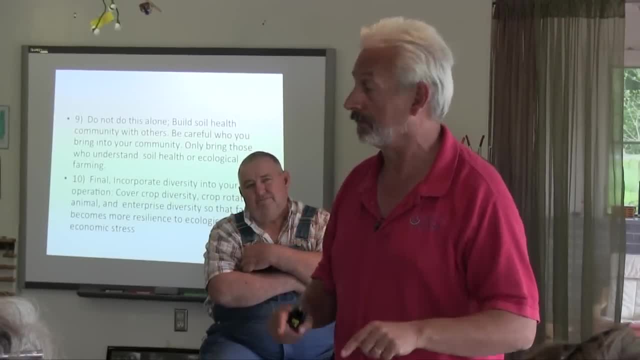 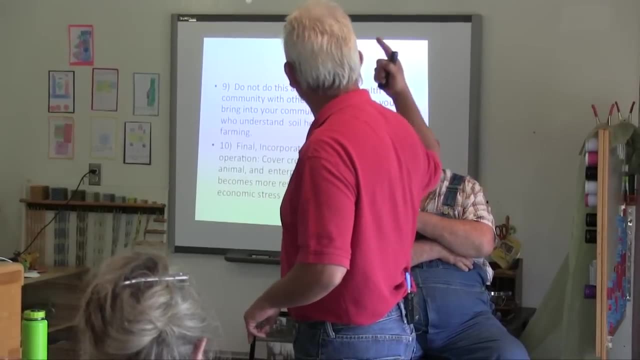 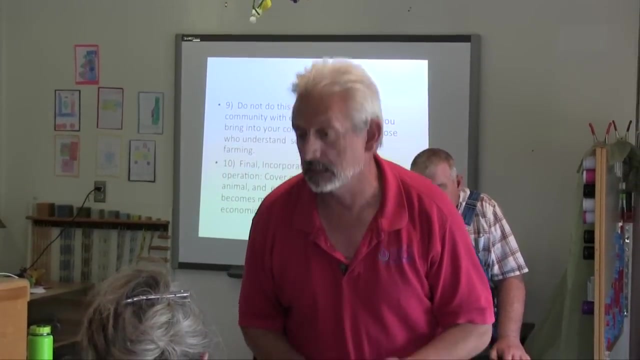 can improve soil health, the community. you don't have to do this by yourself. finally, incorporate diversity in your operation: cover crops to crop rotations, animals to help further our community. When you keep doing that and stacking operations, then you bring economic and ecological resilience. Diversify, diversify, diversify. 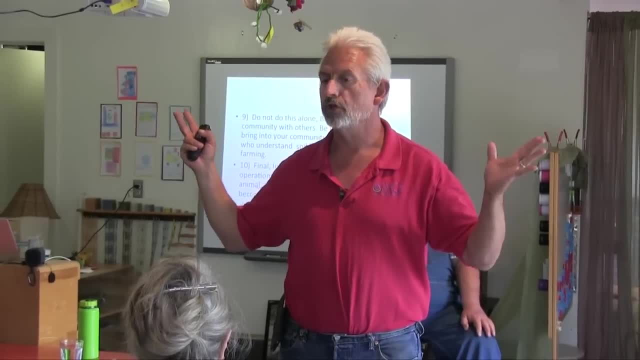 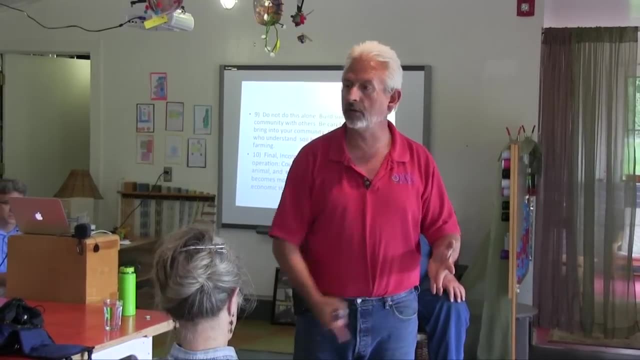 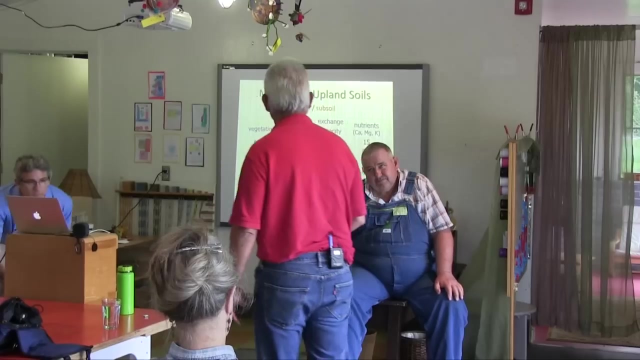 If you grow nothing but tomatoes, you put yourself at the mercy of the market. Now, if you have animals, you have livestock, you have tomatoes, you have squash, you have all this. you're resilient. Okay, And now we're ready for the. let's go into the mix: design mix. 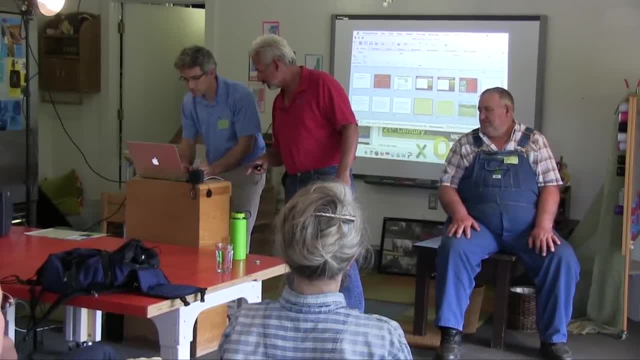 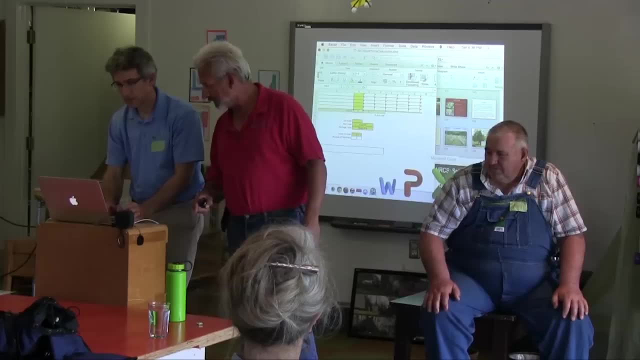 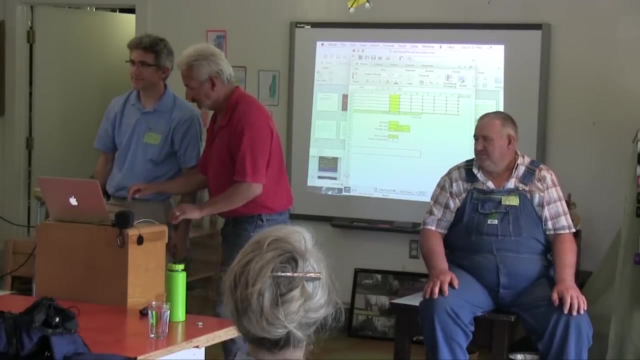 It's right. go to the bottom here and then you've got your calculator There we go, There we go, There we go And just pull it up inside there, Drag it. Yeah, it's a Mac, It's a Mac. 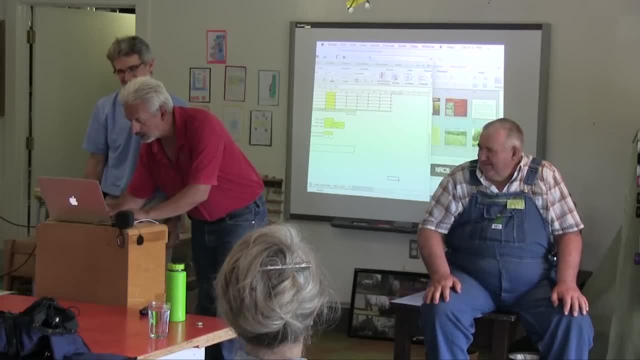 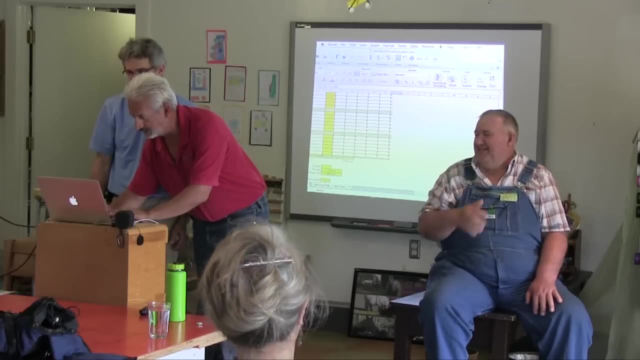 He's a PC guy, but we still love each other. man, We work. You can actually click with one finger and drag with the other. Yeah, yeah, and I'm a slow Mac guy, He's a quick guy. Okay, there we go. 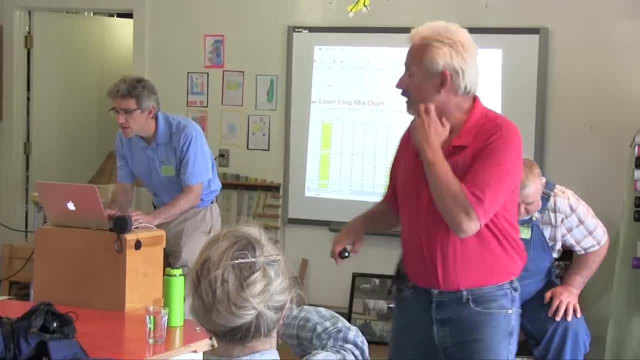 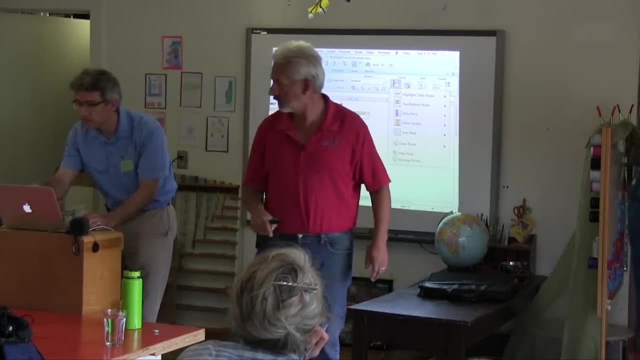 Okay, now we're going to show you the calculator that he made and then you can use. let's bring it over. Can you bring it up? Can you make it bigger? Yeah, make it bigger here. Just go right here. 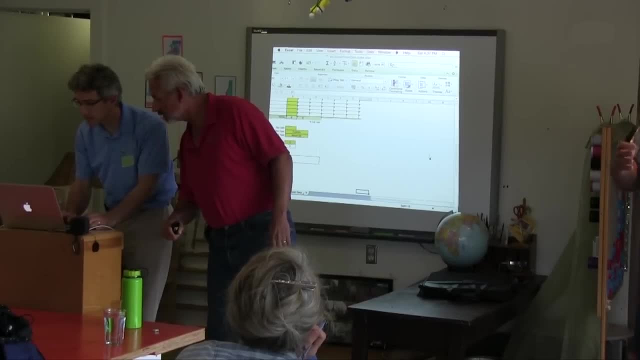 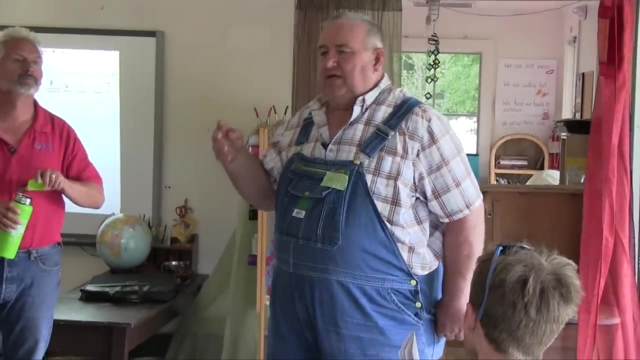 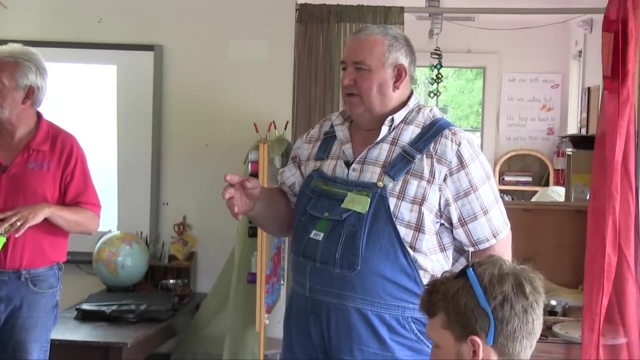 There we go And remember. I guess the biggest key on all this cover crop thing is, if you're using nitrogen-fixing cover crop plants, make sure that your seed distributor has the right bacteria for those plants. Good point If you pick up cow peas, for example, that grow really well in the heat. 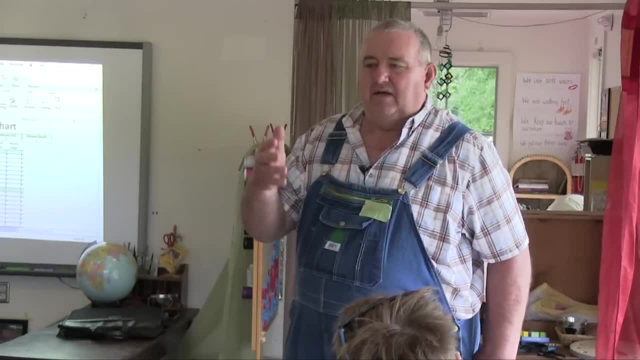 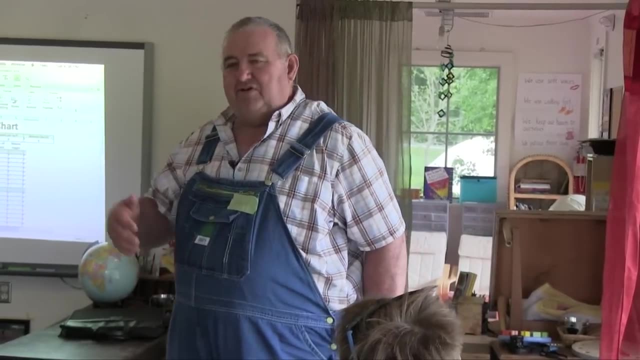 they don't take soybean inoculant. They use peanut inoculant. So if a guy throws 10 bags of something in your truck and you ask him where the inoculant is and he gives you soybean inoculant, you're going to get it. 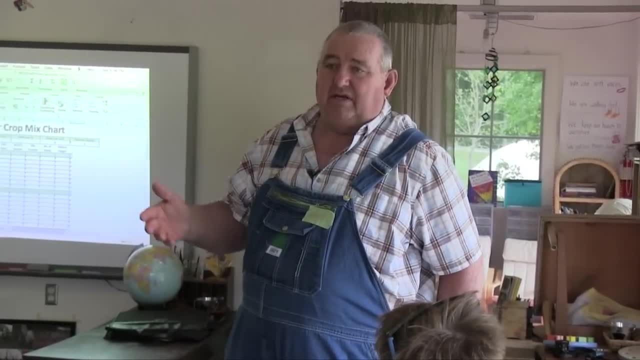 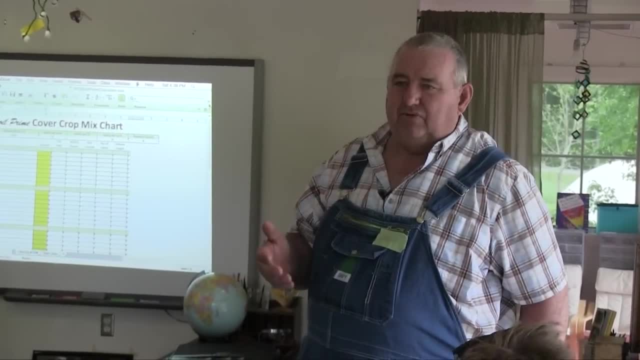 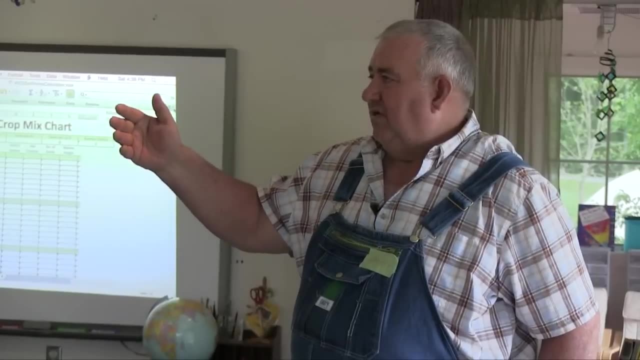 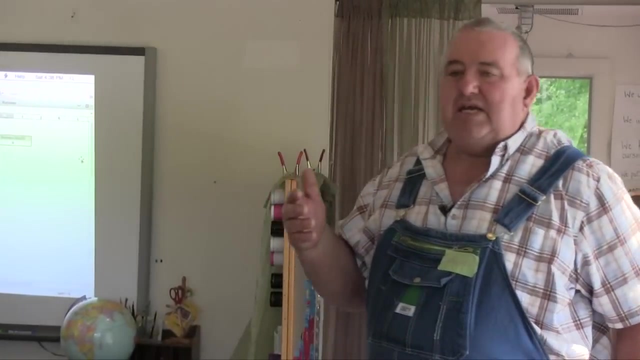 than you can reduce the nutrients or get benefit from yield. In some cases, like this research farm, they're going to have lots of money in this field, But in two years they're going to see how much they've changed it and how loose it's going to be and not need any nutrients for a good many years. you know. 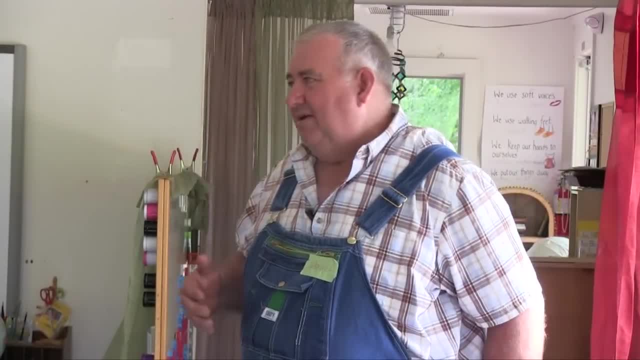 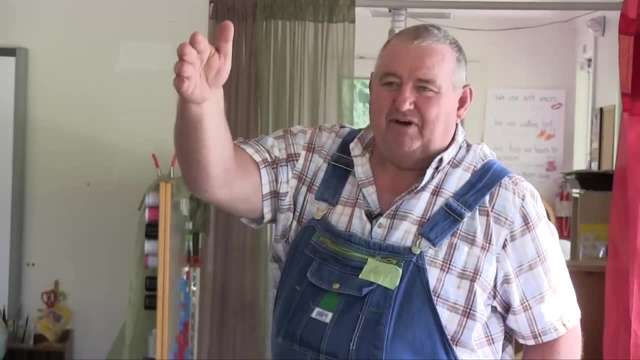 I'm a greedy fellow, I would be out there. you know, I almost want to go steal a neighbor's corn planter down the road here he's making hay somewhere- and go plant. show you how to plant corn, you know. 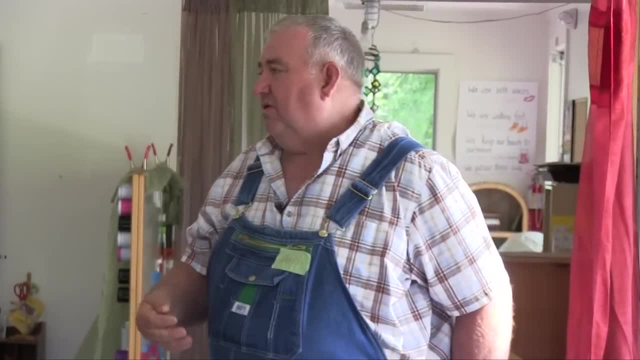 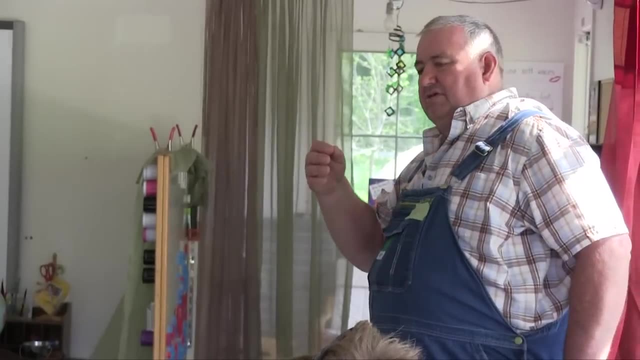 But their goal is to have another year of cover to really jumpstart the soil system. you know, Could you say it again- about the phenoxy, The nitrogen, The nitrogen, the bacteria, The bacteria you need to put on your legumes are different. 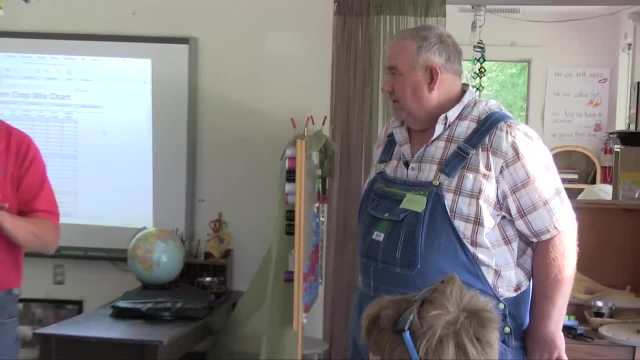 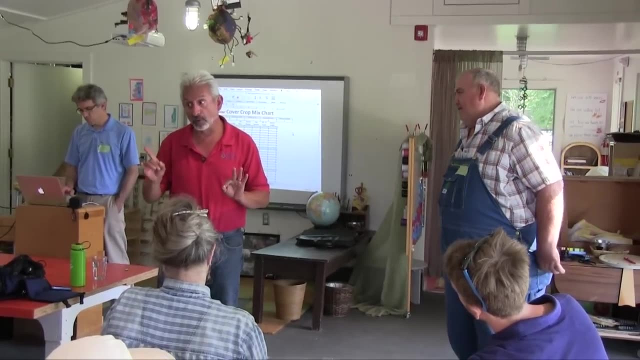 Yeah, so if you have crimson, clover has a different inoculum, peas have a different inoculum. A good certified seed dealer will already inoculate for it, or you ask them to inoculate it, okay. Okay, It's really important you've got the right inoculum. 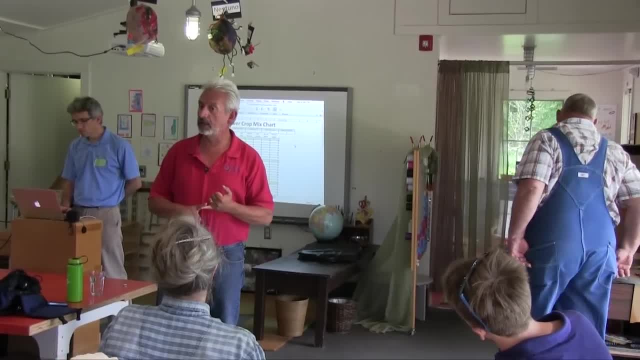 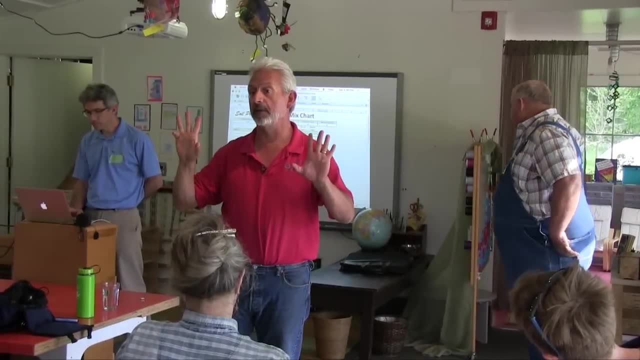 Right, Because if you don't, you're not going to get the nodulation. Now, when I remember, I told you I've got one, three functional groups. If I have about an eight-way mix, I like to have at least three. There's three legumes in there. Yep, I want the legume to feed the rest of the mix. I do not want to use any fertilizer inputs. If I'm asking you to spend $35 in seed now, you're going to spend another $25, $40 an acre for fertilizer or some. I'm not going to do that. It's not cost-effective. Let the legumes do their business, okay. So I like to keep a good margin: $40, $50,. unless you have a really high-cost crop like tomatoes, then $70, $80 an acre for cover crop seed is not unprofitable. Unreasonable. Ray Steyer spends about $75 an acre for his cover crop seed, but he buys no chemical nitrogen, very little herbicides, little fuel. so it works out really nice economically. Okay, now go ahead. Jay, you want to? Sure, go ahead Absolutely. There's small growers around here. If you don't have an easy source, there's one inoculum from Seven Springs Farm that has a really wide range of plants. They have more different ones than others at home. 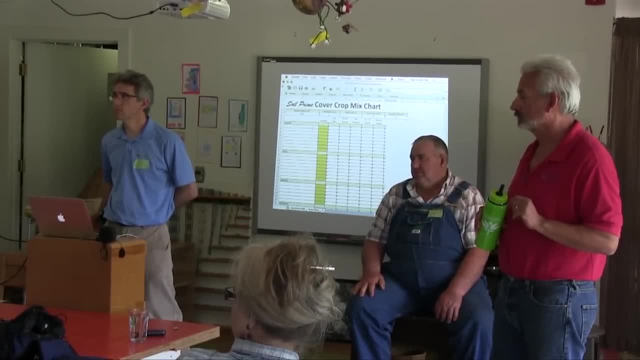 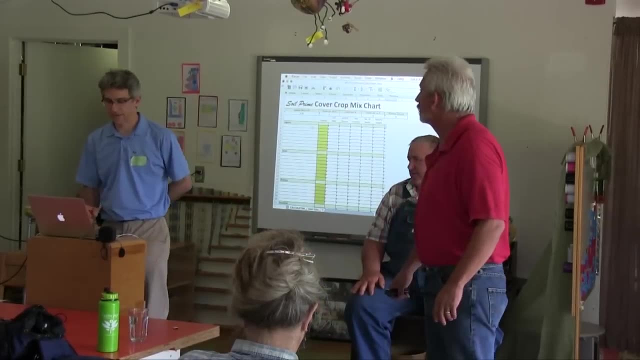 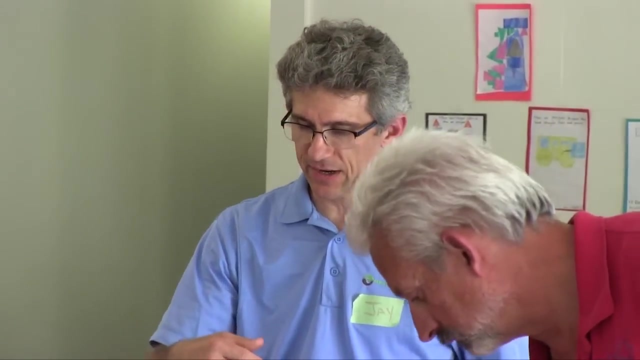 Make sure you ask them to look at it and make sure how great you use it And how do you invest for general use. Okay, now Jay's going to explain this calculator that he's going through. All right, this is similar to what Ray introduced before the Smart Mix Calculator, and I kind of based this design on one of some of that. 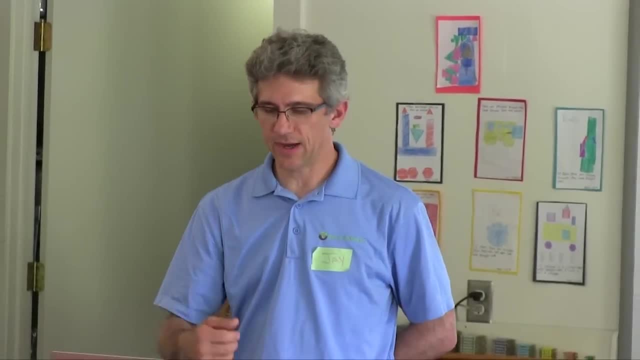 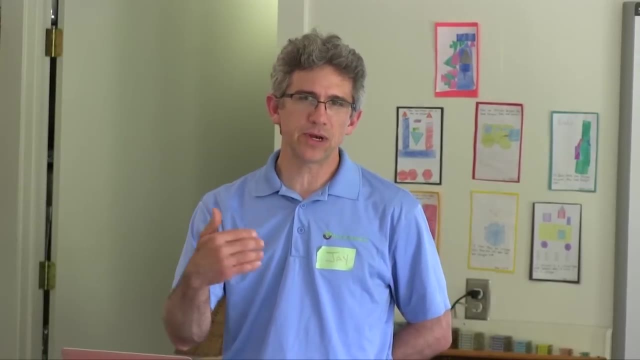 I use it in my business when guys come in and we do some custom mixing for them, because it allows me to look at basically the combinations that we're looking at And the things we want to look at. is that balance based on the goals that we have? 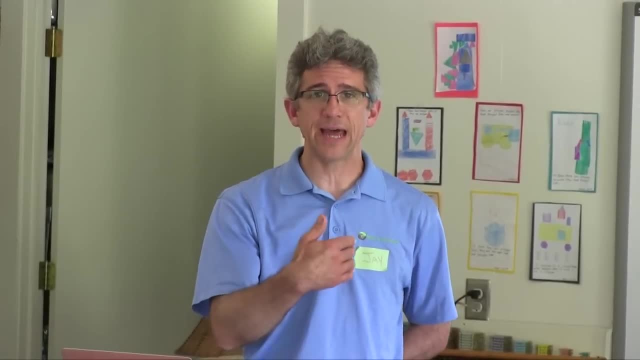 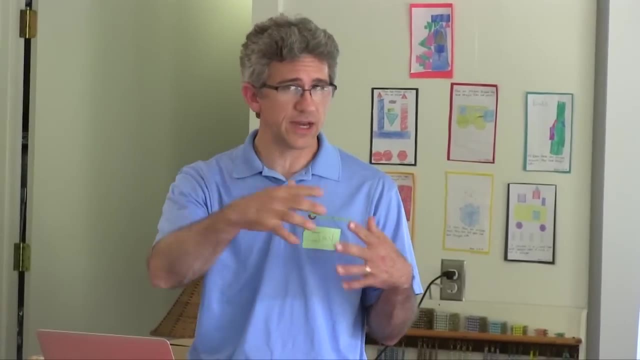 Whether it's for grazing or adding nitrogen, you know, depending on the types of crops that you have in place, adding pollinators and things like that. So because of the study, I'm more familiar with that and have a good idea based on what people's ideas for inputs are. 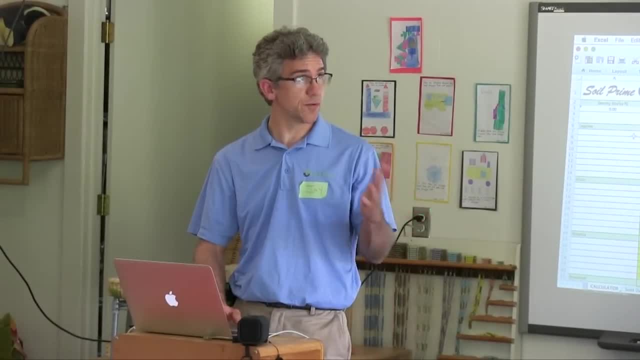 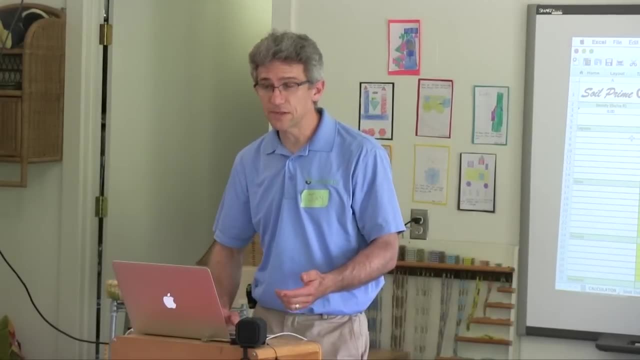 So we were going to work on a summer mix for this. Yeah, we can work on it. Where's Meredith? That's all right, Okay, Okay. So let's start on that summer mix. You're going to see a beautiful winter mix and we're all going to walk out there in a little while. And one of the things that I look at too is for the rate of coverage. So we figure, when we're putting a mix together, we want to have between 30 and 50 seeds per square foot. So we're talking from a gardener's or small plot standpoint. you can understand that. 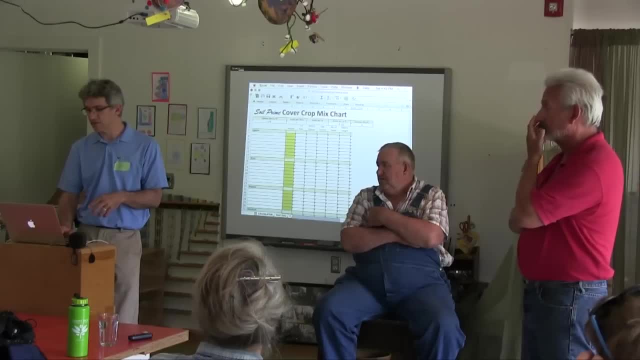 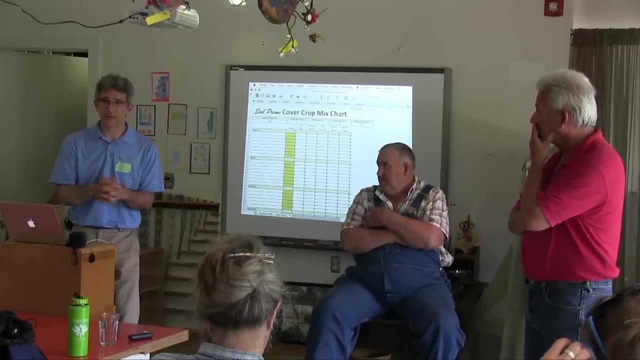 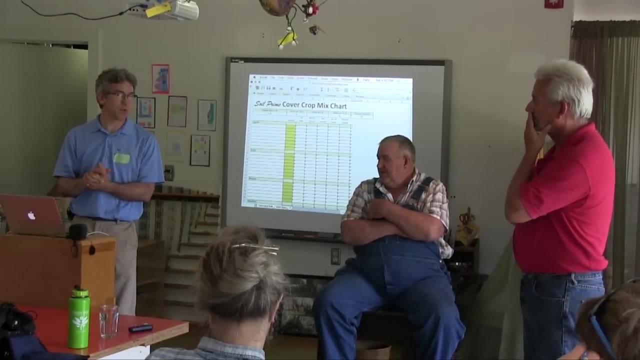 And you can see in the calculator- I've got that- where it calculates seeds per square foot. The other thing we can look at is the amount of biomass. This is a calculation based on that managing cover crop book that estimates height of growth. So it's a calculation based on the maturity. so we keep that in mind if it grows through the whole season. from that standpoint. 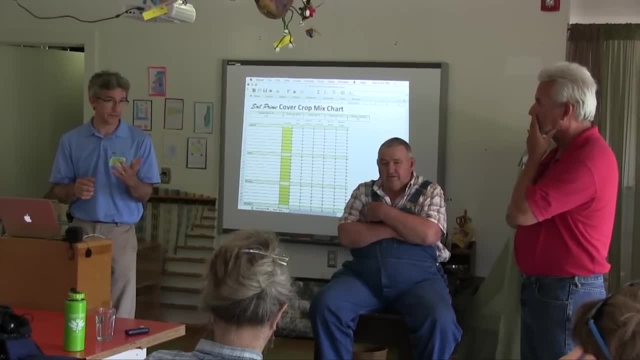 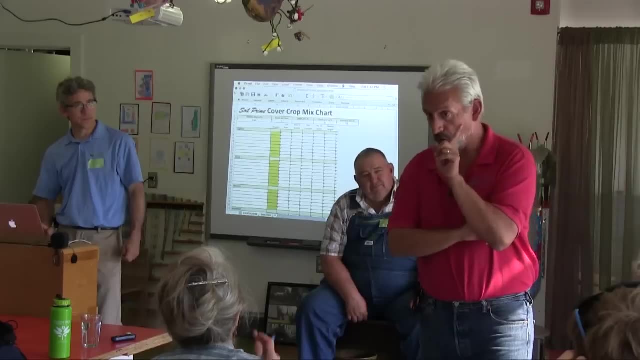 I could actually calculate nitrogen based on that too, but it's a real iffy number. And let me share something with you. Well, look, the resource goal of this farm. this farm has been used: heavy fungicides, insecticides, all the sides right. 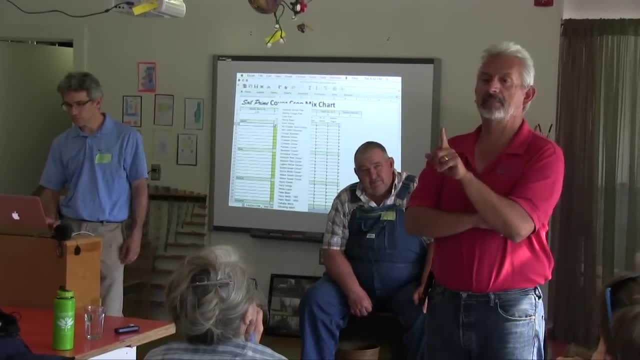 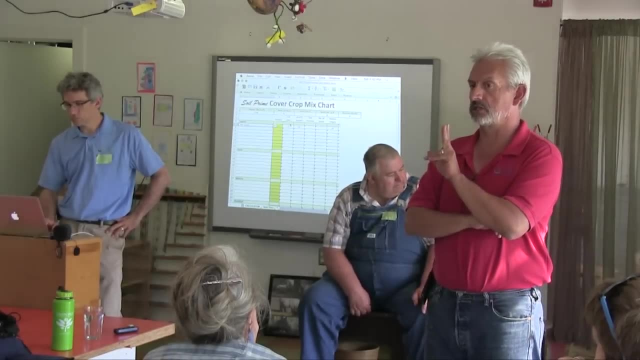 No cover crop, No cover crop, And the soil is absolutely had been nuked. Their main goal- correct me if I'm right or wrong, Pat- is to bring soil restoration: Two seeds per square foot, Two seasons of cover crops and then going to start it into the rotation, correct? Yeah, and it's always going to be soil quality first. Yes, We understand that's the path. Their goal is to do it from a soil health perspective. So we already have a five to seven day weight mix. They're going to go ahead and plant a summer mix into the cool season mix. okay, 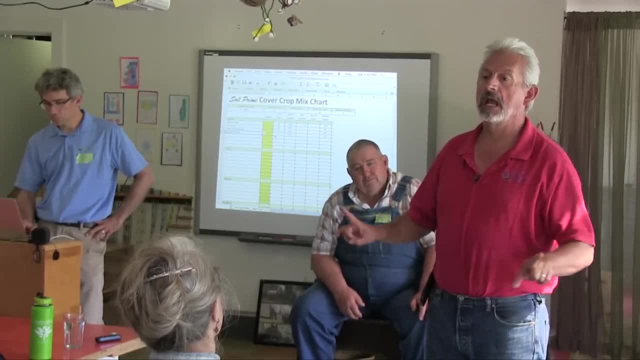 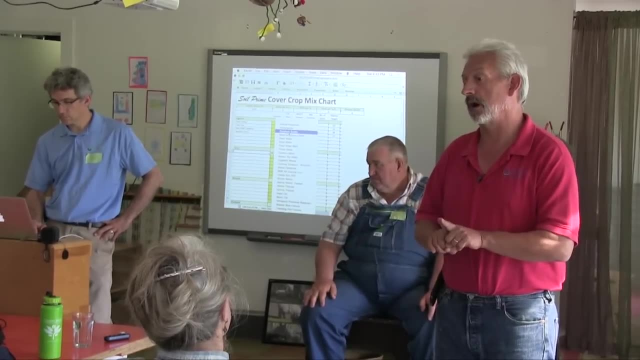 So what we want out of this mix is we want to build a lot of carbon, and it's going to have to deal with the heat, and we want to bring soil restoration. So that mix is going to require. So one of the things, what's one of the things you would think about right off the top of the bat. 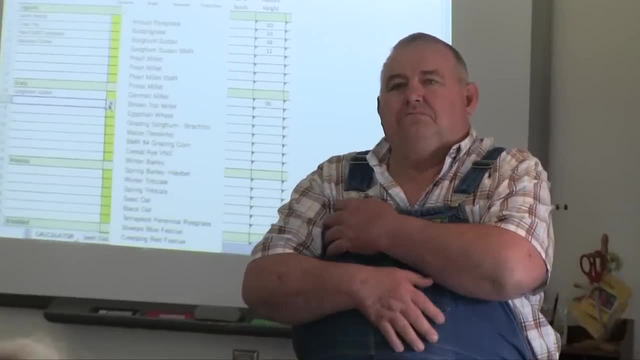 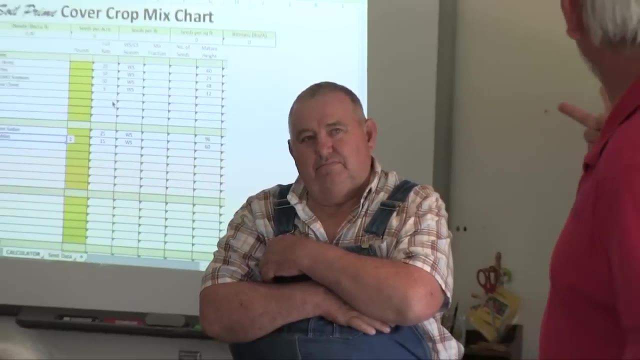 I want three legumes. What would you say for summer mixes, at least at the minimum? Cow peas- Let's do some cow pea. Sun hemp, Sun hemp. How about a little bit of soybean? Do you think soybean would be? 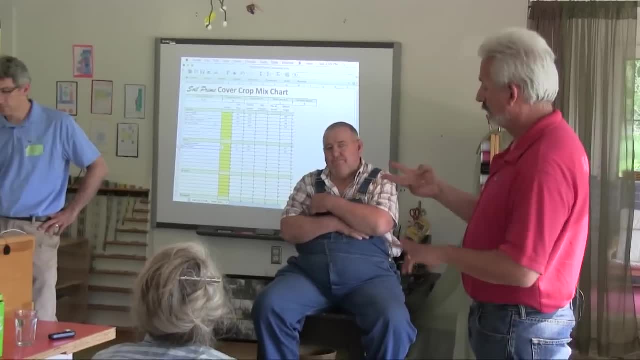 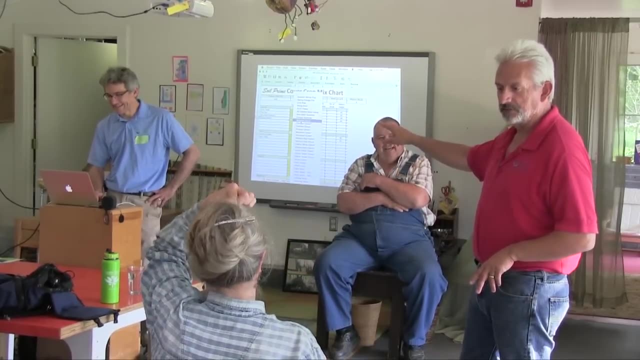 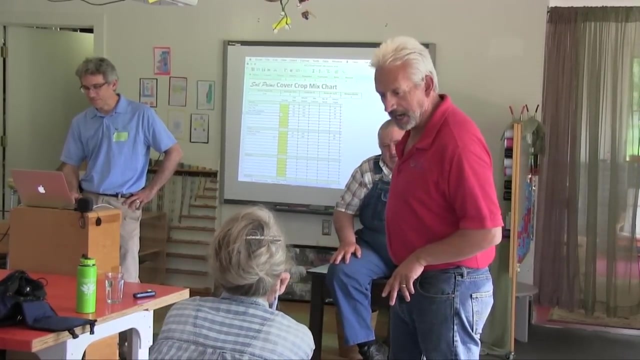 Soybean. Soybean's cheap, Fairly cheap, So he's going to put, we're going to huh, Those two must know each other. Oh yeah, They're dad and son. I know He keeps him in check. Yeah, right, Or vice versa, I don't know. Okay, so we got three legumes at the minimum. Why do we like sun hemp Warm season? It's a warm season. It creates huge amounts of biomass. I want it to feed the heavy carbon mix that we're going to put in there. 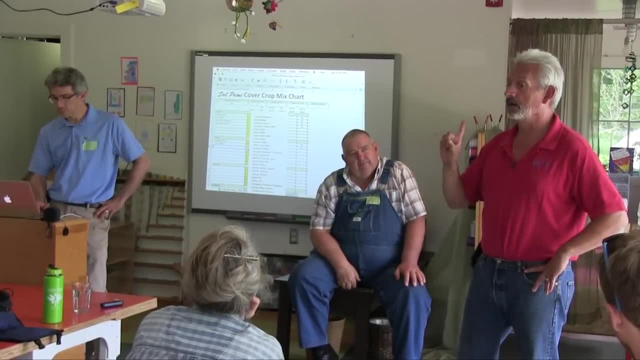 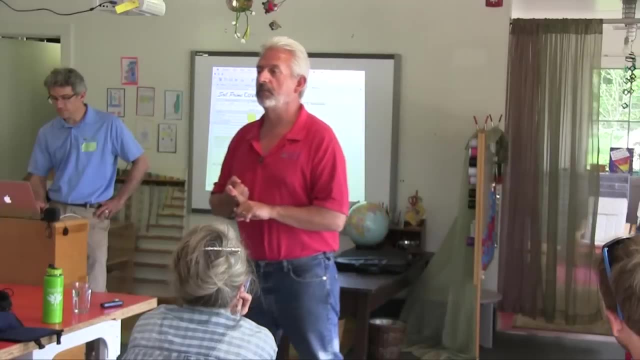 It can tolerate the heat. Okay, so we're building organic matter. So how do we build organic matter? It's okay. Okay, so let's put some. I want something that's kind of a little drought resistant. Let's put some milo out there. 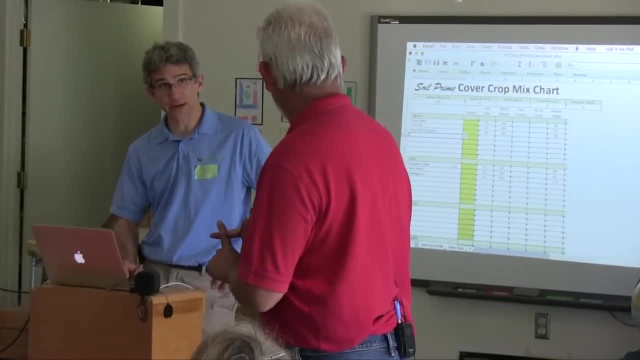 Some grain sorghum. What do you think about that, Jay, The sorghum's sudangrass? Sudangrass, Sudangrass. Yeah, We can put them there. I like that. What Pearl millet. 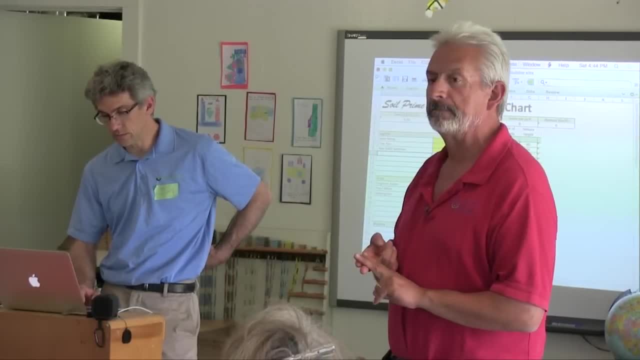 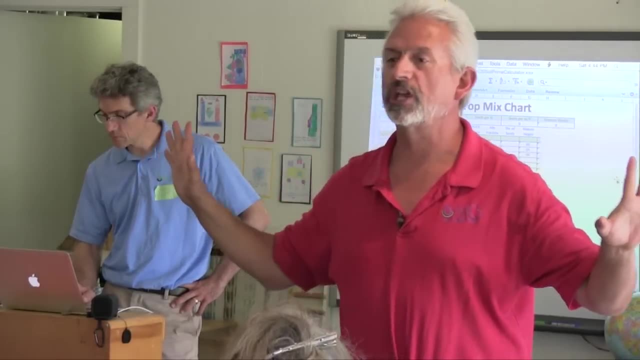 Pearl millet: Yeah, the regular sorghum's sudangrass. Yeah, we can do that. And what else can we put? Sunflower? Oh yeah, Let's put some sunflower. That's beautiful. Who said sunflower? 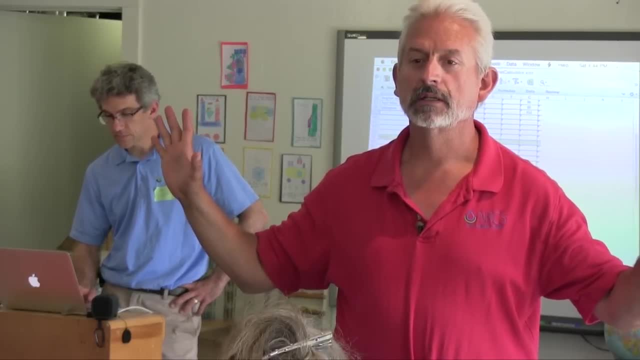 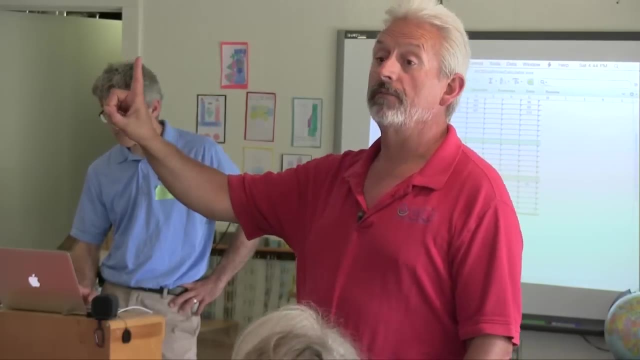 I did. You're a beautiful man, I love it. He cheated out of his little description. Yeah, let's put some: Ah, you cheated, I love that. Yeah, You're a student, right. But I love, let's help the pollinators while we're out there. 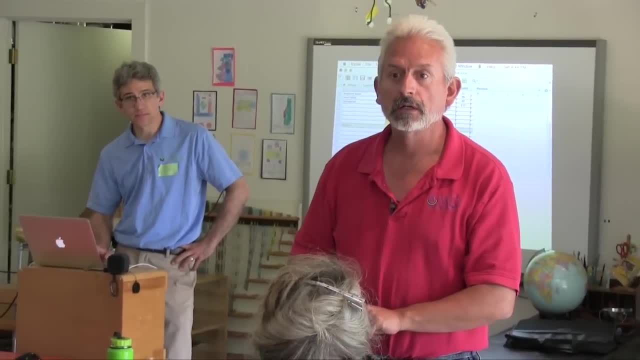 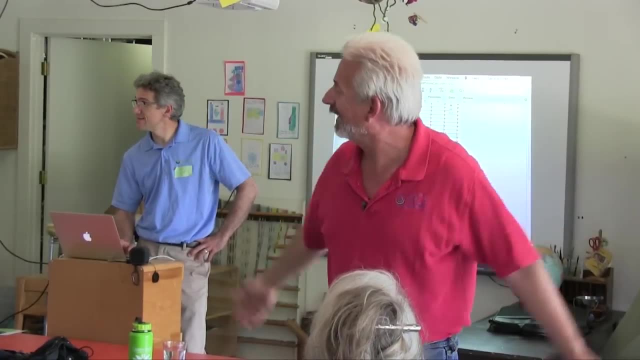 There's nothing wrong with that. What about that one? Which one do you? Which one Forage? You want a forage, Forage, Forage, Forage. What's that? I don't know all of them. It's a farm scaping plant. 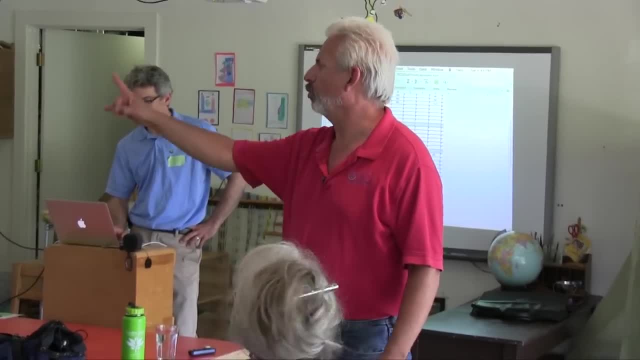 It's a bioaccumulator. It's related to a phacelia. Ooh, Is it summer? Can it handle the summer? It's summer. I don't know how it would compete in that context. It's a summer crop though. 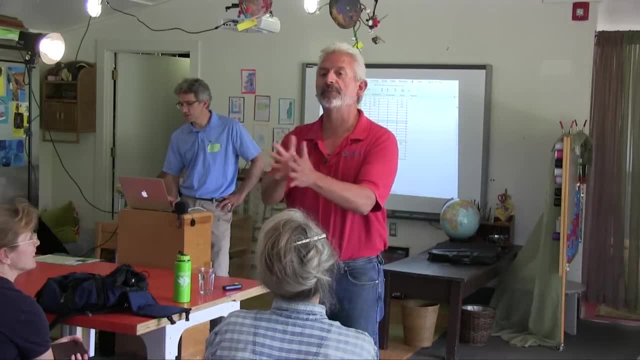 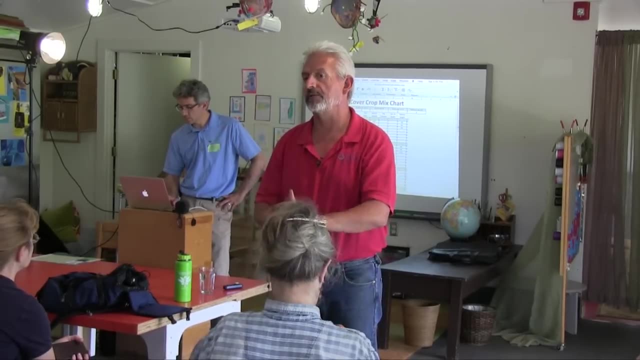 But it's okay, because what do we want from? what do we want from this cover Ecological memory? We want the architecture, we want to prime the biology and we want a lot of lignified material. I want hemicellulose, all these lignified strong carbonaceous material out there. 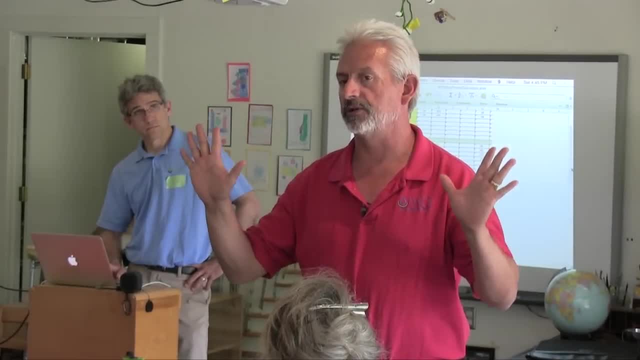 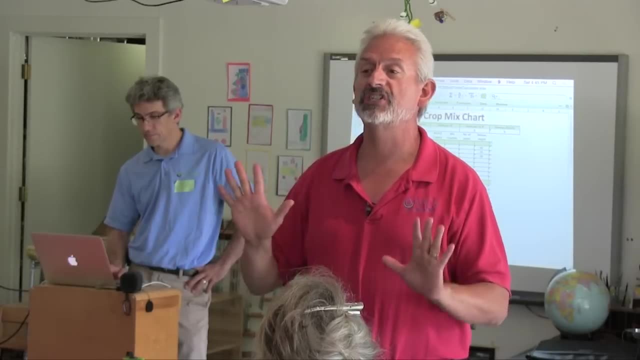 So that's going to be when we have that biomass. if I build 10 to 12,000 pounds of biomass, only 35% is going to go into organic matter. What happened to the other 60? some percent Glass? What happened to it? It went off of CO2.. Eight percent feeds the microbes. 35% actually goes to humic and non-humic to build organic matter. The rest of it goes off the CO2.. Okay, So where you're going to build a lot of organic matter is through the carbon pathway through. the root. Okay, So we got read that out. so what we have so far? We have sunn hemp, We have cowpea, We have soybean, We have sorghum, sudan pearl millet, sudangrass, and let's put some sunflower in that. 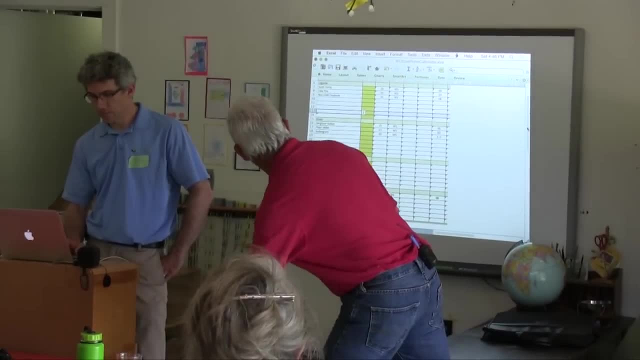 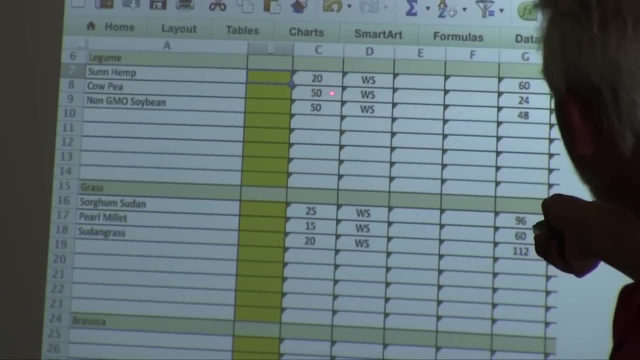 He's got sunflower. You see how he's got it. Now look at the calculations, what it does right off the top of the bat. Okay, notice, do you have the full rate On the calculator? that is the full rate. 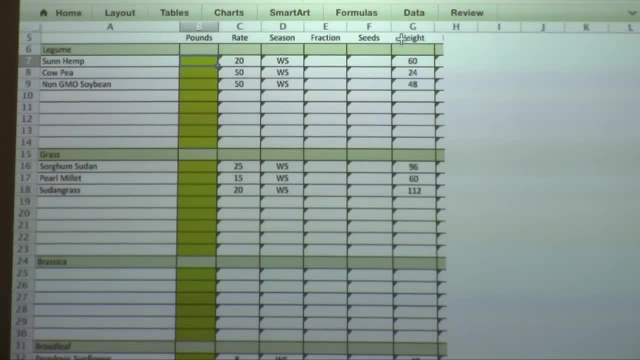 And then we're okay. now what he does in his calculator. it'll show you what the full rate is. Okay, The other one does too. We don't want to use the full rate, Why not? We're growing a mix. 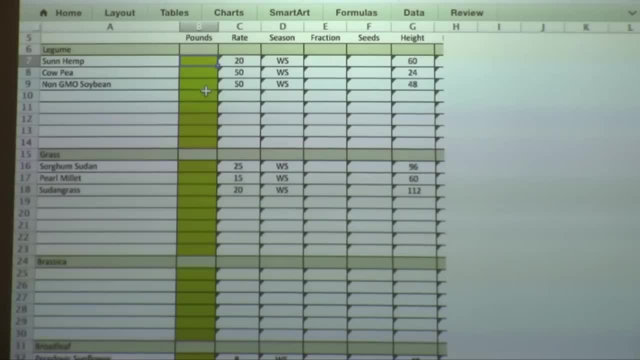 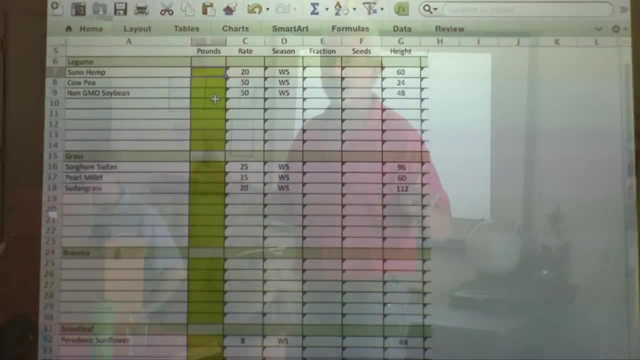 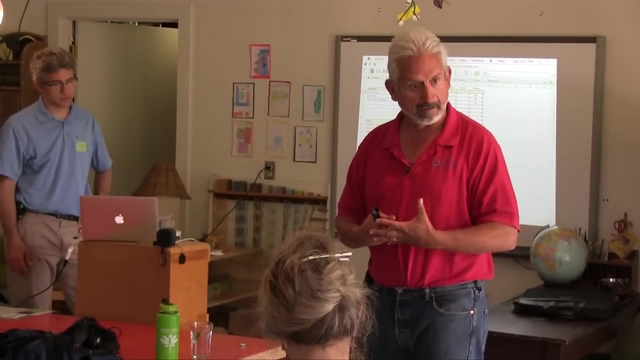 We want to let everything manifest itself and be able to be part of that mix. So what you're going to do is it's as much as art, Pat, as it is a science. This is art. Farming is an art too, but we're trying to just bring as much science into it. 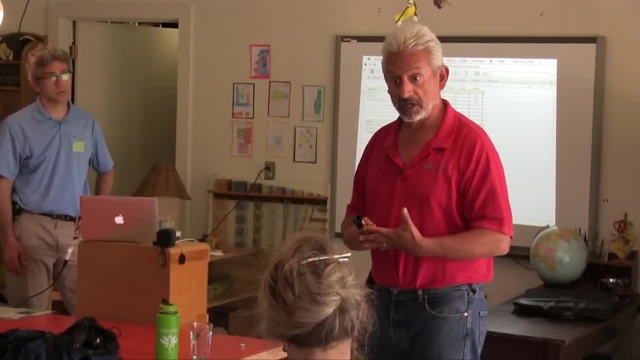 Okay. And experience: Do not dismiss your experience. Okay. One rule of thumb. One rule of thumb that you can use when you're making a mix is: you take the number of ingredients and you divide your full rate by that number as a starting point. Yes, Did you guys get that? So if I have seven-way mix, you're going to divide it seven ways. the full rate? Yes, Pat, I would always put a small amount of buckwheat in, just for the biodiversity, just. 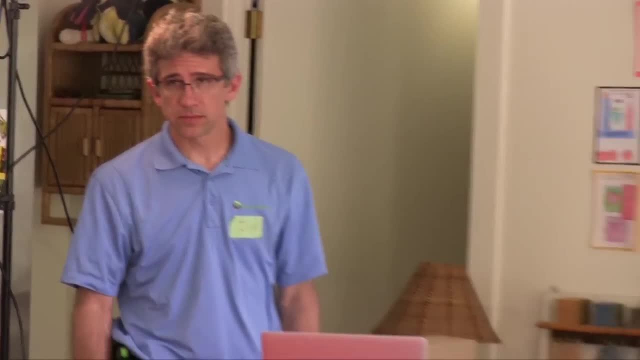 for the insects. Beautiful, I have no problem with that, Absolutely. I love buckwheat. The only thing you've got to remember: if buckwheat germinates on you, it's not going to germinate on you, It's going to germinate on you. 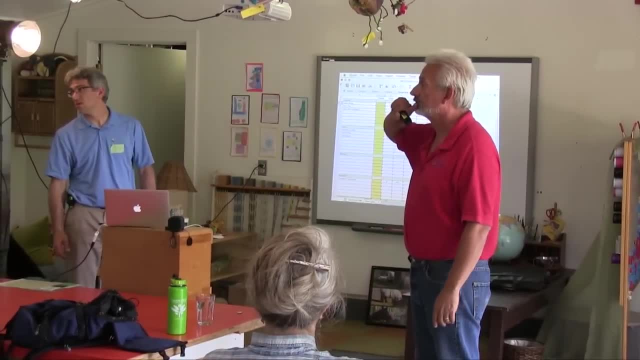 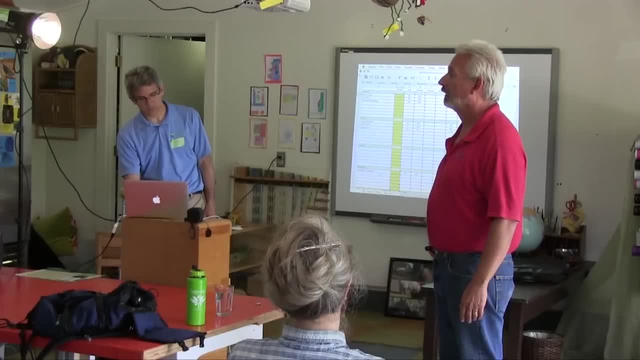 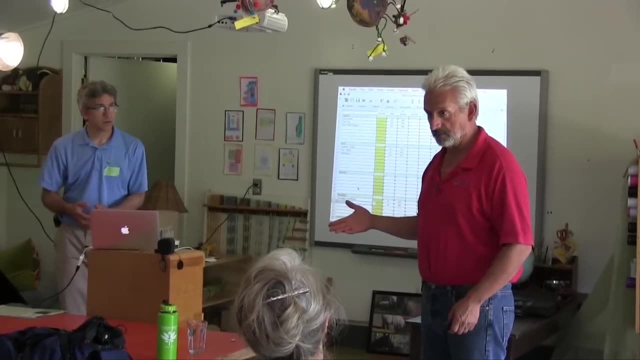 Beautiful. I have no problem with that, Absolutely. I love buckwheat. The only thing you've got to remember: if buckwheat germinates on you over there, it's going to be a seed. It can become a weed issue. 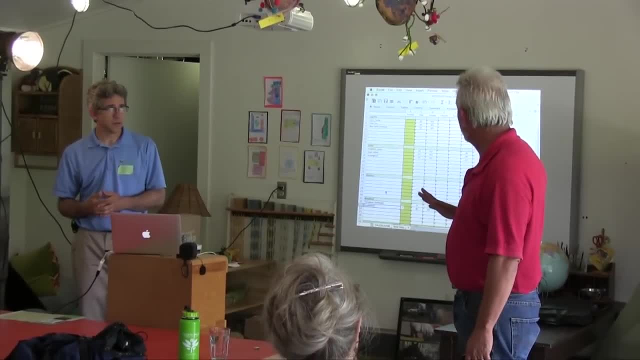 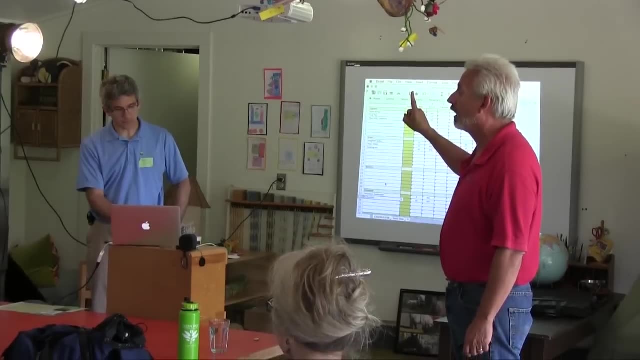 But I don't — but you know, I think again, I think we'll be fine. Okay, So we got sunflowers, We've got the buckwheat. Anything else, Pat Rocco, anything you want, Anybody else have an idea they want to put out there? 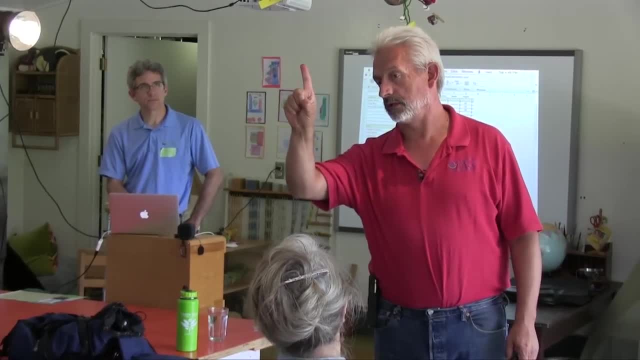 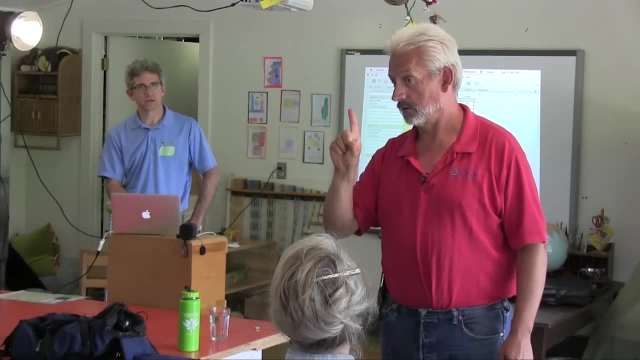 Out of town Country, Afalpha is a cool season. It's a cool season And a perennial, so it's difficult to terminate. Yeah, I don't want to till that ground if I don't have to, Because to terminate it, these guys are organic. So a lot of these annuals we can either terminate it. Afalpha is hard to terminate, Okay, because it's got a massive taproot. Be careful with your perennials. But I love afalpha though. Good, cool season. What about the phacelia? Phacelia? Phacelia is a cool season. It's a cool season and planted now will not emerge well, So it would be hard-seeded and wouldn't come up until the winter. So that's generally what you're going to see. 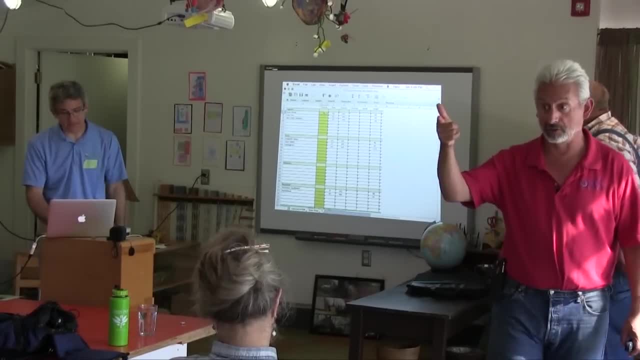 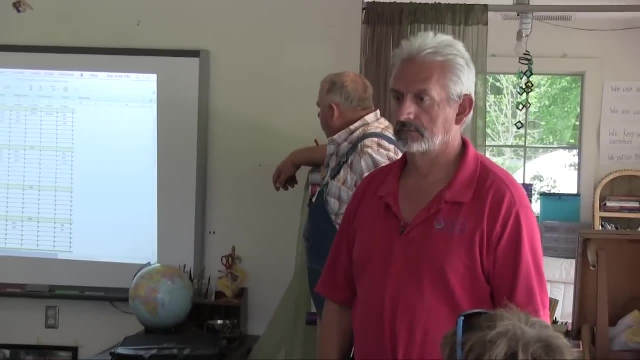 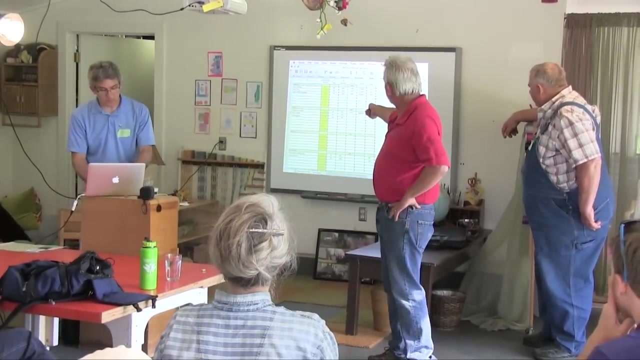 And And the cost of seed. We take that into consideration all the time too. We don't want it to be too expensive. You know why You guys won't do it. It's economics too. Notice how he did from the 20.. He went to 5-pound sun hemp. Regular age for cow peas at a monoculture rate is 50. Put 10.. Soybean regular is 50. Put 12.. Sedan grass is 5.. Look at the number of seeds. Do you know why he went to only 5 pounds? Look how many seeds in a pound 4.. Is that 400,000?? Yes, 400,000 seeds. Do you guys remember the magic number we want per square foot? 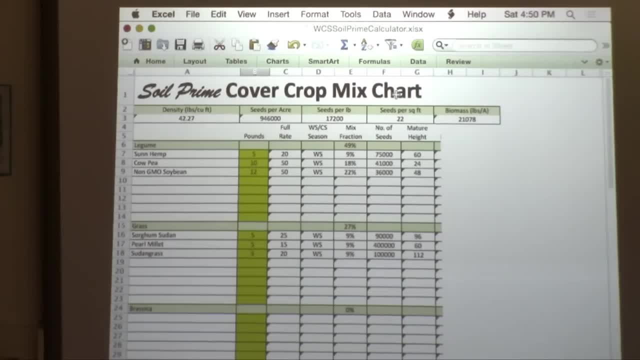 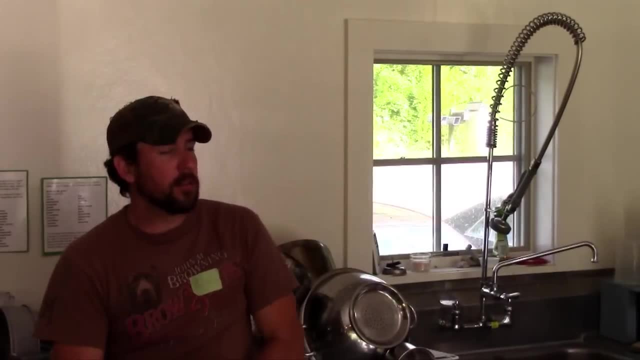 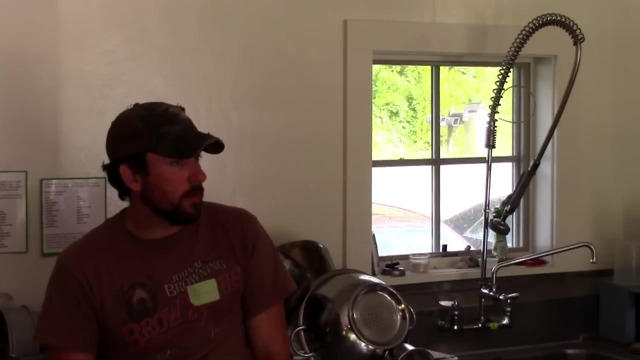 Oh, you guys are such incredible students. Good for you. Yes, When do you mow it? When do you transition into fall? I don't understand. if you let it grow all season, It reaches peak biomass. Yeah, yeah, Is it, you know? and like out here this afternoon, I mean, the peas are flowering, but the veg isn't quite there. 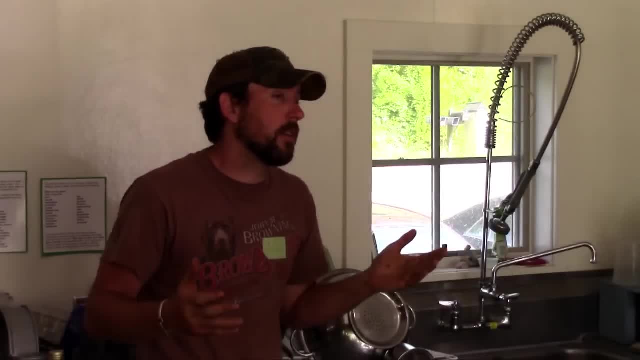 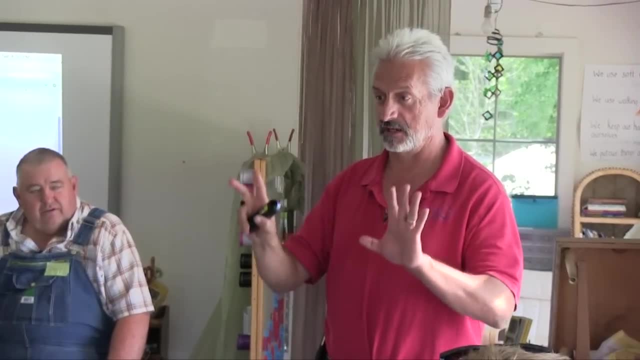 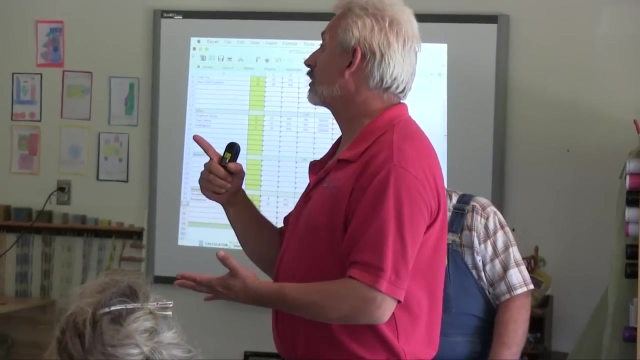 Is it a Good, good question? Do you see what Rock was asking? Is it whoever goes to seed first? Ah, excellent question. If I got cereal rye, I personally watch cereal rye if it's in my mix, Do you know why I watch like my mix in my garden? I got crimson clover. I got some veg. I got cereal rye. 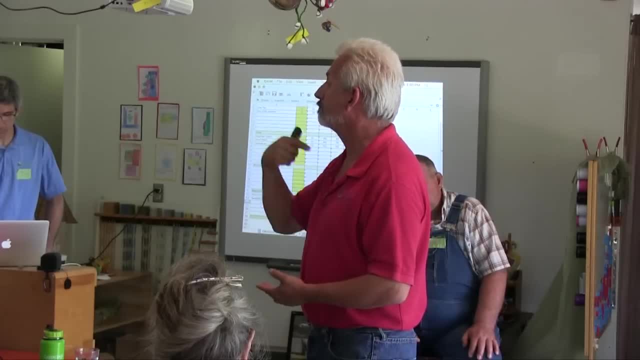 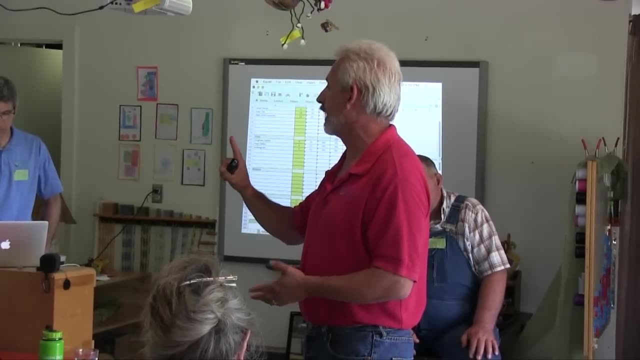 I have some with two or three other mixes. You know what I focus on. I focus me personally on my cereal rye. Why do I focus on my cereal rye? I want to roll it and I know when cereal rye is ready to terminate, at that dough stage and all those little pollination. I focus strictly on the cereal rye. 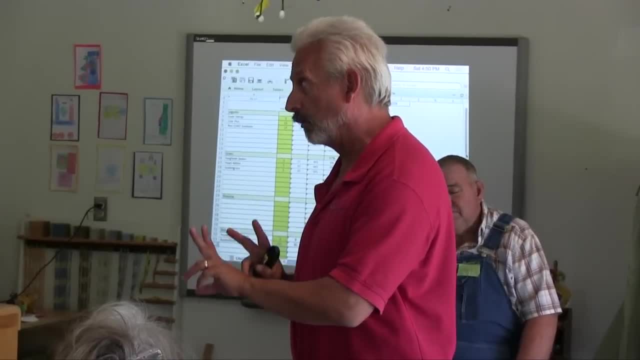 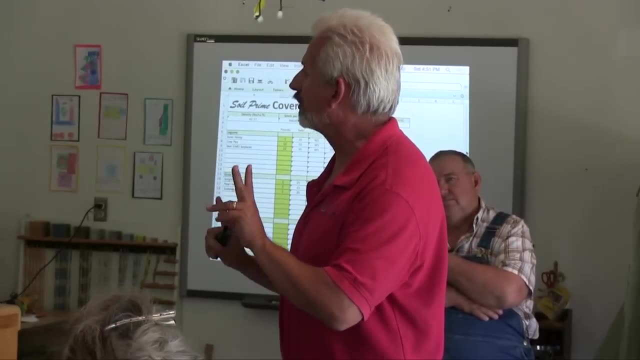 I'm going to get my nodulation what I get, But I don't worry, I don't stress about that. See, I'm not like a bunch of people that stress: well, I don't get enough. No, Build a biology, we'll get the nitrogen. Let me give you an example: Lymatodes eating bacteria. through predation you can get anywhere from 17 to 116 pounds of N, So I focus on the cereal rye. Now, if you want max nitrogen but you don't have cereal rye, you might want to focus on the veg. 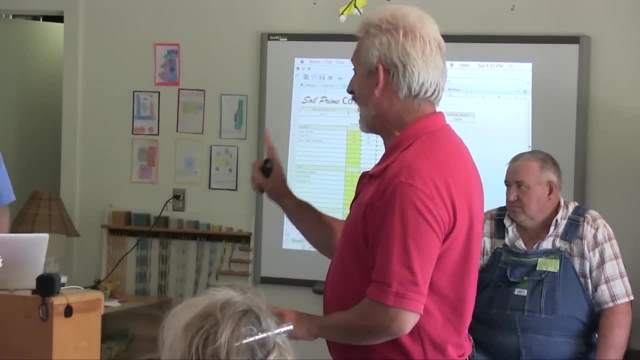 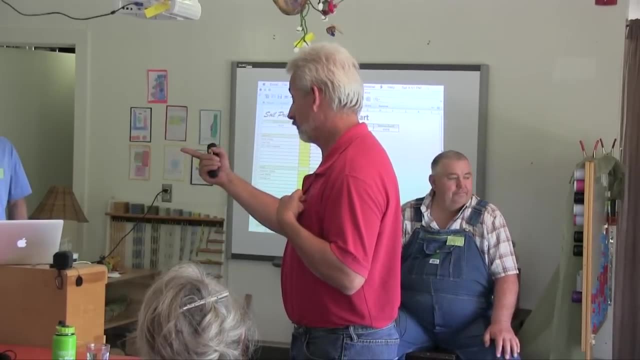 Depends what species and what your goal is going to do. That's what it comes down to. So my goal when I want to roll and cereal rye is the thing I'm going to watch, I watch that first, Because that's what I care about. Because it has go ahead. What's the goal for your garden? My goal is: I want great weed suppression. I want good weed suppression. I want to build organic matter, But I want great weed. What's our biggest bane for all farmers, especially organic? The weeds. So if I don't have a good cereal rye out there suppressing the weeds, it's going to eat my lunch And I'm lazy, I do not want to be out there weeding. So it's all the function of what your goals are. 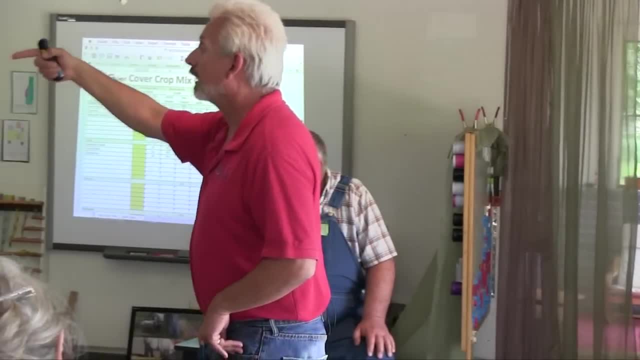 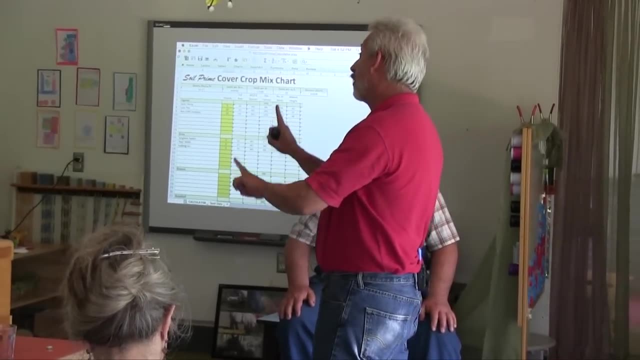 So you watch that indicator species And then you terminate it by then, Because what we're going to do is we're going to have that summer mix And they're going to come in with another cool season mix. Now we're going to have to design a cool season for your following crop. 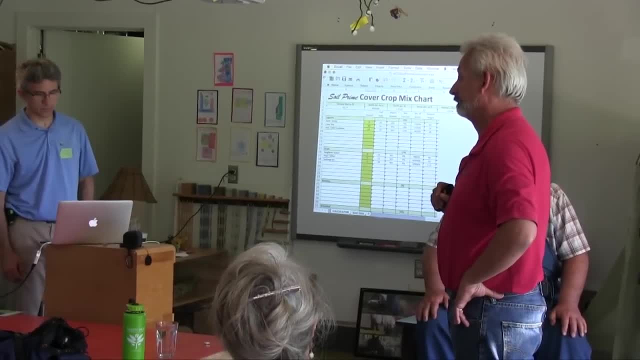 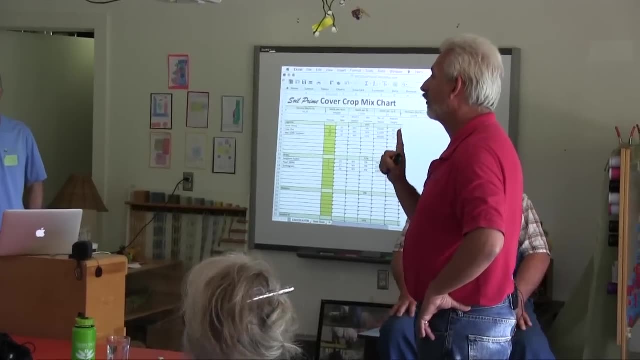 What is going to be your following crop in the spring? Pat, Very, We're going to do tomatoes and sweet corn, for sure. Squash peppers, it's going to be mixed vegetables, basically. Aha, So what's a common thing that you would do? if it's going to, we know it's going to be tomatoes and vegetables. 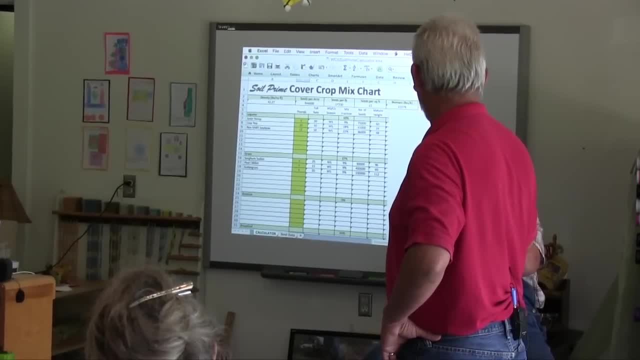 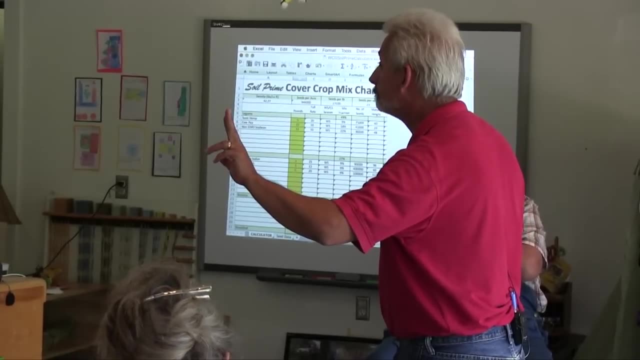 Lots of legumes, Lots of legumes. And what else? Cereal rye, because I want wheat suppression, because the tomatoes are going to love the cereal rye. What else did you talk about? Sweet corn peppers, The peppers, all those grow wonderful under cereal rye. 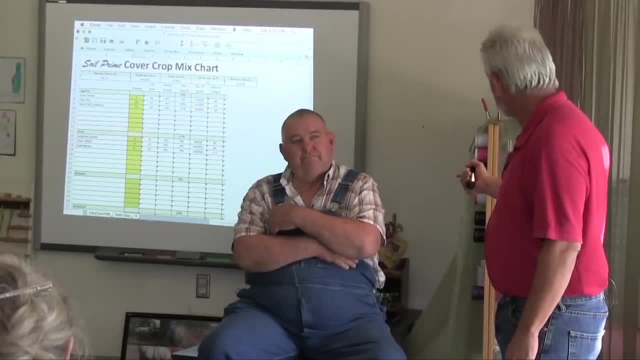 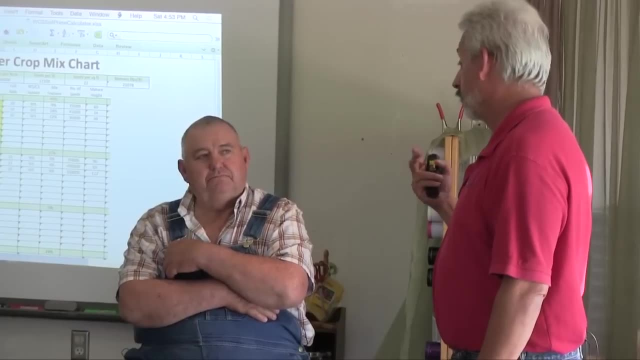 Would you agree with that or no? Yeah, I would keep the rye reasonably low. Yes, because you're going to do a mix. You're going to do a mix, So I don't want to see that. over 35 pounds per acre. 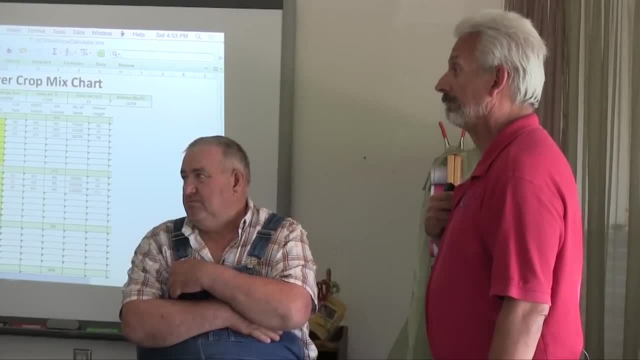 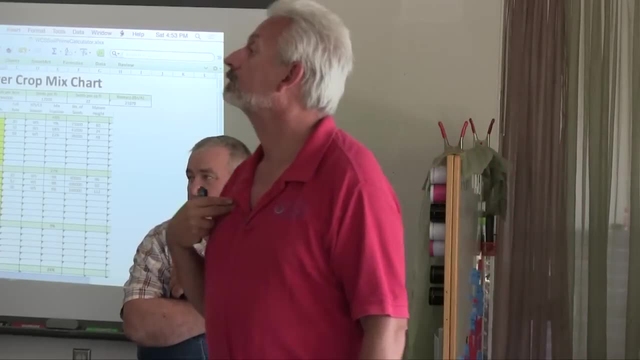 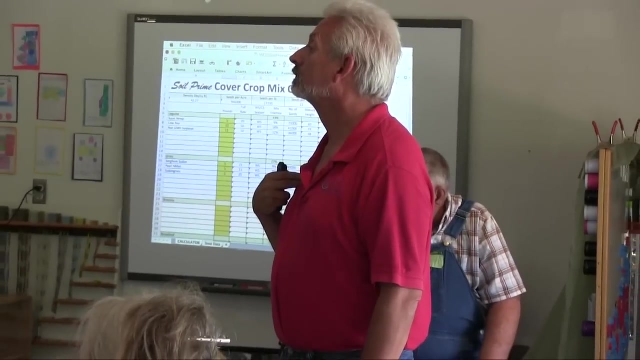 Do you agree with that boss? Yeah, So you're going to put the legumes in the rye and the grain for the wheat suppression? Yes, Yes, Got it. And what Ron Morris does- have you ever looked at that? is he plants the he actually. it's probably more work than you want to do, but he actually plants the legumes in the actual planting zone and has the grains on the edges. 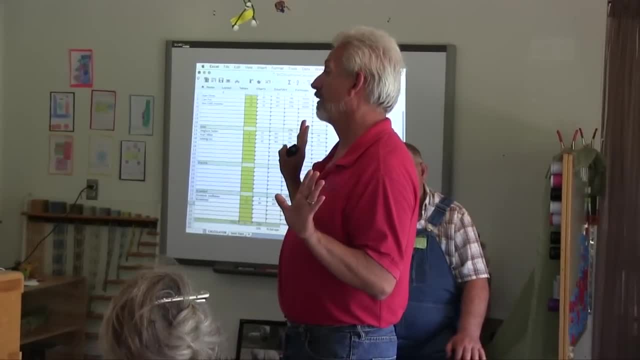 Yes, you can do that. You can do that. But you can do the fundamental mix: roll it down, you can plant into it, you can roll it down, and then you can come back and seed that. There's nothing wrong with that. 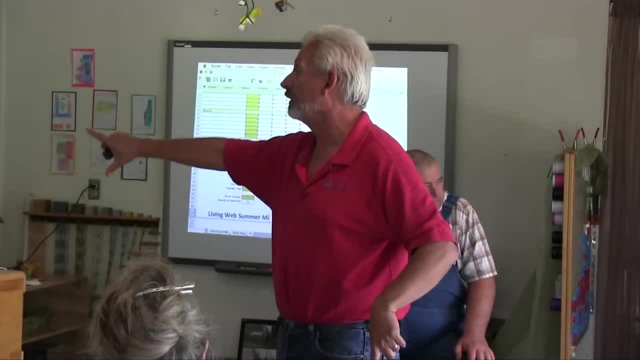 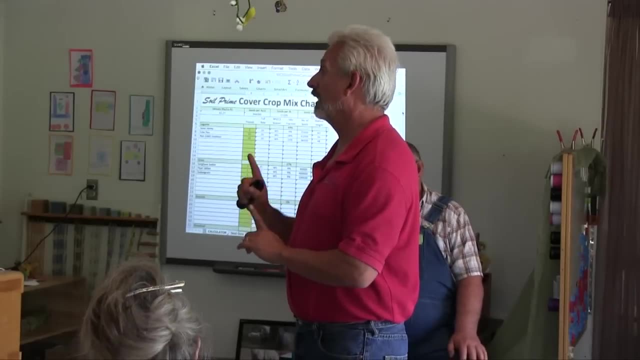 Nobody says that you can't come back during the summer and put a legume right in there, But the thing is I want to do is I want to get great wheat suppression because you're organic And I don't. if we can reduce the tillage as much as possible, that's what we want to do. And we want something that's easily terminated with mechanical rolling Right. Yeah, totally Totally. My whole goal is to reduce your tillage, build your soil biology. so this summer mix is going to be wonderful. Then we have to design a winter mix for you to come in into your crop. 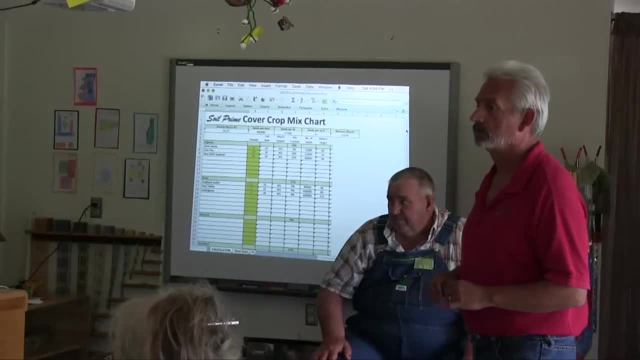 Okay, Yeah, one question. Yeah, You might have mentioned it because I had to go away for a little bit. I know we're going to do it, We already talked about it, But what about making sure you got mycorrhizae out there? 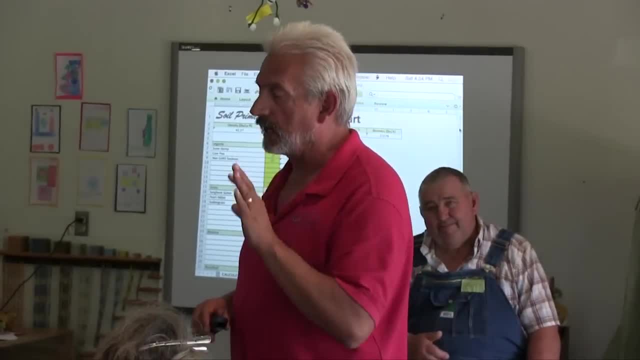 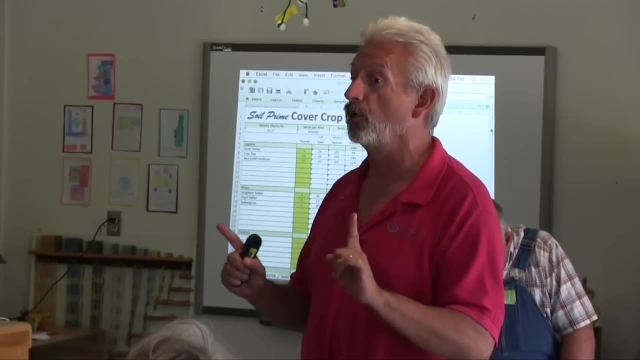 Should you inoculate the seed at least once with mycorrhizae? Yeah, here's the thing. I have a great. there's a guy called Soil Smarts. He does probably one of the best seed inoculants. That soil you're going to see out there is absolutely nuked. 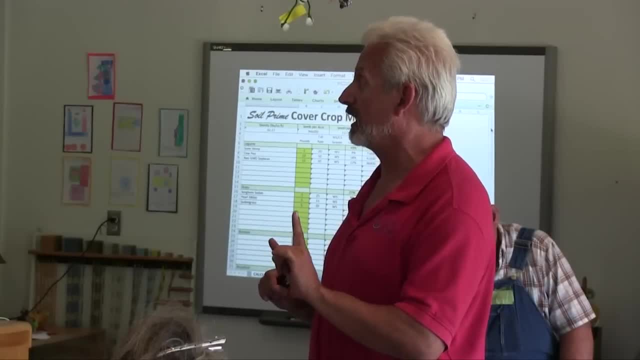 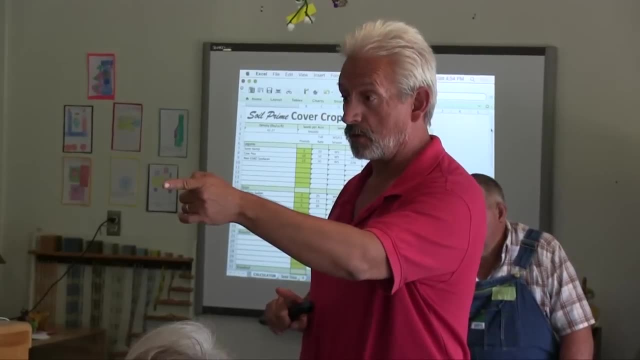 I think we can do it with a mix, But for 25 bucks an acre only one treatment, it may be worth to go do that. mycorrhizal inoculants: Yeah, that'll be a good one. Mark, you had a question. 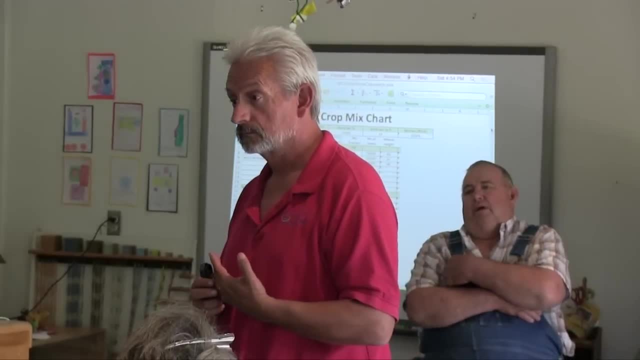 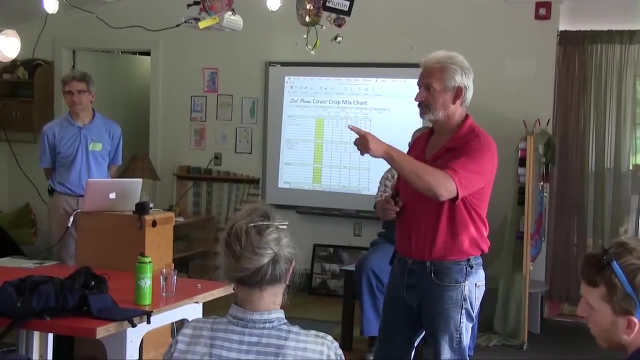 Yeah, I did So. you were advocating using a lot of cereal rye for weed suppression. Yeah, What are your thoughts, or all of your thoughts, on how that affects your nitrogen for the cash crop? Ah, good question, Do you see? 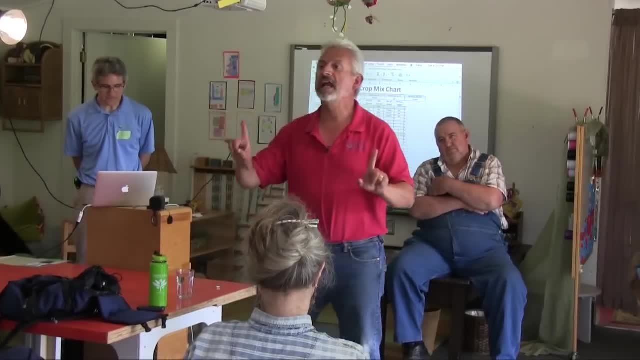 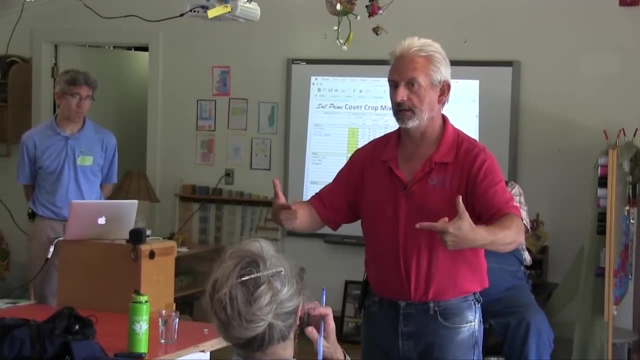 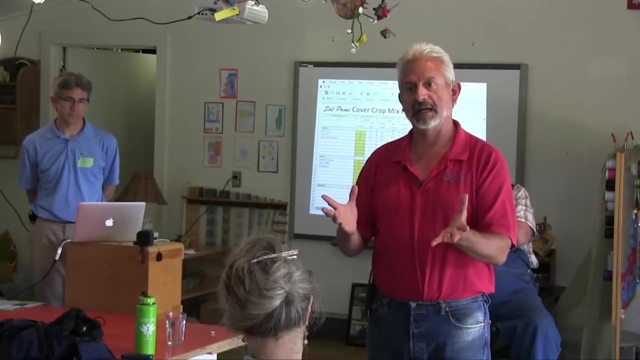 Here's the kicker: When you incorporate the cover crop. this is very important. There's a difference between lay it on the surface and incorporate it. If you incorporate it, you're going to tie up all the nitrogen in your system Because the microbes. what you've done now is you increase the surface area. 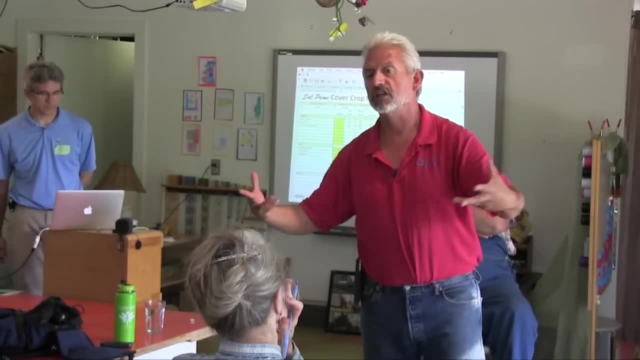 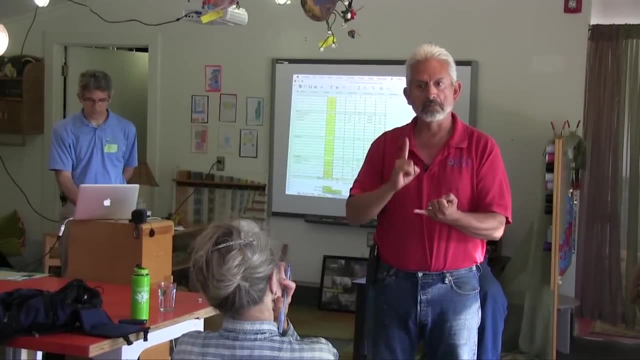 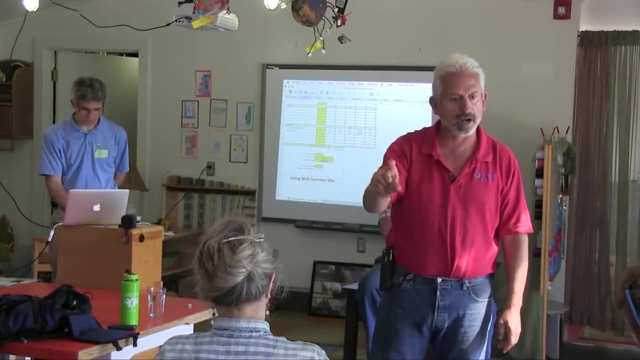 You incorporated all the vegetation, You're going to tie up nitrogen and you're going to have problems with the tomatoes. You're going to have nitrogen deficiencies. Let's make it very clear: Microbes are the first feeders. They have done radioisotope studies and they follow N15 all the way through. 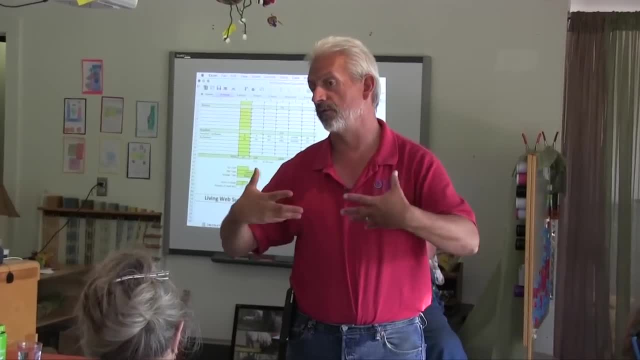 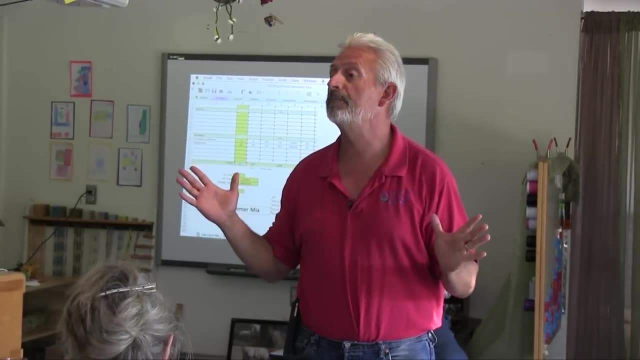 And it's microbes get the first nitrogen. They did chemical fertilizer display and they threw chemical fertilizer out there. Only 40% of the chemical nitrogen ever reached the plant. What happened to the other 60%? It went to the microbes. It went into the complex pools. 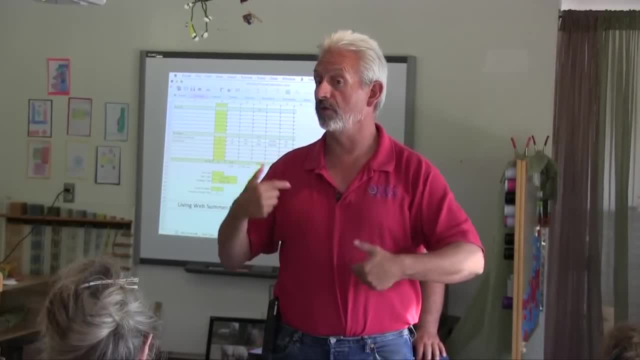 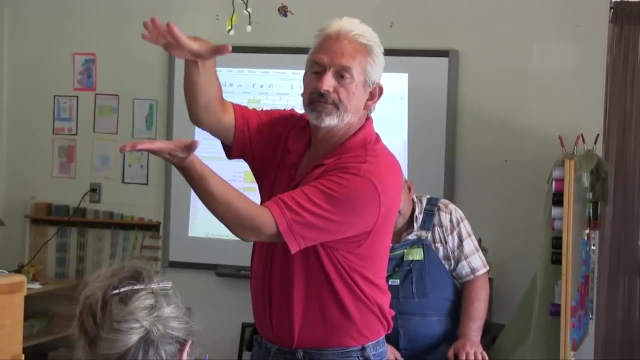 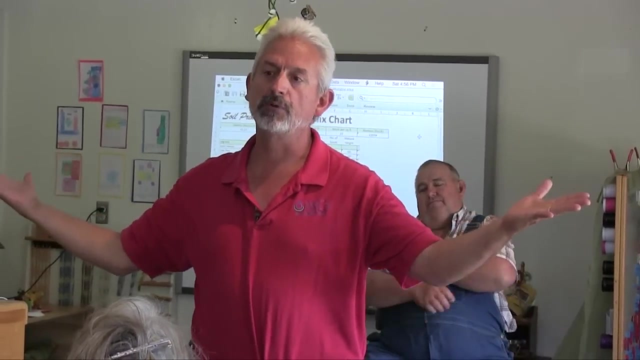 My point is: microbes are first feeders. So if you incorporate that cover crop, you're going to tie up nitrogen With this system. you're laid on top of the surface, You're not incorporating it, So the regime changes. It's going to be attacked mostly by fungi. 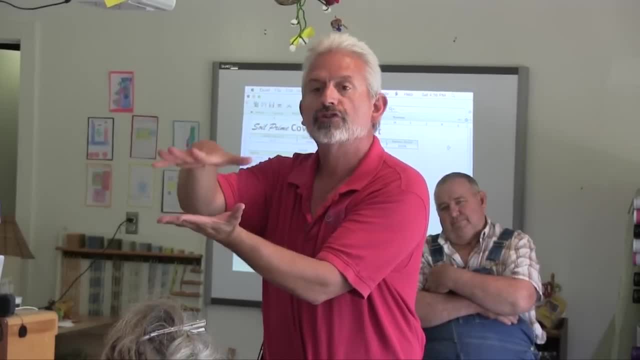 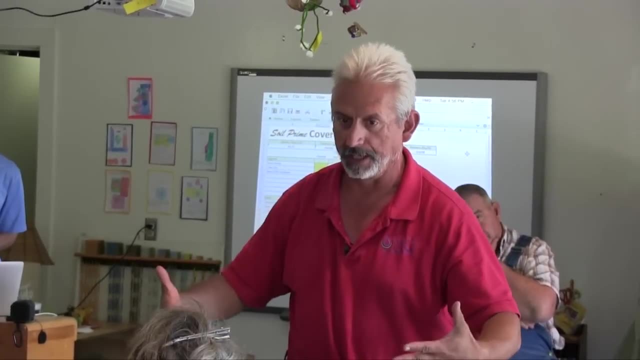 Fungus- Saprophytic fungus- on top of the surface. So you're not going to rub the nitrogen that you think you're going to rub if you lay it on top of the surface Versus incorporate it. If you incorporate it, you're going to tie up all kinds of nitrogen. 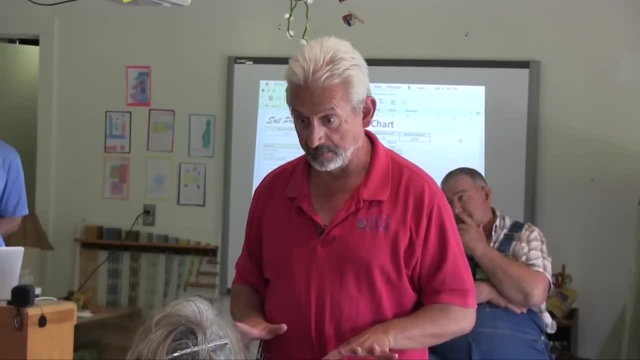 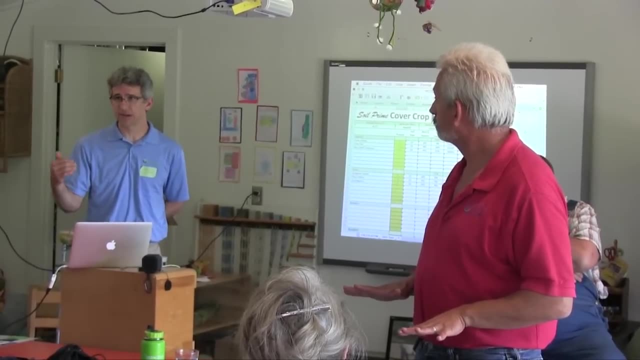 But when you roll it, that's not an issue. Okay, Everybody with me. There's another aspect to that is that it's not a monoculture of rye, Yes- Which, if allowed to head out, will have some nitrogen deficiency because it's holding it. 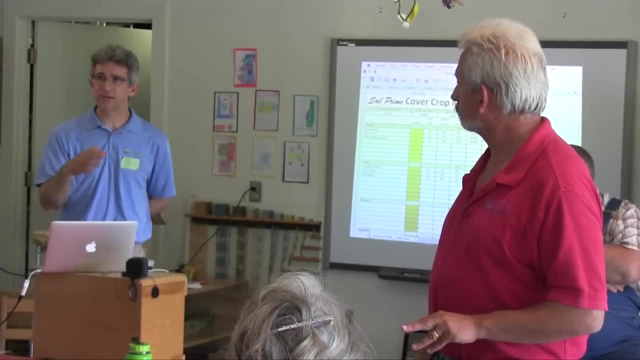 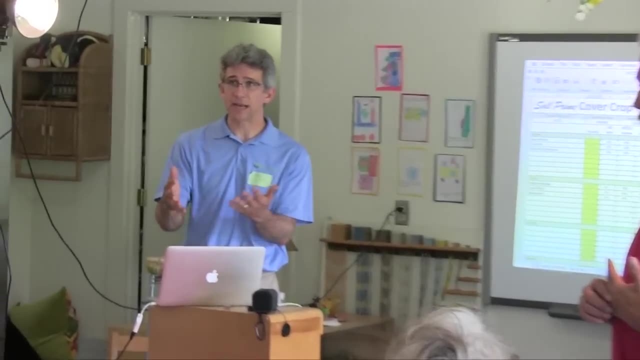 It's bound tight. So now that we're adding a succulent legume in the cool season mix that aids the decomposition of the cereal, whether it's rye or barley or anything, And that makes that more available or more readily available to the plant throughout the season, 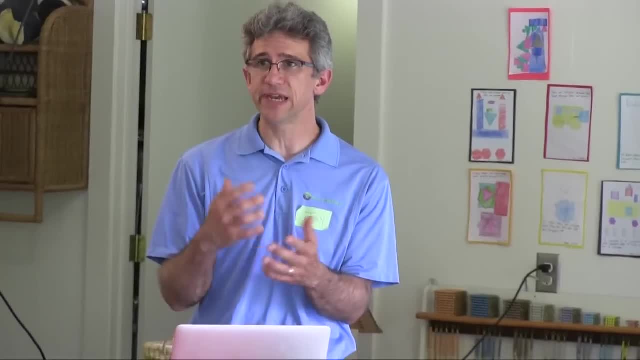 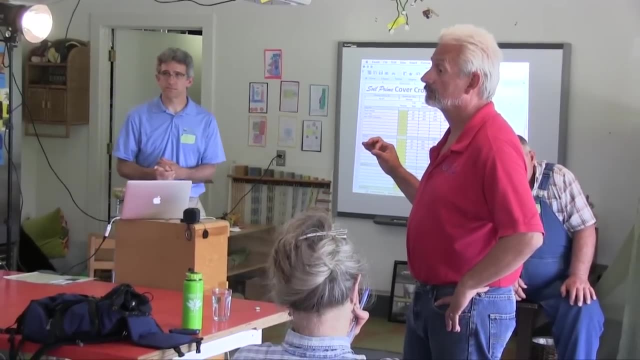 So that's again. the purpose for doing the mix is to alleviate that nitrogen deficiency issue from the cereal. So are you thinking that if you have enough legume or a little bit of rye, like that ratio is right, you won't need to supplement with nitrogen? Right, right. But here's what I'll note, And let me put a caveat to that. Mark That soil is so degraded I wouldn't mind, right by the long tomato plants go ahead and put some fish oil and some other stuff in there to supplement some nitrogen, because it's degraded. That is not a functioning cycling soil. So I would not be afraid to put some compost teas, put some fish oils right by the tomato plants. It won't hurt you a bit. Okay, Because I'm telling you that soil is very degraded. 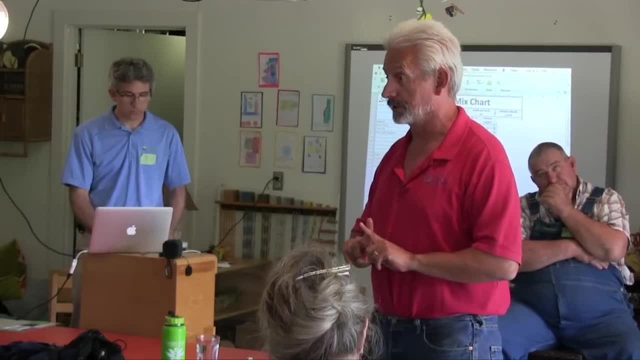 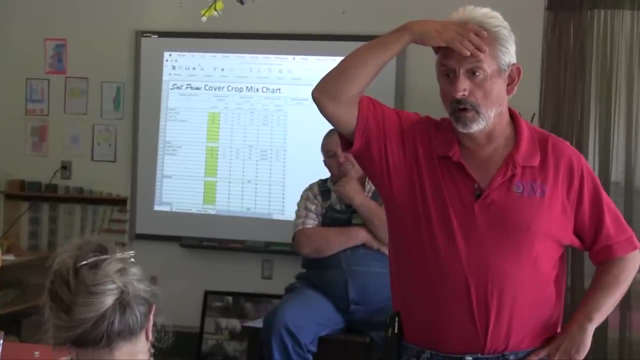 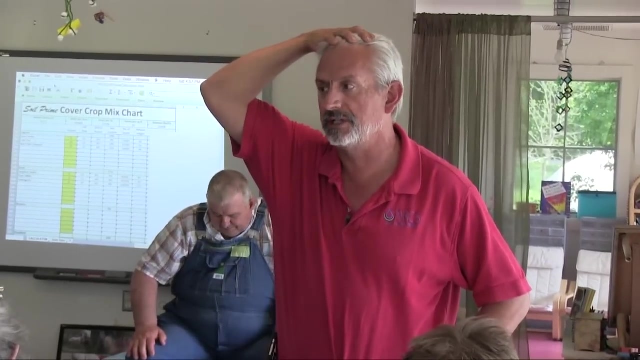 We'll show you how it's been absolutely nuked for years. Good question, Mark, Because they got to understand that. Here's another thing: Everybody write this down, The ones who learn about this. You need to buy the book called The Nature and Properties of Soils, the 13th edition and above. 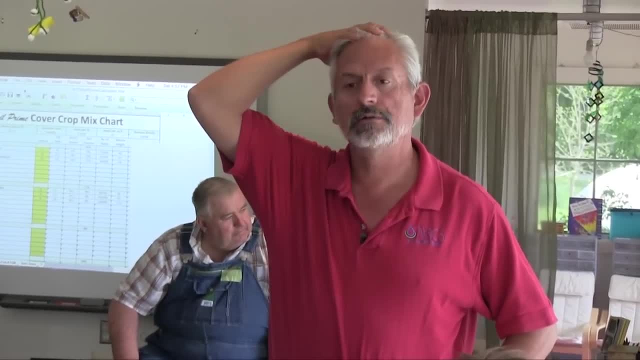 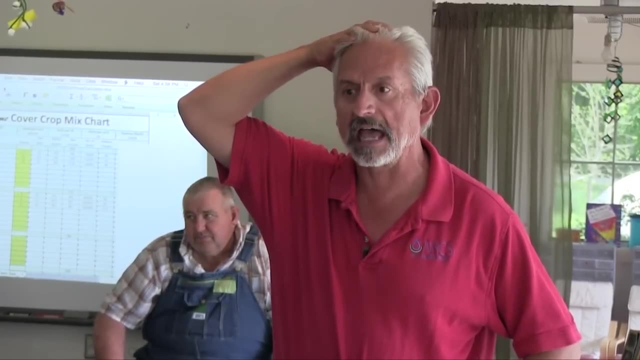 Don't buy the 12th, Don't buy the 10th, Do not buy the 11th, 13th and above. I want you to read the carbon and nitrogen chapter of that whole. That is a basic sophomore soils class. 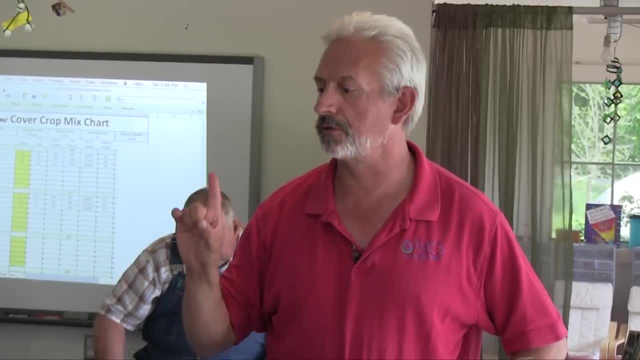 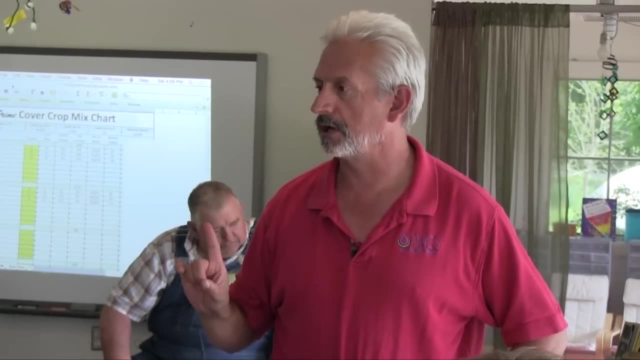 You need to understand carbon and nitrogen ratios or you're going to screw things up. You're going to hurt yourself. Buy that book and go to Amazon and get it for $30, $40 and go to eBay. Some sucker sold that book. 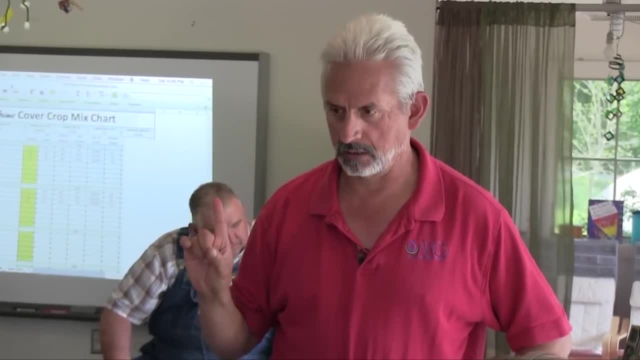 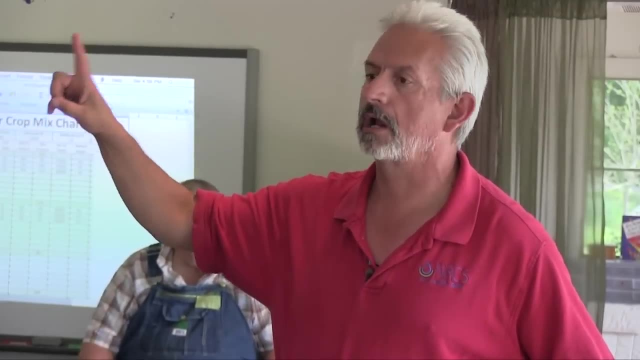 You don't sell that book. You don't sell that book. That's your Bible of soils. You need to have that. There's a lot of other books. If you send me, If you post on the website, I'll post all my reading literature that you need to read. 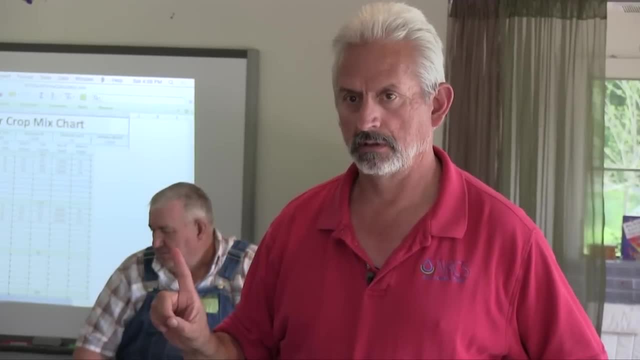 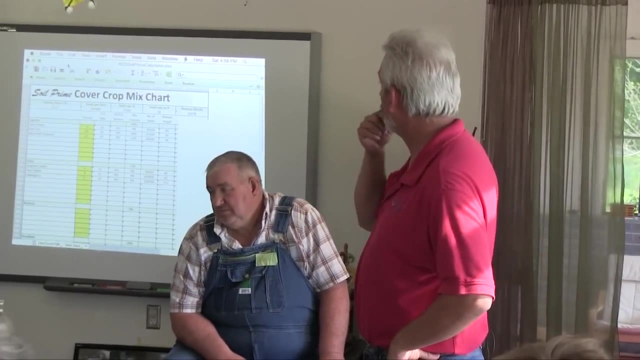 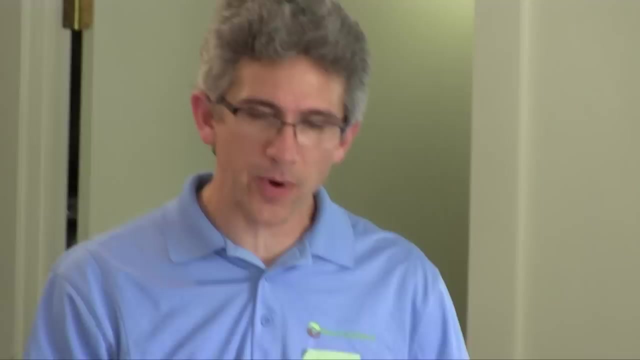 And so ecology and all that. So you become a student, You need to understand carbon and nitrogen ratios. or you're going to hurt yourself Or you're going to cut your fingers off. Go ahead, Yeah. So in the case of this, the summer mix chart, if we look at the mixed fraction, is the other part that we look at. 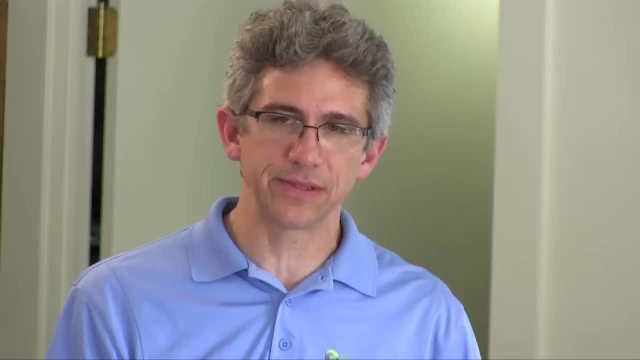 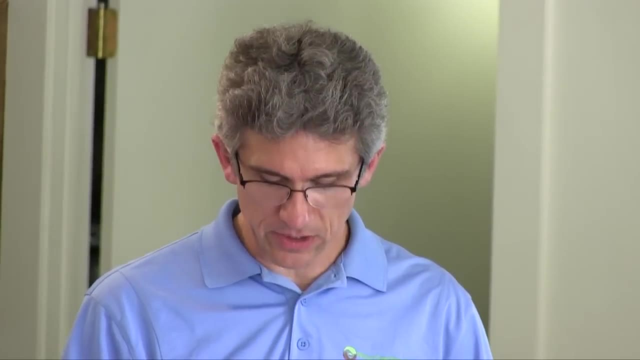 And again, I like to have about 50% of the mixed fraction, being the legume in this case, And we split the rest up. And we split the rest up between our grass and the broadleaf, which you consider a grass In some cases, I just consider it a broadleaf. So we add diversity that way, And the other way is to balance in. as far as seed counts are things that you would consider when you're building the mix here in this case, But a 50% legume mix is very normal and a good place to start and look at where you want to build your mix from. So it's always interesting to look at the different companies that are offering. There are prescription seed mixes- like we at Walnut Creek Seeds what we have, And you can look at what those combinations are and get a feel from that. So the prescription mixes are indeed a starting point where we recommend you start. 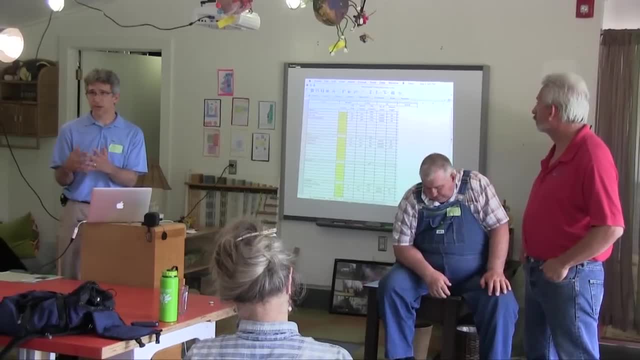 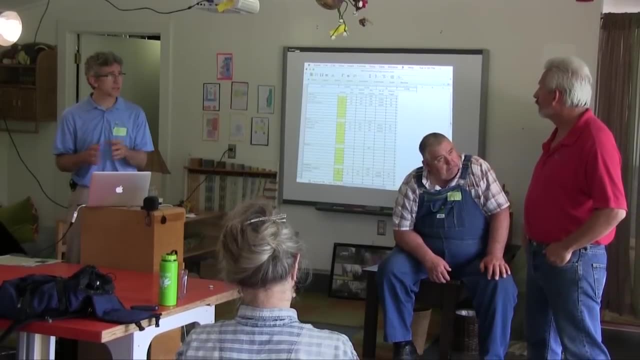 You get a chance to see what the different species are, how to manage them and what kind of performance you get, And then you can decide how you want to change those things or use them differently. So that's the key part- is to look at how you use those in your management. 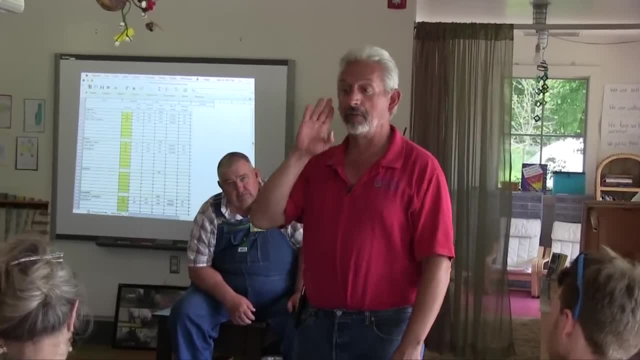 Jay, tell me about the tree. If you don't want to do all this thought process, just say I want a summer mix. Call Jay, They have a summer mix. If I have a cool season mix, he's already got a cool season mix. 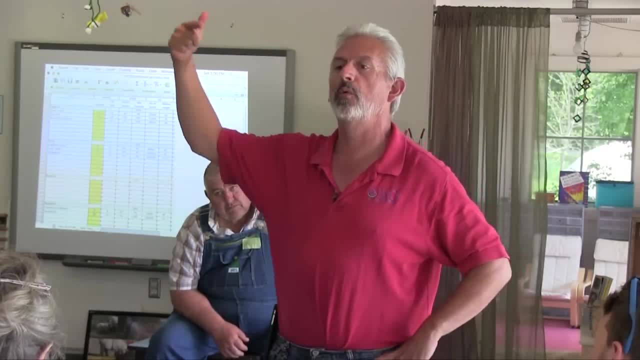 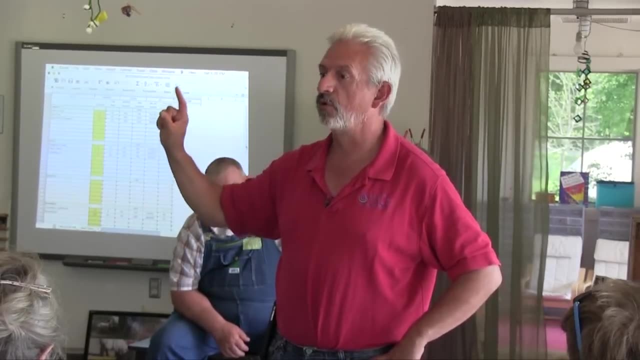 But it's better that you think these things out so you know what your crop rotations are going to be If I'm going to go to corn the following year. it's a heavy nitrogen feeder, So I'm going to have more nitrogen in my mixes, but I'm still going to have cereal rye in there. 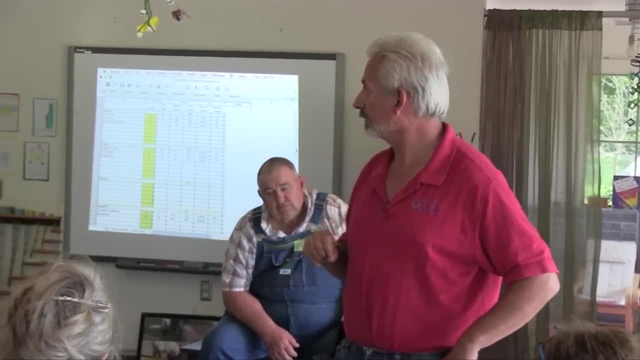 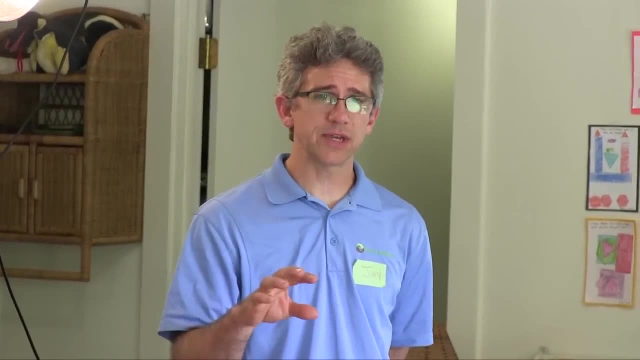 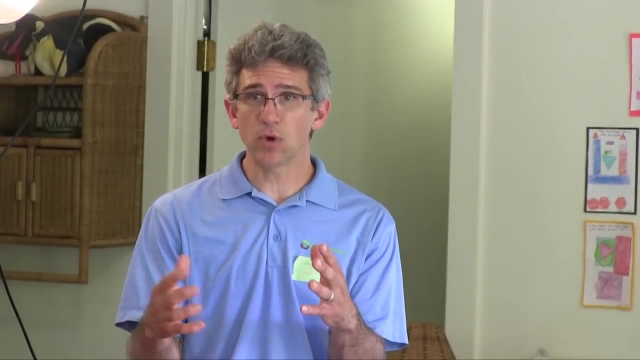 You see where we're going with that. Or tomatoes, or gourds Tomatoes- yes, As far as that. And another place on the web to look for is the Midwest Seed, The Midwest Cover Crops Council. they have a cover crop calculator also that really incorporates your region and what your goals are. 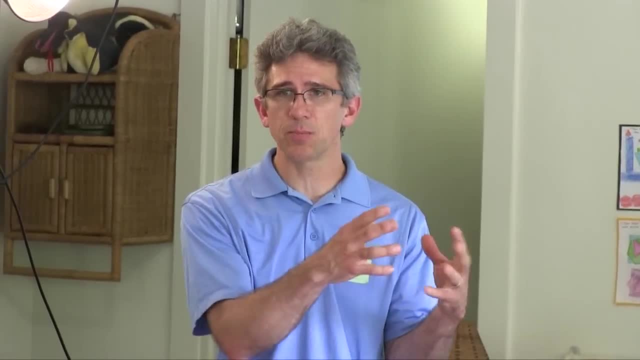 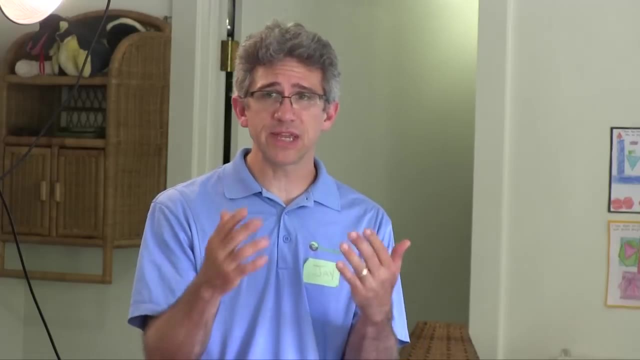 So it doesn't give you specific mixes, but says that here are plant species that work well, based on when you are planting and what your goals are, What type of crop you're growing and stuff. So the limitation there is that it only has three component mixes, but it will give you an idea what to look at. 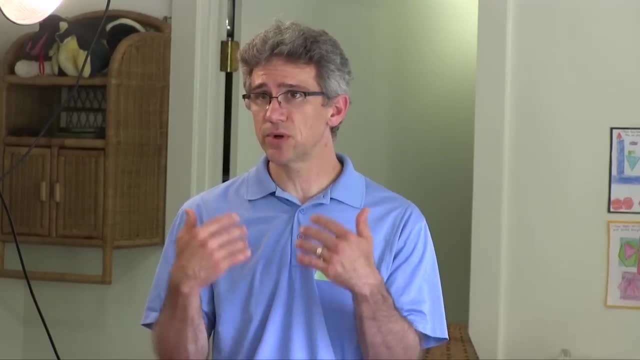 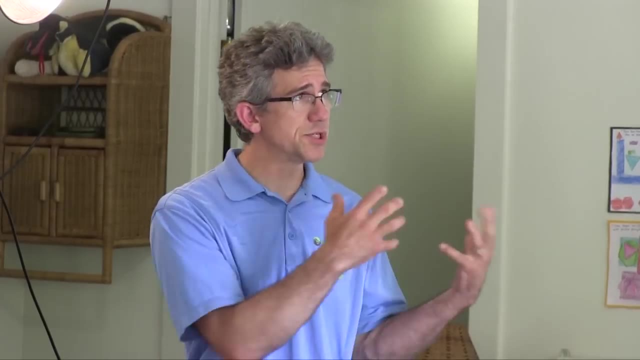 And it's a starting point. All these things are building blocks that we build our knowledge and experience on and go from there. But the thing to keep in mind that we point out is some diversity And, as we showed through experimentation, you want to have three different types, right? 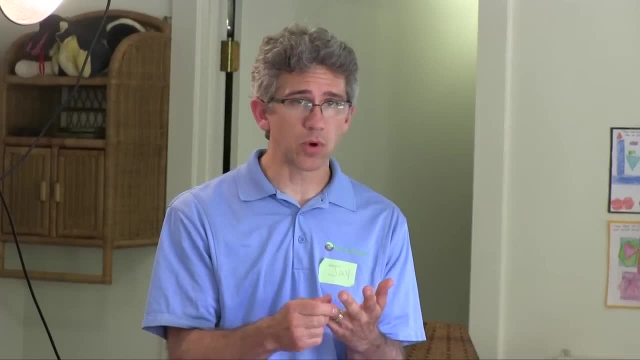 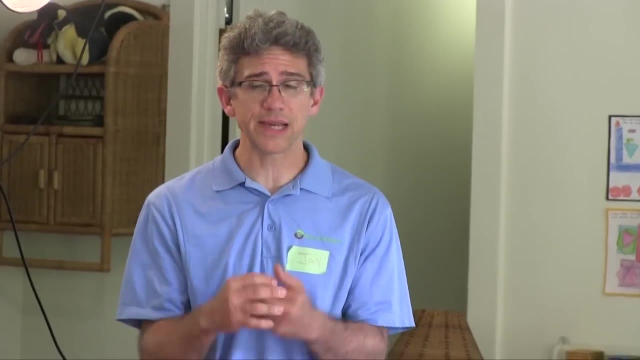 A legume, a grass or grain, and a broadleaf or brassica. You know brassicas don't do well in the summer. That's why it's not in the summer mix. But if you have something in cool season, a brassica is a great way to add some diversity there. And then to try to get the number of those different things in that five to eight range. There are other benefits to go higher And if you're looking to get specific, once you learn what these different cover crops do for you, you'll be more comfortable going into those higher numbers. 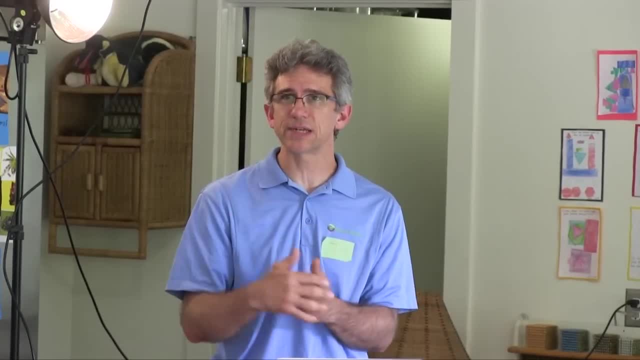 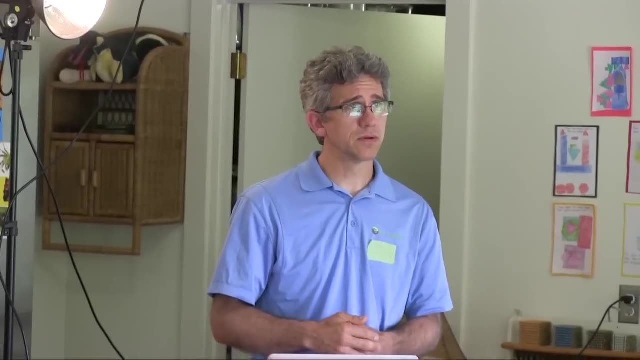 It's just that in the front you may not see the benefit with the more complex mixes from that standpoint. So once you look for what the benefits they are, then you can add them in Now. Rocco loves animals. I do too. 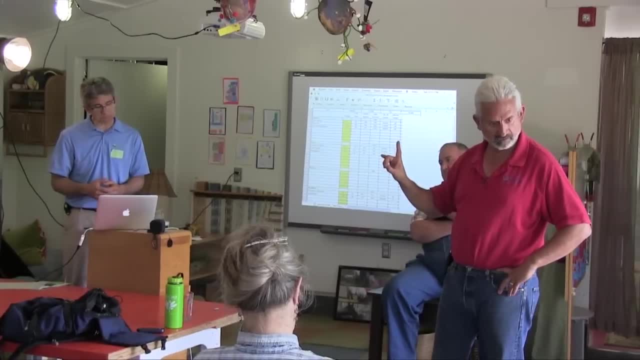 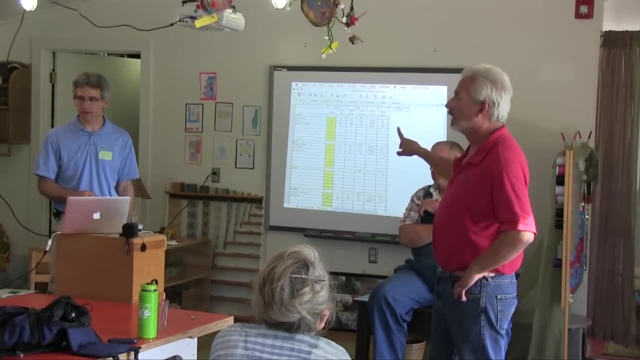 My mix would change. If I'm summer grazing, it changes, Okay, so it depends on your goals. Any questions before we go out there in the field: Jay, do we need to bring anything more up here before? Okay, we're going to save that mix. 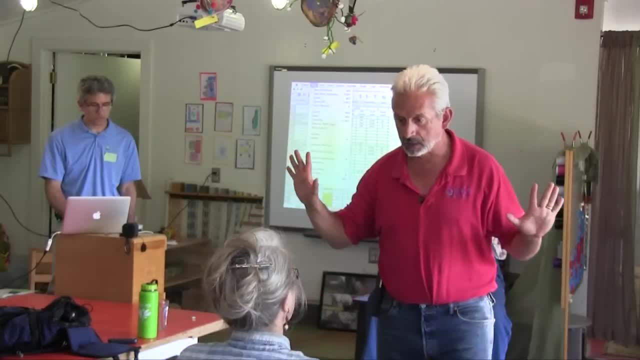 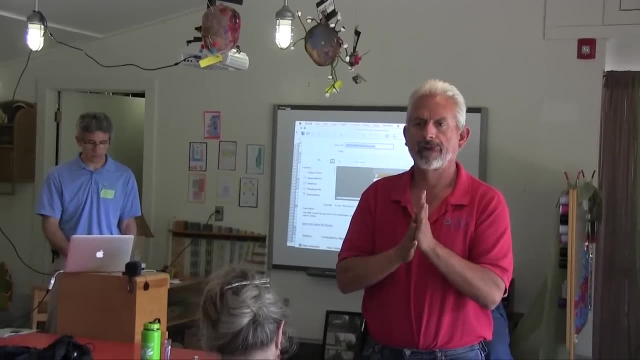 And we're going to talk about. okay, was it like drinking water through a fire hose? I have a question. Okay, question, yes. How important is your soil test to determine the type of mixes that you're going to use? Oh, you are slick. 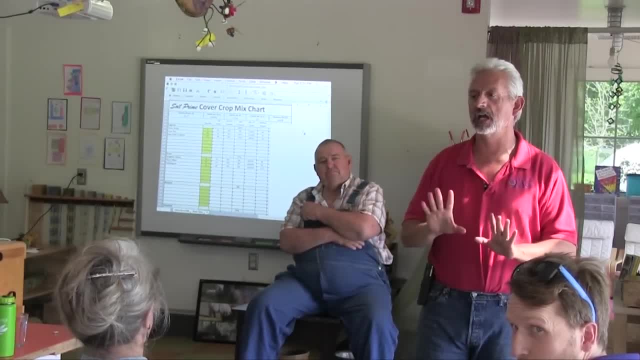 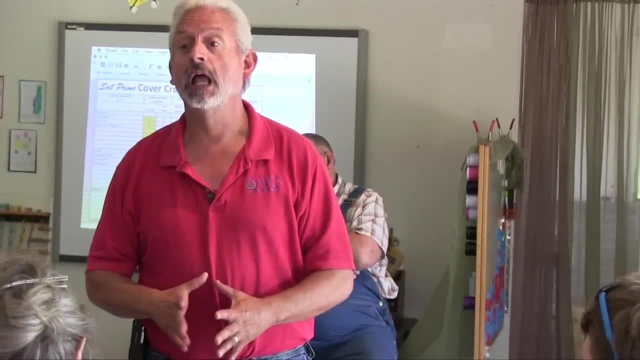 You know what? Let me tell you something, And I didn't want to go into this. I got a new soil test by ARS, USDA that I used to help design my mixes. Ah, I'm going to come back. I think we overwhelmed you. 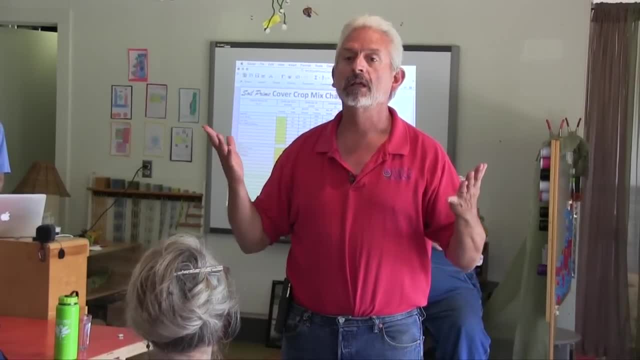 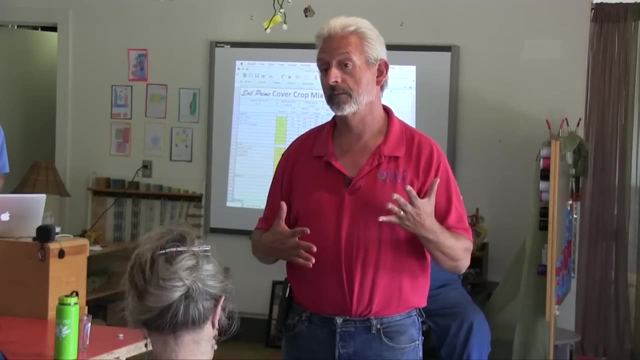 I'll come back and we'll do another class and we'll focus how we'll learn how to use the Haney test. go out in the field, learn how to read it and interpret and I'll come back. okay, You can't. 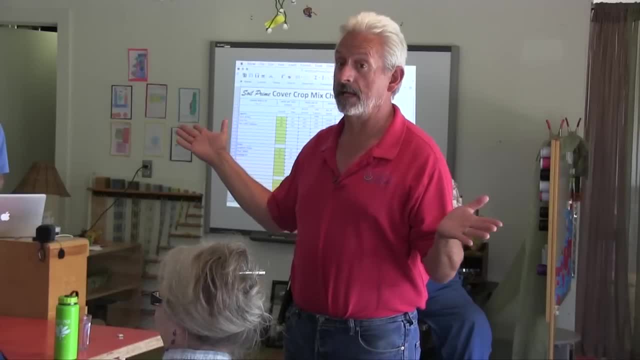 You've got to tell us now You've got 20 minutes. No, we don't. We have a very tight schedule. Well, but I'll come back. I promise to come back and I'll show you the new test. 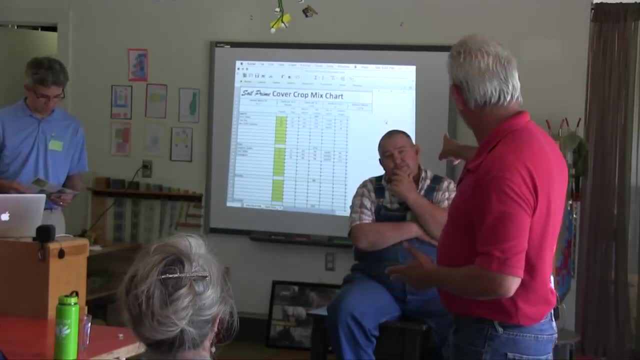 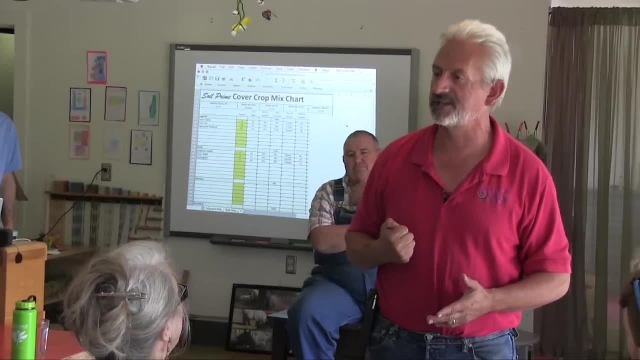 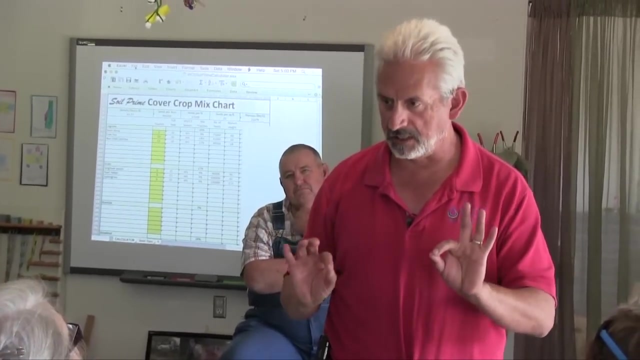 We are saving. what do you think of that test? Great, Awesome. We have saved some of my producers. one soil test saved them $60,000 on nitrogen fertility, Our no-tills. this soil test works very well in systems that are dynamic equilibrium. Pastures, no-till forests. they also work very good in conventional. The regular university soil test works very well for destroyed soil systems, but do not work very good for dynamic equilibrium systems. okay. So this soil test brings up the biology and it brings up the water-soluble carbon. 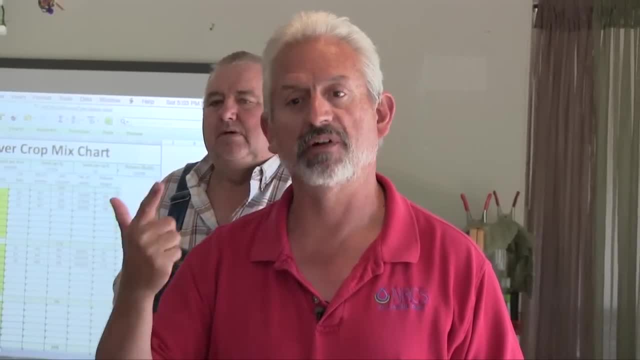 If I know how much water-soluble carbon, I know how much food. If I know how much food, I know how much nitrogen they're going to produce. What's the name of the test? It's called the Haney test. 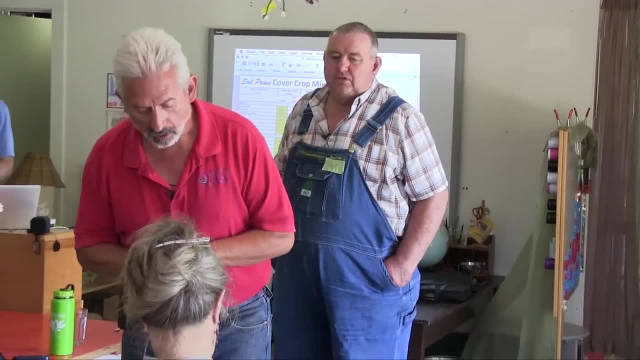 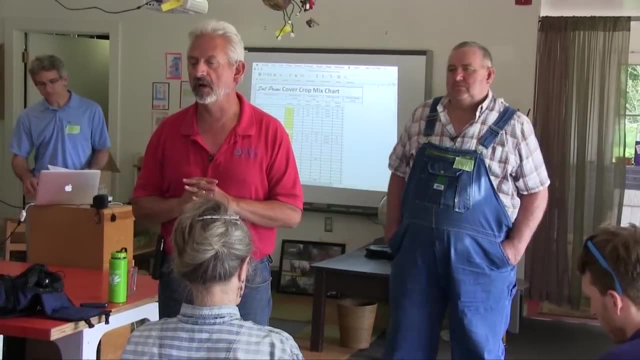 Here's where I would take it: Woods End Laboratory. Write it down: Woods End. Woods End Laboratory. in Maine We've already been. NRCS has already put money into this test. We are excited. We have taken this all over the country. 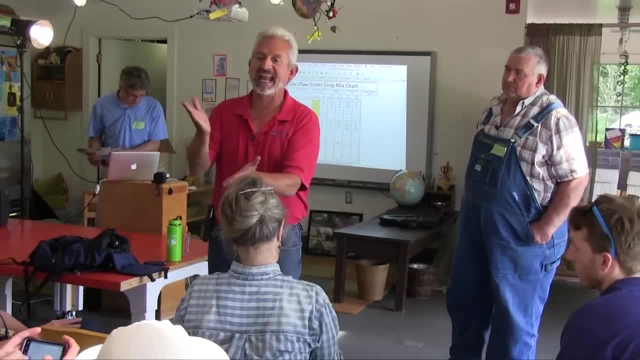 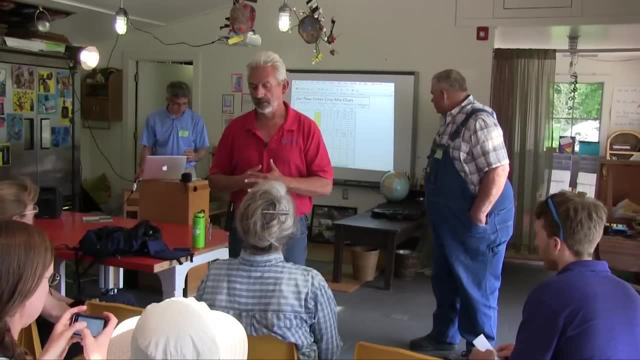 It's called Woods End Laboratory. You need to ask for the Haney test. It gives you fertility, It gives you aggregate stability, It gives you all kinds of parameters. If you need help, we'll help you. interpret it Okay and I want to make an announcement. 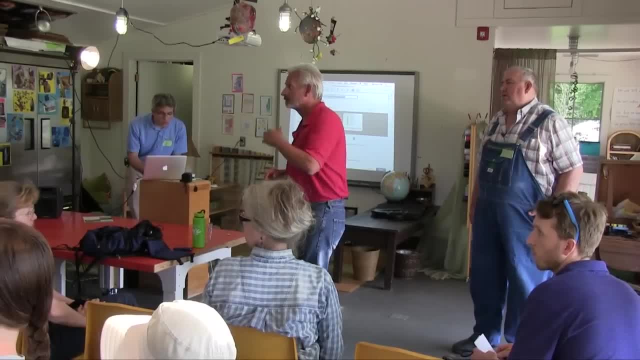 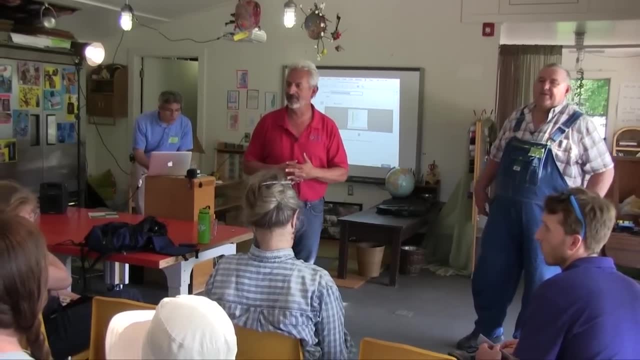 Yes, Pat, If we actually get back and eat dinner quickly and stuff, there could be up to a half an hour after dinner when we could do that. I could do 30 minutes of that and I can give you a good foothold and then we can move on there. 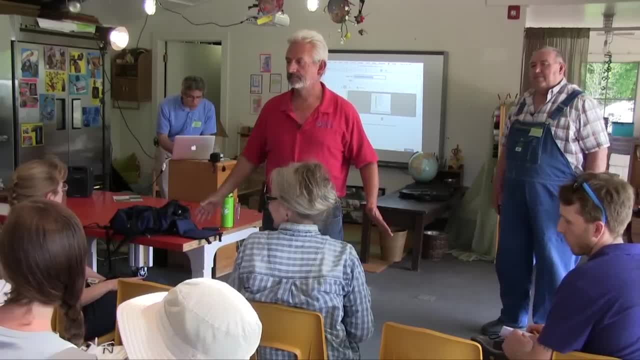 How's that? You've got to move fast from one place to another and not dilly-dally, and be aware of what you're about to eat. Yeah, but I know you're going to get excited about the covers. I know we're going to. 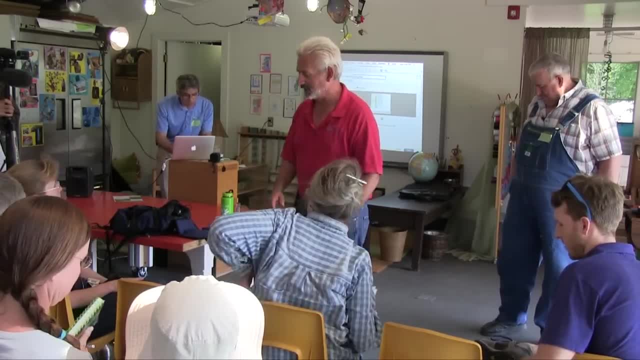 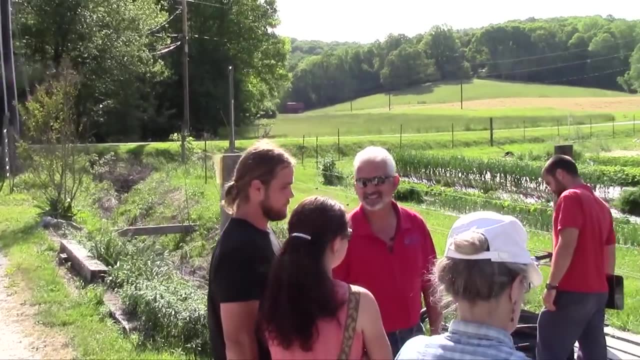 Yeah, I know so too. Okay, let's get out in the field. You guys need to get out in the field. I can see it in your face. Yes, It's a big, important thing to understand. Yeah, and that's the problem is that we've reduced it to what chemistry said. 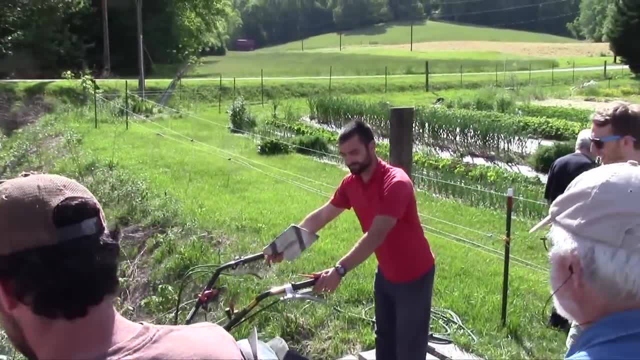 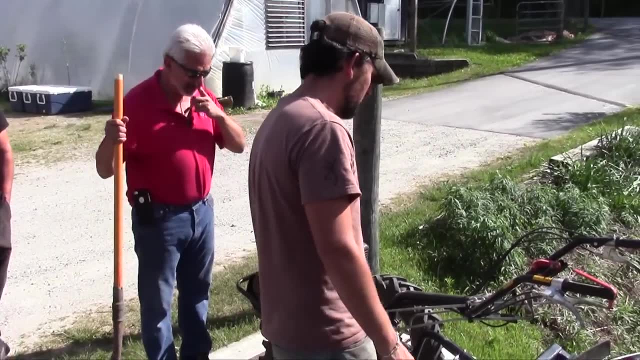 Exactly. Does it work that way? No, But it's exciting that you guys are picking up the right concepts. I'm not the operator, Am I drawing it? Yeah, You go ahead and just take him out. Are you going to roll it? 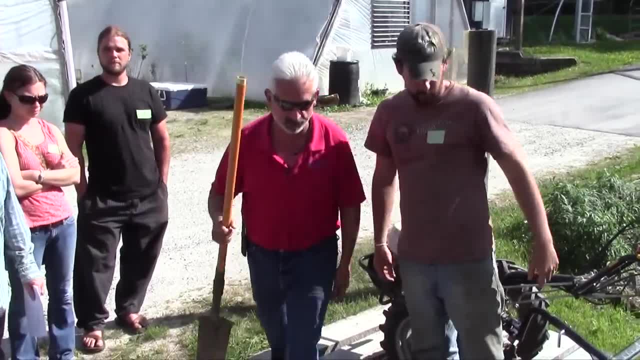 Yeah, Let's go. Which are you going to roll? Yeah, let's go to this side. guys, Come over here. I'll meet you all there. We'll just meet this over here. I'm excited if you're going to back up too. 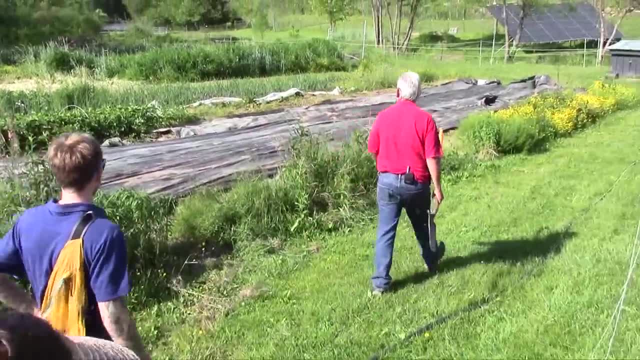 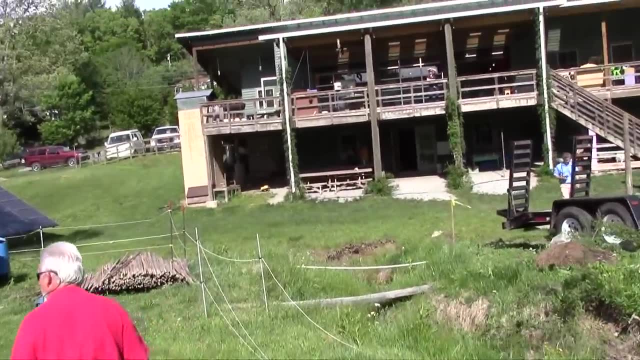 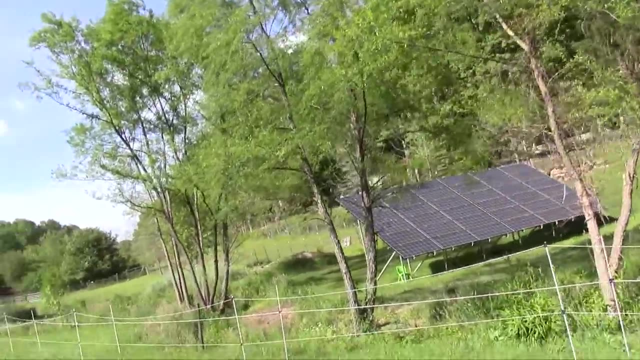 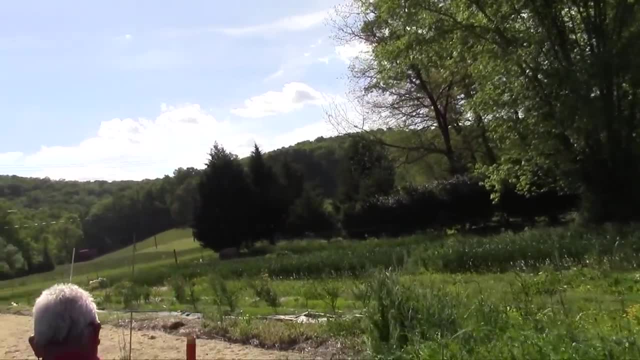 Oh, that's okay. So we're we're still going to the other farm and just doing this right now. We're going to do this and then we're going to go to the other farm. Okay, Because I want to show them. 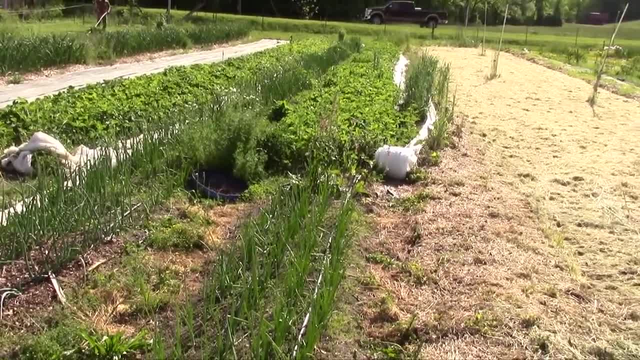 I don't have a mic, so you have to talk at me. You can't. I got your mic right here. No, I don't have that. I don't have the mic. Okay, class, get over here. I'll just real quick. 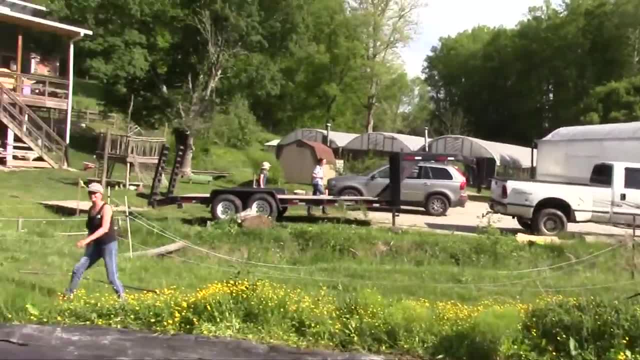 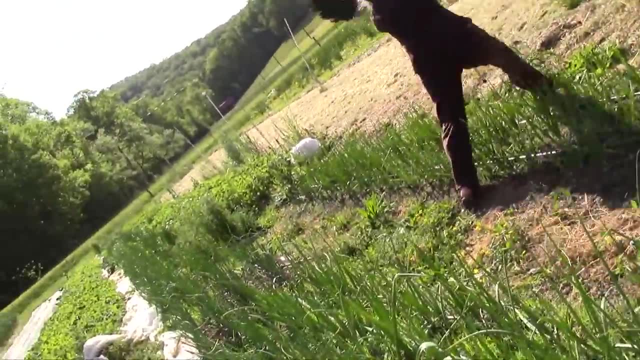 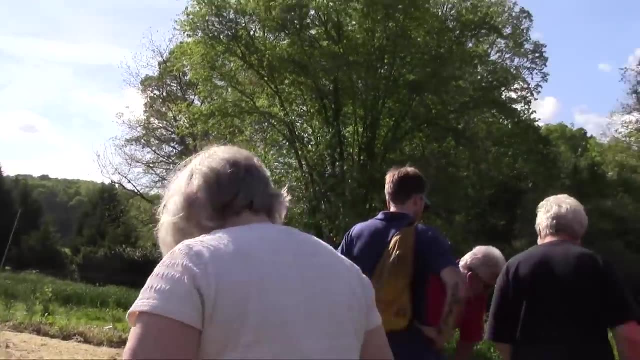 Like, don't run off without telling me what I want. I'll give you a call if I want to. Okay, I'm going to show you guys. I want to show you something and I want you to. Okay, everybody gather here. 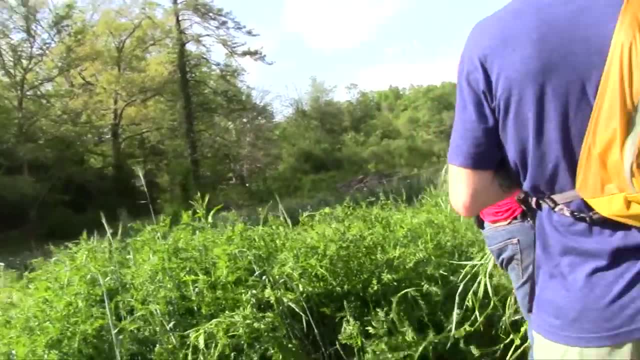 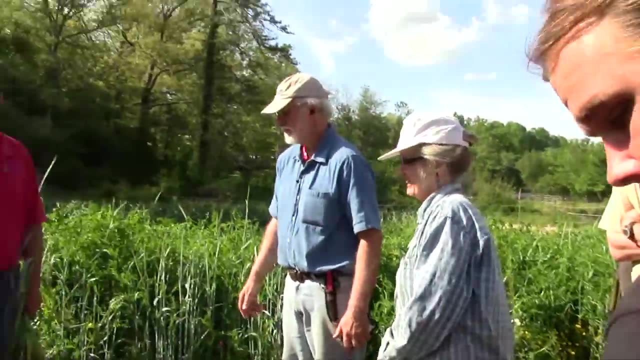 I'm going to show you something. I want you to see how you're going to start being an observer. This right here. you guys ready? Let me give you some time. This is going to be the most powerful instrument you guys use, okay. 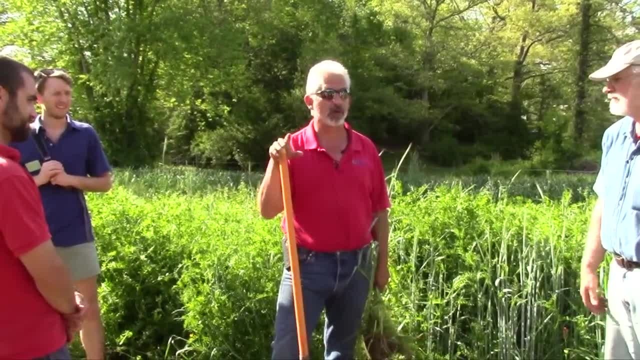 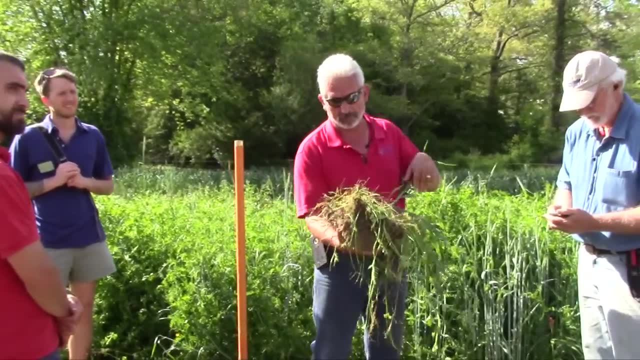 And I'm going to show you how to start identifying what's going on in your system. Ready, Okay, everybody close, Okay, here this is the cover crop mix When I walk on any farm, I don't care if it's organic. 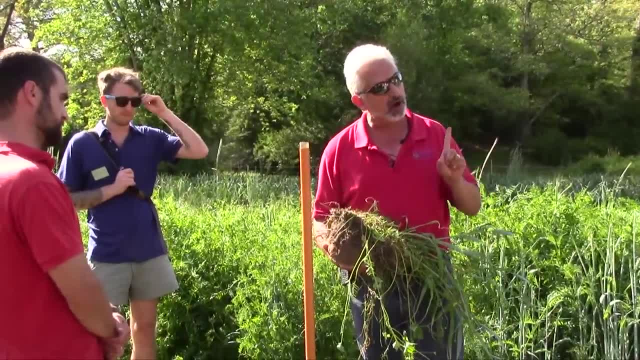 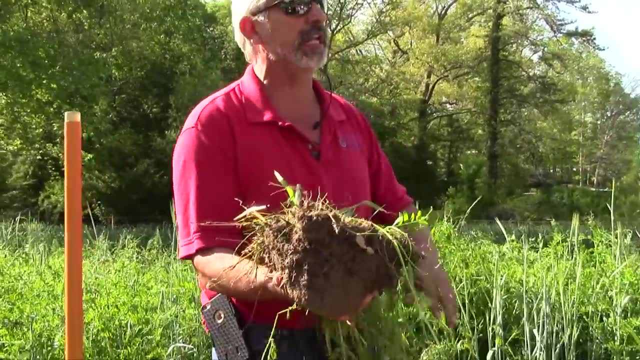 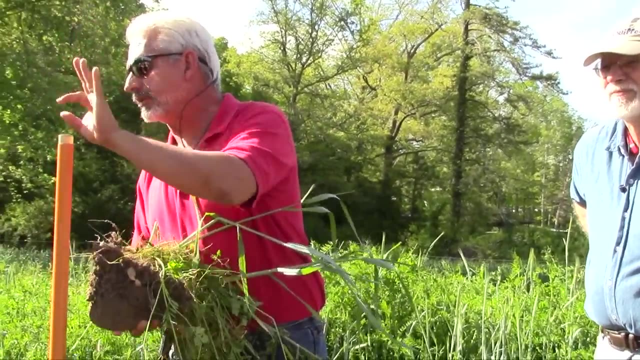 no-till conventional pasture forest. I want to see all these spheres present in the soil. okay, Now, every good, healthy, natural ecosystem, soil ecosystem will have all these spheres present. I want to see every one of them present. 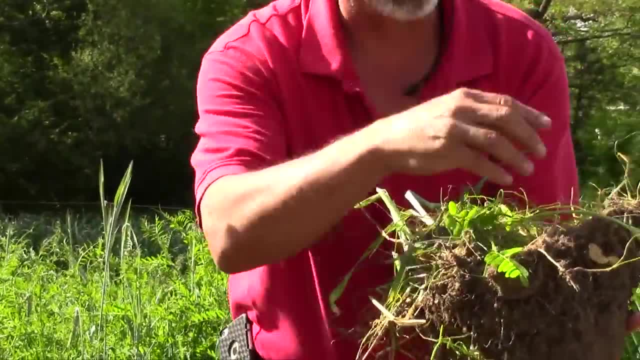 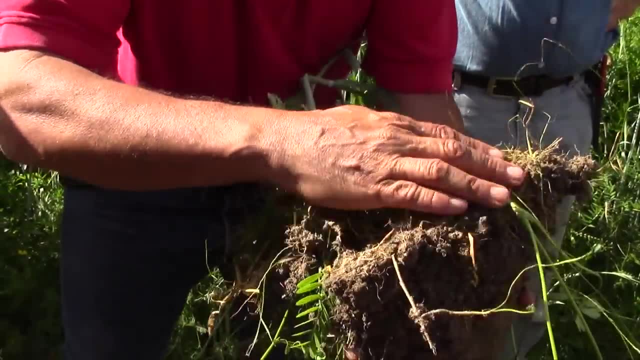 The first one is: you got it close. Come and see, because I want you to start learning how to do this. Okay, you see those broken up pieces right here and this little duff layer of broken up pieces of residue That is called the detritus sphere. 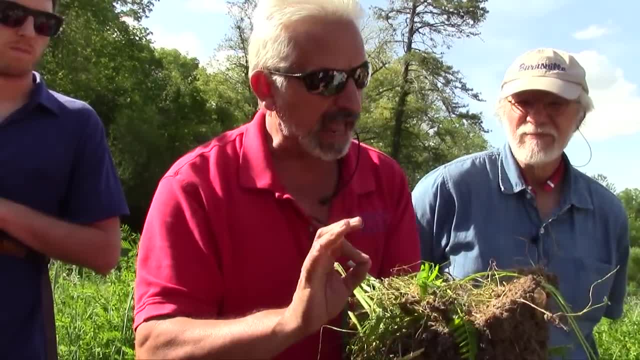 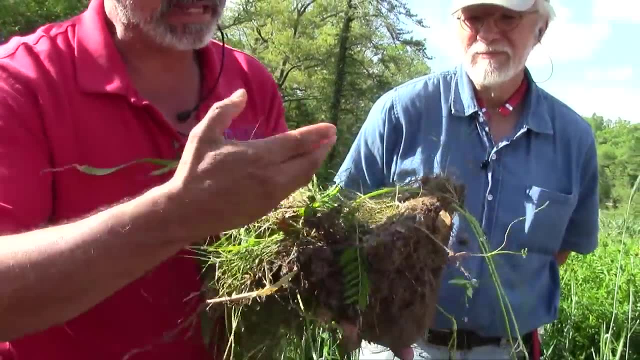 Soil called detritus. The archaeologists call it the detritus sphere. What that means is these unrecognizable pieces becomes that skin. That skin is very critical. In that skin layer you have a lot of meso, microfauna, saprophytic fungus. 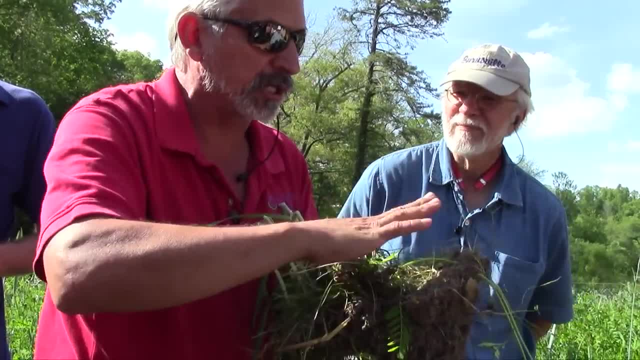 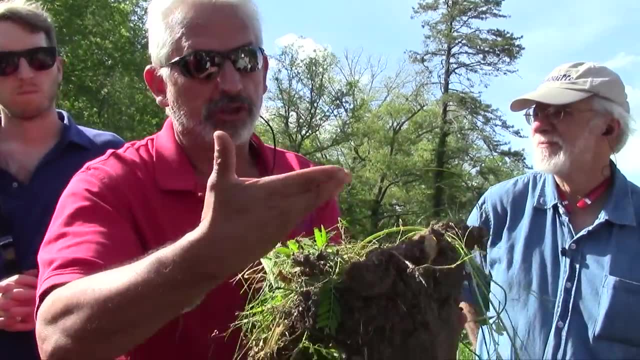 you got all these cumbalimbola. you have all these grinders, mixers. This is critical. When you pull this back, I'm going to show you. when you pull that layer back, you'll see aggregation. When you don't have that detritus sphere. 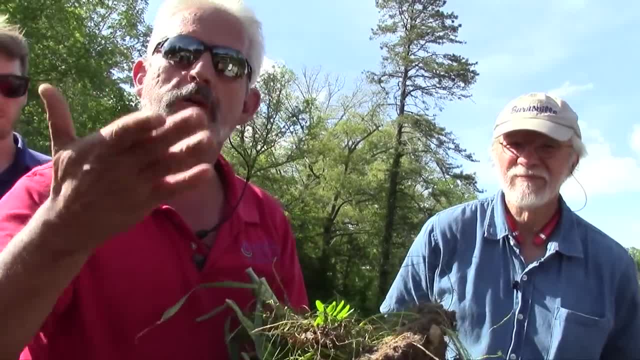 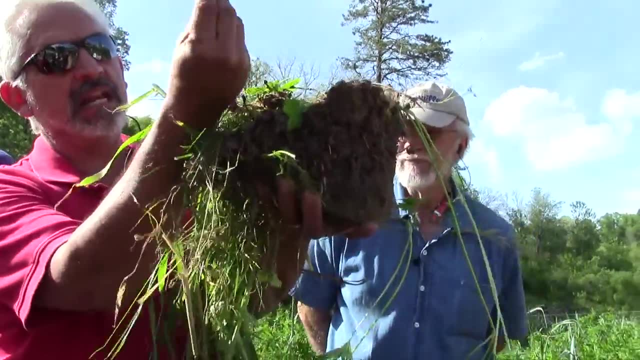 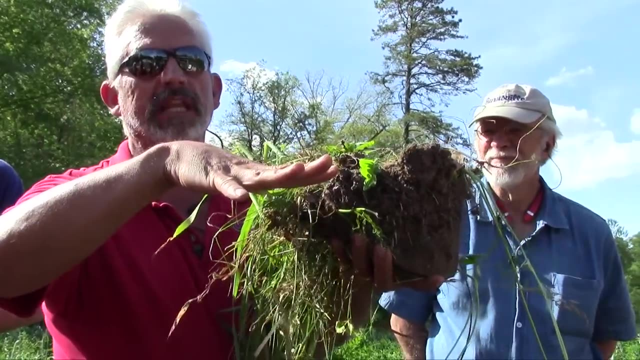 you will get crusting. You will get crusting. So it regulates temperature, protects from rain impact, it feeds the biology and, as it's broken down, it goes through a catabolic process and leaks all these materials into the soil ecosystem. 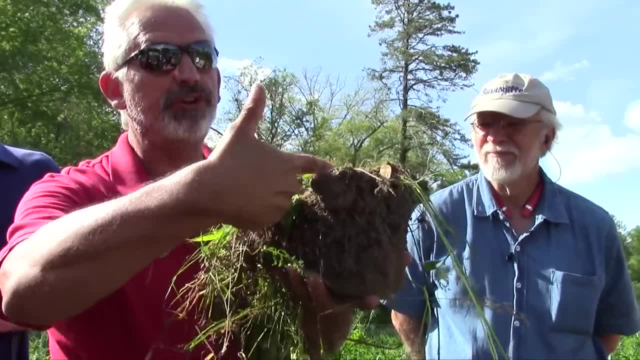 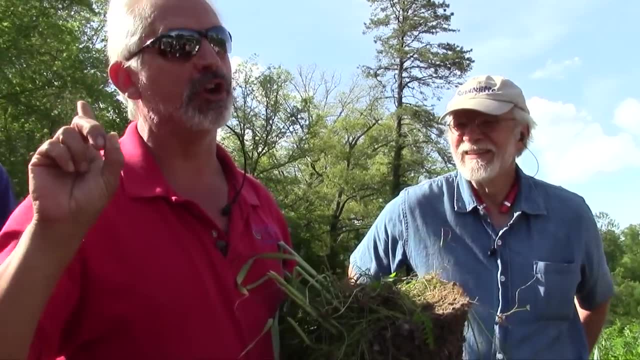 and feeds it. Okay, so I need that. If you don't have that, I know what you're doing. You're doing way too much tillage. You're tilling the snot out of that ground and you're burying it. 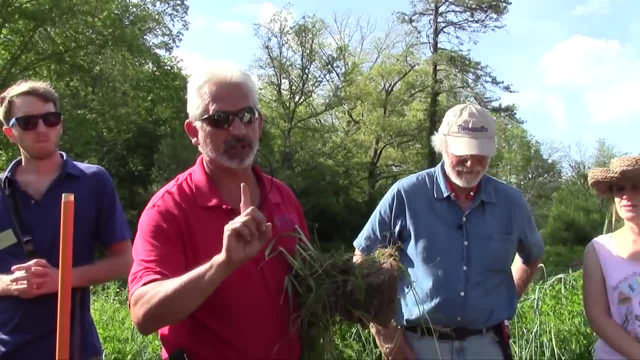 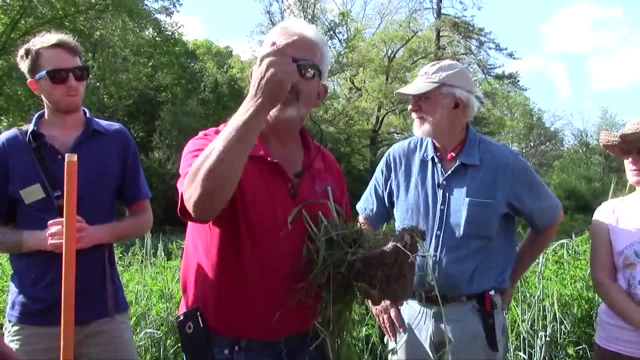 I don't want that much tillage going on there, So I watch that. You'll see this in the pasture You go to. that woodlock it will have a detritus sphere. Prairie will have it present, A pasture will have it present. 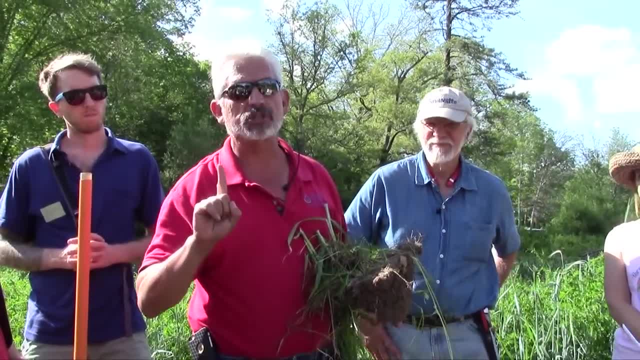 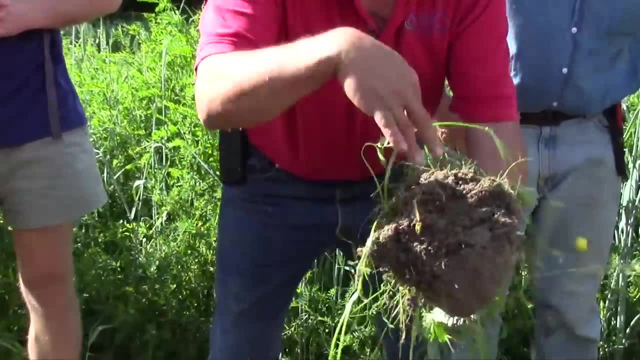 All of it will be there In a system that's doing way too much tillage that will not be present. Now, look at here. You see this cottage cheese area. Look at this. Everybody can you see that? See those big aggregates. 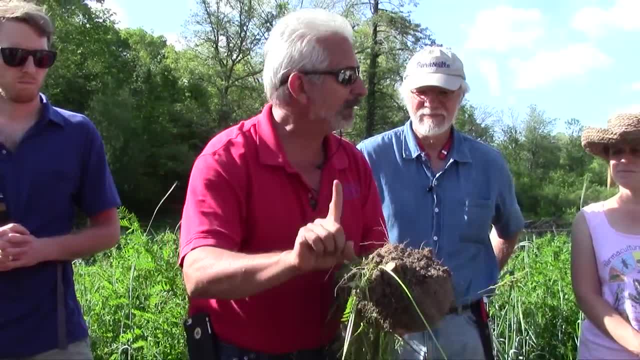 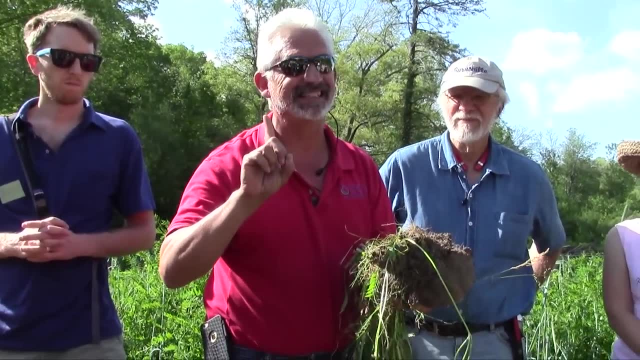 That's called the aggregation, That's called stratosphere. I want to see huge amounts of that cottage cheese present. If I don't see it present, you're tilling a lot Or you're overgrazing In a pasture that's overgrazed. 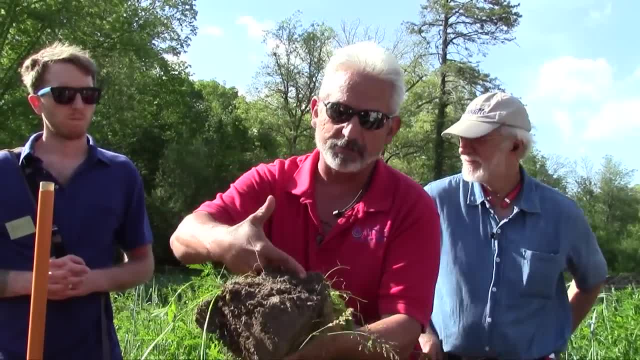 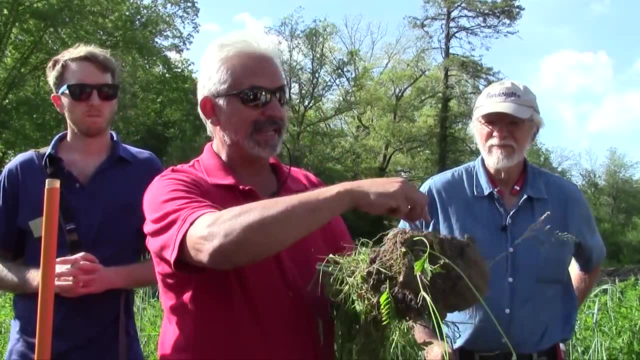 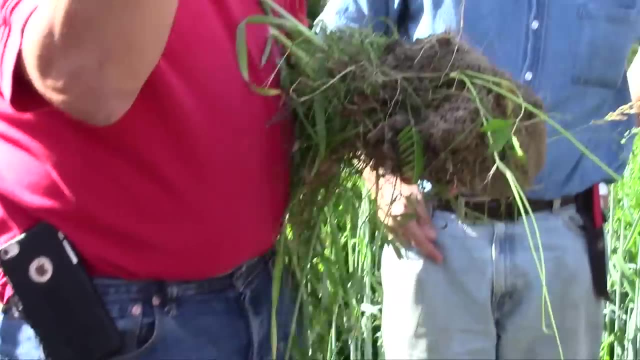 you will not see as much aggregation because it takes huge amounts of energy for the fungus, the bacteria and all these organisms to create that aggregation Inside the aggregate. look how it's dangling. See that Cottage cheese is the porous sphere. I got cottage cheese. I got pores. 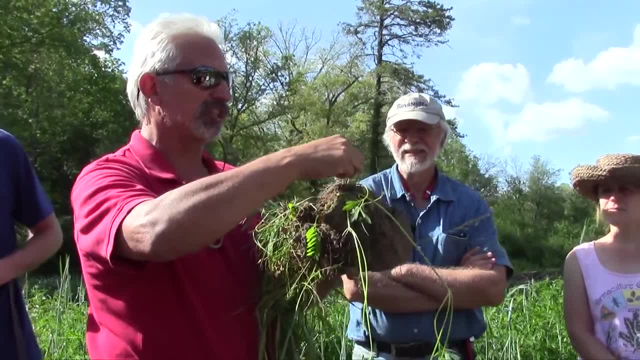 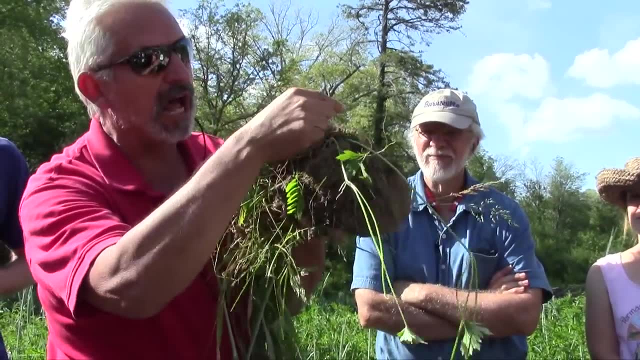 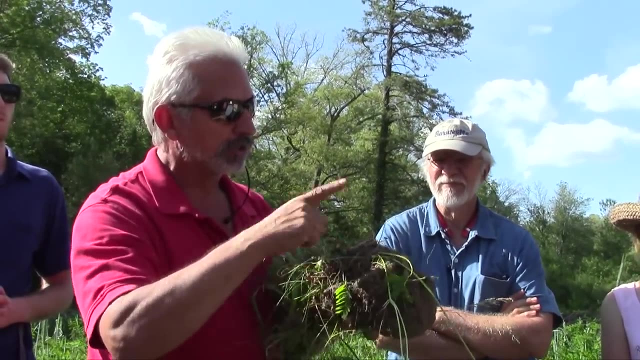 then I got the rhizosphere. This is. I got to see lots and lots of roots. This is the conduit for liquid sun to feed the system. No conduit, no aggregation, nothing. I got to see present roots all the time. 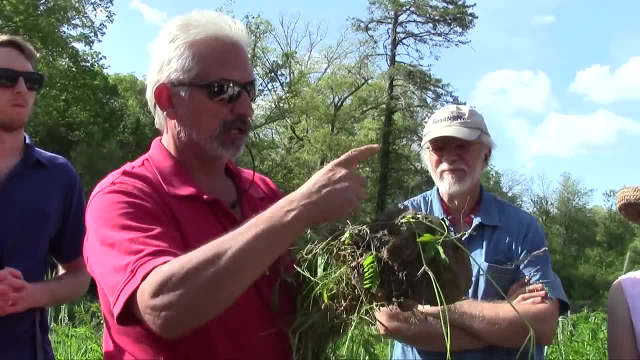 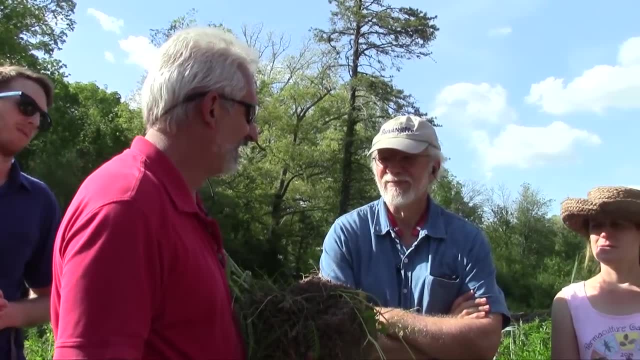 So if I go out there, I want to see this present. So I want to see detritus cottage cheese aggregate. I got to see a living root And the last one, the drillosphere. I didn't make that up. 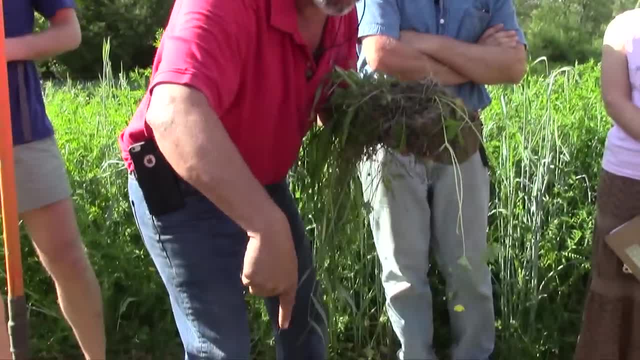 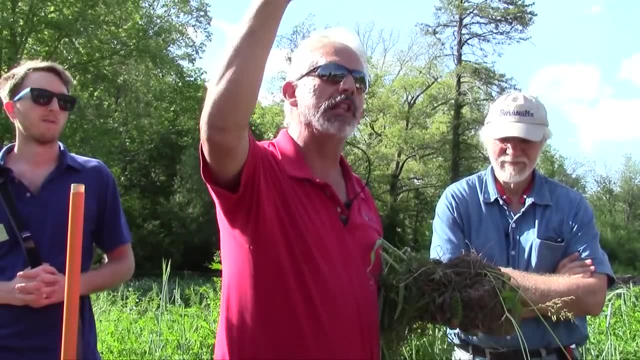 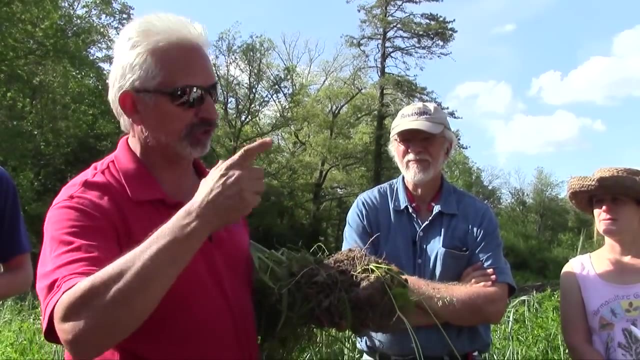 It's called the worm sphere. Drillosphere in the Greek means worm. That passage of that earthworm is latent with bacteria and is latent with phosphorus and nitrogen- Huge plethora of bacteria and you'll see this beautiful glazing. I want to see four to five earthworms. 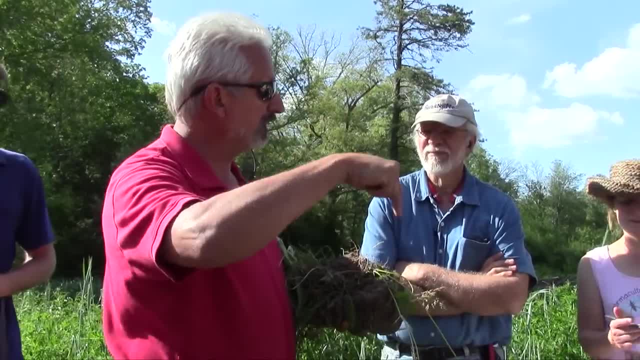 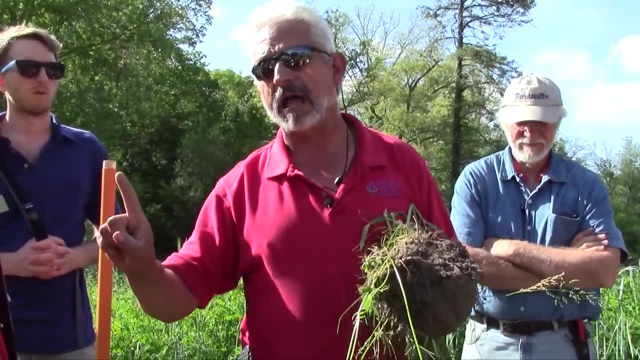 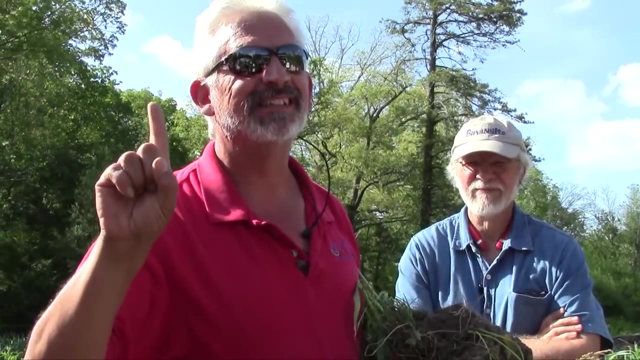 per square foot Per shovel full During the spring. That means I got 850 to a million and a half earthworms per acre. That means they'll move 18 tons of soil in a year And I don't have to put diesel. 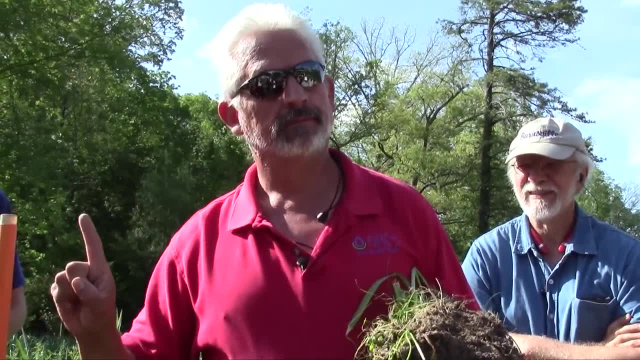 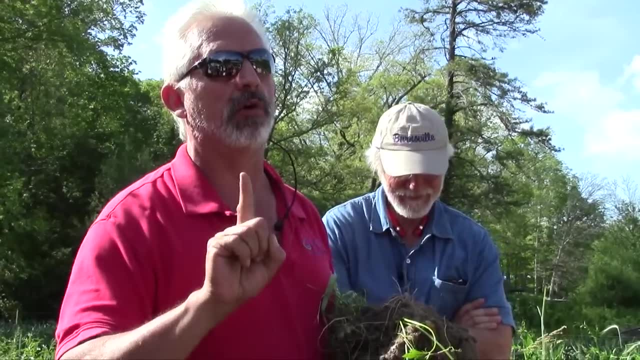 They don't complain and they don't whine. They don't break down. They don't break down. And here's another thing: If you have that many earthworms, they will completely regenerate your whole farm in the upper six inches. 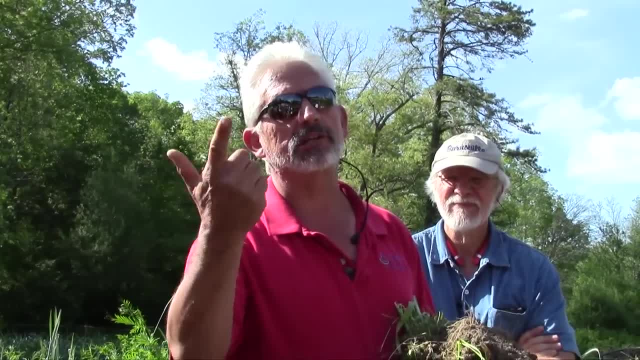 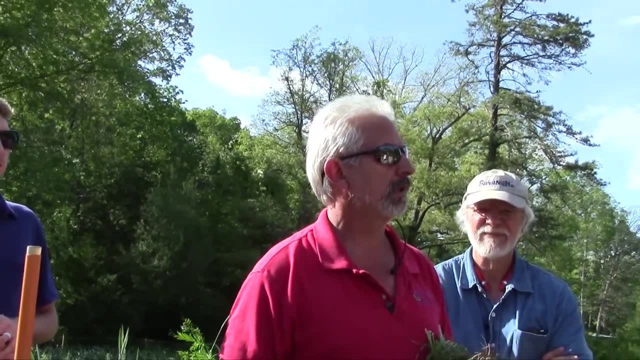 After 27 years and actually purge it of E coli and salmonella. Earthworms are phenomenal. Those are keystone organisms. So you take this in the early spring. So in the summer if you take the earthworms. 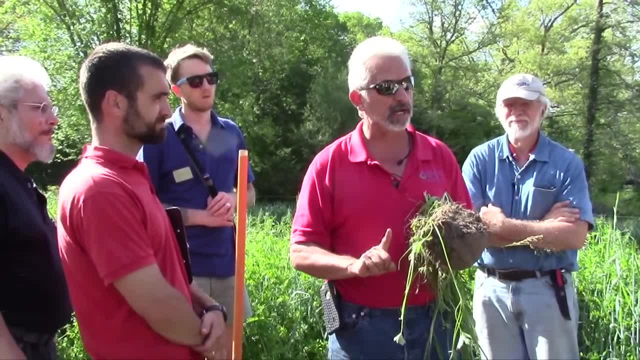 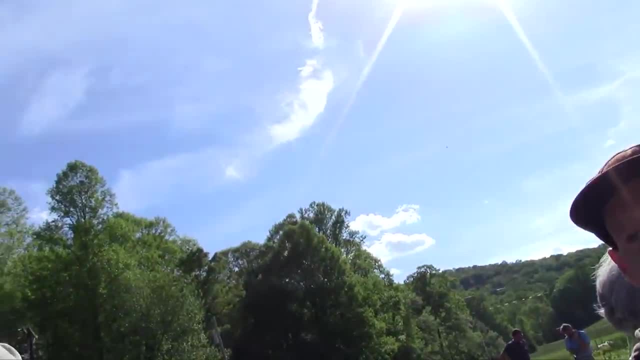 they might go down deeper. So if you're going to check, do it in the spring, Do it consistently, Everybody with me. So what do I want to see? right, Kimberly, Kimberly, so Kim name, one of the spheres I want to see. 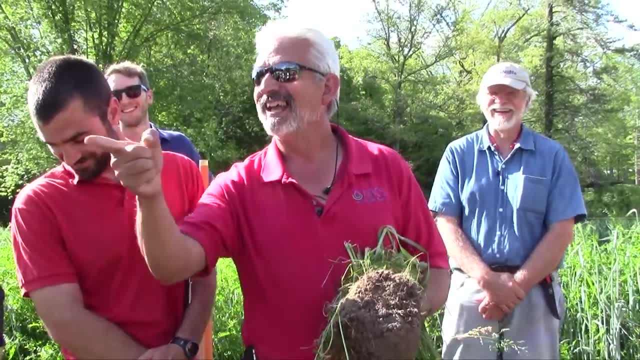 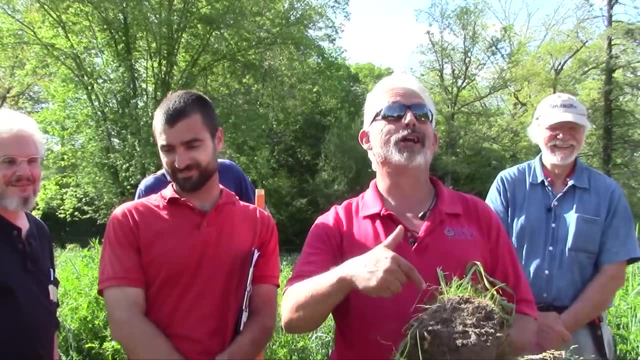 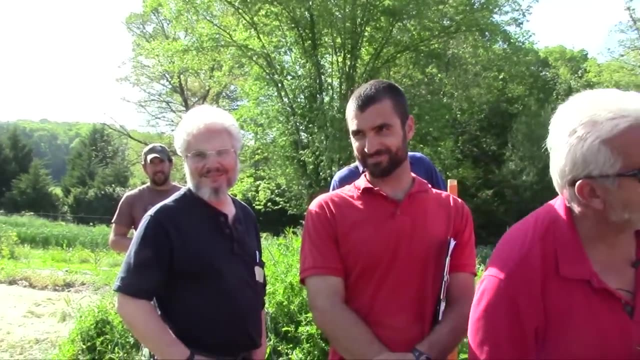 Millisphere. Yeah, the last one, Reagan name another one: The detritus sphere, The residuous sphere, cottage cheese is what Wade Agratosphere, And inside the agratosphere, Mark is the porous sphere. 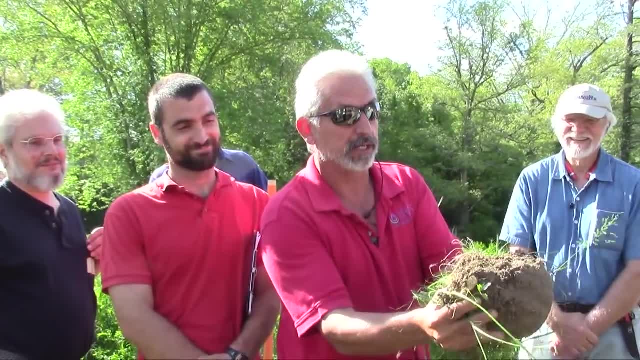 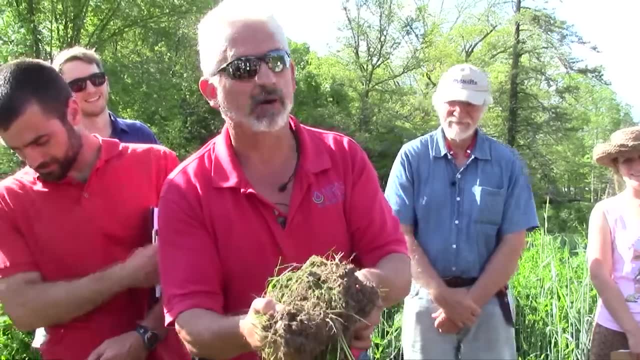 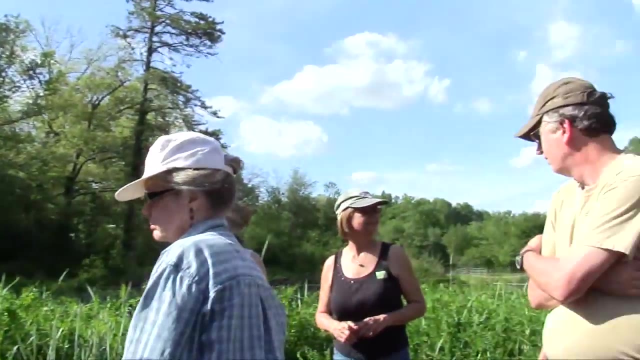 All of them present. OK, I want to see them all present. I want to see soil like this. That's what I want to see: Every shovel full. Now let's look at what happens over here in this demonstration. Dave, come up here and you want to talk about this. 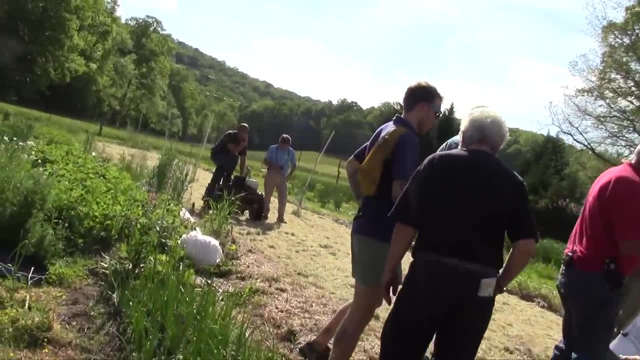 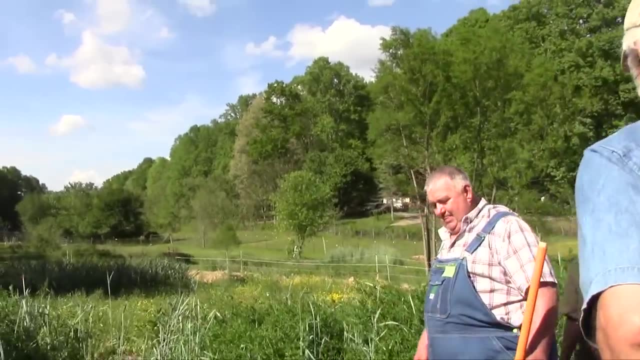 Why you want to do what you do here at this time. Now, this is beautiful. Look at the aggregation over here on this system by the cover crops doing that. That's what I want to see. Now Dave's going to explain why you don't want to plant into this. 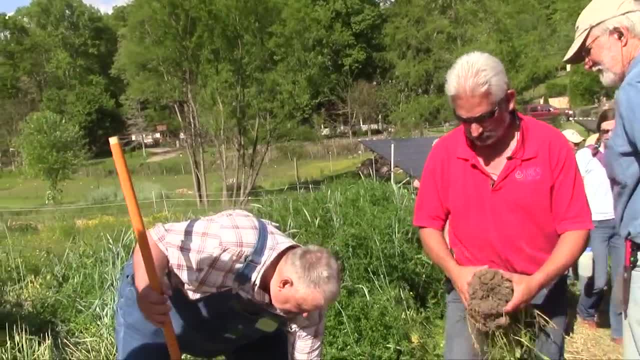 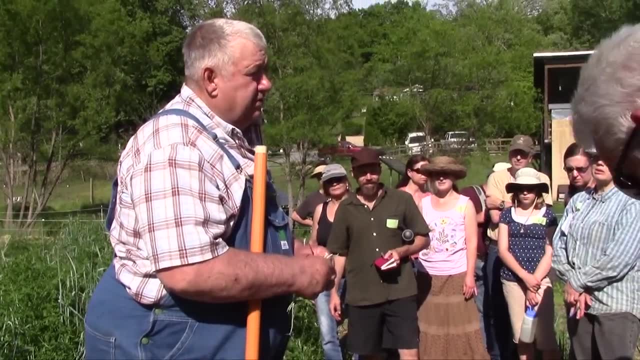 versus. you want to plant into this, Dave, yours? OK, What we have here. they used to flail more And it's still starting to get crispy, But this morning it was real doughy. So if you were to try to plant something in here, 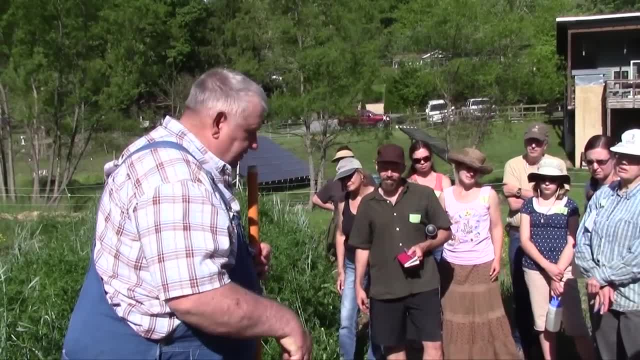 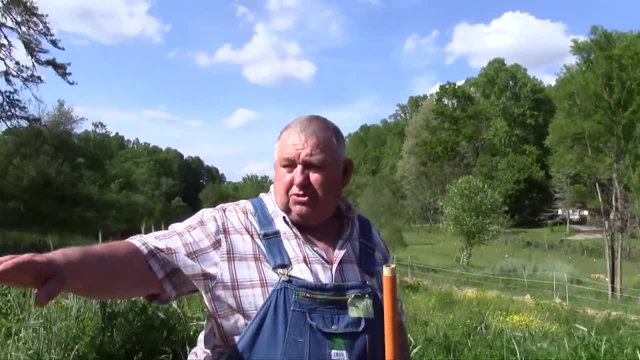 it would actually pinch this residue in the soil And then the air would get around the seeds and it wouldn't grow. Plus, the fact is we got this mulched. If it does rain before they get it planted, it'll probably be two or three weeks too wet to try to get anything. 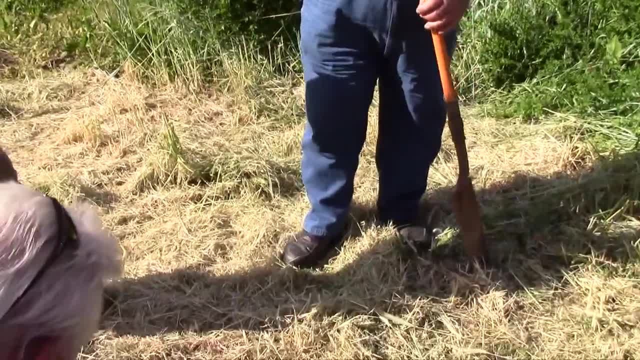 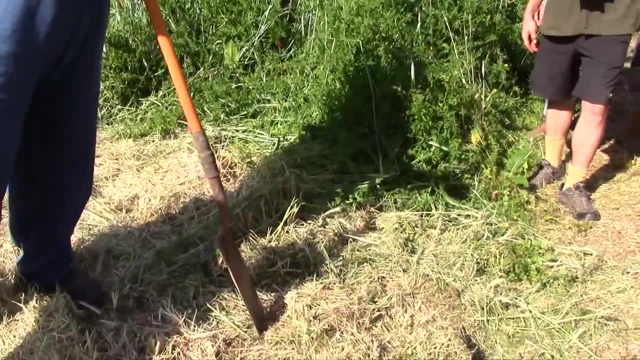 This is a real wet farm too. so, Yeah, right, Yep Right, OK, It will pinch. It will actually pinch this moat residue in the soil, Because he's using a machine. right, A machine, Oh, that's right. 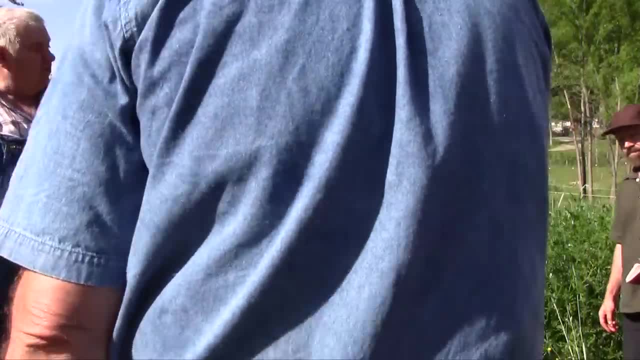 That's right, And the stuff gets pulled in with it. It gets pinched in there. So if we use the roller, which he'll do here in just a second, any time, they're ready OK. But before you do that, let me show you some things before we do that. 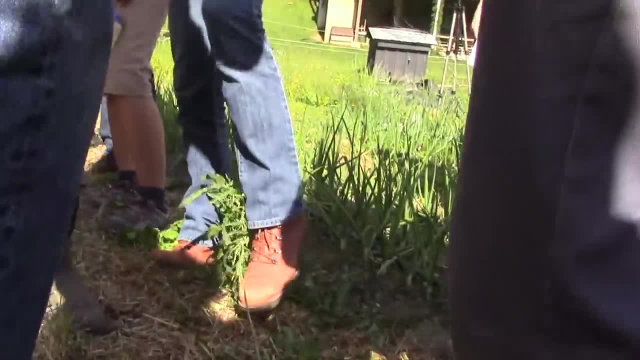 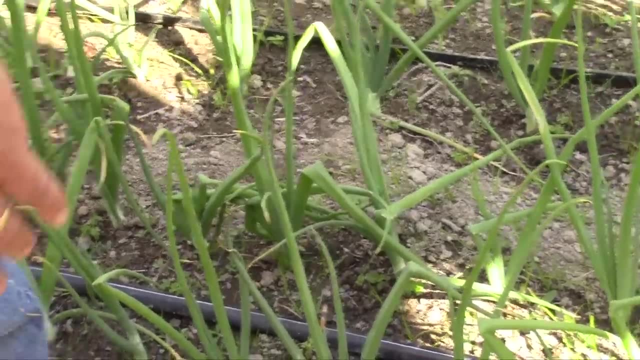 I want you to sit behind here. Look everybody here. What do you guys notice on this surface? Right here you're going to have crusting. This will have crusting. Now walk over here, Everybody. come in here, Get on your knees. 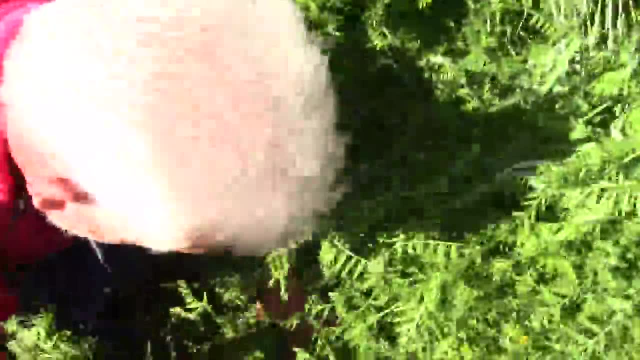 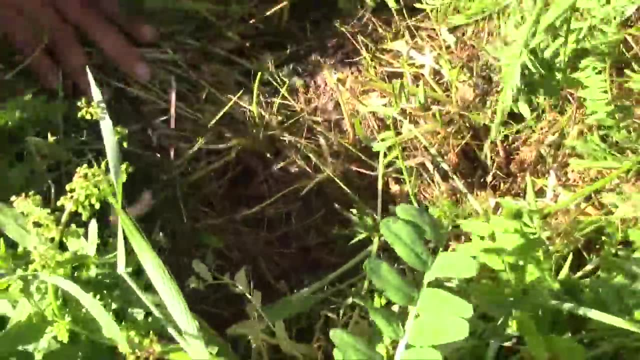 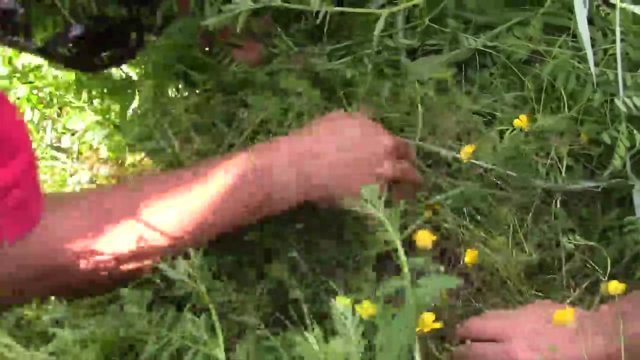 Come here, Everybody. I want you to observe this. Come here and open this up. Guess what? No crusting. You'll have aggregation. You see right here, Look at that. Look how cool. There will be no crusting. 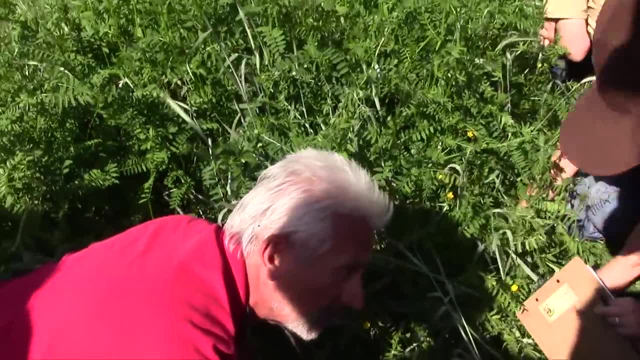 That ground over there, Anywhere there's bare ground you will have crusting. Get your fingers in the ground and see how cool it is. Look how cool it is. Come on, Get your fingers in here. Look how cool that is. 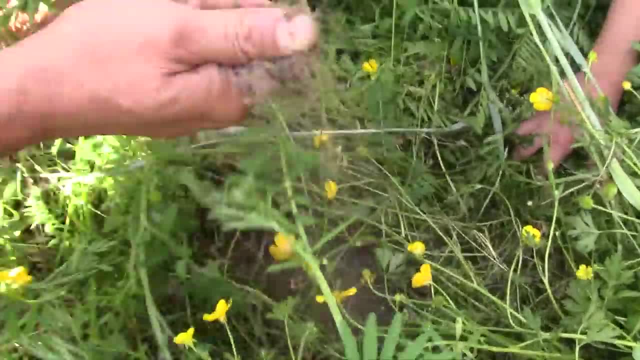 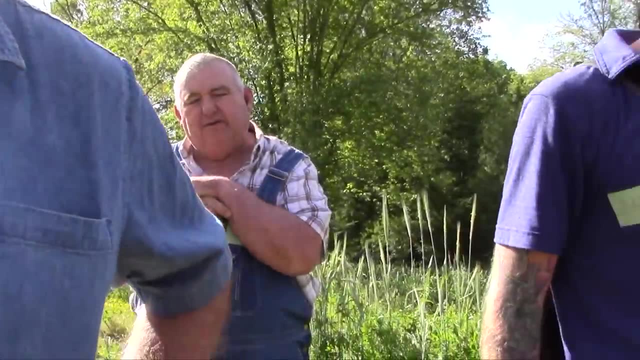 And look how soft it is. Look how you run your fingernails and it doesn't hurt These covers. do that. Move over beside the onions and touch that soil there and see the difference. Touch the temperature there Now. look in here. 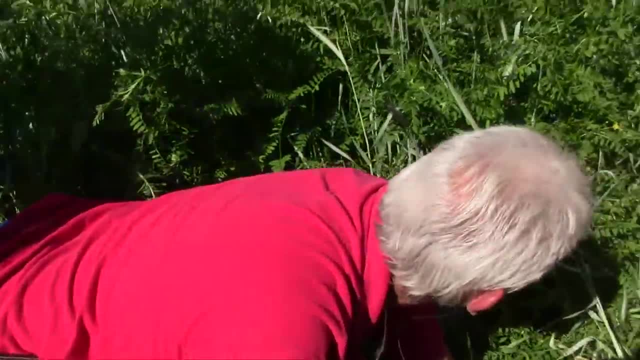 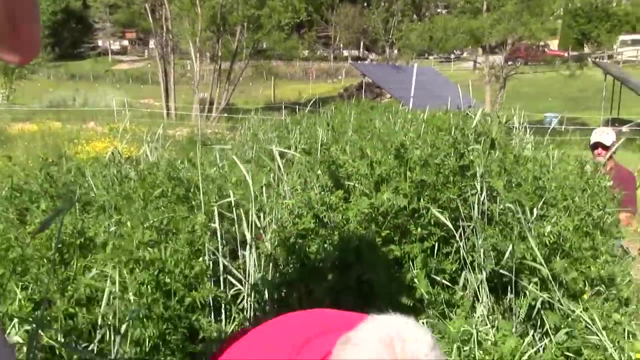 See how cool it is And you're going to plant right into that And we got a real bad nut sedge problem and it's just getting to grow here where it wouldn't get to grow there. Yeah, Beautiful, Thanks, Pat. 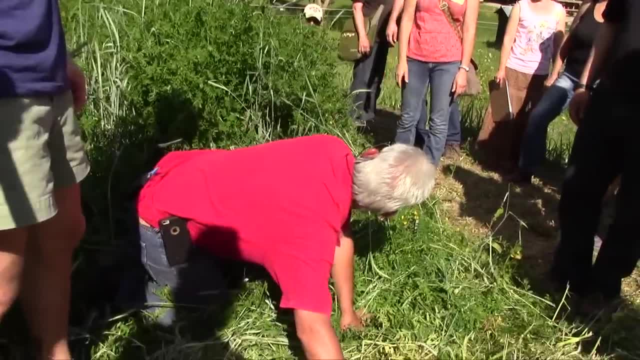 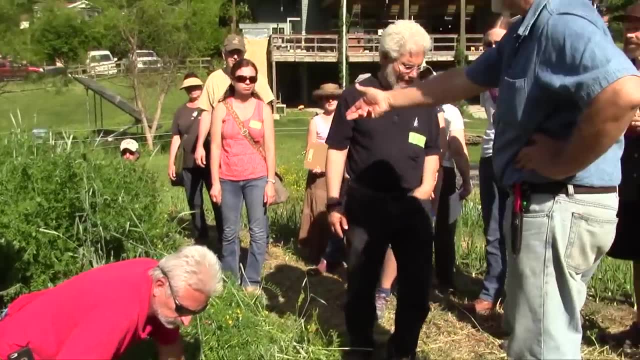 And look at here, Same thing. So I want to see green armor or brown armor, but I never want to see bare ground. That's brutal, And so what we've been doing- because we didn't have the roller until just now, and it was- 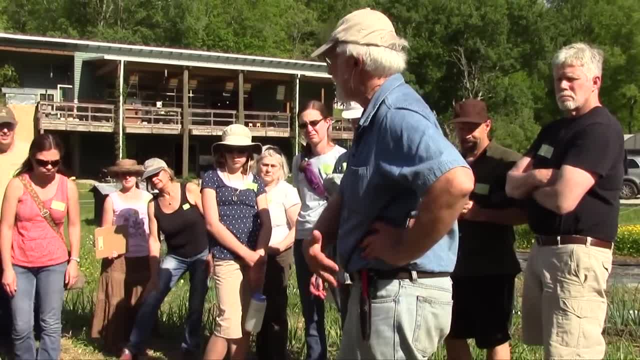 definitely just people being used to what they were doing. it just got flail mold instead. We're not going to roll anymore because we come back and we mulch this pretty quickly, So we don't have bare ground, We don't get the mulch pretty fast. 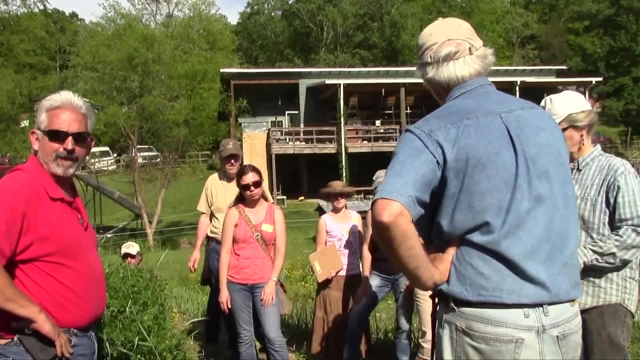 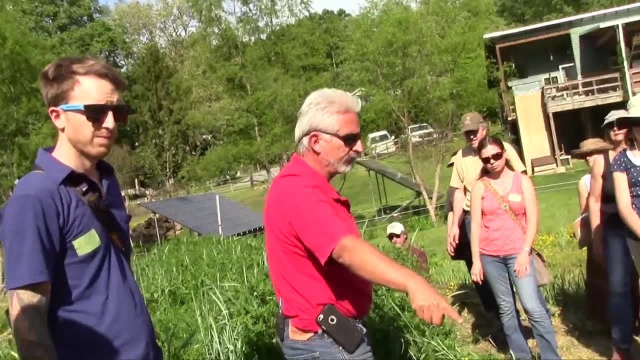 We always do, So it's going to be way less work to lay the mulch down and plant through it rather than come back and haul it in. It takes a lot of time to mulch- Great, Any comments? No, Any other one. 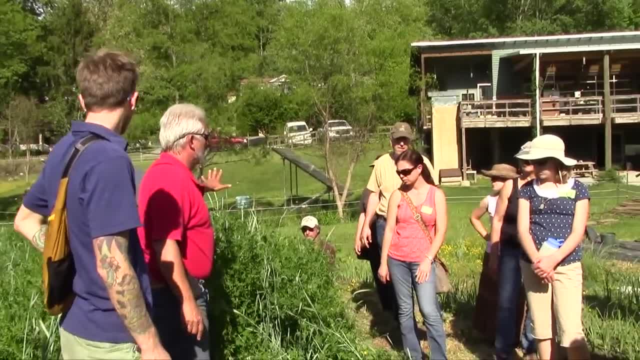 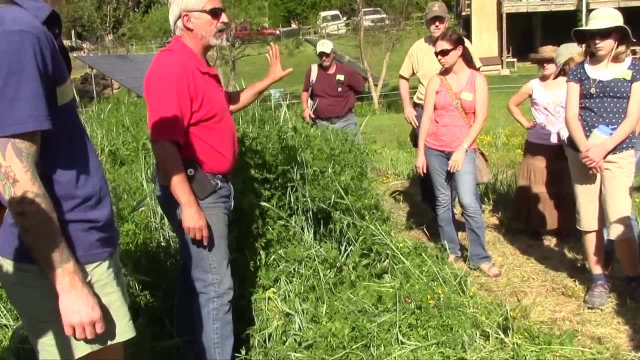 So you don't want this, Ken. you want to be planting something like this. This is where we call it green planting: Soil's softer, It's cooler. There's a great book called by Dr Geicher. I'm going to save you the pain: 405 pages. 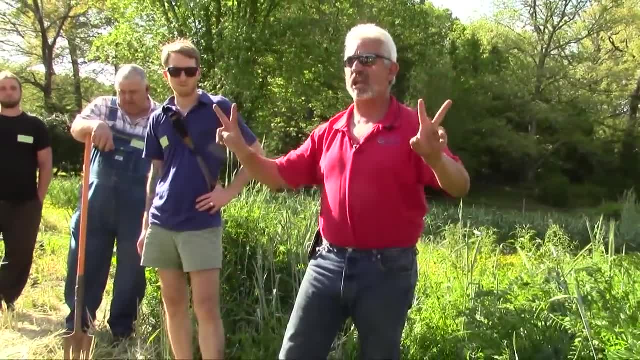 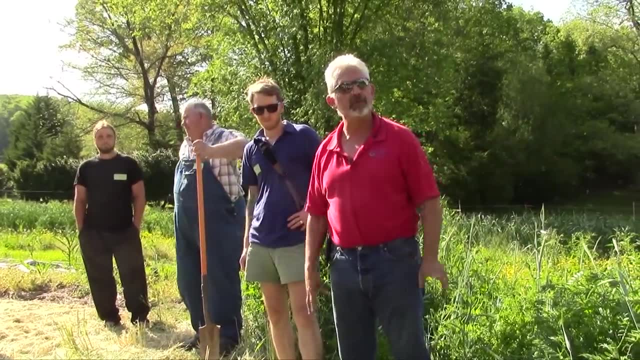 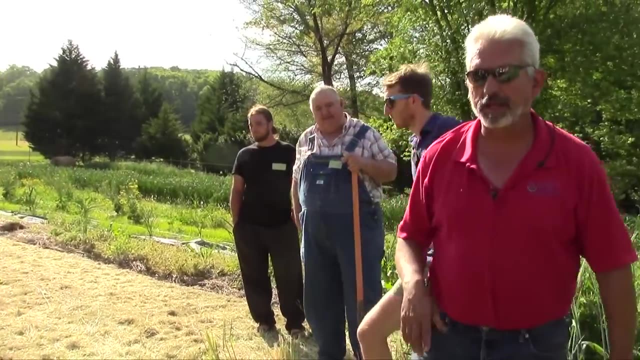 of intense calculus and soil temperatures. He said: the best way to regulate soil temperature and moisture, a living plant. Yep, Oh, my goodness Saved you 500 pages. Okay, Run the roller, Probably in September. Okay, Now go ahead and run the roller and then you guys can videotape that. So you don't want this because the planter's going to have problems with it. So how soon after rolling it should it be planted? Oh, right away, Right away. Yeah, One or two days. You either want it very tender or you want it very brittle. 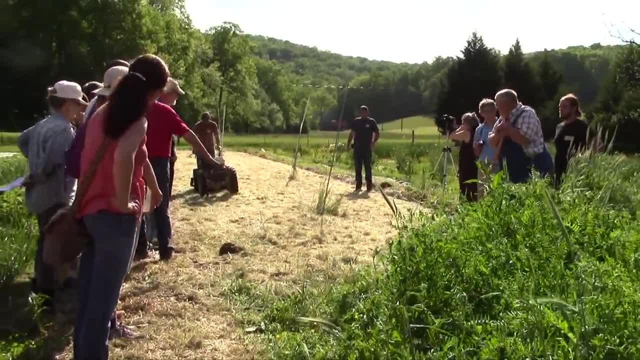 Now he's going to have to wait until it's brittle, Then it's going to drip Without dripping. Without dripping, That's right. That's right. And don't let it drip again. That's right. You don't want this. 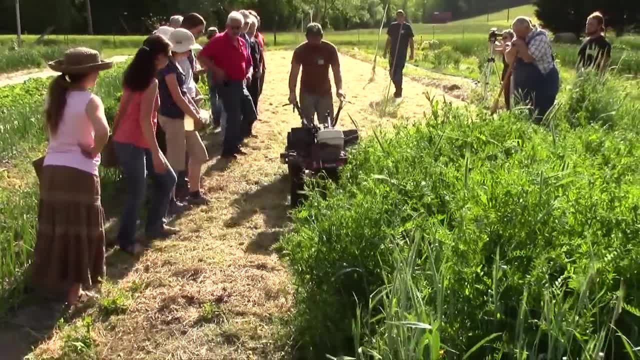 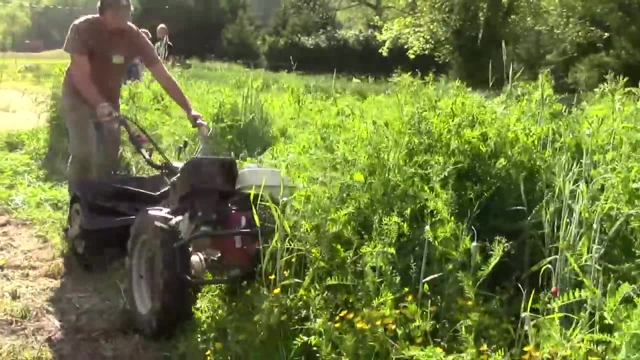 That's good. You don't want this? That's good. Now we'll have to wait. Let me try again. Do you want this? I'll get this one. I'll get this one. No, That's fine, Okay. 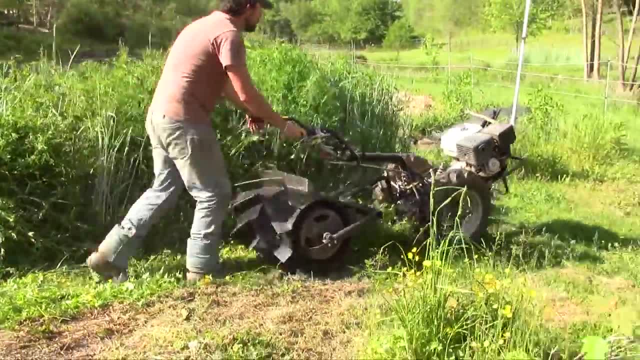 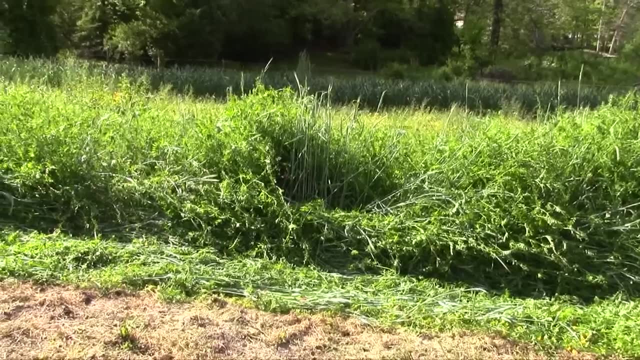 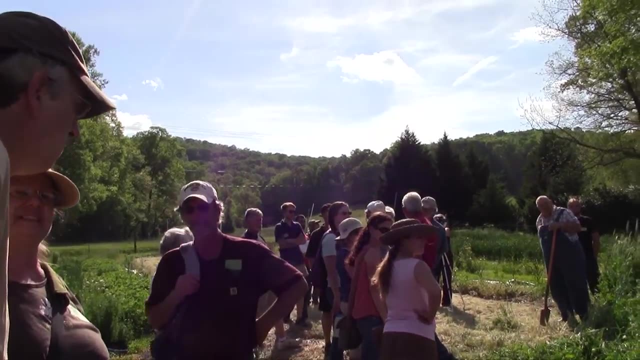 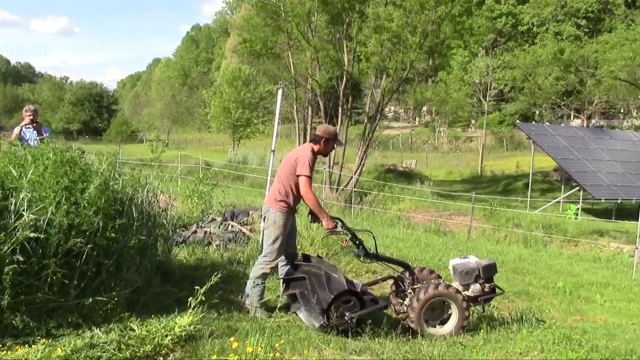 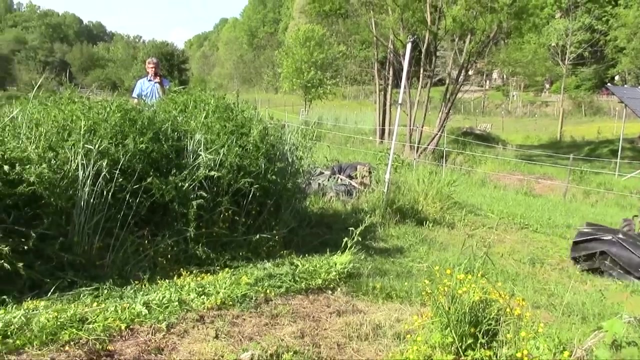 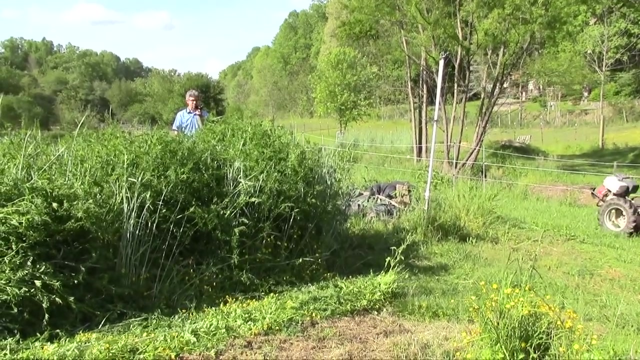 That's good, We're getting into it, But couldn't you just do that anyway, to break it down, instead of just or try, or to try to make? I want that to be heaven. we gotta get more. mine is an old, you saw my. I used my wife, my. 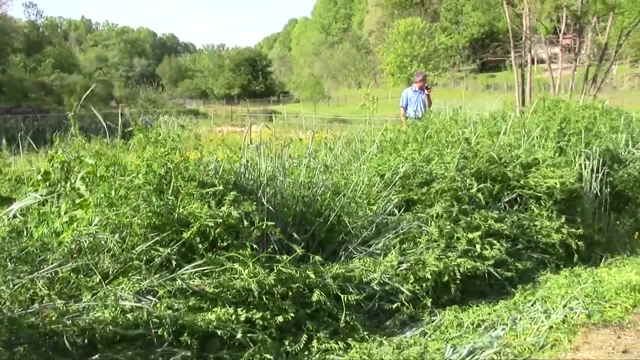 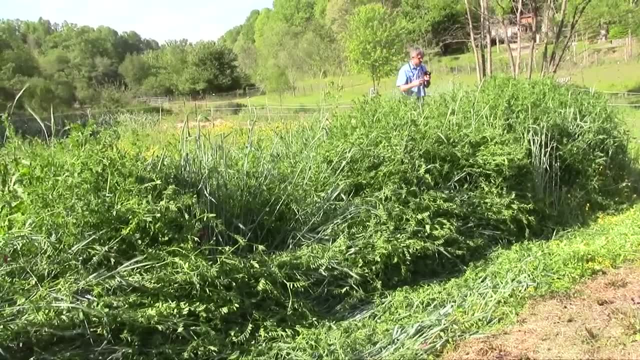 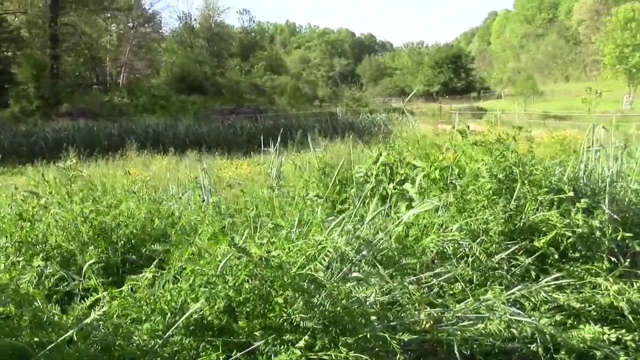 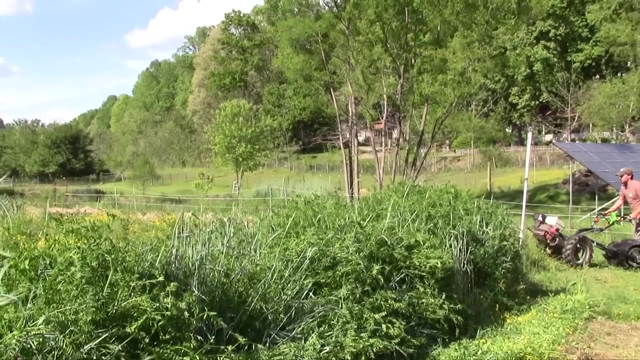 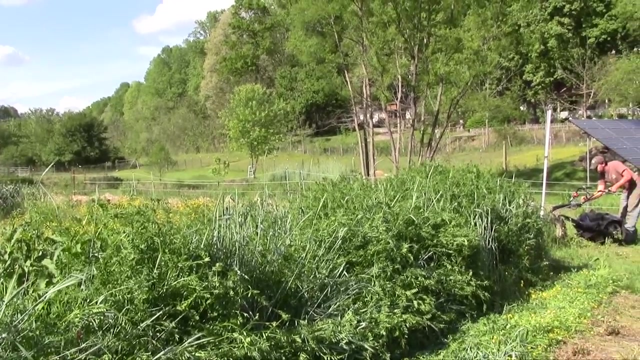 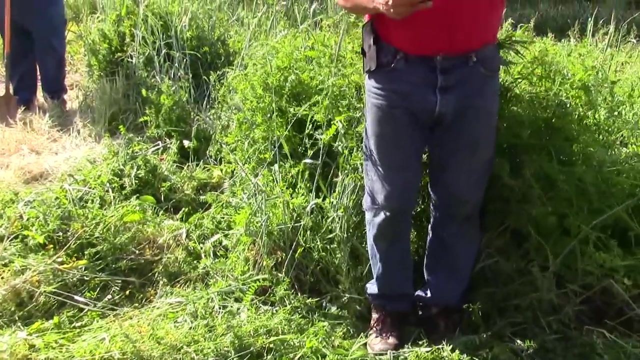 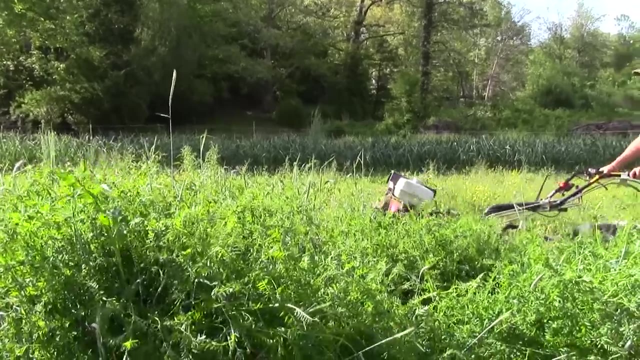 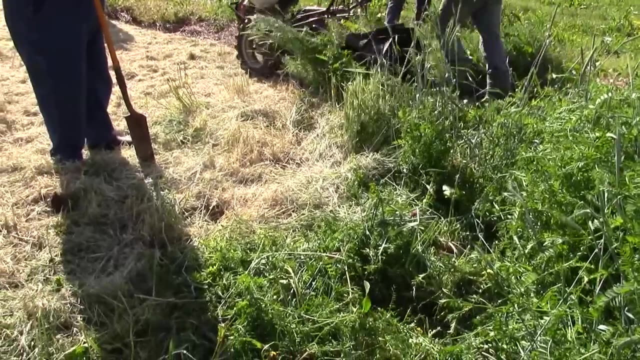 daughter's car get a haircut. nobody stand on top of this. and and guess what? those biotic glues and cementing ages keep the soil right. so fun thing to see that we saw. we just just went through a plastic can look at what we thought. we needed: more land, which 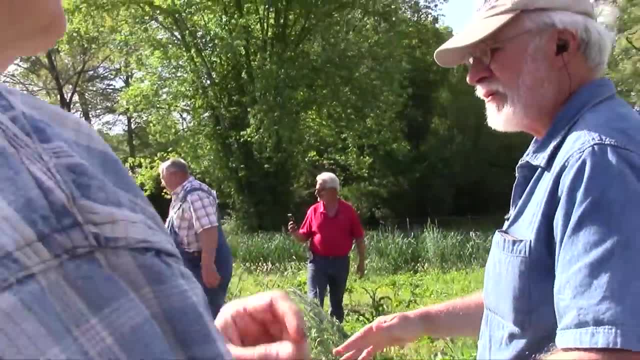 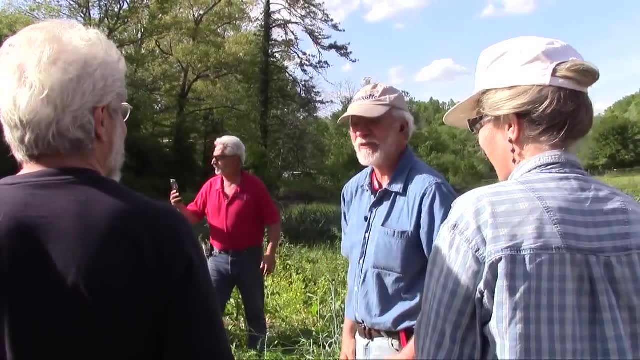 you can find local rows of blocks. take a. we used this in the greenhouse And after we finished we watched these toads like working their way up out of the cover crop right, Shaking their heads like what the heck just happened And hopping away. I've got a video of them hopping away, So that tells you how little. 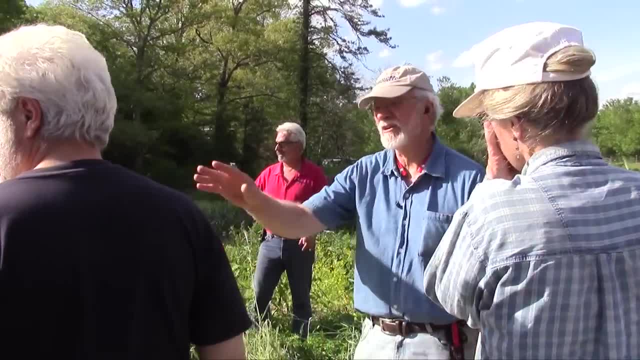 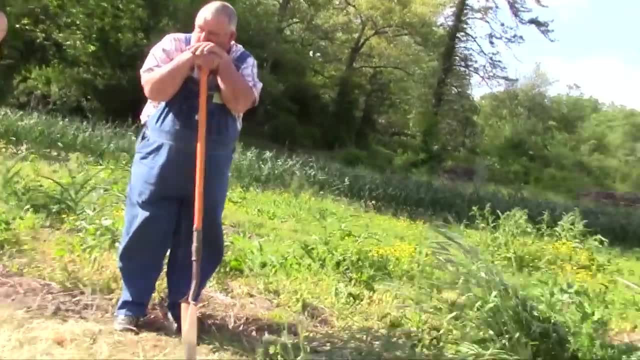 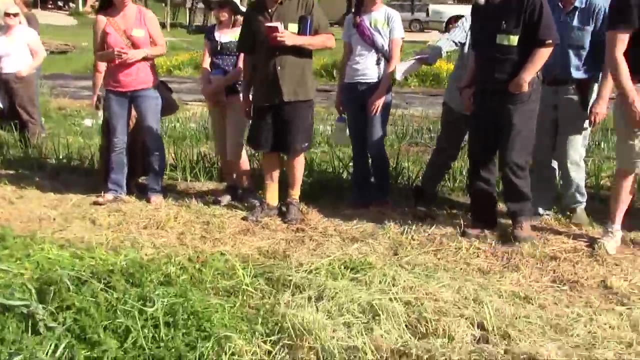 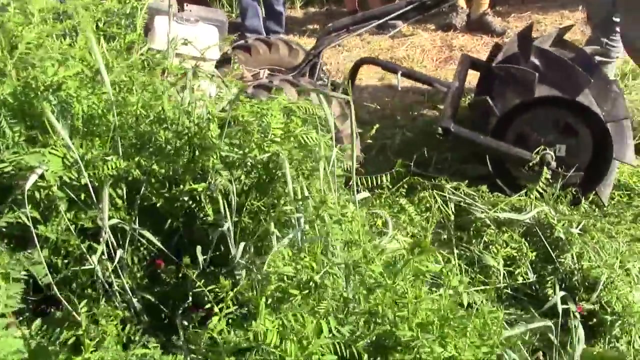 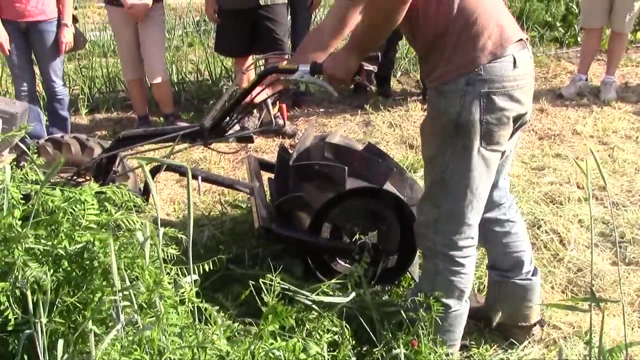 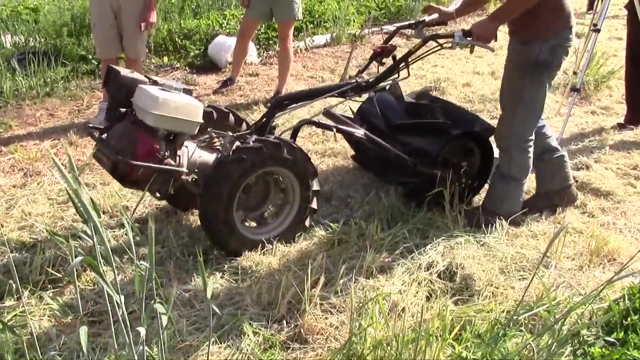 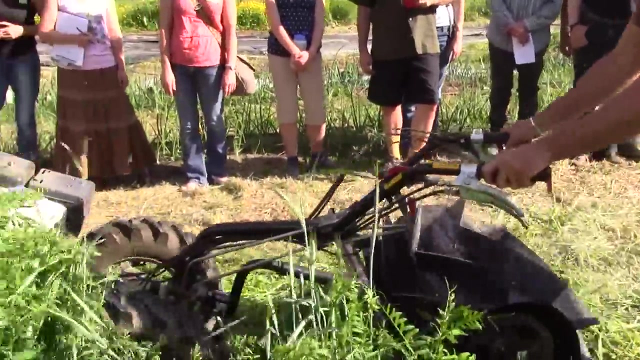 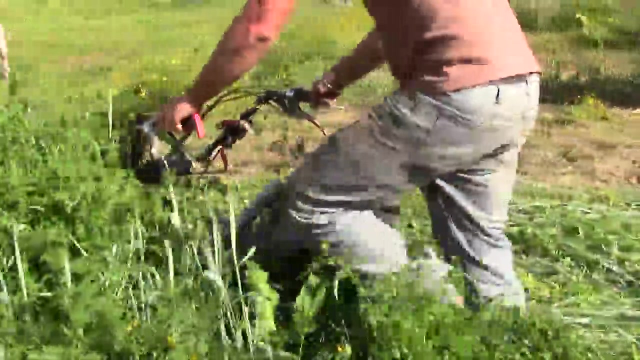 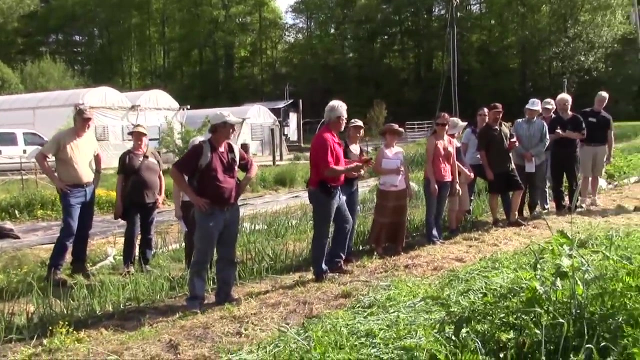 compaction. we just had Three toads carrying the cover crop. That's how they come up with the spacing. That's how they come up with the spacing. Thank you, because I always like to. I work with a lot of small producers. 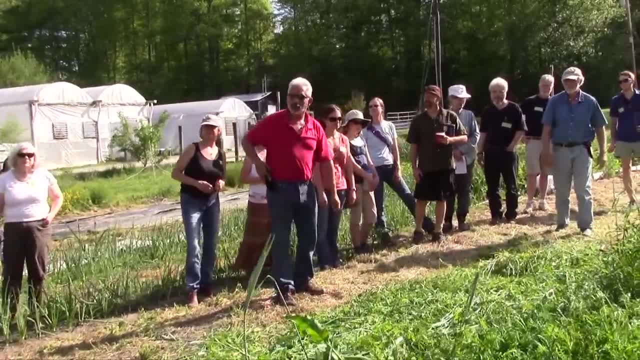 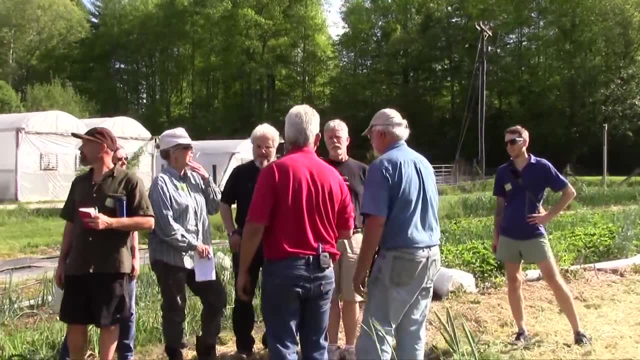 Great, thank you. Yeah, I don't know why. Yeah, Ray, at home you know, for like a smaller garden, we do a cover crop like this. We can lay down whatever. Yeah, If you had to use a board or whatever. Absolutely I want to hear that. 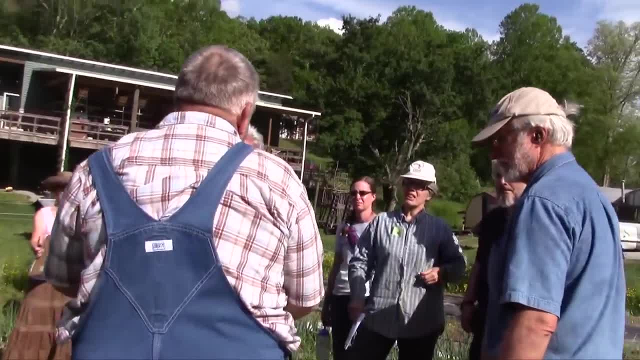 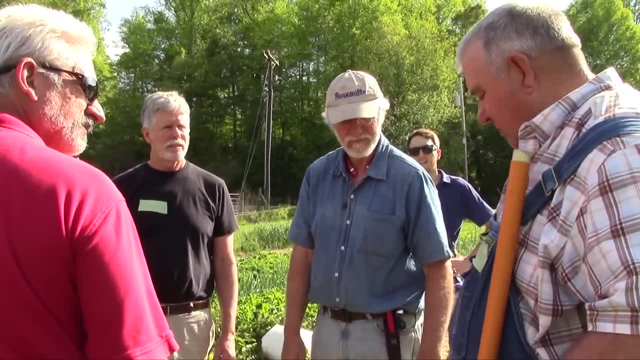 because that's what Dave said. I don't understand. You can take a. you can take a four by four, make it three foot wide. Yeah, Put two rubber bungee cords on it, some handles, then you step on it, step back, Just keep working, your way down, Just keep working. 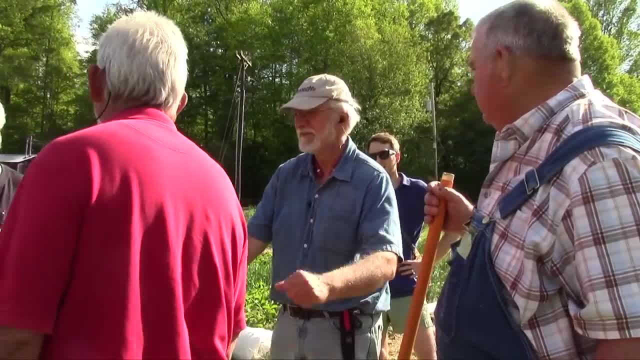 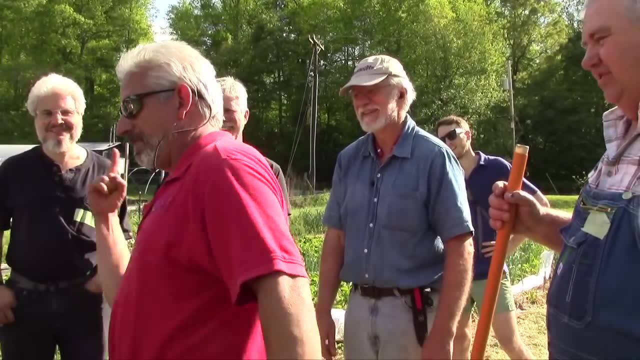 your way down. You saw him one time. he used a heavy chain. Heavy chain. Or invite your relatives and say, look, have a keg of beer over there in your hand and let them run back and forth, And then have human trampolines. The beer's at one side and the chip's down the other. You got it. 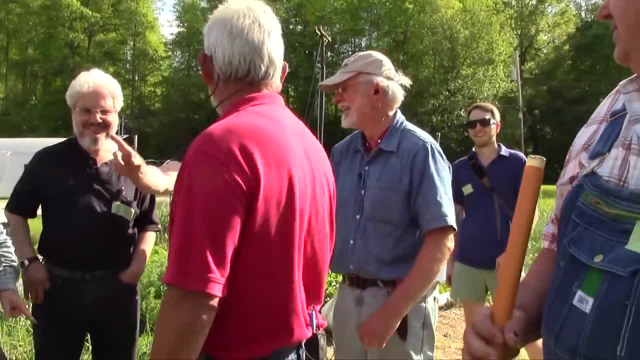 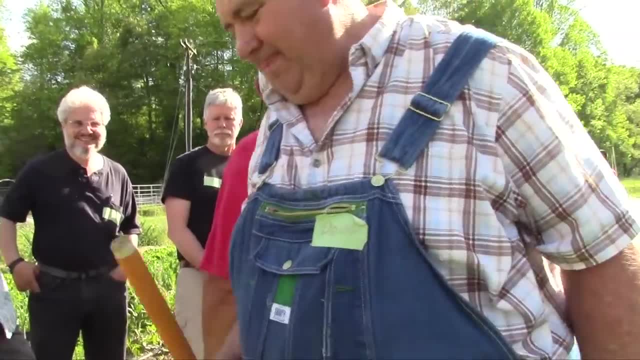 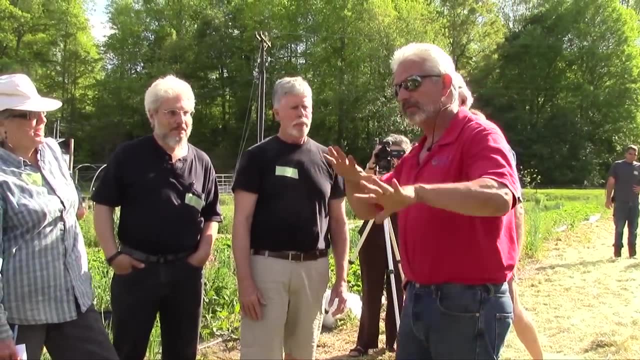 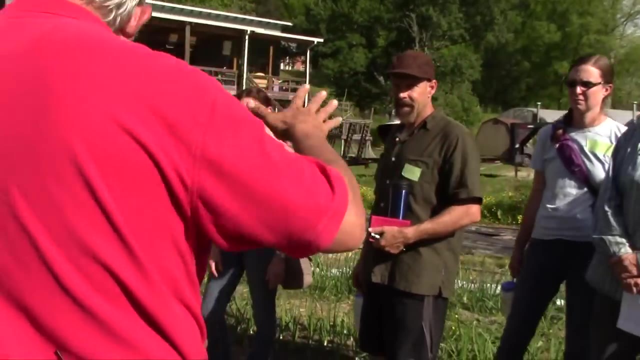 got it. Excellent idea, Just be creative. Okay, This is enough to terminate this cover crop. It's got to be very heavy. Probably not heavy enough yet. Humans are not heavy enough. But just joking around, Mike, notice how I used my daughter's car. That was enough, But here's the. 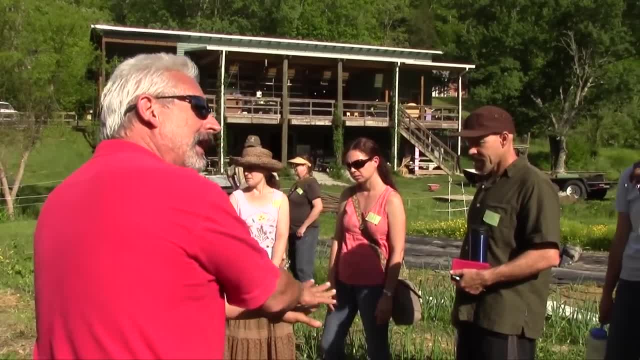 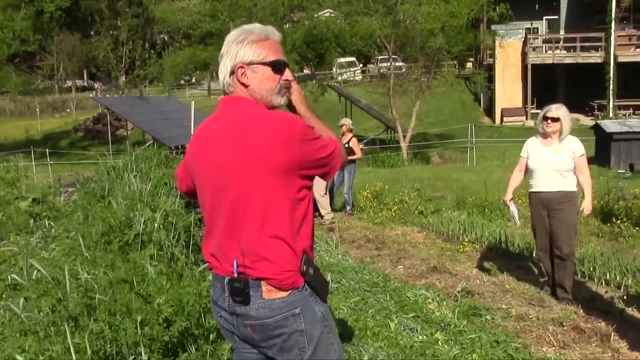 key. We have enough vetch to keep the rye laying down. That's why I watch the rye. When the rye is at the dough stage and all this thing's pollinating, it's ready to roll. Oh, it's in the. 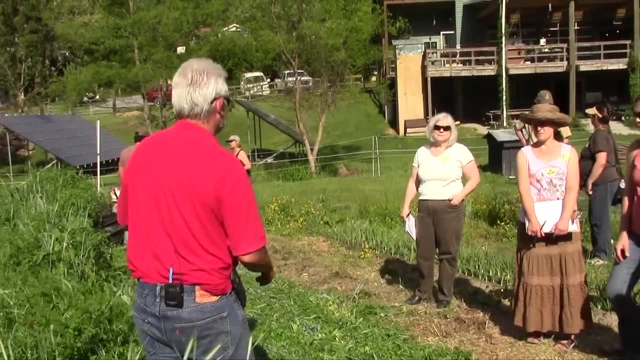 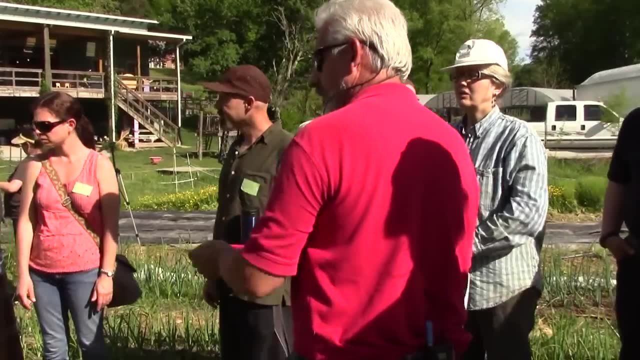 greenhouse. Look at it. Yeah, we'll go watch and show you. Yeah, let's go show that When this is starting to get this green pollen, it's starting to come off. it's ready? Yeah, so we can show. 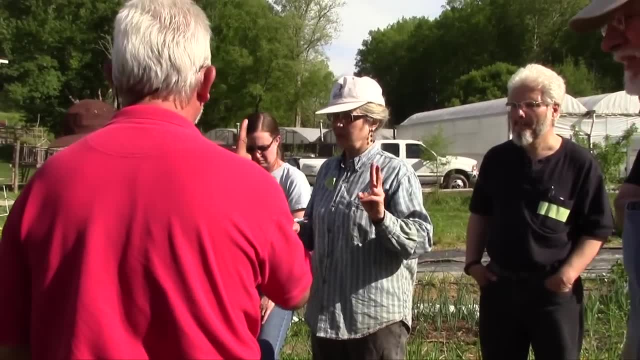 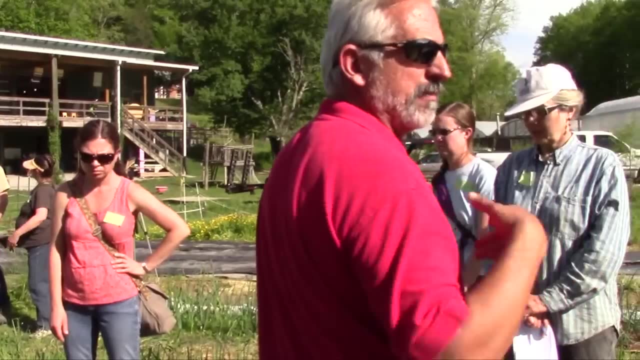 people in there. That's my indicator species that I'm watching Because that's gonna be my weed suppressant. So I want 30,, 35 pounds to the acre as my weed suppressant and then put my mix in. So let's go look at that and then head to the other place. okay, Then we'll go to the. 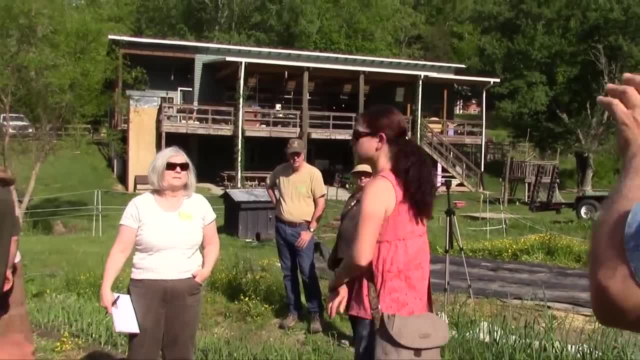 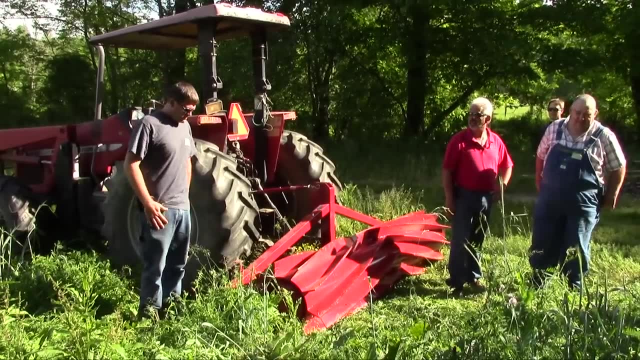 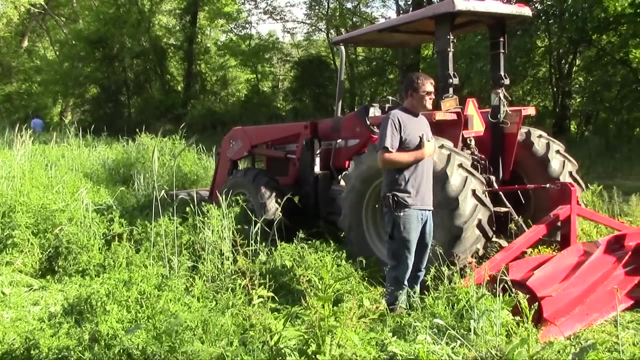 other place. So, okay, I'm worried about getting to the other place. okay, I'm gonna tell you what the management was here. Ready to go, Marsha? Okay, so we've watched this farm a long time. I farmed conventionally up here a long time prior to coming to work with the Living Web. 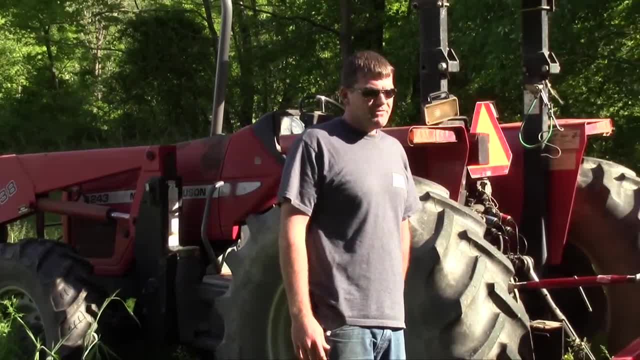 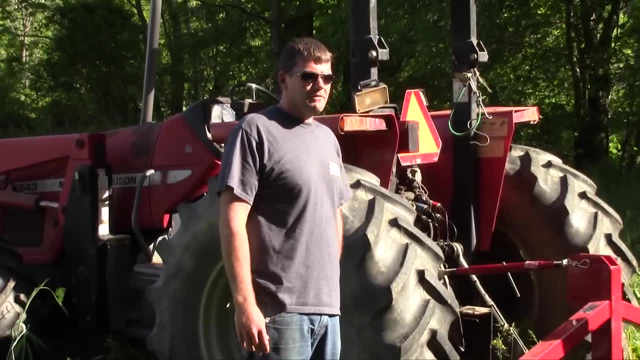 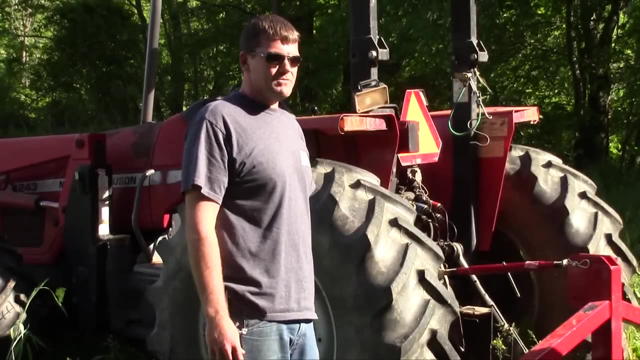 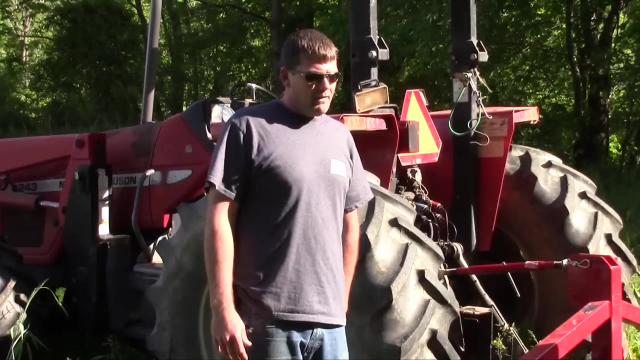 This farm was conventional tomatoes on raised beds, on plastic, Conventional every meaning of the word. A lot of chemical use out here weekly, whether it was needed or not. When we purchased this place, the folks that were leasing. they were a little sore and they left all their rows. They pulled their plastic and stakes. 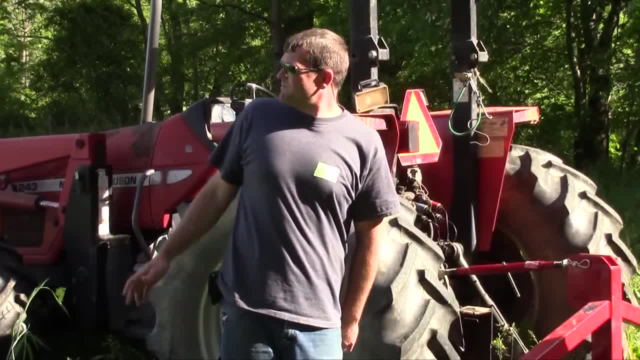 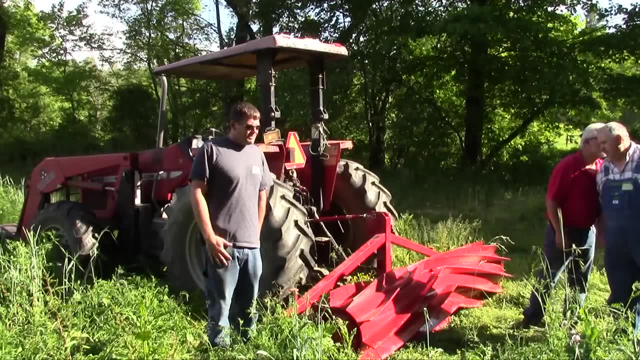 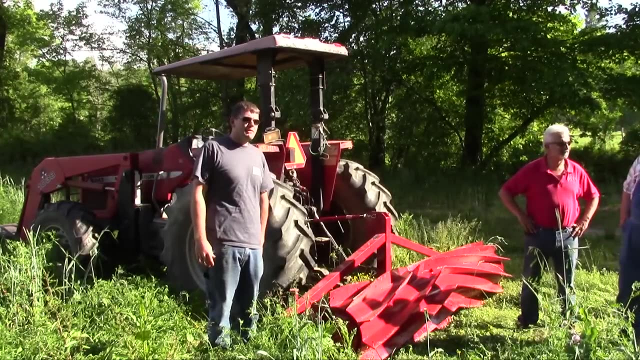 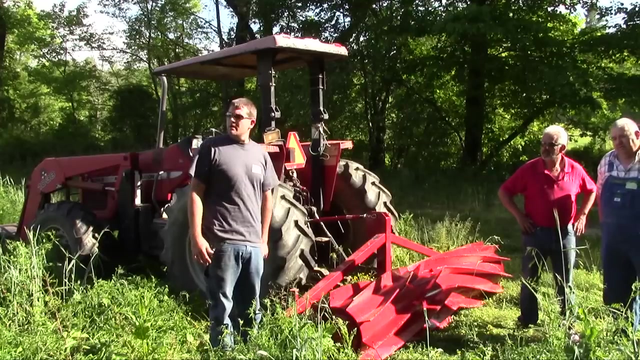 but they left all their rows. So what we had were just an ungodly amount of rows on six foot spacing, just sitting there looking at usholding water. every time it rained, Weeds were six foot tall or more. We decided that we obviously had to prep it down to a flat surface. So 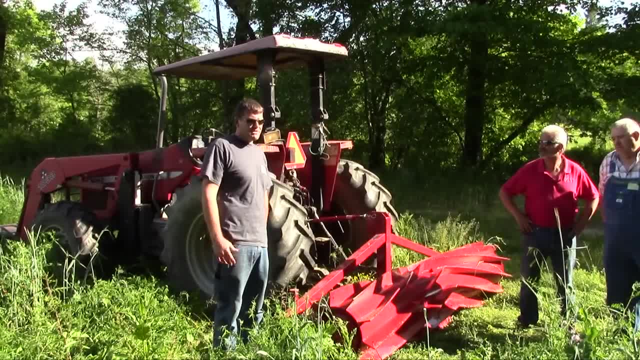 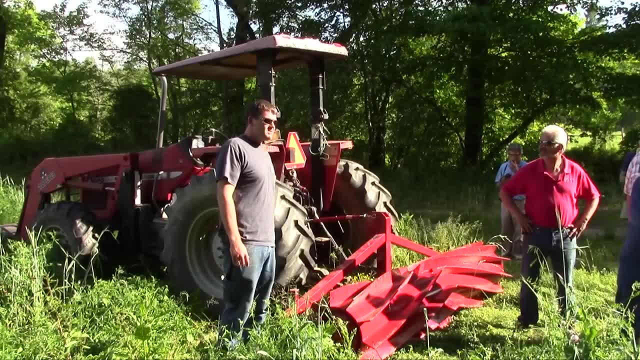 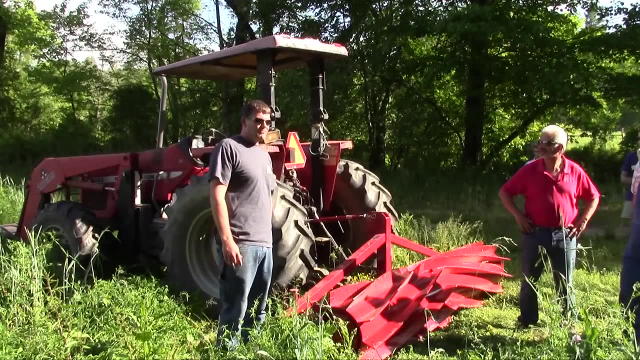 we came in with about a 12-foot bog disc and disc'd everything down and got it smoothed out. And then we came back with a 20-foot finished disc and really tried to smooth it out as best we could. from there we drilled directly using an eight foot no-till drill. 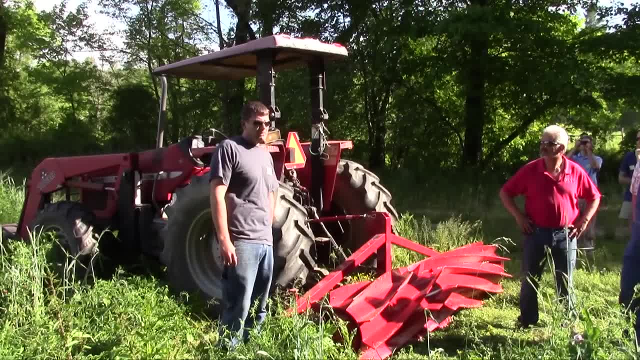 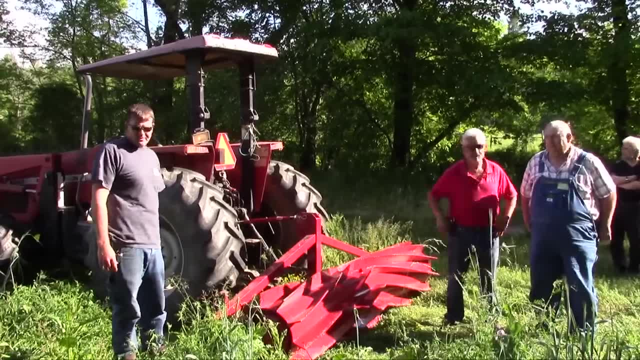 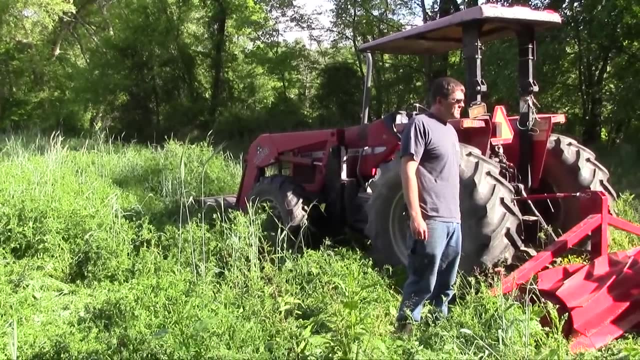 planting the the diverse species that you see here, and that's that's really where we are as of right now. this is one year's growth. this is one year's first cover crop. this was planted- we did this in in early october. we got it established. we got it established probably. 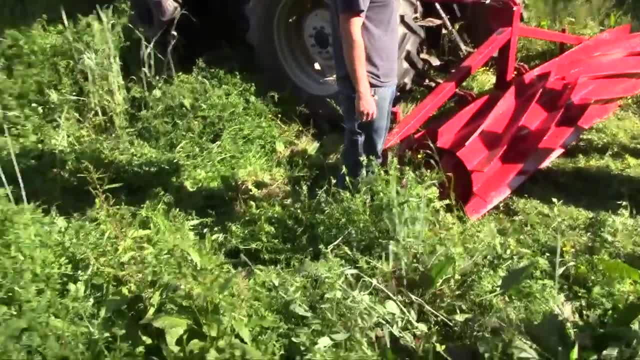 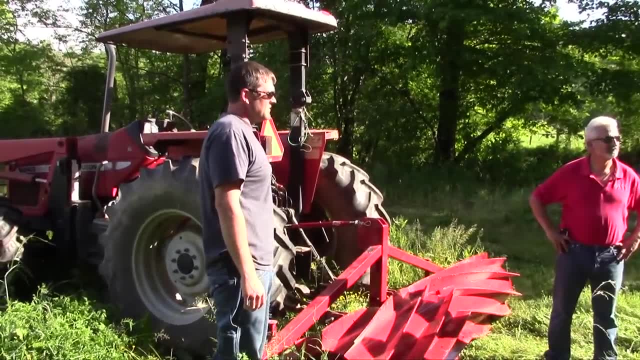 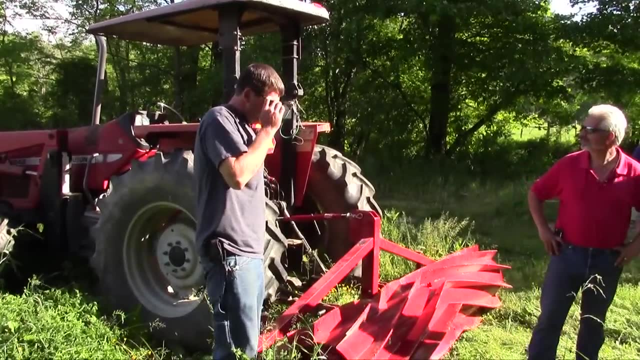 six inches prior to winter and it survived obviously well through the winter and just really started taking off as we got into spring. and you, what's your intention now, after you roll it through? well, what we're, what we're going to do right now, is we're going to. we're going to. 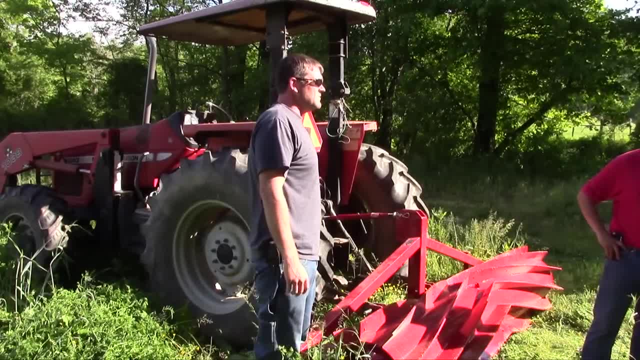 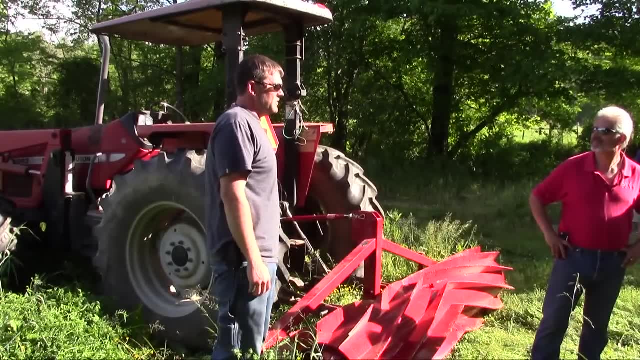 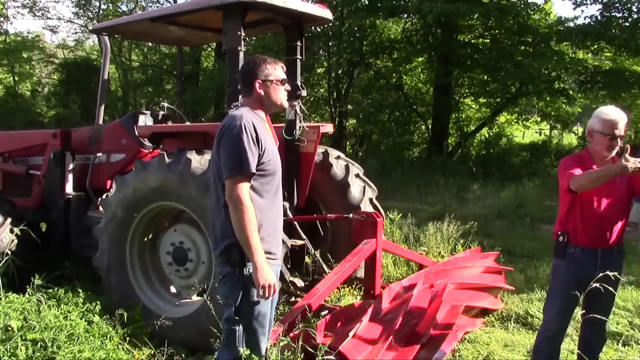 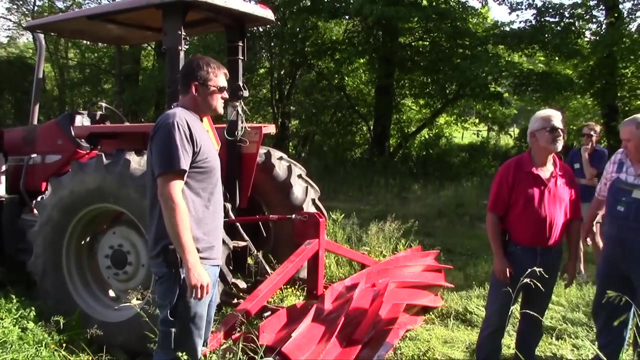 plant it with a summer species cover crop and we're still collecting the equipment that we want to use to push forward with venison vegetable production. We also have intentions of grazing animals and doing a number of different things, just on a succession. Just to do soil building Right, just on a succession. This 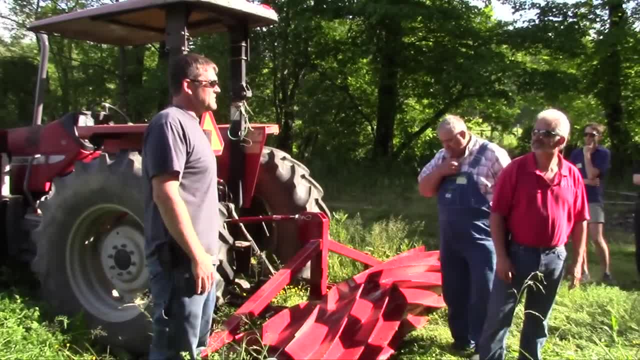 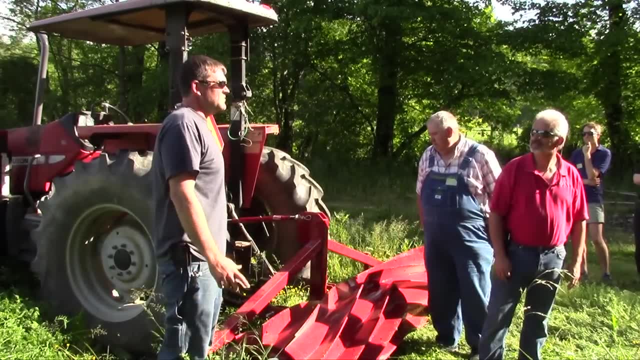 obviously would be very expensive for someone that was just trying to start out. They would be not using their property initially, but it's the investment that we have to make to get the ground where we need it to be: to produce organically, If you think about what they're. 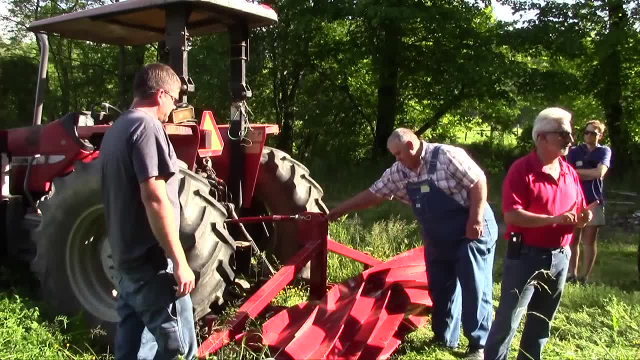 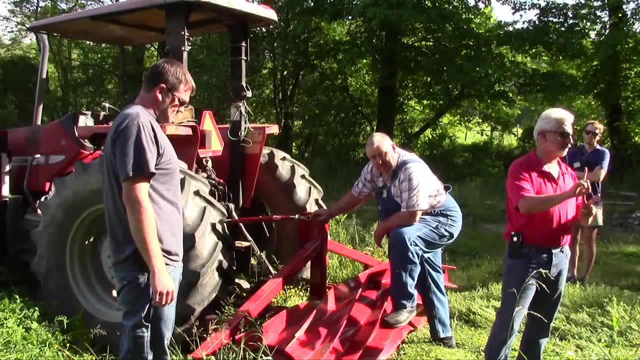 doing, they're really saving money in the long run because in two years of these mixes it's going to make a huge change and get them turned around. If they started with a conventional system, they're going to be in that vicious cycle and never get a chance to repair. So 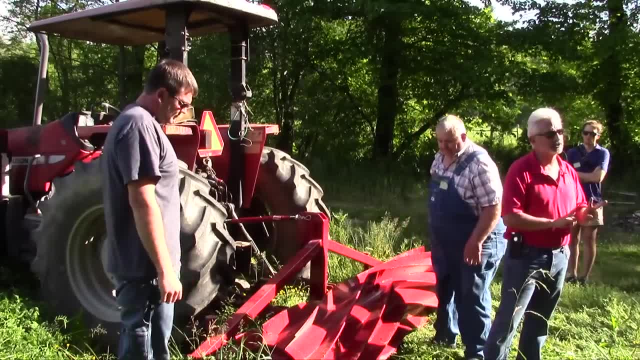 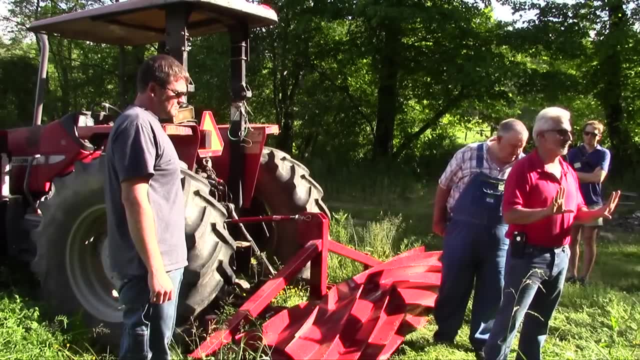 we're doing bioremediation here and we're using the covers and the biology to do that And we're going to show you. after he rolls, we're going to dig. We've already seen aggregation and guess what? we saw folks, An earthworm. We saw one earthworm. That gives us hope. 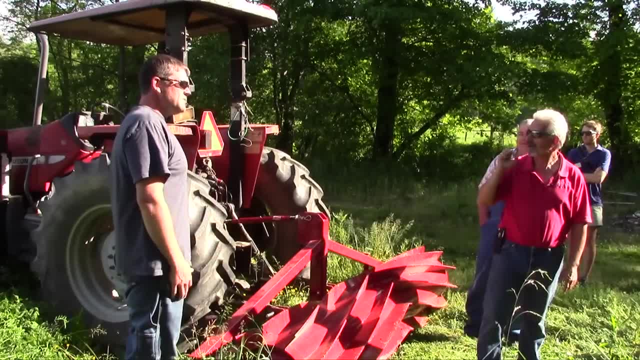 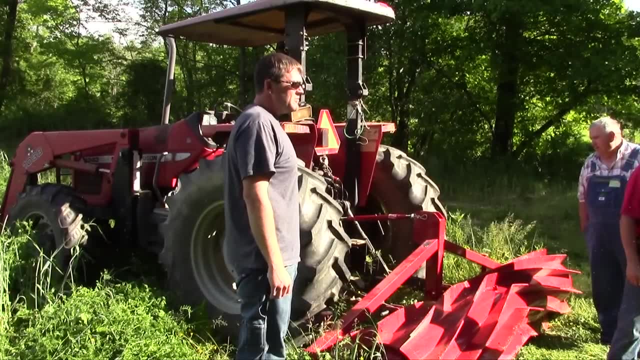 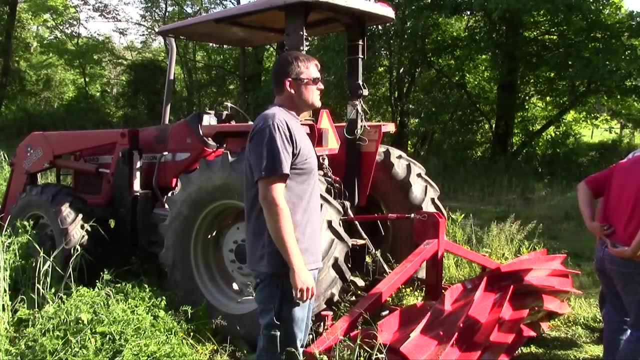 So that was encouraging. Yeah, this stuff has been worked and worked, and I'm talking disked and plowed and just standard conventional practice, but it never was cover cropped. There are no soil tests They'd run through and instead of doing any soil testing or anything, just try to put. 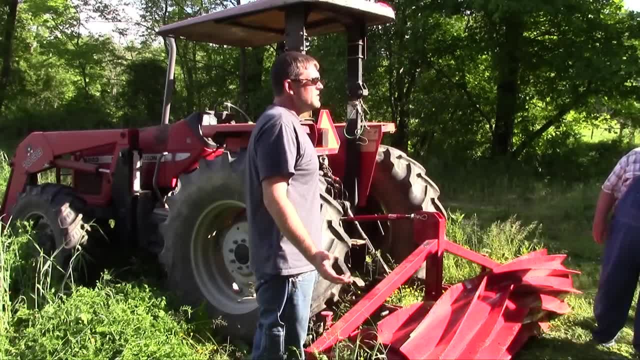 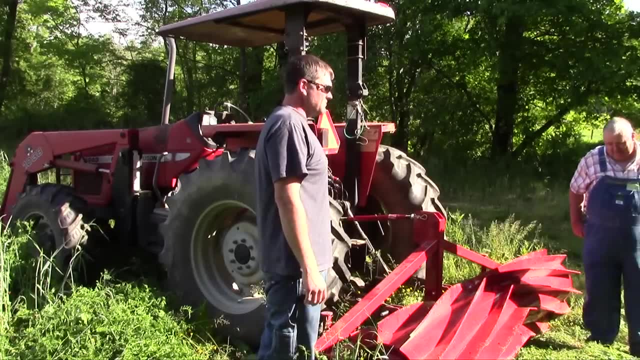 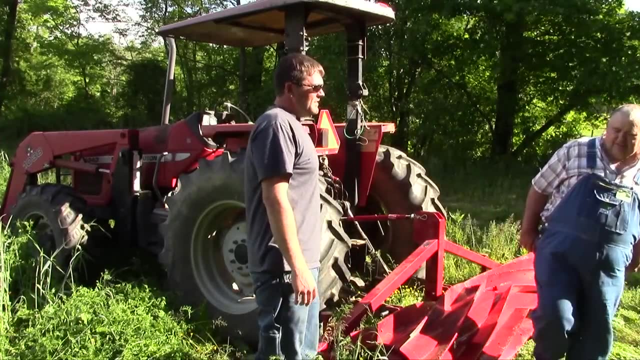 about a ton of lime per acre every year and let it go. Never did anything to really try to improve the soil. Their motto, how they treated this stuff was: if we're not doing as well as we were last year, we just add more fertilizer. 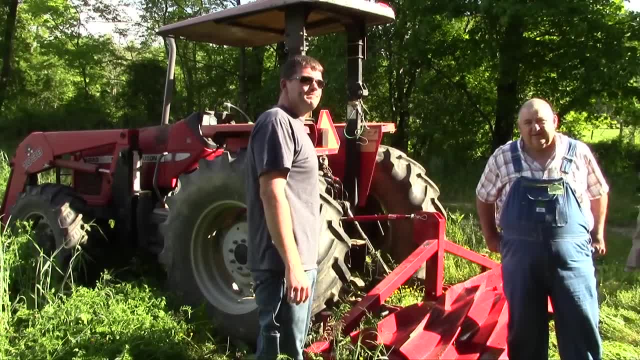 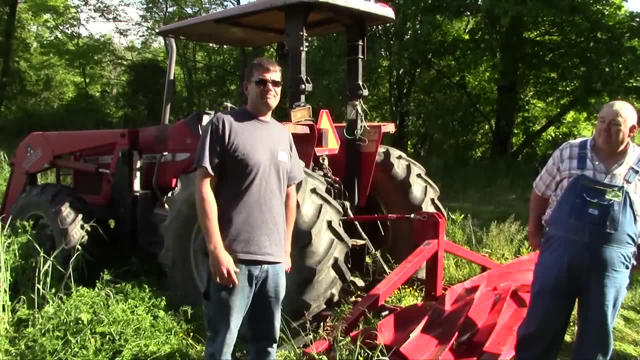 How did you get? you didn't amend this, obviously right, You just let it. you just went right into a drill. We disked everything down and went right in and drilled it And your soil test said that it would come out like this. I mean gee. 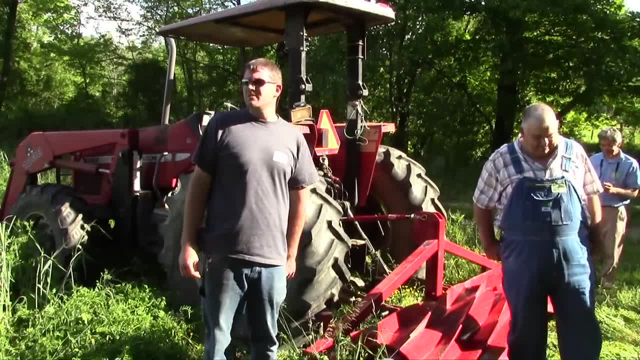 It's Mills River, If you know what I mean, It's Mills River. It's Mills River. If you know what I mean, If you know what you're, if you, when you're looking for, when you're looking for property, 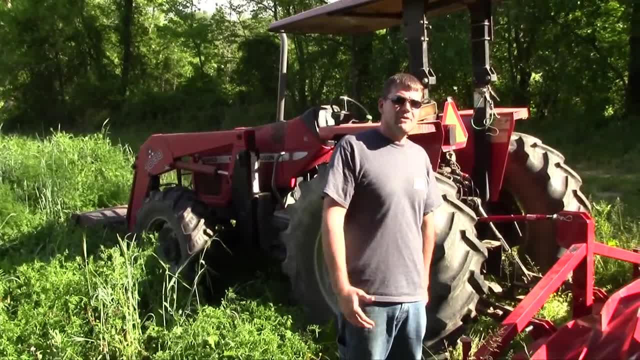 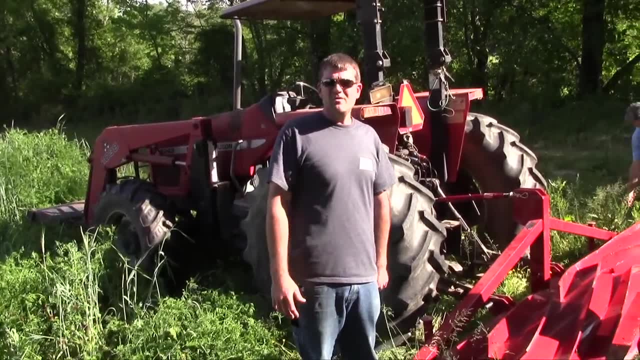 in Mills River. if you know what floods and what doesn't flood, if you know what's been taken care of in a certain way, you know where you're looking, And we worked on this property purchase for the better part of a year. 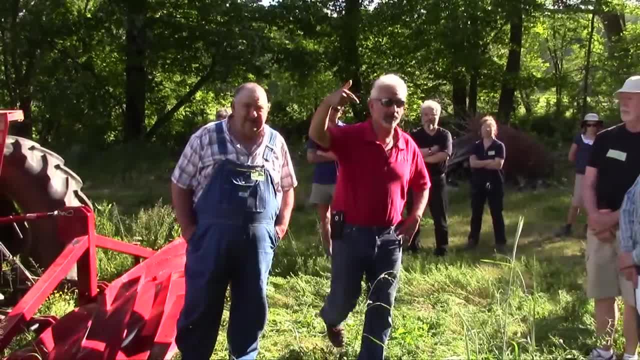 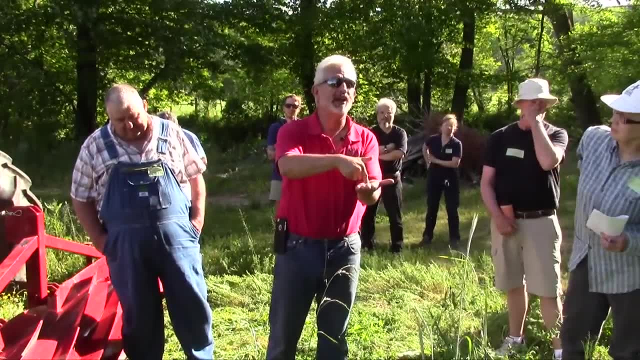 And remember we told you about that soil web on your iPhone, Mm-hmm. It will tell you if that soil has been flooded. It's that the type of soil types. It tells you all that on that, on that web Soil web app. It comes from our agency. It's the soil. 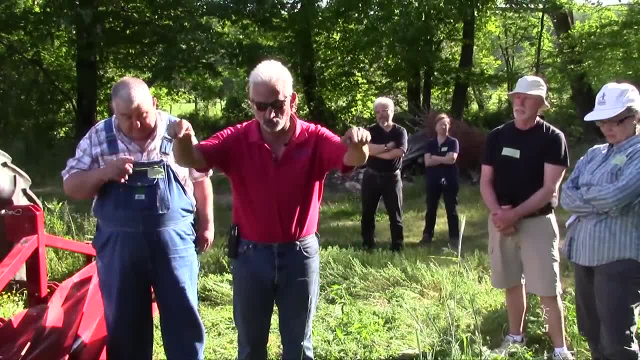 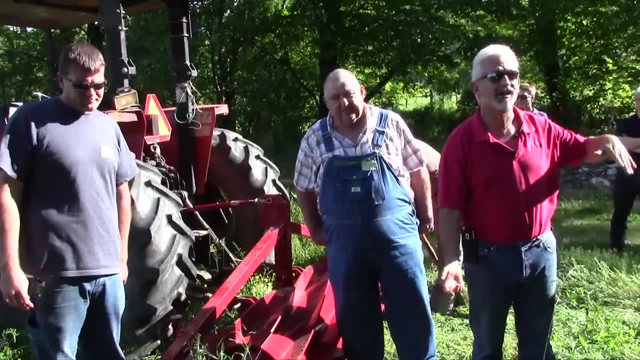 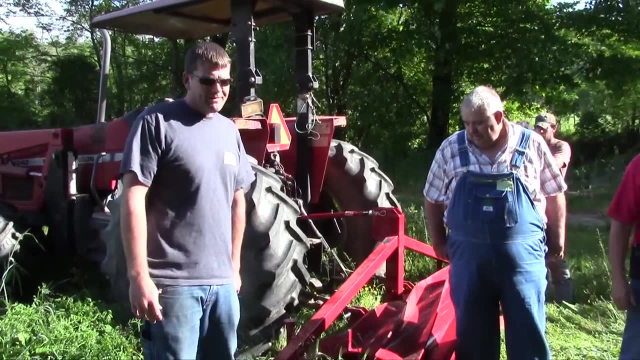 survey. So if you get that app, it'll tell you what the soil type, what's the hydrologic unit here if it's used to flooding like you talk about. what's the depths of the soil? Very cool app. The way that we chose this property was you, we have. we got you know. word of mouth from: a couple of generations prior to me, which helps always. Mm-hmm, But what we really? what we really did was we had two hurricanes in 2005,: Francis and Ivan. They were back to back during the fall of the year. They put a lot of rain down. 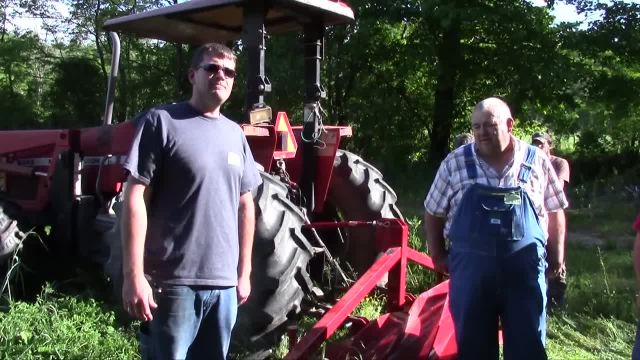 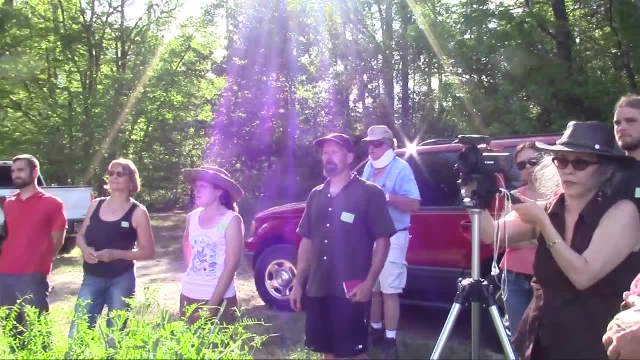 What we did was, while everything was raining and flooding- myself, my dad, a couple of other large conventional guys- we just got in the truck and went and rode, Saw what flooded and what didn't flood. Mm-hmm, These fields, every single, everything we own right now. 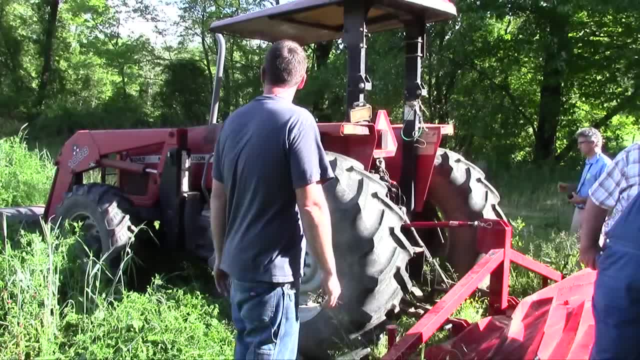 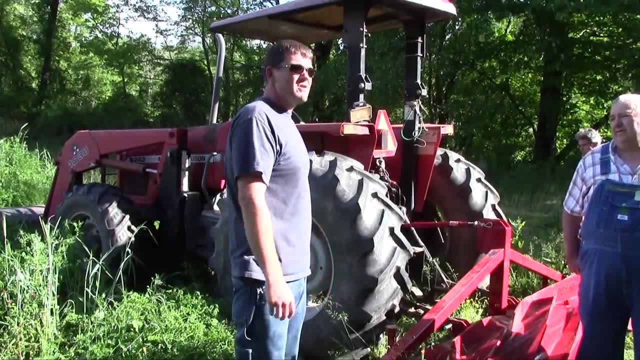 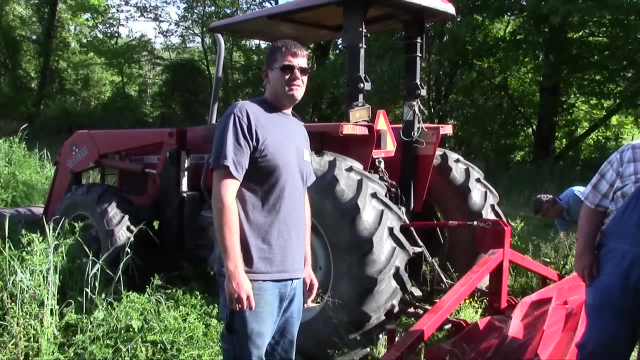 Mm-hmm, Right here, The worst thing that's ever gonna happen out here. unless if we get something worse than two hurricanes three weeks apart, about maybe 30, 40 feet off the riverbank, you're gonna be okay. You might lose a little bit, but you're gonna be okay. And unless 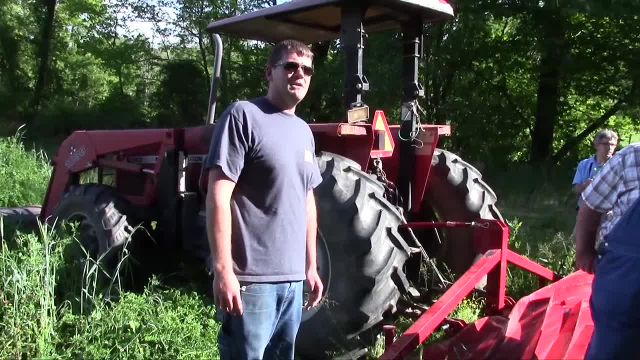 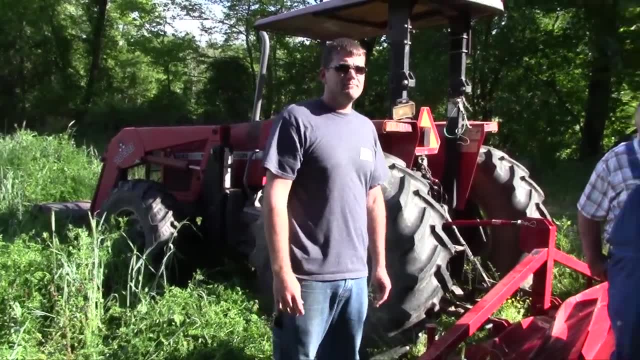 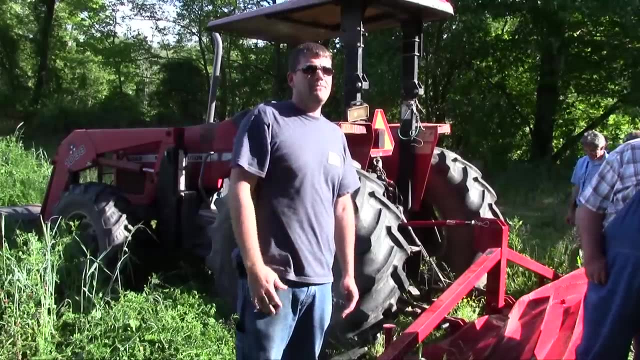 if we have two hurricanes back to back, it's never gonna come out. It just doesn't come out. It comes out way down low in the valley below the Ingalls where we were. How much acreage is here? It's 49 acres total. There's 34 acres of bottom land and 15 acres of upland. 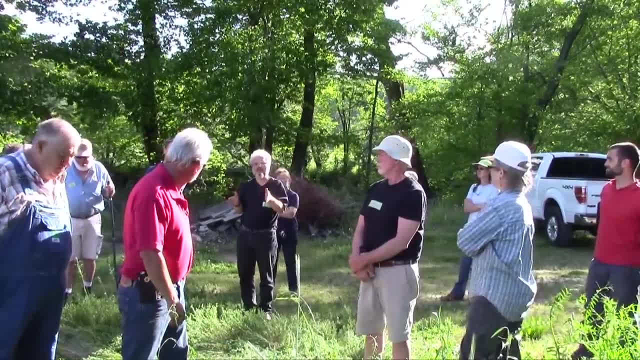 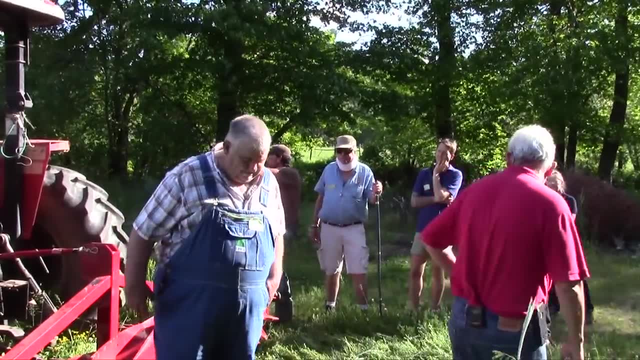 So is there an explanation of why it did so well? Is it in the mix? It is in the Seeding rate, The seeding rate, Seeding rate. We seeded heavy. but I think that just the explanation really is just Mills. 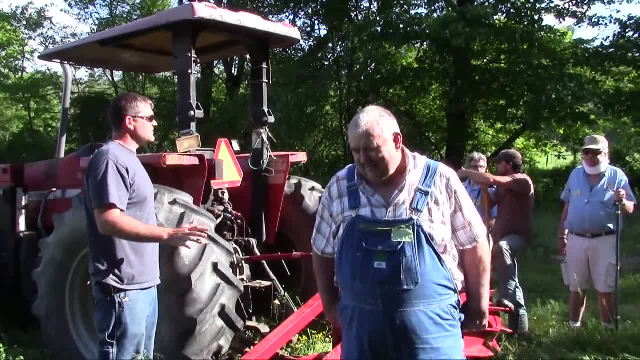 River just got good ground And if you're on the right ground, you're not in too much clay, You're not in too much sand, It just has a real good field. All right, Well, thank you, Thanks, Bye. 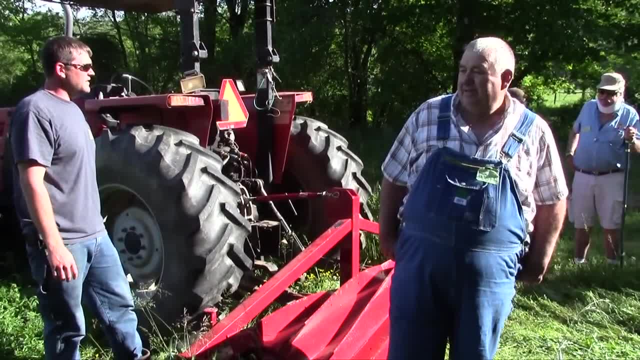 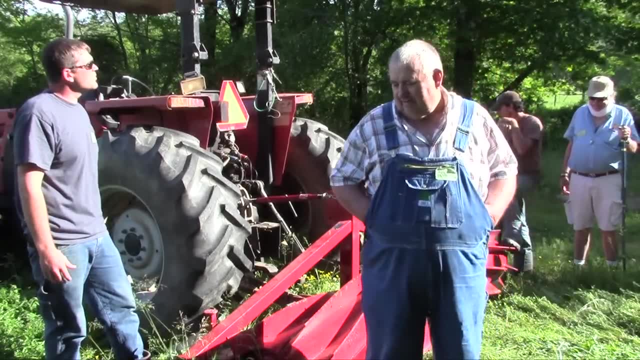 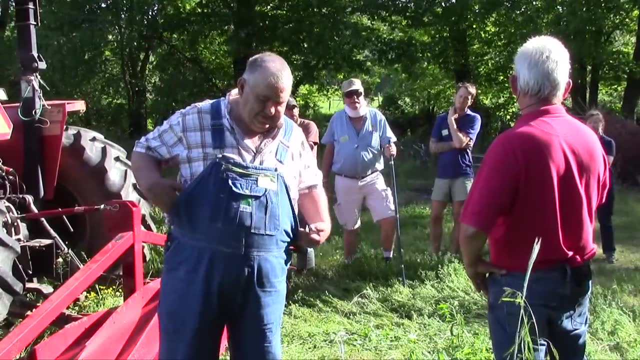 Bye, Bye, Bye, Bye, Bye, Bye. really nice mix of soil and I had all the confidence in the world, prior to us owning this property, that we could do anything we want to do out here. and another thing you never forget: the power of diversity, right synergy, yes, nature's. 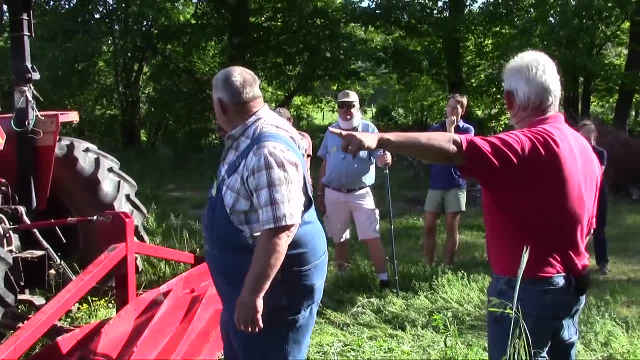 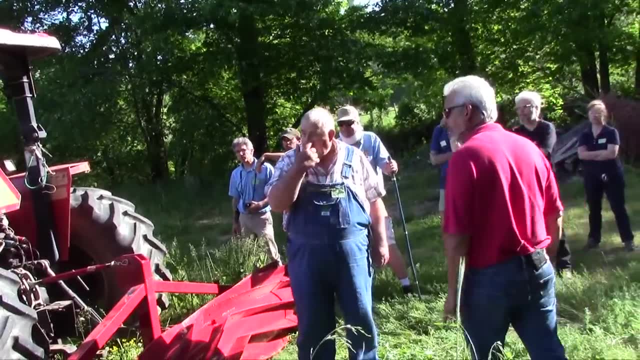 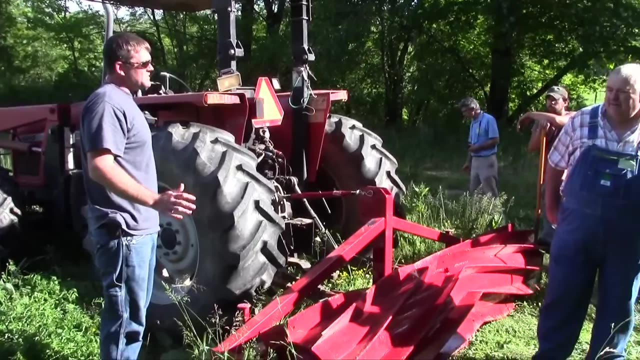 first is she synergistic. that's what we did here. don't ever underestimate her power. I think we way underestimate that. yeah, I certainly looked around and saw some some of the diversity coming up better than others initially, but as soon as we got into spring everything came up that we planted. I'd say we have. 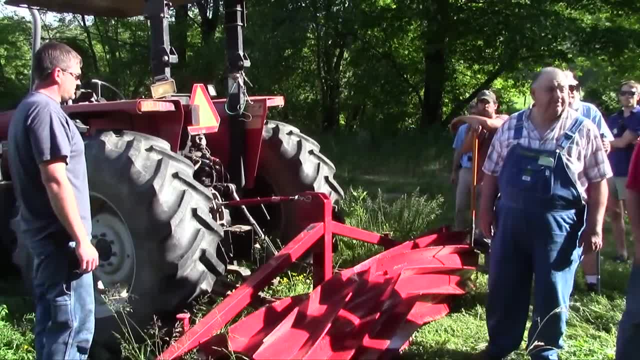 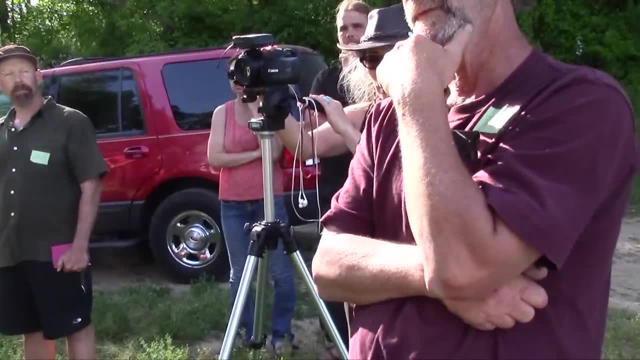 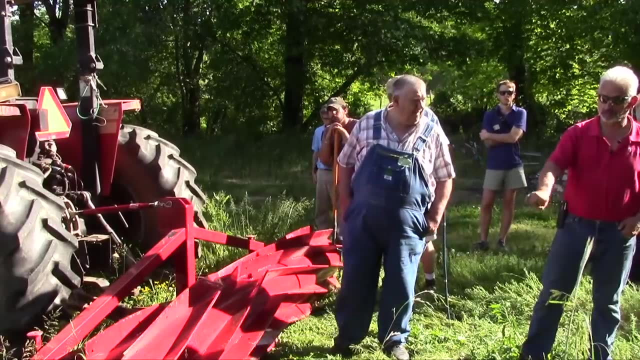 a hundred percent stand. really, you'll drill for the summer cover crops. we're gonna. we're gonna drill right into this. how long will you let this lay before you drill? two weeks, maybe three? this has got to be brown, this one. there's a reason for this one being brown, because the vetch is really thick. 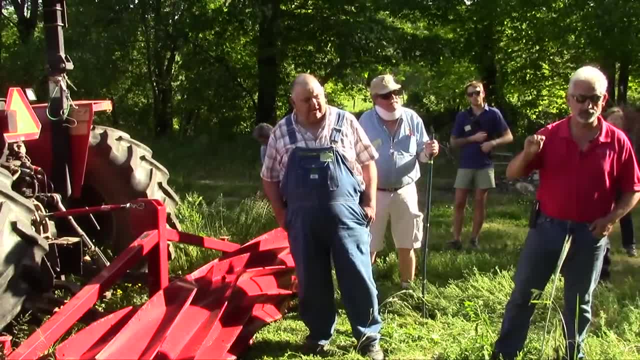 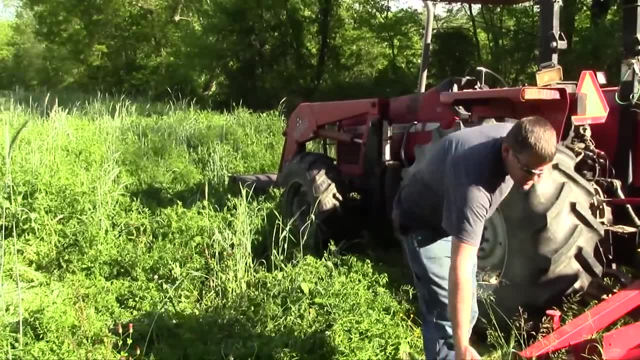 you're gonna get it tied up in the equipment, so we're gonna want this brittle huh. completely opposite, we told you the other one. right well, this vetch is adding us a lot of nitrogen. it's, it's viney and it'll just give you a lot of. 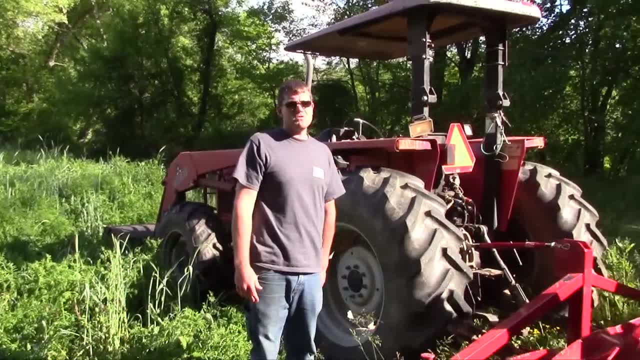 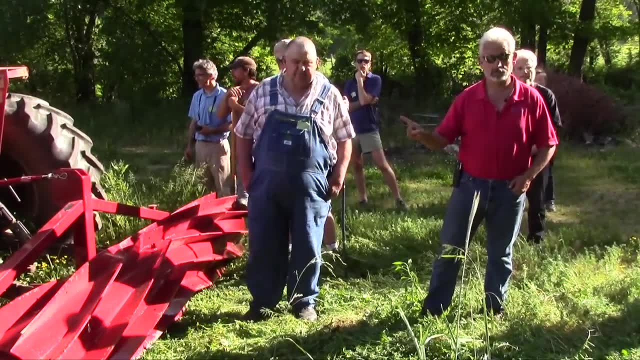 trouble if you don't don't let it run its course prior to trying to drill it. but my mix that I have, I have very little vetch in it. I'll do it green. yeah, this one you won't. Dave's got a lot of experience. you'll see that in the next couple of weeks we're going to have a lot of. 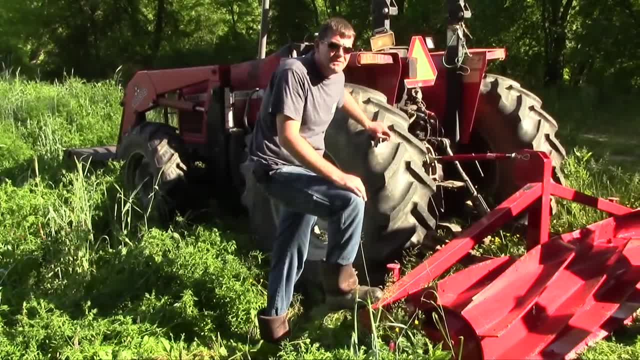 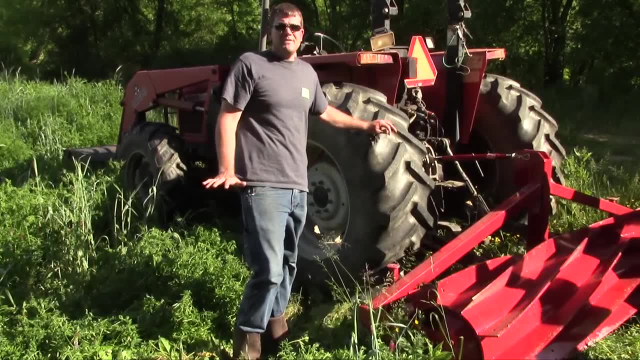 vetch in it. we're going to have a lot of vetch in it. we're going to have a lot of headaches. yeah, we went at it almost approximately twice the recommended seeding rate for a number of reasons, but mainly we've we're trying to revamp this. 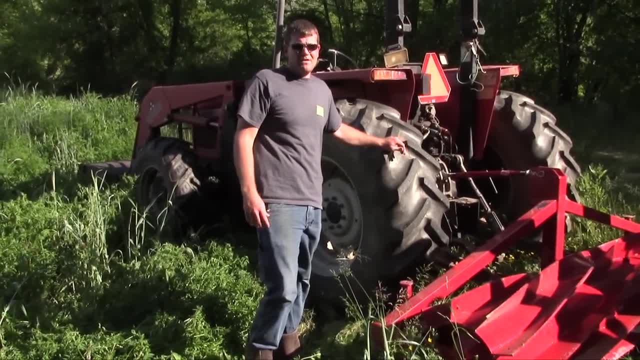 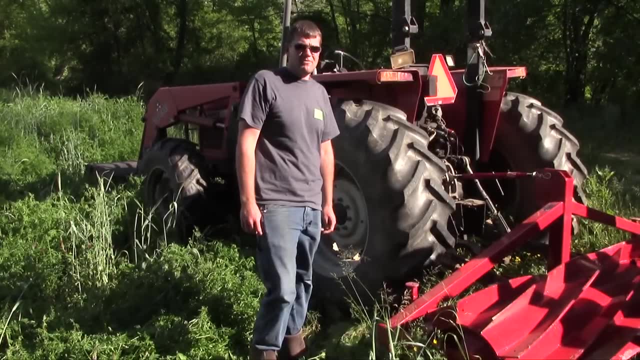 soil. we're trying to fix this ground, so to speak, and at the same time, we're trying to drown out any weeds that we don't want, choke them out, get them out of the way, make them not be part of our program. it doesn't work 100%, as you can. 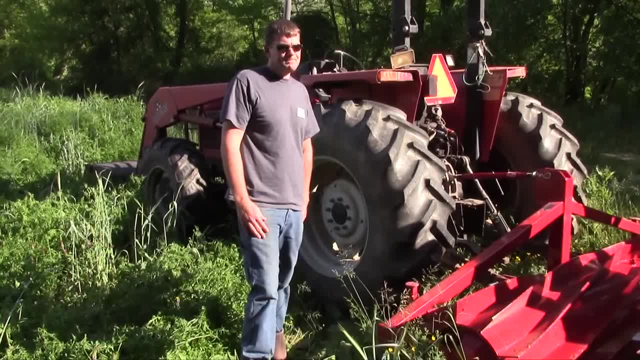 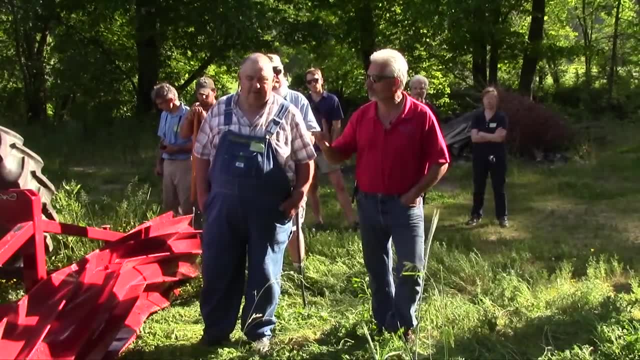 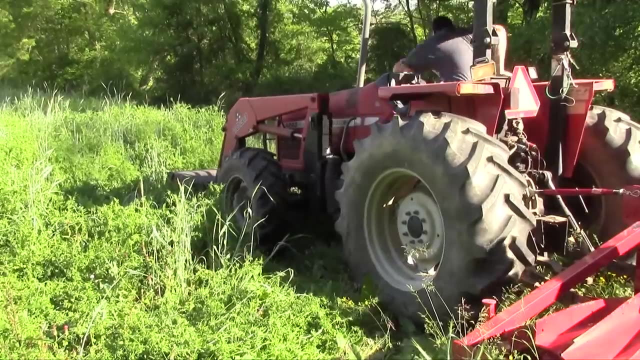 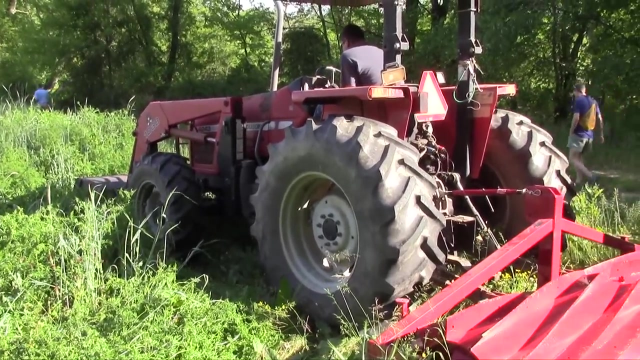 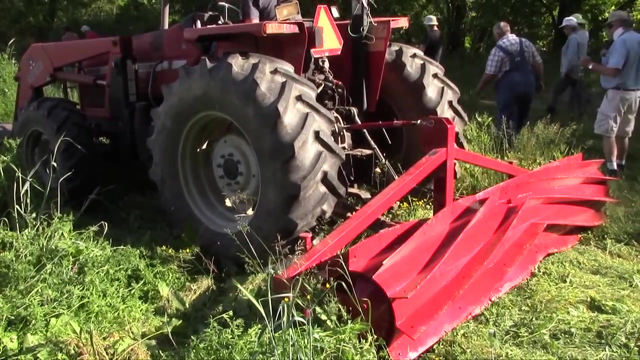 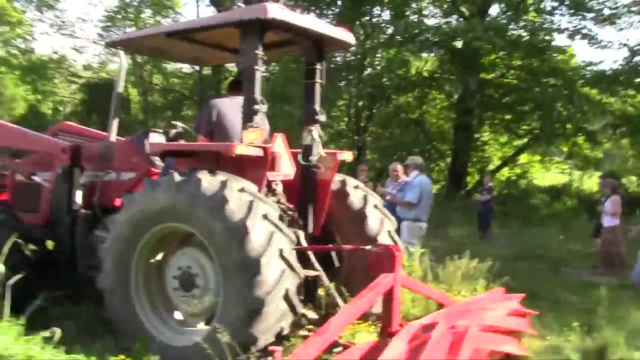 see right there, but look at how much the covers suppress the weeds, tremendous. nature is not a nudist. it wants to be covered. I always remember the powers of the covers. go ahead and roll this and then we're gonna dig in the field. beautiful, let's go. 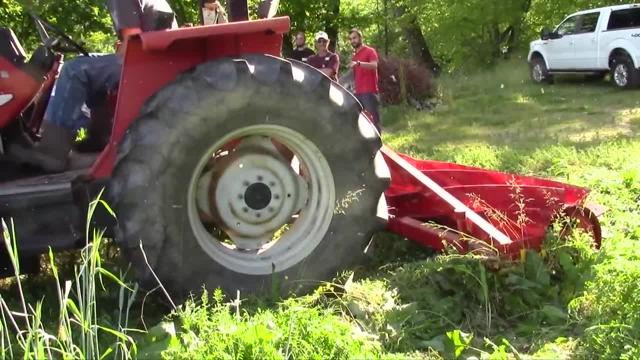 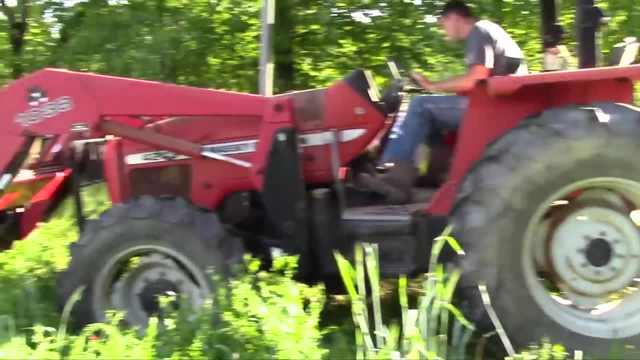 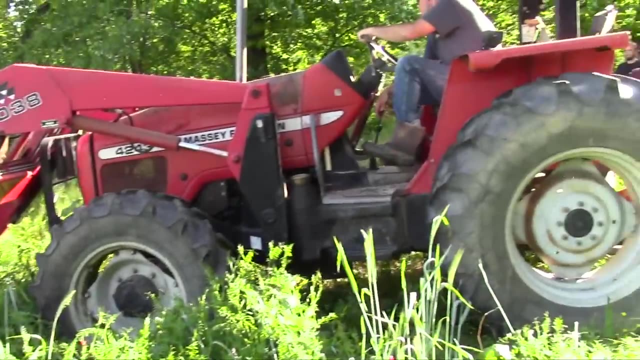 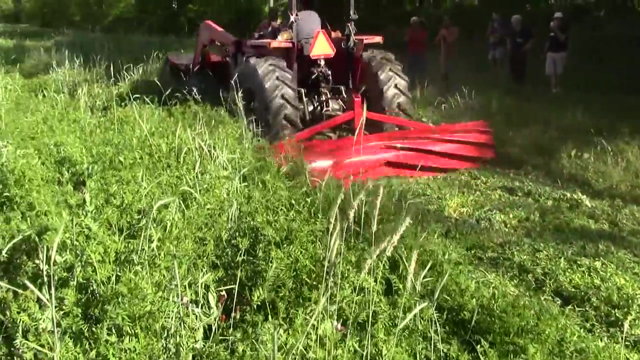 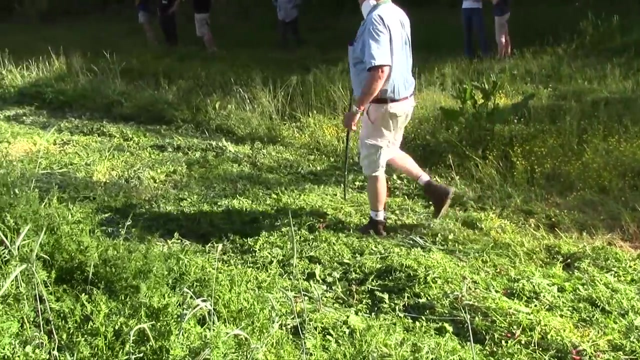 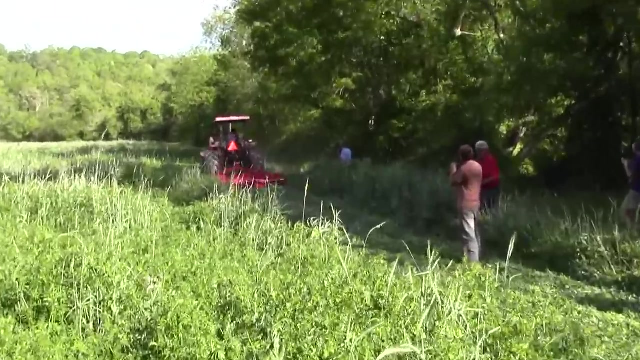 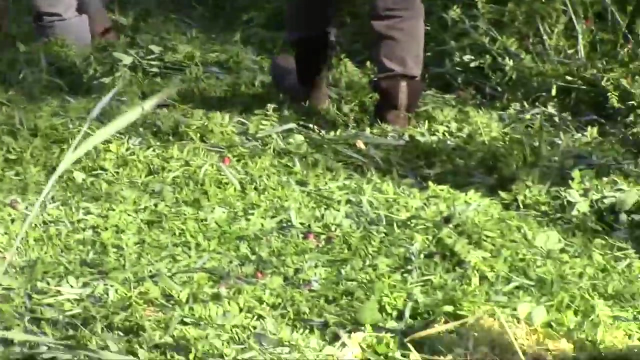 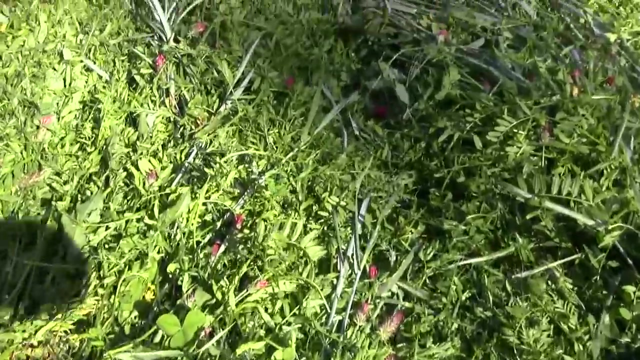 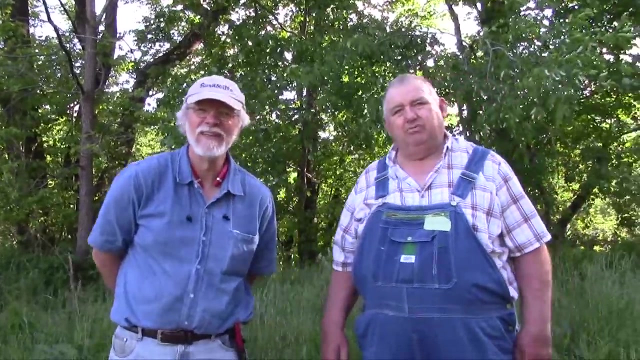 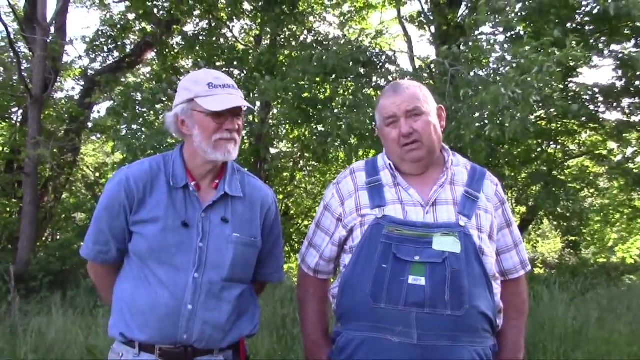 yeah in, yeah, yeah, yeah, yeah I said: do you think one pass will kill it? yes, one pass should kill it. you should be able to see it turning blue tomorrow, the next day, and I'll tell you whether it's going to die. if it stays dark green, it won't. and then we'll come. 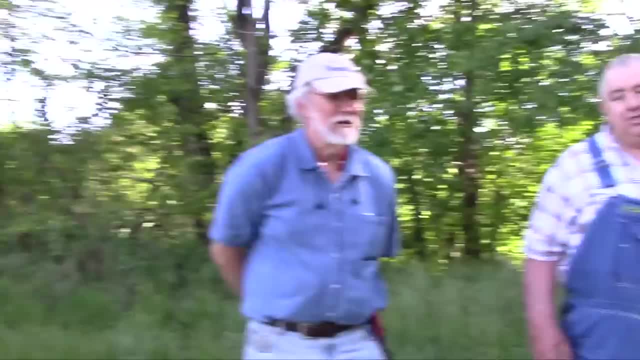 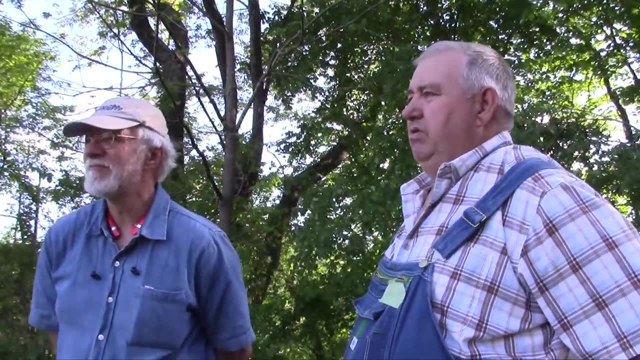 back and hit it again. that's a nice, you know, yeah, but it should. it should take it out. purple bloom in the vetch. the rye is blooming, what you want to do? if you got close then, in this regard, to listen to the tractor, you can hear that. 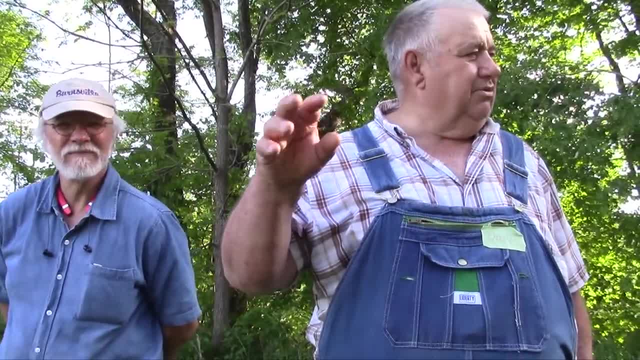 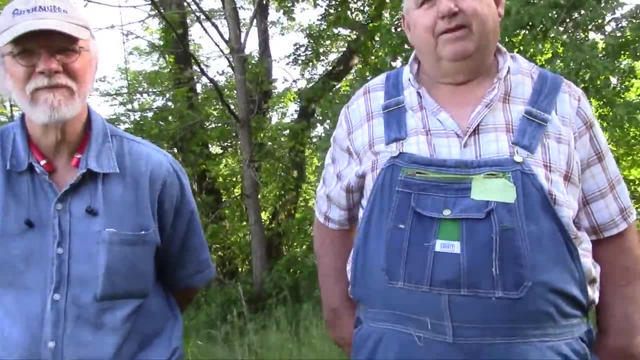 crop. popping and cracking like popcorn, that's when it's ideal to roll. when you hear that, popping and cracking like popcorn, popping, yeah, yeah, right. well, the stems gets hollow. yeah, they get hollow, and so that's why it's popping. that's the best compost material, yeah. 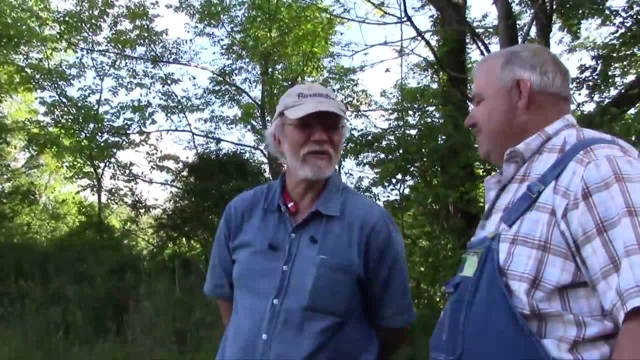 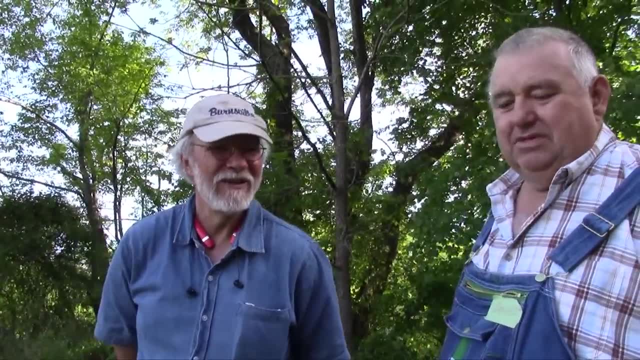 how quick can we get that cover crop seed here Tuesday or Wednesday? all right? well, let's get that set up. you know I'll get on the phone with my nonprofit, make sure the money's lined up and we'll just go for it. you know we want to get it in. 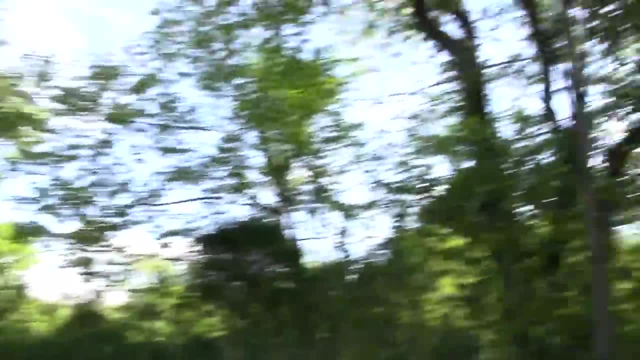 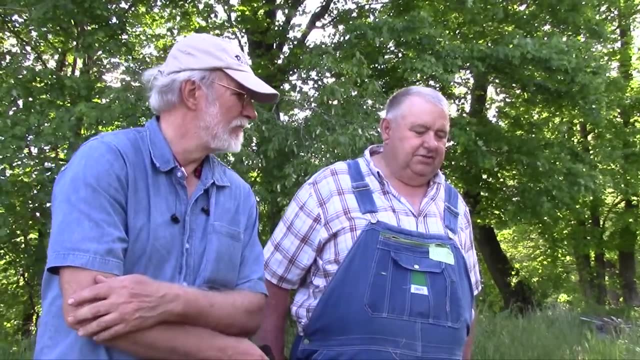 get established. you know, I'd like to get your and Ray's opinion about whether or not we should change the mix for the mugwort suppression, or should we just go with the same diversity? I'd use the same diversity because we got big, tall sorghum stand and pearl millet. 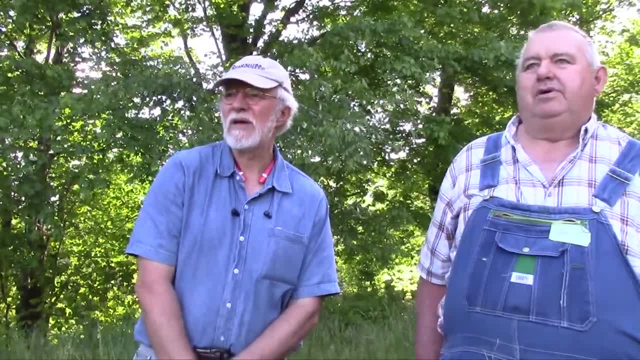 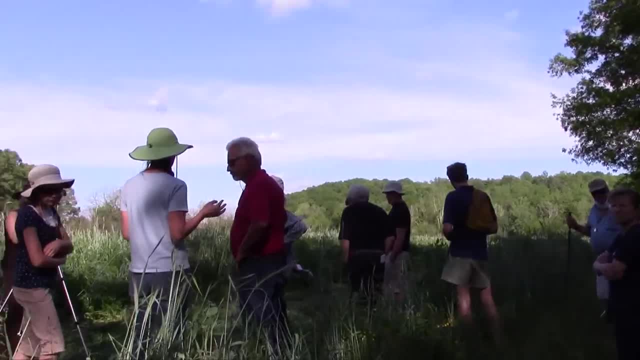 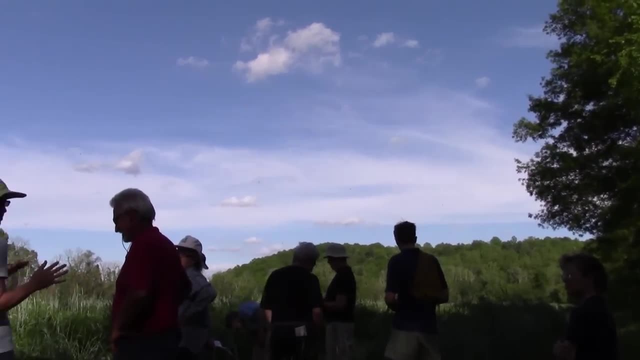 mm-hmm, I think it crowded out. you go do it, okay. yeah, going over there next. pardon, we're going back there next, if we have time, we sure should. yeah, the lady before me live there a year, but before that has been a riding field so it had been gravel and floor, and then she actually has planted some cover. 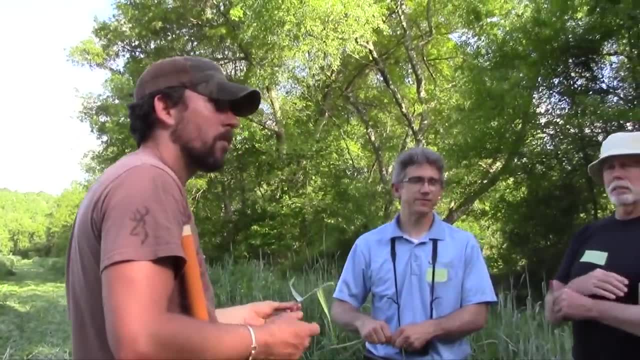 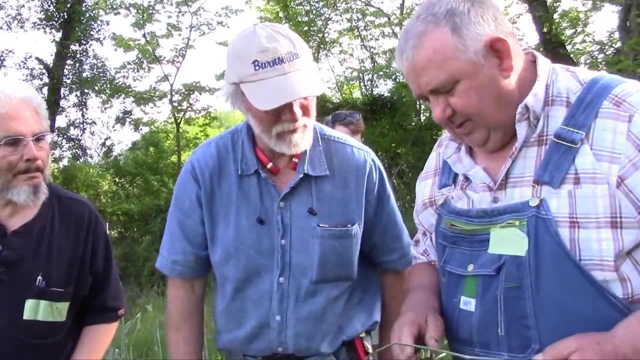 crops and I'm trying to restore it, but I'll lay there for a year. 45 foot sprayer. you can spend about the same amount like a small spring sprayer. yeah, 3.9. yeah, it's a lot less than the long one. yeah, let's make you do that. 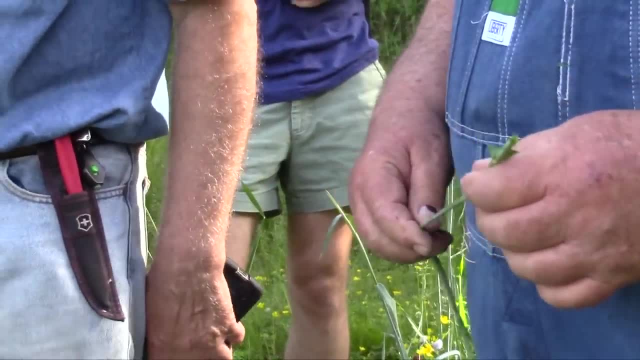 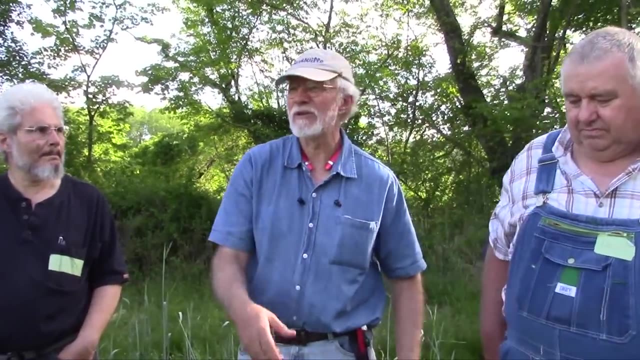 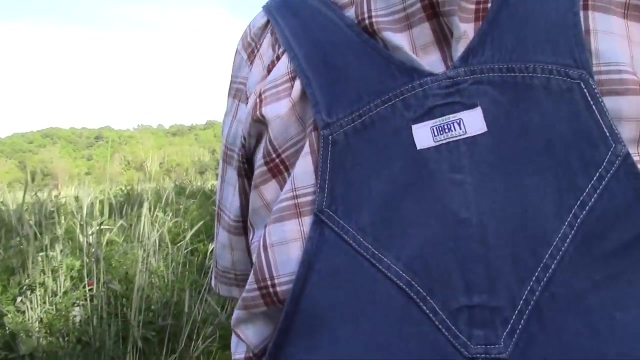 So we're going to look at the soil and then, if we have time, I'd like to go back and look at the mugwort for a minute too. We've basically got a half an hour to look at stuff, talk about it and get back to the field. 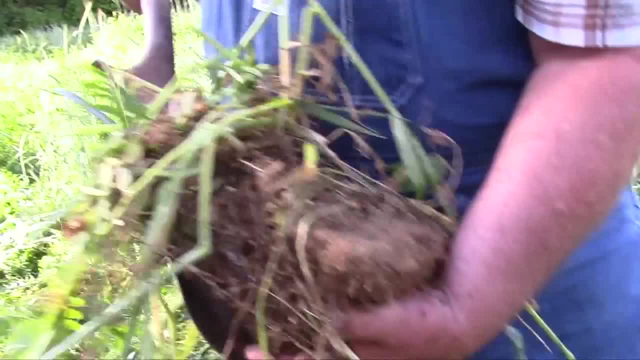 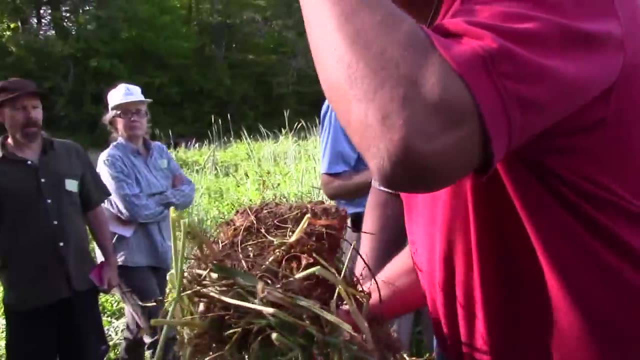 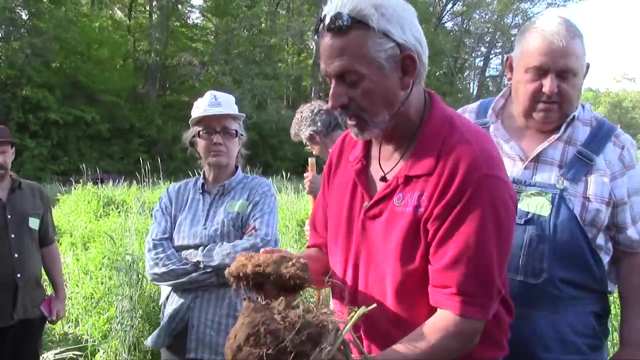 Where's Ray? Come on, Hey Ray. Yes, sir, Here. Yeah, come and look at this. I want you to notice, Notice this soil. Now what do you notice on the other one that we just saw on the cover crop? 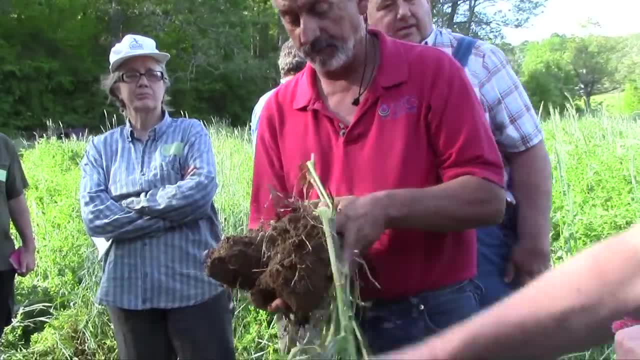 You guys see anything? Remember all those spheres we were talking about? Yeah, those kind of sheets, right? Ah, do you notice it doesn't have very much. Do you notice that? Oh, I notice it. You noticed it right away, didn't you? 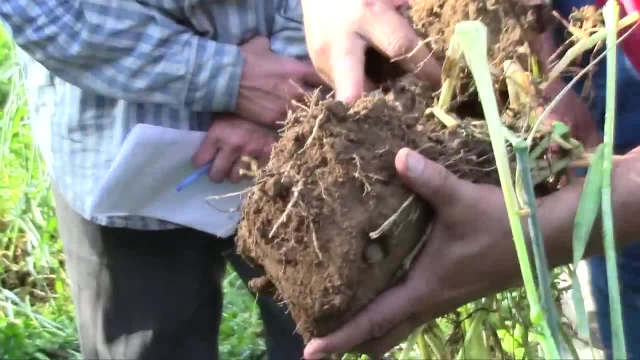 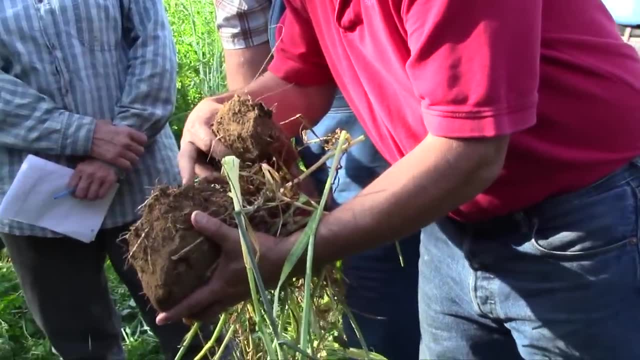 Look at it: It's starting to aggregate. look, It's starting, but it's not nearly like the other one. This is its first year of reparation. Look at this. Look at the nodules. See those nodules right there. 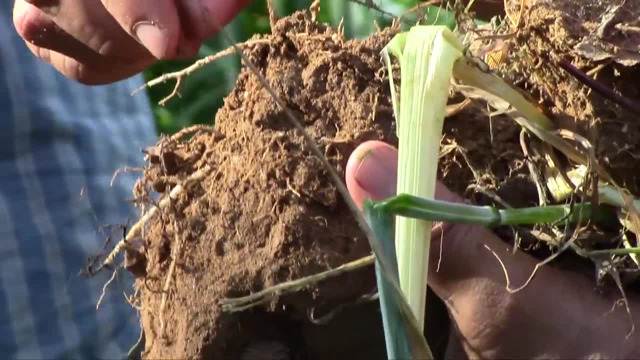 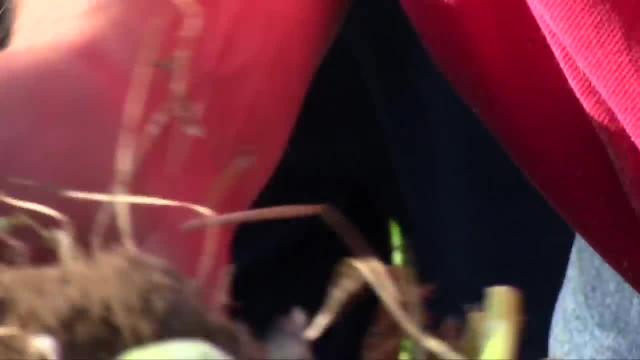 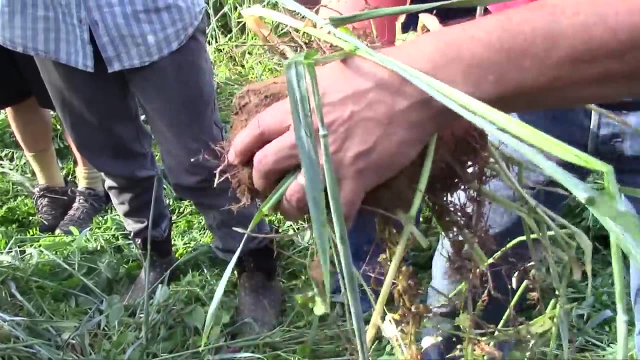 Squeeze that. and it should be pink inside. And it should be pink inside. See the aggregation starting to happen. That is by the covers. But notice the lower layers. There is no cottage cheese, It's homogenous. Look at that. 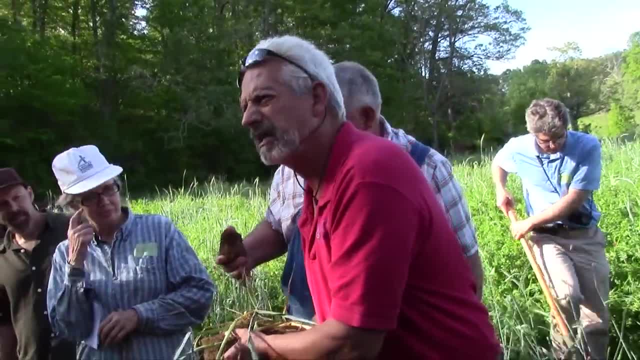 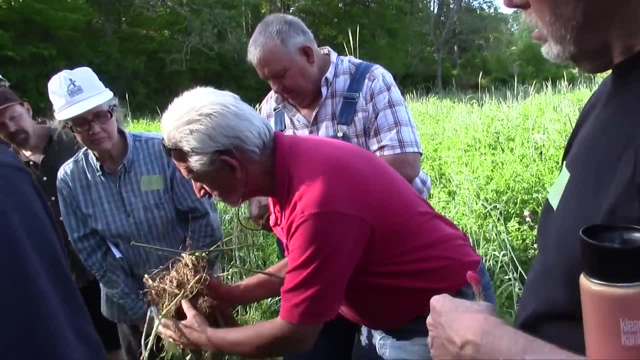 It has been brutalized, Hammered Big time. But look at the cover Now. look at my rhizis, my detritus starting to happen. I'm starting to get some of these spheres and we actually saw one earthworm. 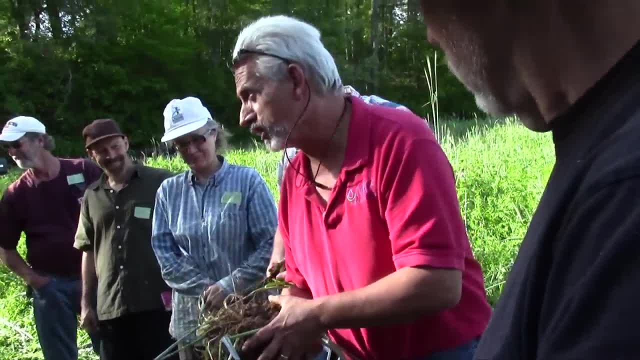 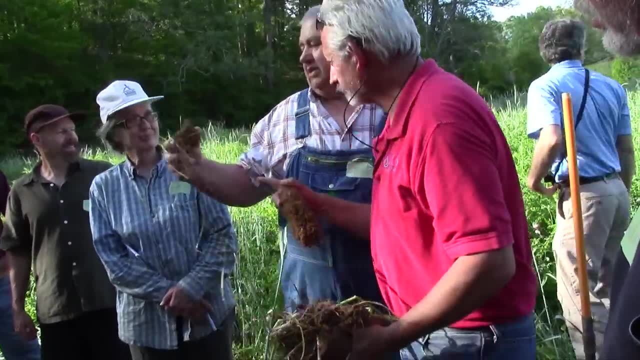 Which is exciting, You guys. that's a keystone organism. I know we got all the One earthworm. Oh yeah, We saw that, didn't we, Dave? Yeah, If you look at this, by not having the crack, you know, there's no way the water can infiltrate down through there. 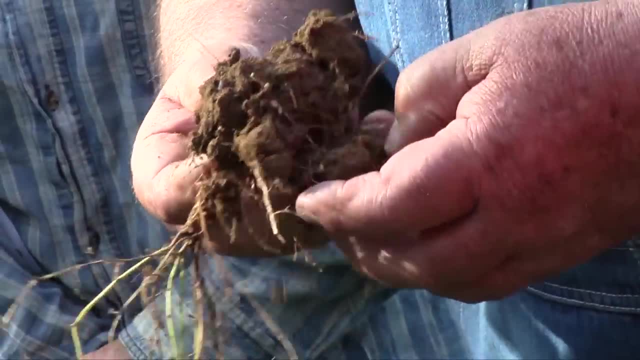 You know, But it's coming. You know he's starting to get. What we like to see is, you know, we like to see these. Look at this root: how much dirt it's holding. Yeah, that's that. 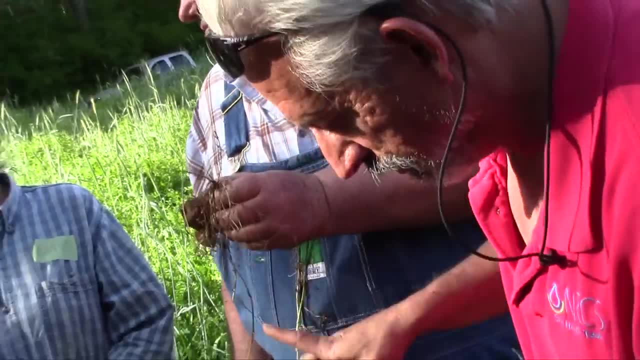 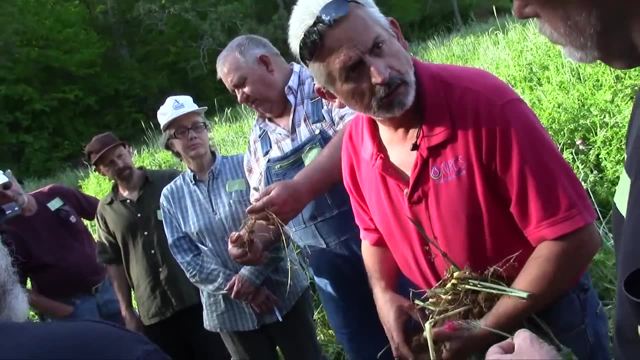 Look at that, See, It's breaking it down. It's breaking it down. That's biology, Bacteria, fungus, all those root exudates. They do that, They do the aggregation. This is a hairy vetch plant. 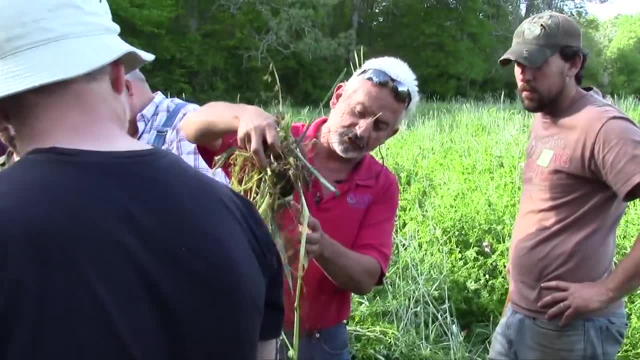 See that, You know. See how it's starting to dangle, See that dangling. This is the modulation we're working for. So what we want to do is, the next time we come out here, Pat about two or three years of these covers. 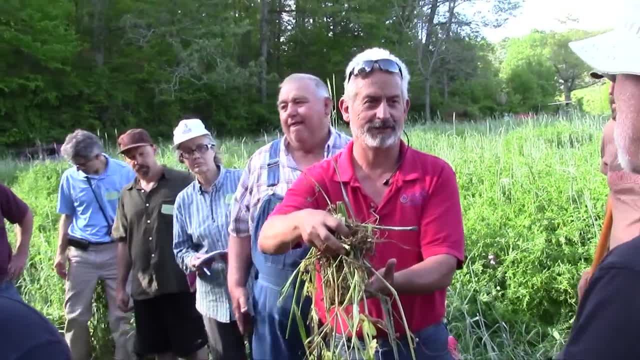 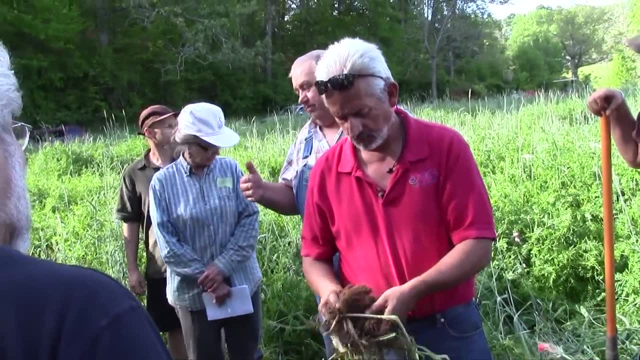 and doing the right farming, this soil is going to look very different. It will, It will, Oh, it will. I'm very confident. You know this is a great farm and I'm glad they're going to really try to build the soil. 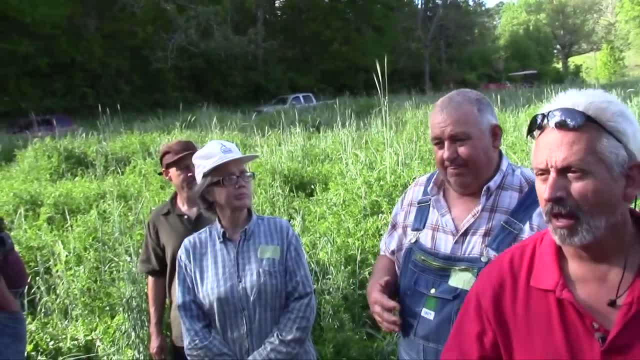 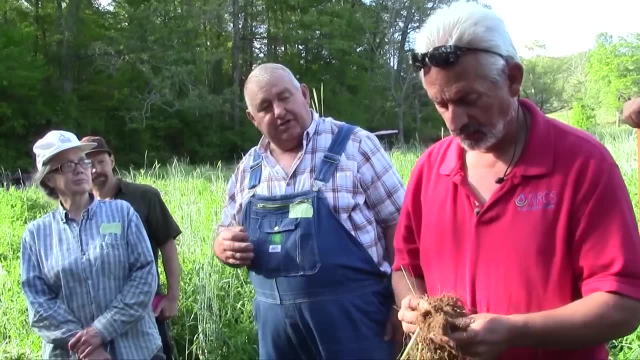 because I'm hoping they have a soil sample before they start it. Yeah, we do. Oh good, We did the test with you. Good, Okay, good, Yeah, we got that. After they roll this, we should pull another and send it down to Rick. 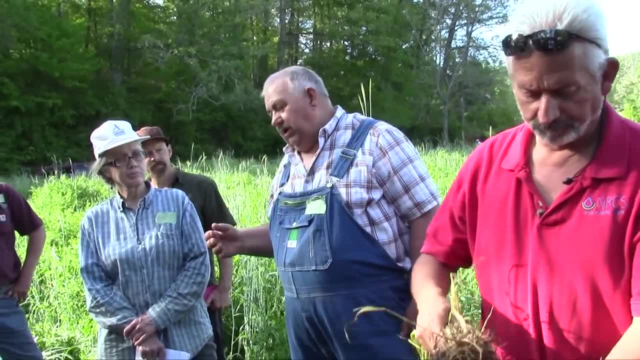 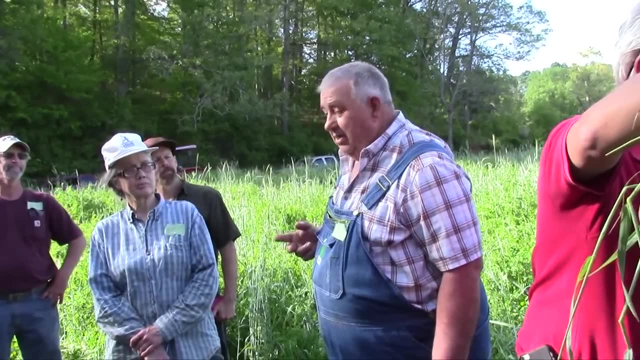 Yep, Yep, Right, Yep. And then after, by going back in here with the summer mix, which has actually given us two years of history in one year, then the diversity is really going to change by fall. How long would be two years of history in one year? 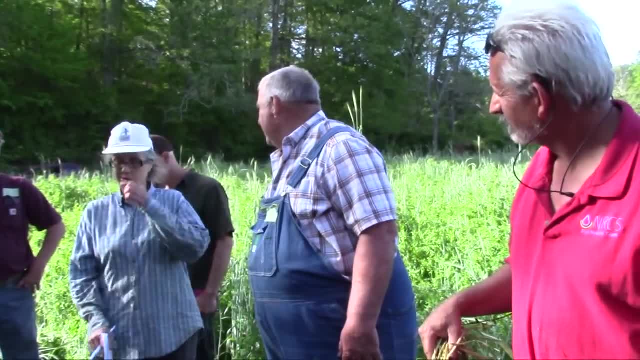 Usually it's one cover crop a year. One cover crop a year. Oh, We're skipping crop season and doing cover crops instead. We're doing cover crops. So think about what we're doing here. We are putting five or six rotations in one period of time. 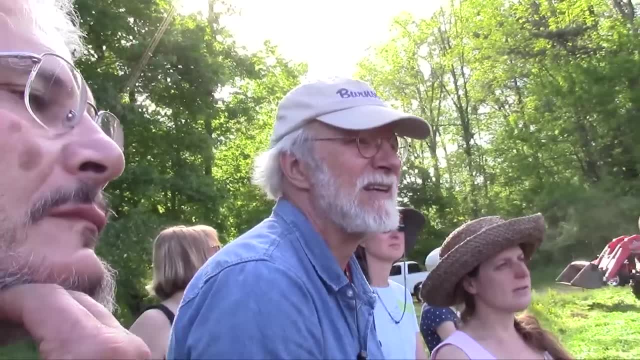 We're going to do that again now with the summer. That's going to be another five, seven, eight species, Yeah, And then we're going to come in for the last winter cover crop mix and then we're going to start going into the rotation. 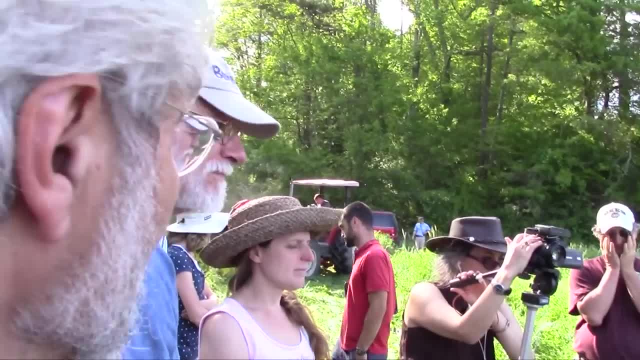 We won't do all of it either. I mean, some of this we'll be getting cover crop in next year. Yeah, We're not going to put all 30 acres in in one year. Oh great, You know, I mean. 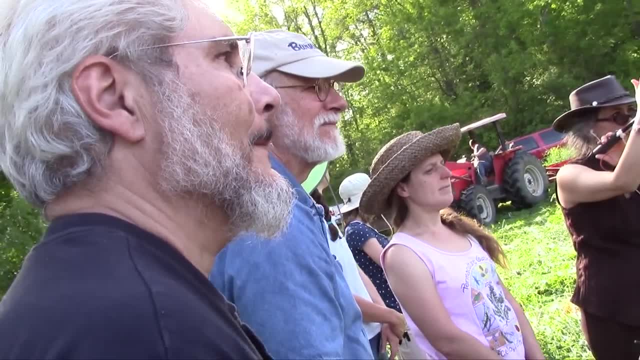 We'll always have a summer cover crop mix. We'll always have a summer cover crop mix. We'll always have a summer cover crop mix. Can you imagine if we had animals here? Oh, I can, Oh, my goodness, I can. I can definitely imagine having animals, So you, You didn't have to lose the money. You could put 300 of these sculpers in here for Oh, For like 65 days. Mm-hmm, Oh yeah, And eat all this out. 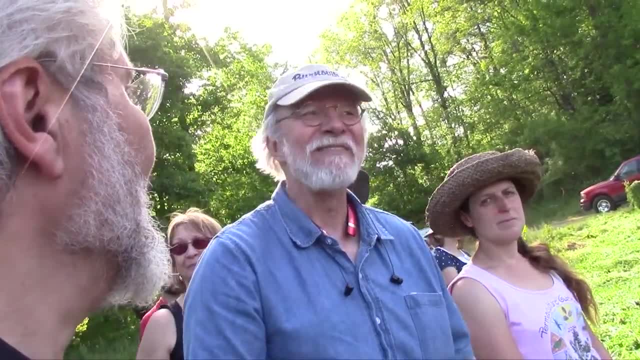 Oh, absolutely, Absolutely. How do you feel about that, Ben? The best thing you could do for the summer is to put it in the water. Oh, absolutely. How do you feel about that, Ben? The best thing you could do for the summer is to put it in the water. 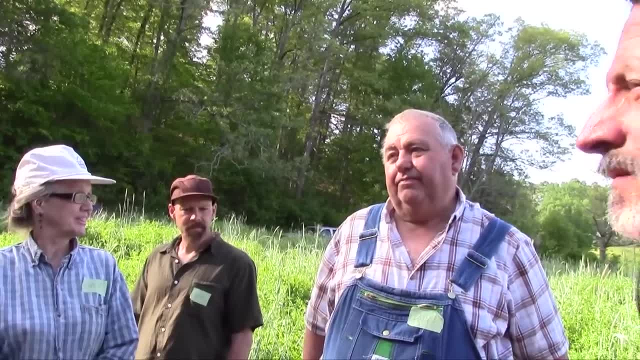 Oh, absolutely. So that's why we're doing this, And that's why we're doing this And we're going to do this to support the river. You can eat all this out. Oh, absolutely. How do you feel about that? 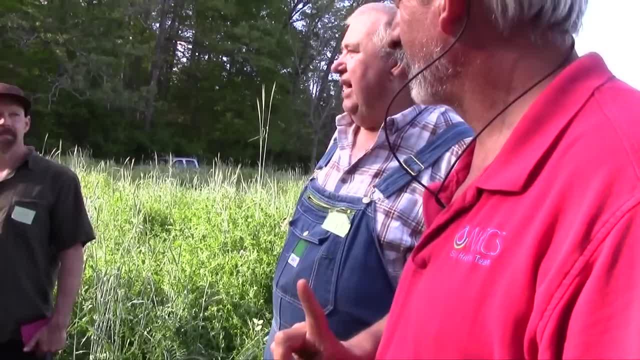 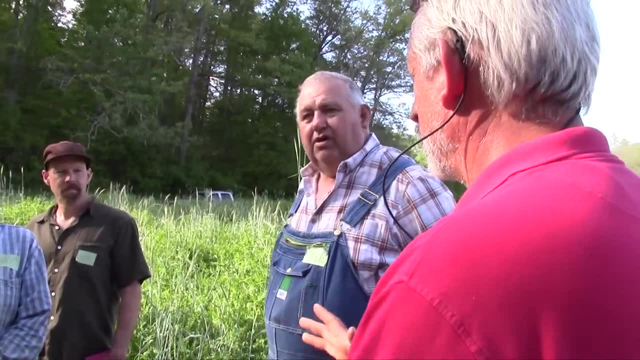 Well, they wouldn't eat it all out. right, You only take half of it. You could put 300 animals in this field On half of it. No, no, you're going to group them up. You're going to group them tight. 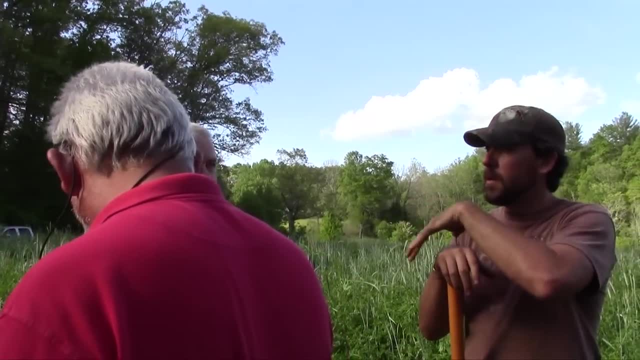 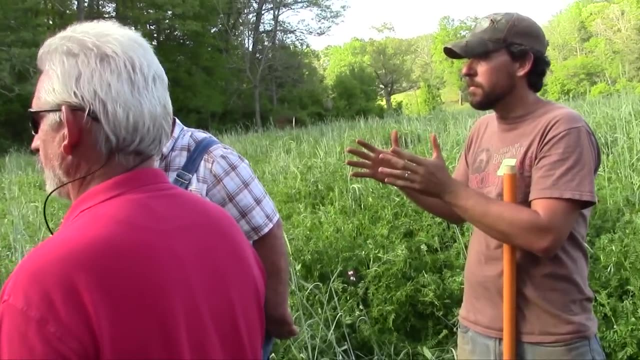 You're going to group them up. one acre blocks. You can regulate how much they graze versus how much they trample. It's all a relationship of animal units, space and time Got it. So you're going to make sure they only take half. 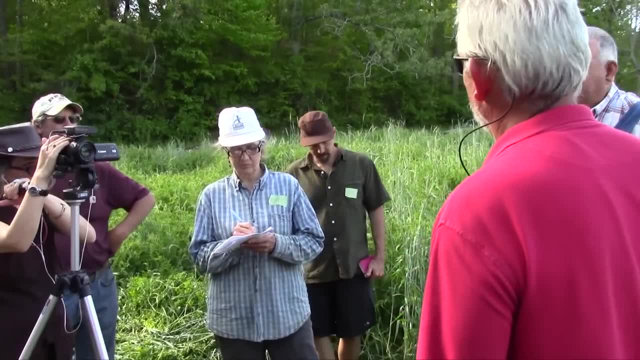 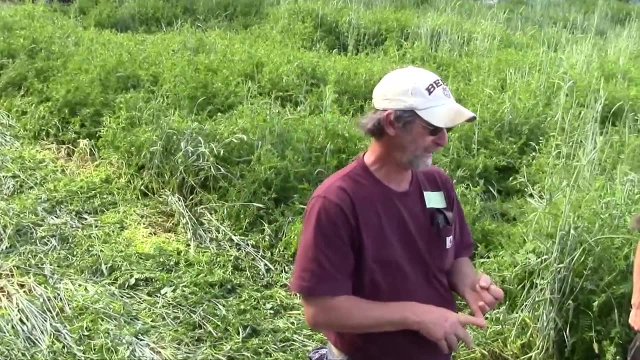 Grazers are going to want to graze this to the ground. No. So in your estimation, restoring this land, would you seed this for a summer crop now, or would you graze this now? I'd have grazed it. 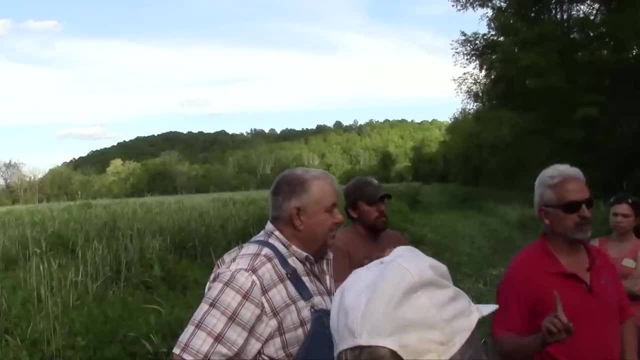 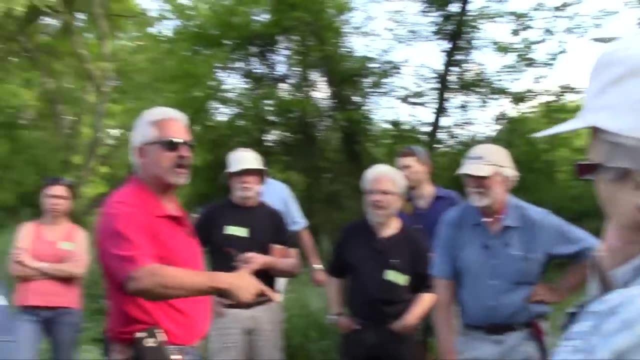 I would have grazed it because you would have made money, Plus you plant the cool season mix. you would have been beautiful Because, remember, a cow is like a giant soil vat. They got protozoa, they got all kinds of things. 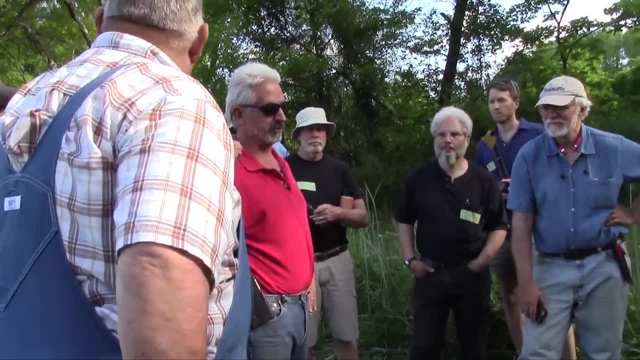 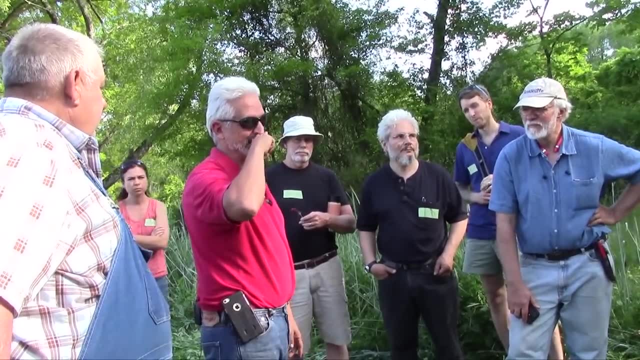 If you have manure, you cannot beat manure and urine. And then it helps the cool season, the warm season. So you would have made money and you wouldn't have lost. you would have paid for this mix easy, But as you graze it, you would then. 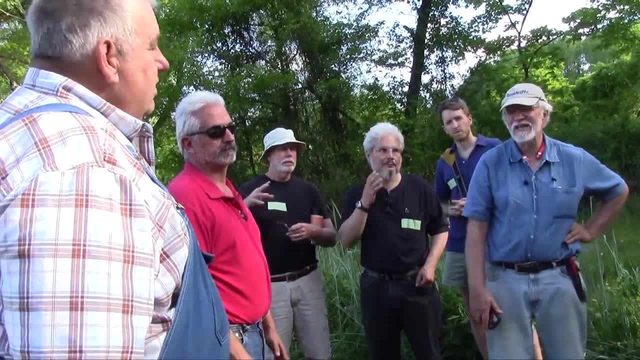 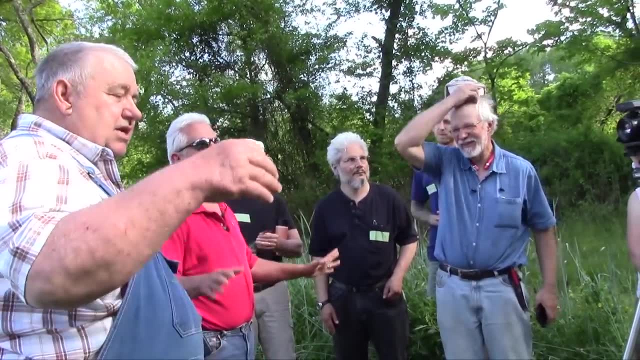 be coming behind and put the summer cover crop in. You got it. We're just not set up infrastructure wise for that Right. If there was a fence here and they could graze this in one or two acre grid blocks, then every time they moved they would. 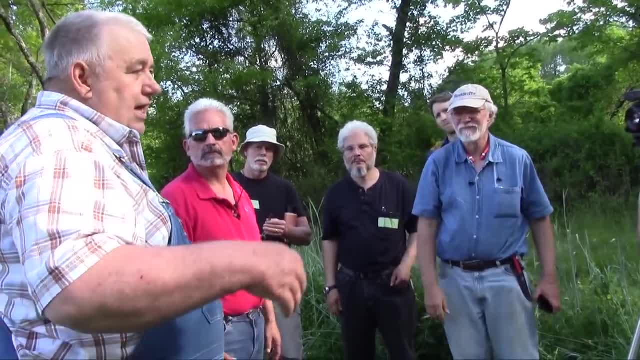 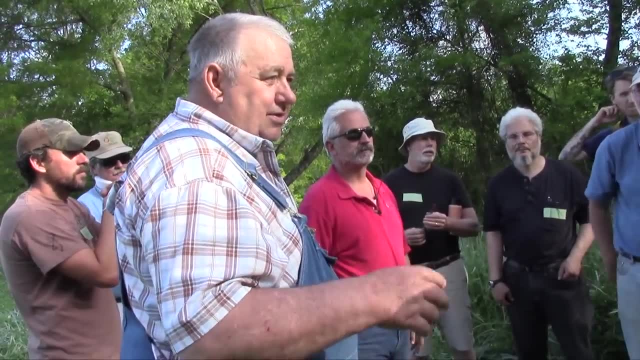 put their summer mix in. or maybe what they do is broadcast their summer mix, leave the cows there and then leave the cows there another four hours. They grind it in Four hours. They'll do it in a two acre block. So you got to remember. we're running now. 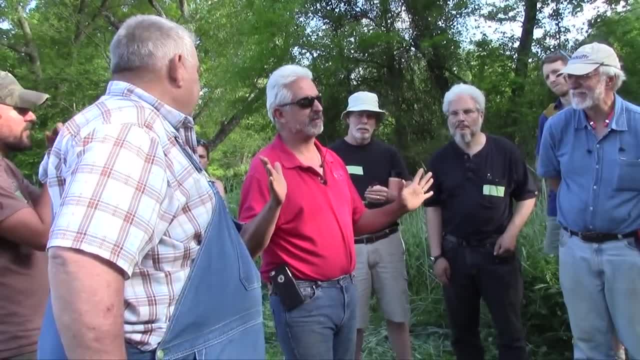 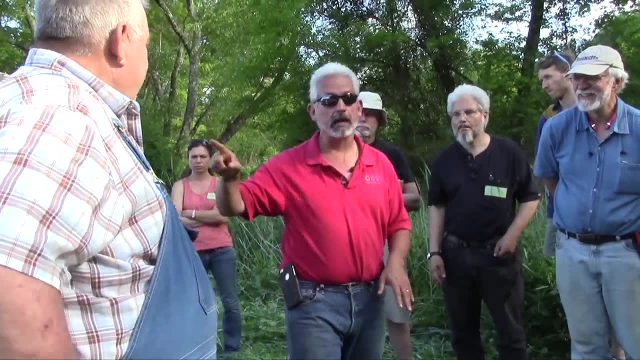 two hundred cows. Say a cow weighs a thousand acres, I mean a thousand pounds A thousand acres, A thousand pounds a cow, One cow. So you got two hundred cows. this will be mob grazed. You can run two hundred cows in an 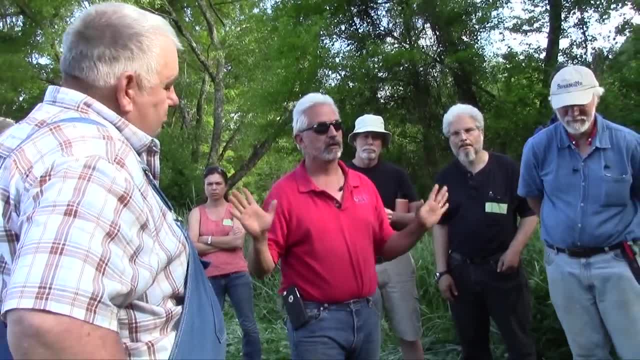 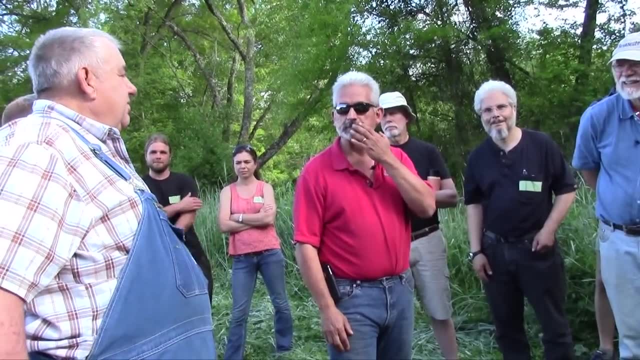 acre block and you'll be moving them daily. What about other animals? Sheep, pigs, goats, Chickens, Chickens, Chickens. They won't eat all this. They won't eat all this. You couldn't buy enough chickens to put out there. 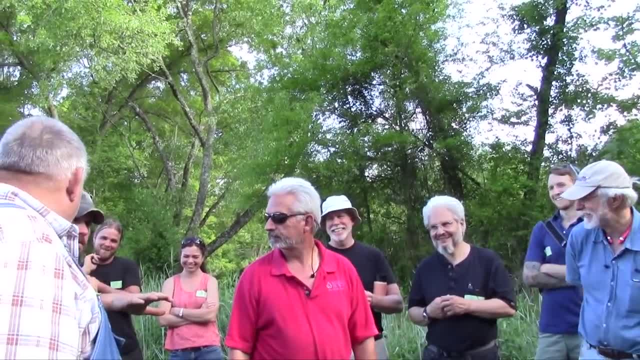 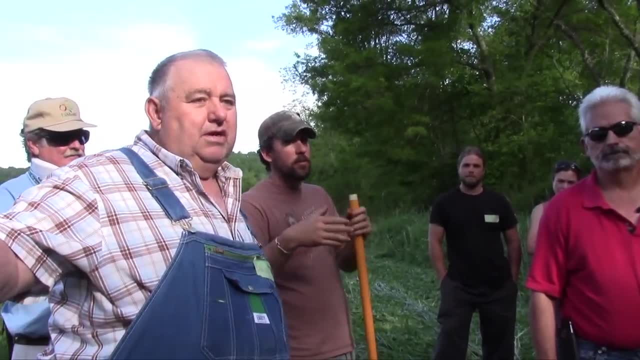 They'd be a little overwhelmed and you could lose them in here. You can do some management stuff there. You can do some management issues With animals. it's the same principle. Now, if you wanted to, you could use the two acre grids with the cows. 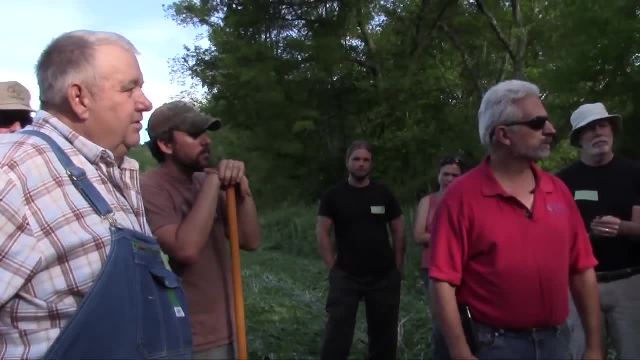 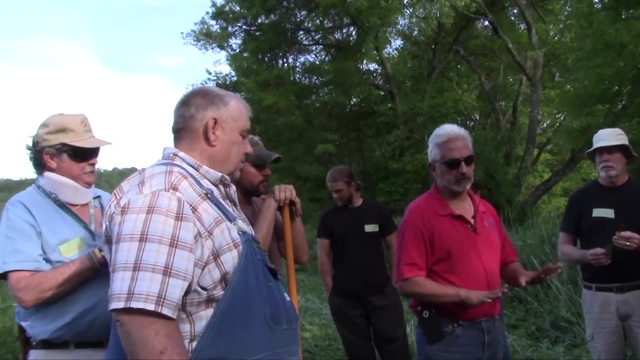 then follow it up with sheep, then make the seeding, But chickens go over it and then seeding Sheep will take it down a little further: Sheep, goats and those mixed. But imagine, imagine, if we had two hundred stalkers here weighing five hundred pounds. 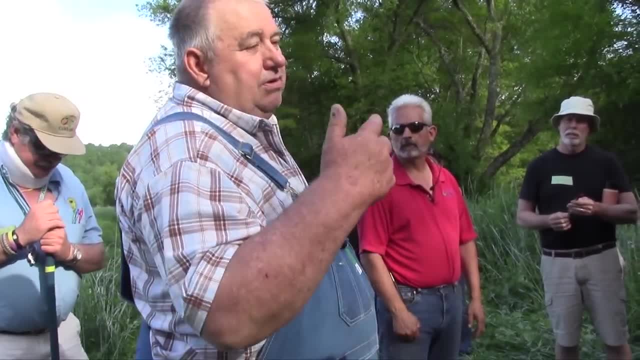 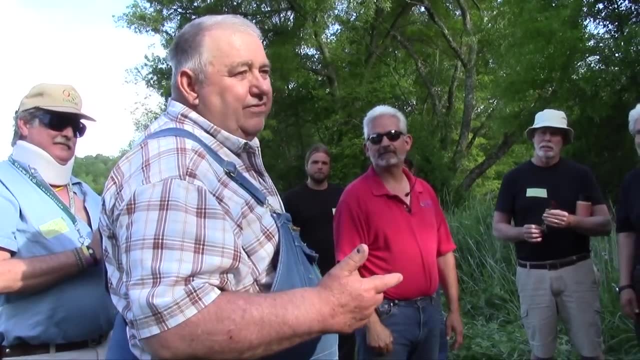 They were here for sixty days. They put on three pounds a day. Oh, Oh yeah, Do the math. Do the math: That's a hundred and eighty pounds per calf times two hundred, That's thirty-six thousand. And they're paying a buck a pound. 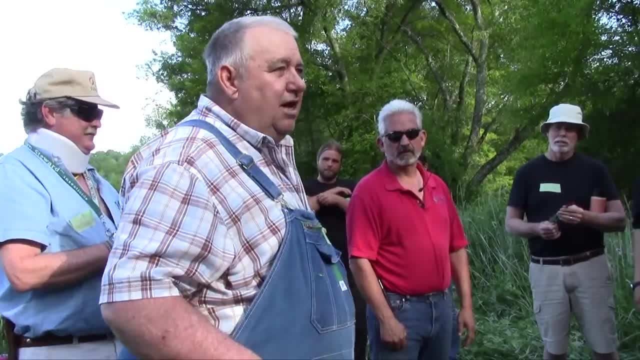 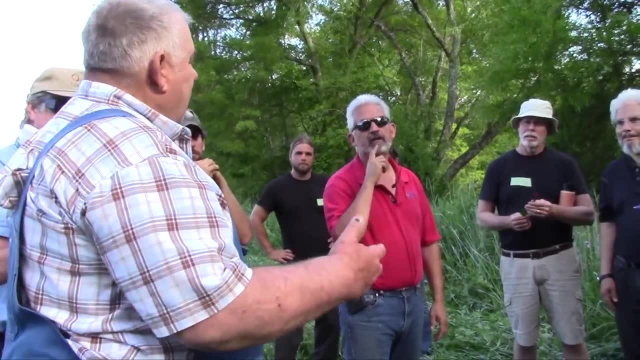 So you make thirty-six thousand dollars. You make thirty-six thousand dollars rather than rolling down here. Yeah, it's even more. now It's two or three dollars a pound. Right, You know, I'm just using easy math, Easy math. 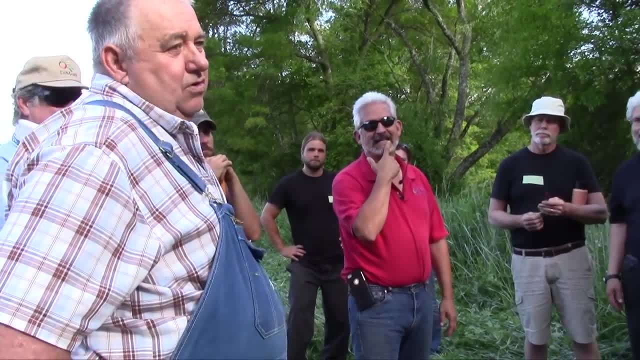 Well, for pasture-raised beef, Oh yeah, Well, pasture-raised beef would be a whole different. I'm just saying, you know, we got guys in Virginia that want us to do this and they'll pay us a buck a pound Yeah. 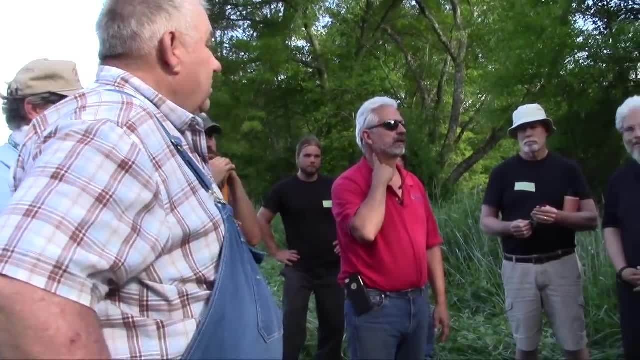 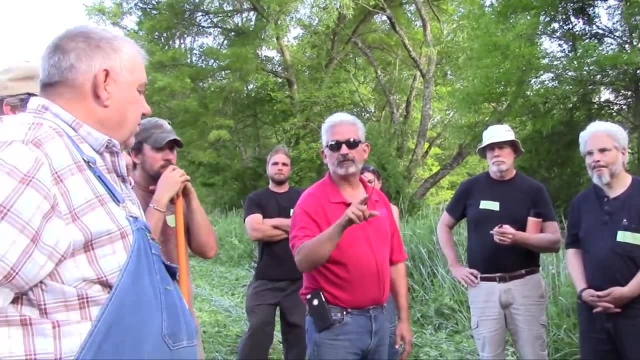 So whatever weight we put on them. But see now, but pigs are? I mean, they're the rototillers. You're talking about men. No, they will not root in here. A pig will not root in here. Why? 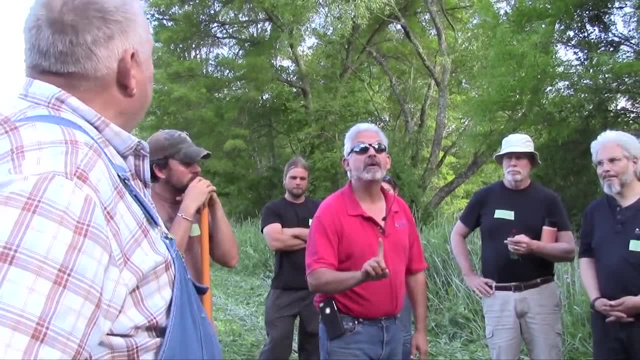 Because he's got the grass. Yeah, You're gonna move them. You're moving them Because you're not gonna leave them there for a long time, because they will tear it up. They're gonna go after legumes, basically, Yeah. 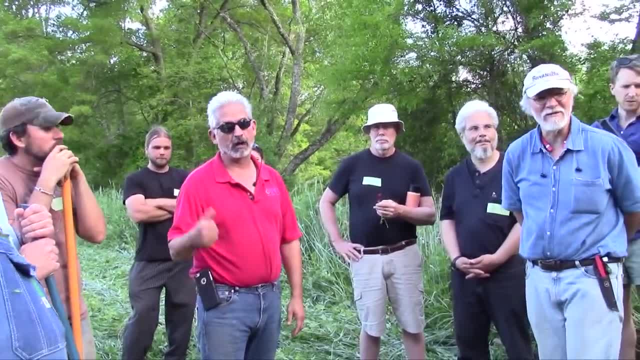 They're gonna feed really well here. You just move them before they get. Like Rocco said, you gotta manage. They're gonna keep going. after that salad bar They're gonna go for that lush stuff and then by the time they're ready to start digging. you are beautiful. 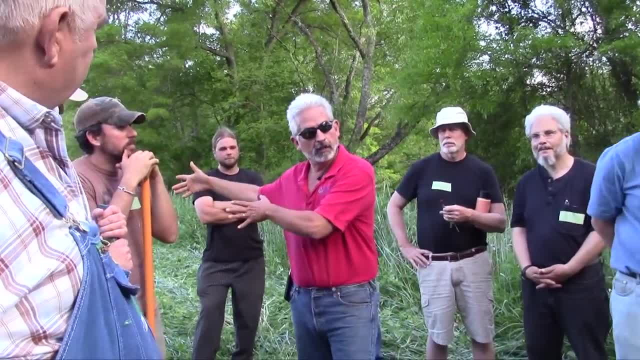 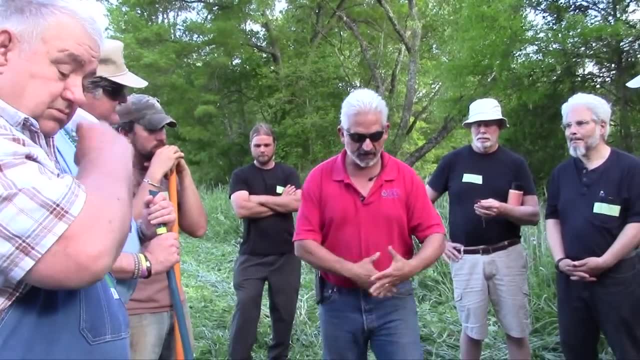 Yeah, because you gotta remember you're gonna move the pigs, just like you're gonna move them, because they will tear up soil. Oh yeah, I went to the NC State at the University. They had pigs there and they had these huge ruts. 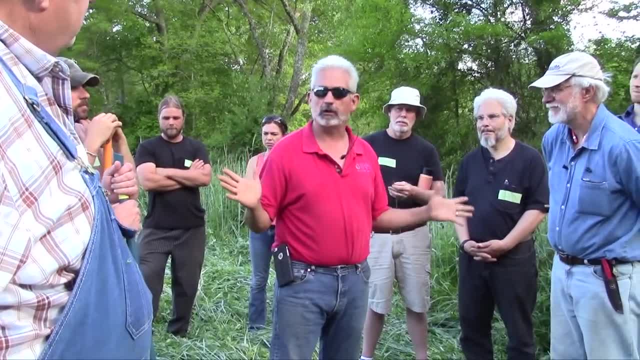 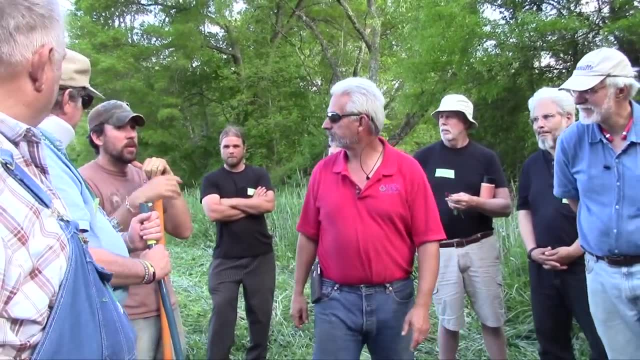 She kept them there for many days and they were gaining weight. Yeah, They're gonna destroy it and they get bored, But you're going through this. like Dave was saying, you're not gonna have an issue With this. veg and clover and peas- the only thing a pig's. 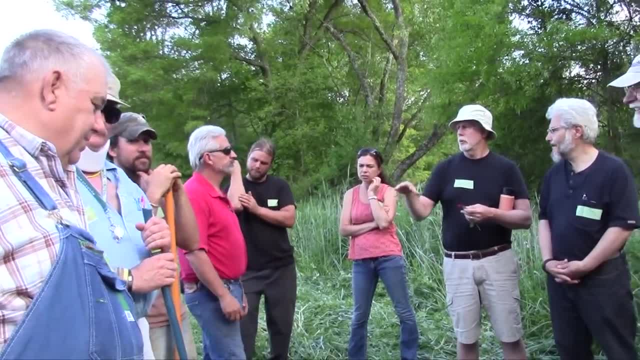 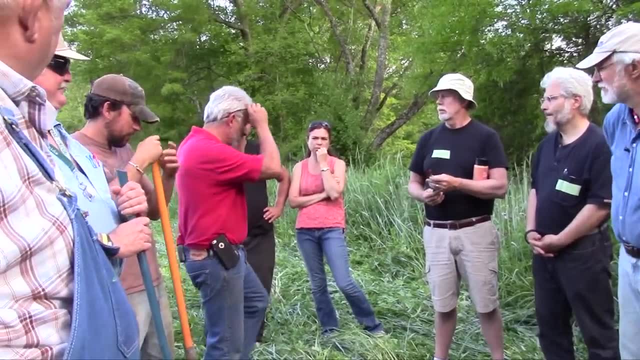 gonna do out here is gain weight. Okay, I'm eating poop, So they're not interested in the grass, They want the legumes. Within a couple of days, you'd be moving them. Yeah, got it. Here's what you do, The way you calculate. 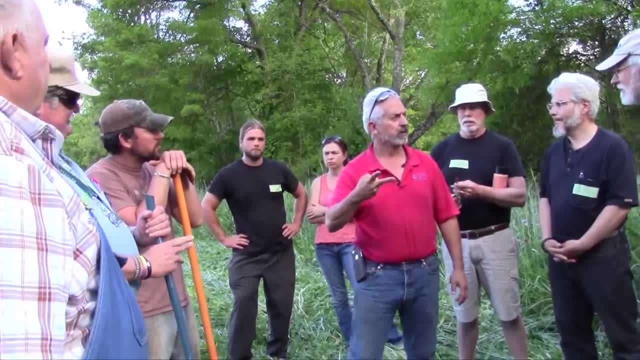 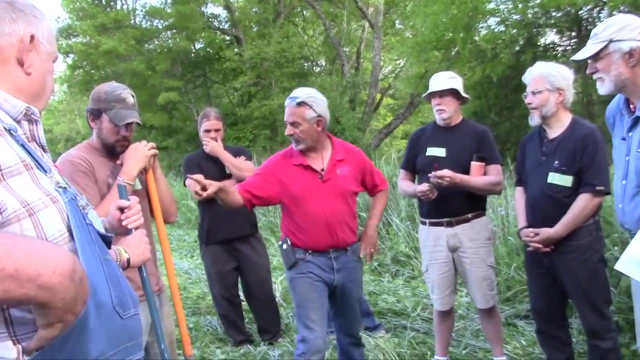 this, you'll get a ring and you'll clip it. So if you want to figure how much animal, how many grazing days you have, okay, 80% of this is water. Yes, So you're gonna subtract that You're gonna want dry matter. 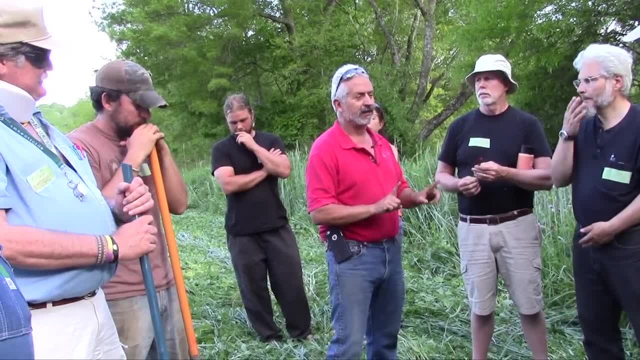 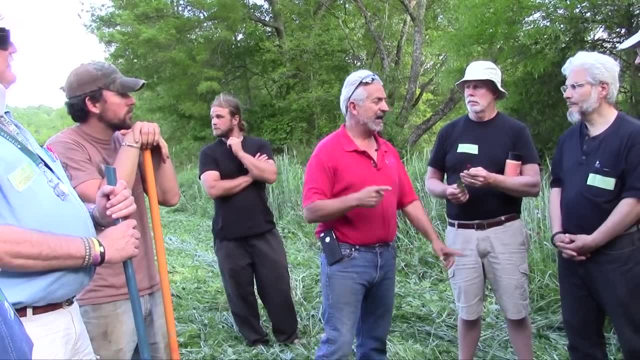 Say, a cow will eat 35 to 40 pounds of dry matter per day. So you throw your calculation, you do some basic arithmetic, then you can figure how many grazing days you have out here. And they say, okay, I'm only gonna take. 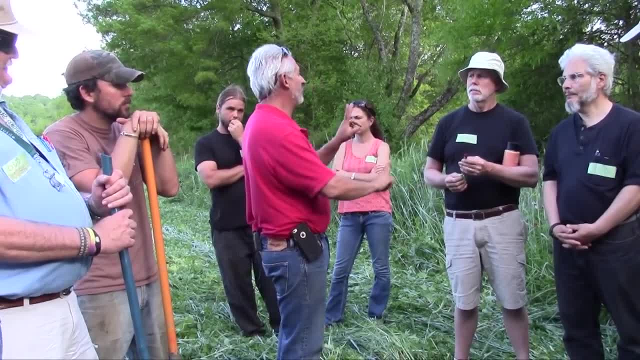 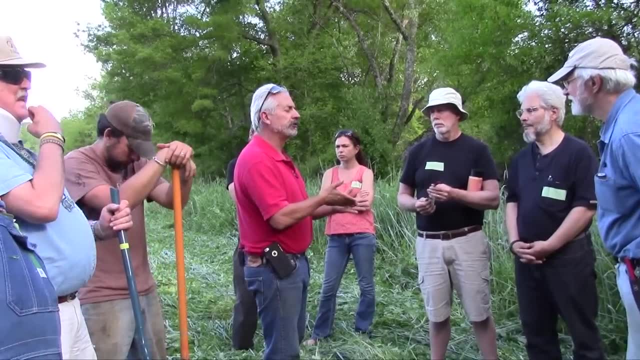 half. I'm like I told you half, So you're gonna cut that number in half and then you're gonna do your calculations. So here's where you go to do that. Just type: do grazing, calculate grazing days. Any university will have it. You'll see this little pamphlet. 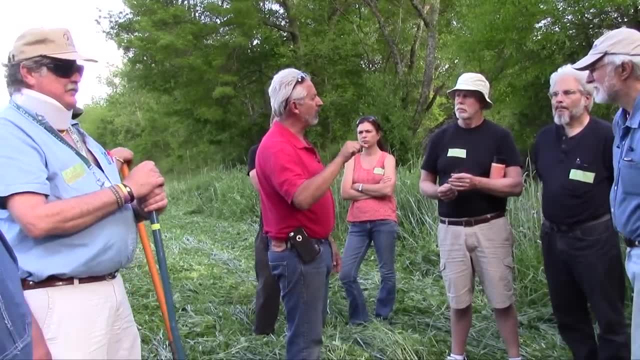 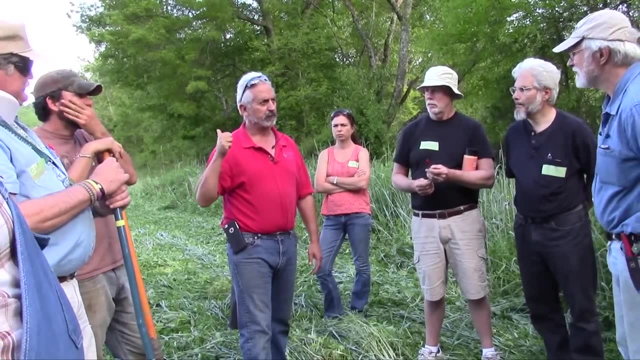 Just follow the basic math. But you can get a. what I would do here is bring one of our. we've got two grazing specialists at the tech center. They'll come here for free, feed them, bring them here and we can have. 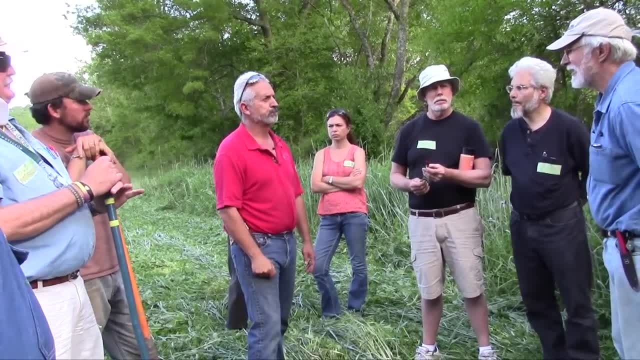 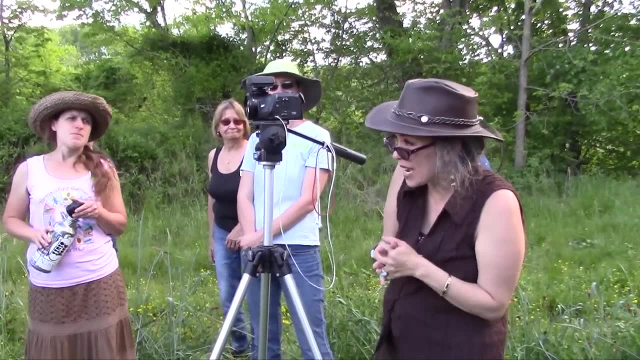 a whole day on grazing, how to calculate and how to do that. Let's do it next year. I want to tell people real quick that we have a big three-day, eight-hour-a-day workshop with Johan Zaitun, who is an ultra-high density grazing expert- Beautiful. 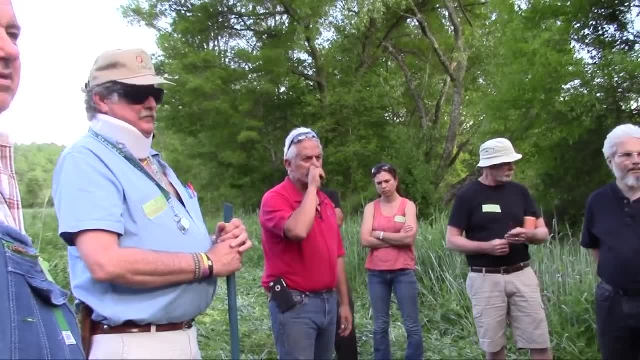 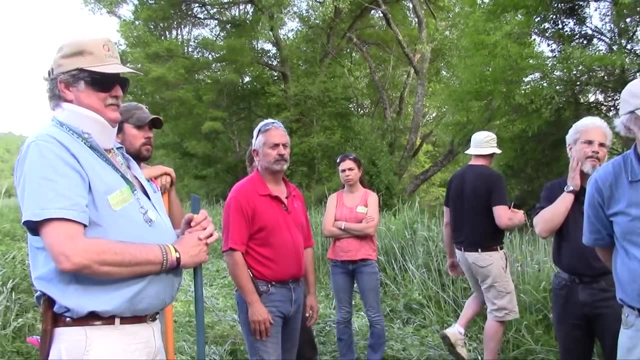 Yeah, bring him here. Twenty-four hours of footage online. Does he go through the measuring and cutting and clipping? He goes through every detail you can imagine. Oh, beautiful, It's already online, Ray, with your cover crop mix that you recommended for our Florida LivingWed farm. 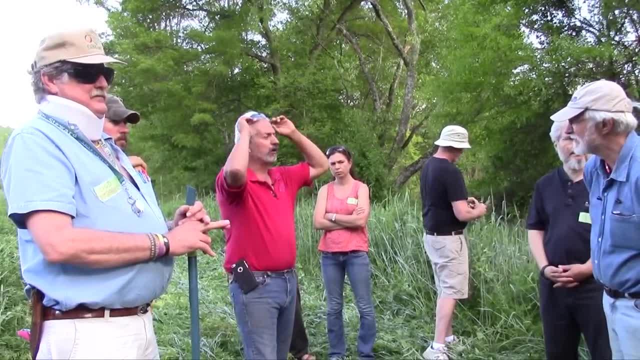 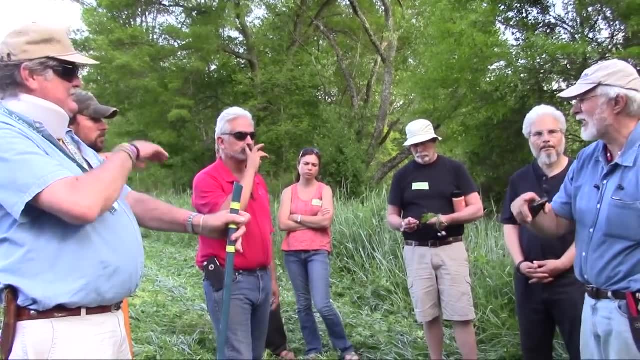 we've got a full video called Regenerative Ranching and it shows everything they're talking about. Oh, great, Excellent, Excellent. It's already online. We're also bringing Jimmy Elizondo out this year to talk about that stuff at the other farm, but we could also 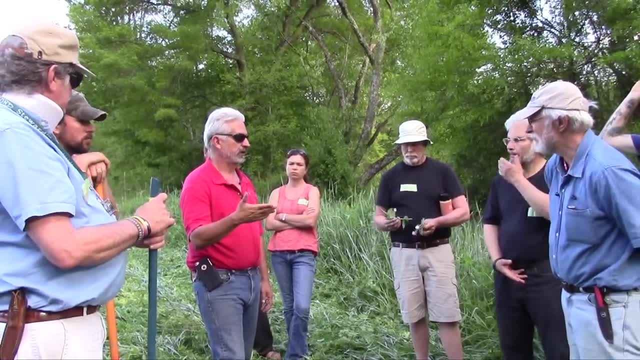 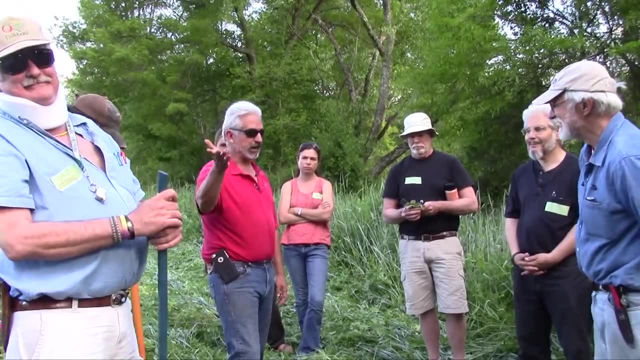 talk about this one, And then we're gonna try and bring Gabe here next year. We can get him here. He's one of the most sought-off speakers after Dave Grant. He's like: there's Dave, there's Gabe, and then well. 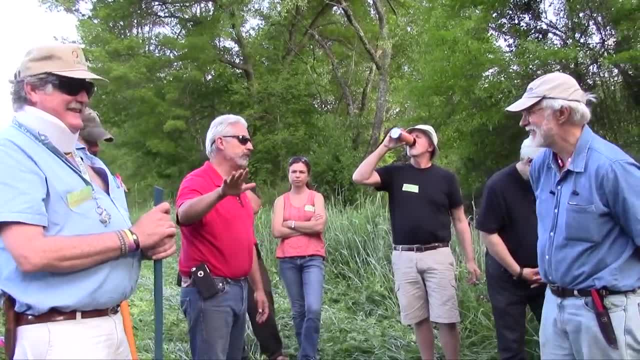 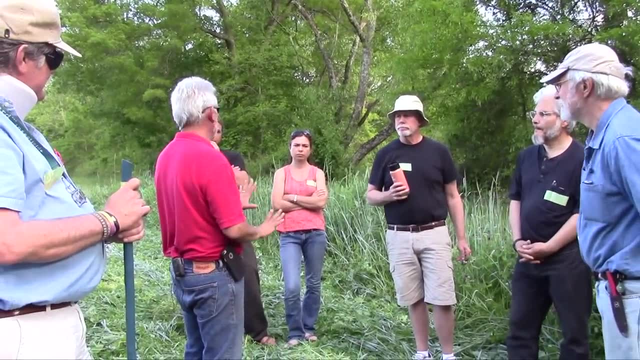 there's the rest of us. What can we say? So, but we need to bring him out here, because once you get to hear him, then you'll bring in the grazing, the cropping and all the enterprises that you need to learn about. 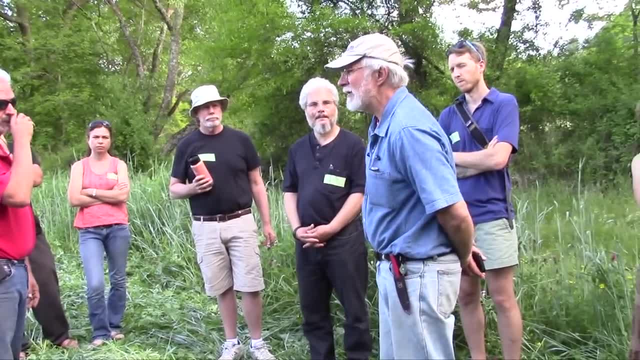 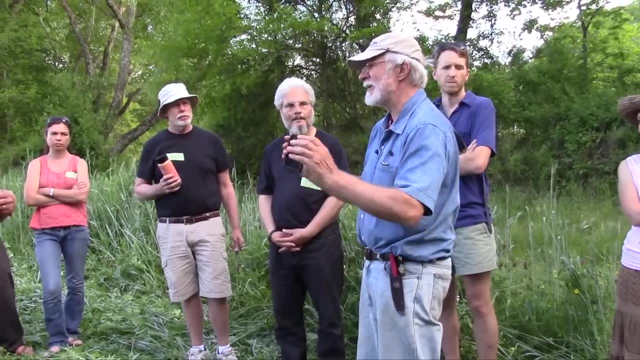 So Pat's gonna try and bring him in- I mean long-term- and we go back and forth because right now there's no way to do animals here. Oh, we can't do it. Maybe we'll just do chickens. It's like no, we will. I don't know when. 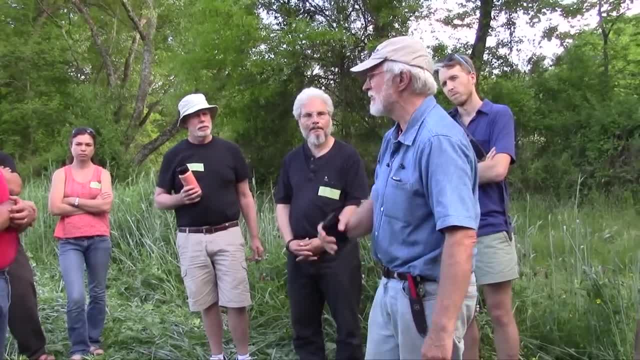 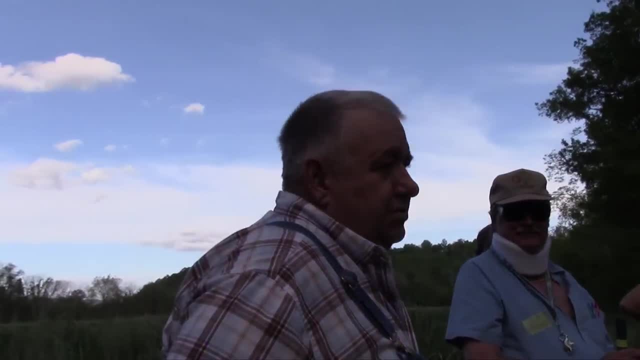 but we will eventually get to where we'll have animals here and we'll be incorporating them, Because that's the future of farming. That's what we have to do. If you're estimating the biomass out here now, I'd guess there's 28,000 pounds per acre. 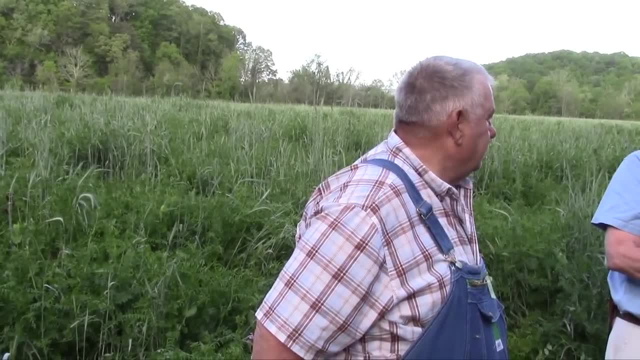 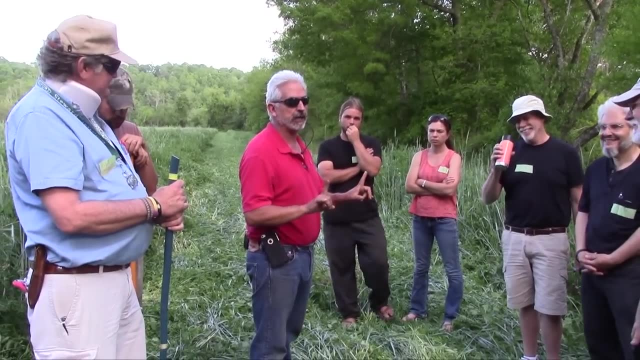 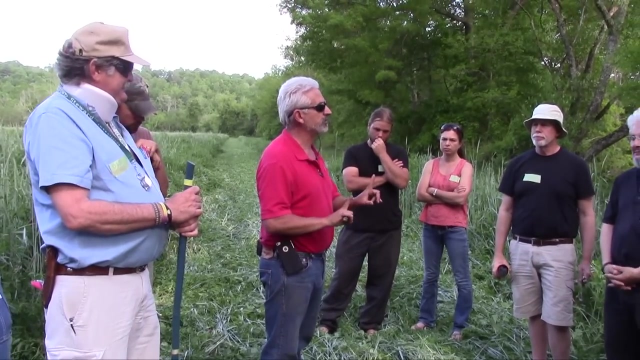 dry biomass, That's 14 ton of hay, Wow. So the thing about it is: we want our farms to run on new sunlight, not ancient sunlight. Ancient sunlight is diesel. So all the inputs that we've talked about, that's what's making us go broke. 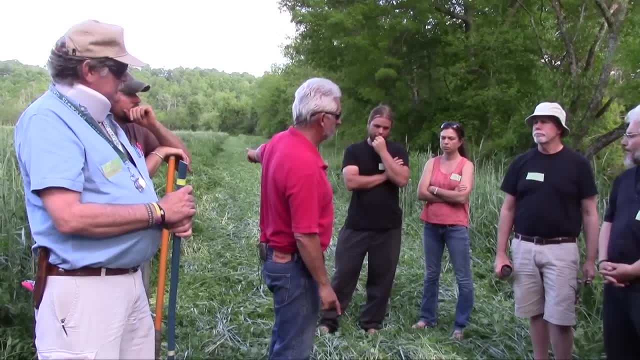 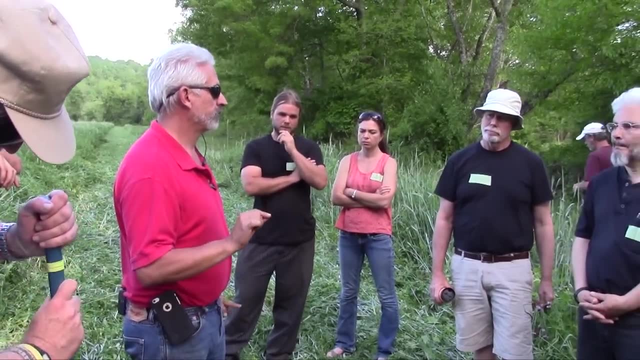 We want to run on new sunlight, So I want you to walk away with that. Another book you guys need to get is a book called Agroecology by Dr David Gleesman. It talks about all those principles and learn how You need to. 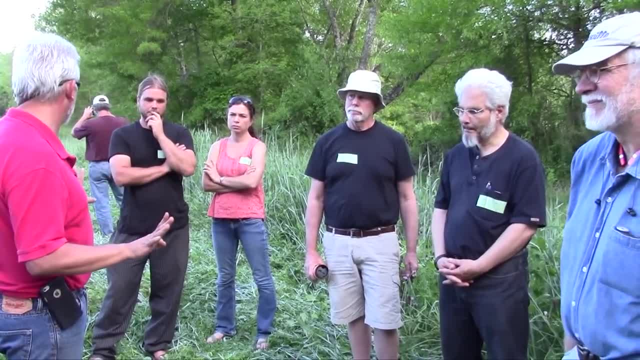 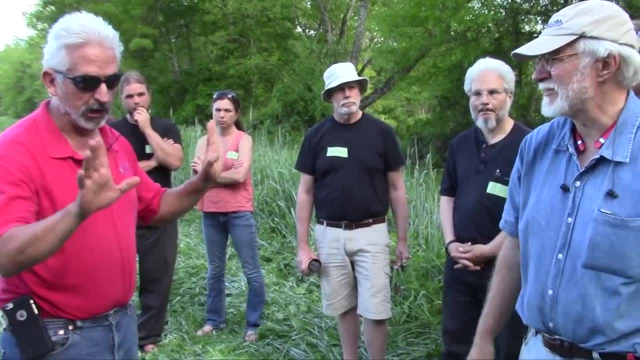 understand what's going on in these systems so you can understand the flow of energy. Okay, Dr David Gleesman Great book on agroecology, And you are gonna get your whole list on the website. Yeah, I'll give him the list of the books. 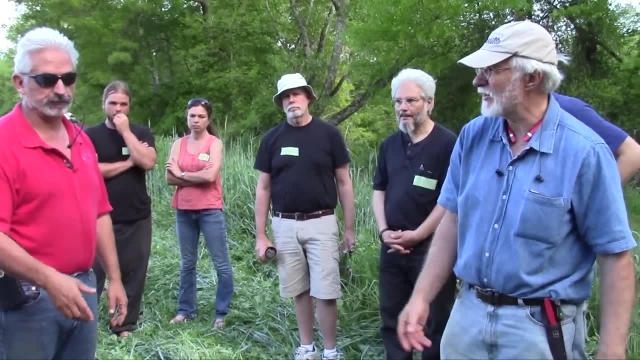 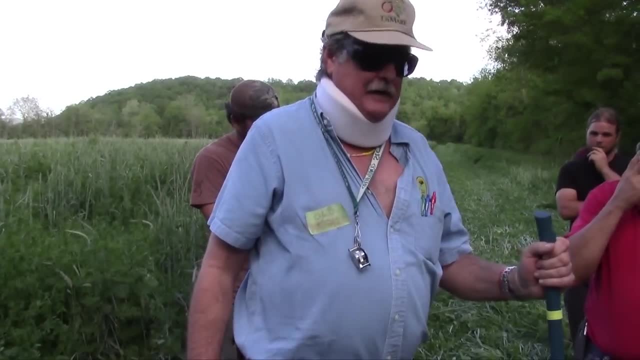 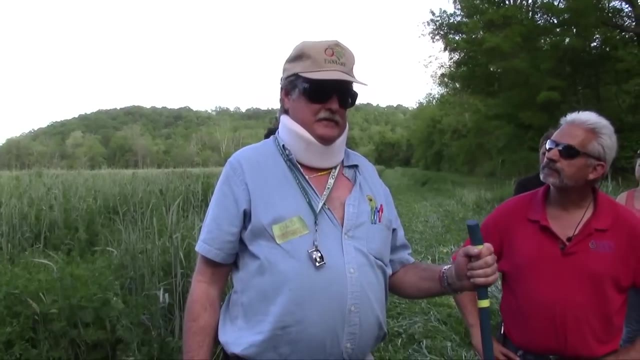 and then you'll have all those reading: Okay, All right. so Would you like to hear anything from a retired conventional farmer? Yeah, I am Marshall Hagen the old guy. I used to grow 4,000 acres of fruits and veg. in four states, Had 3,500 plus employees. Annual gross 450 million dollars a year. Wow, And it broke in 2001.. Yep, From the input, The last seven words of a dying business. that's the way we've. 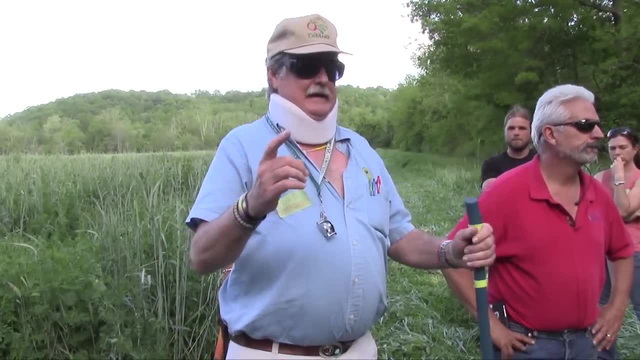 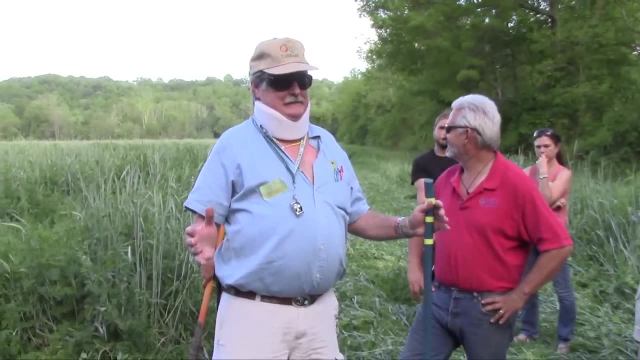 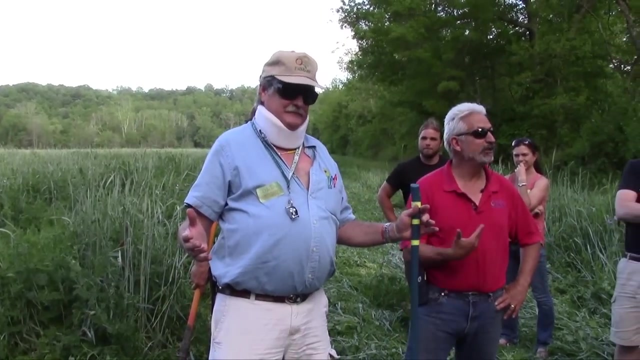 always done it, And I'm here to tell you folks. This is a new wave. This is so exciting to me. I only wish I was 20 or 30 years younger. Me too. Hey, me too. Thanks for sharing. 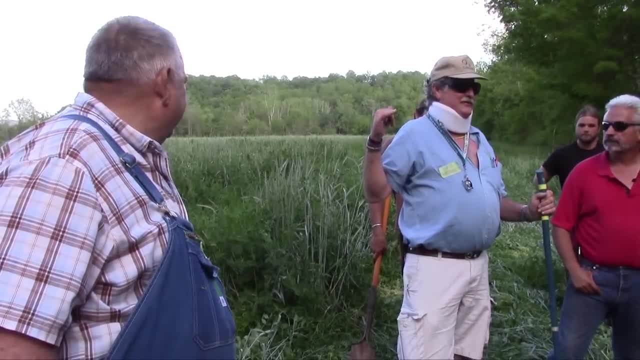 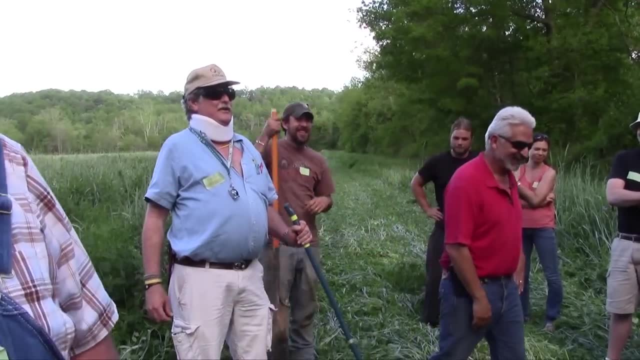 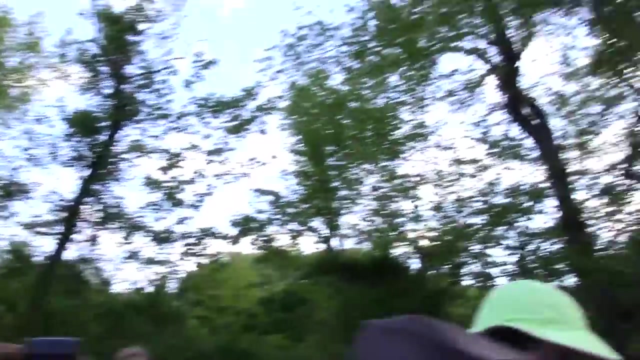 That's awesome, Thank you. I'm going to tell you, man, This is good stuff That goes on YouTube. Thank you for sharing that. That's really important. How about let's go eat guys? Let's go to Mugwort. 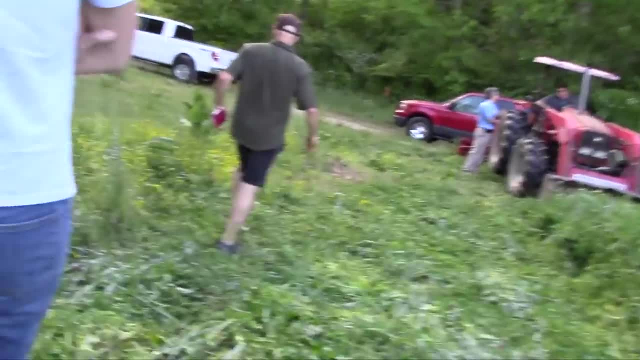 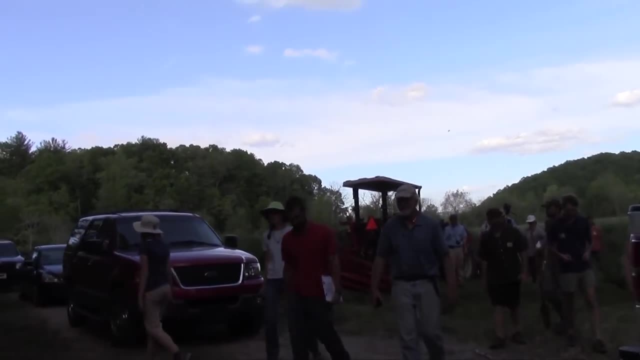 Mark will do the experiment, And then That's a beautiful little flower. Ask that question online, Any questions you have about it, let's just have it. It's the perfect thing to talk about. right? That's what we want to do on this kind of video. 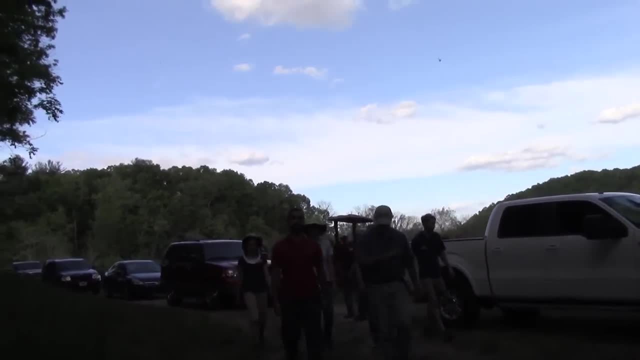 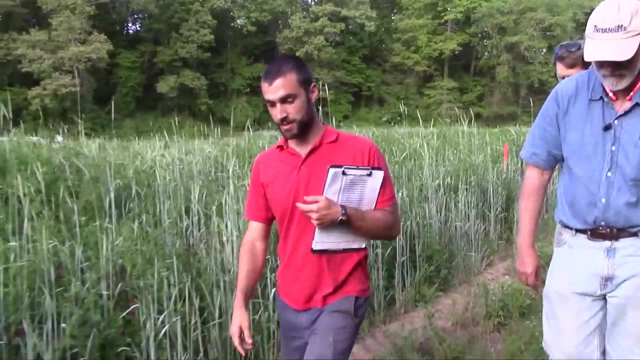 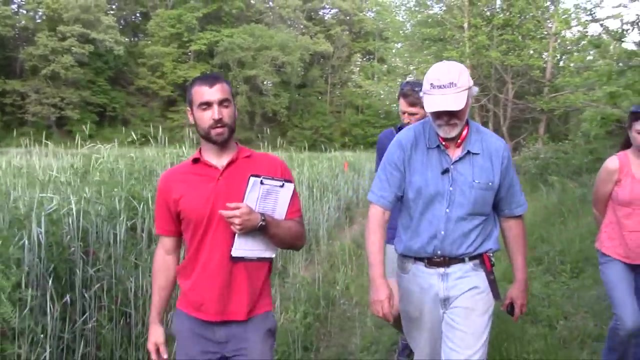 Totally show the process While we were looking at, or they were talking about, nodulation and inoculation in there is that if you have inoculated in recent years, you can be safe, And that there's like a lot of research that suggests that. 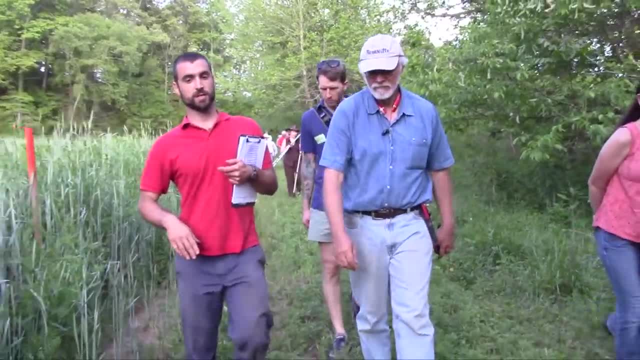 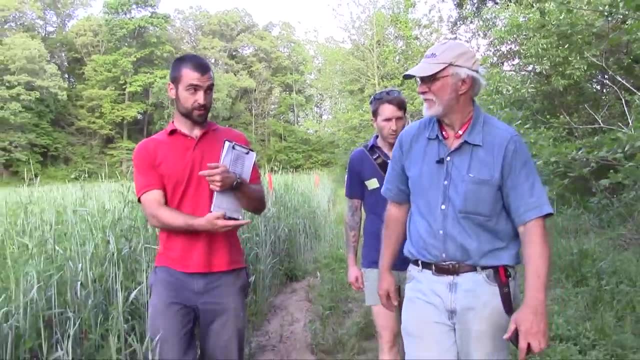 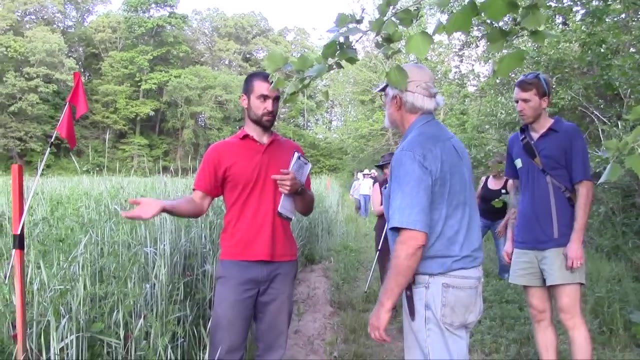 native rhizobia actually take over nodulation and fixation and stuff. later, Once the diversity is getting built up. Yeah, So years down the road you might see nitrogen fixation dominated by native species instead of the ones you inoculate with, Which is another. 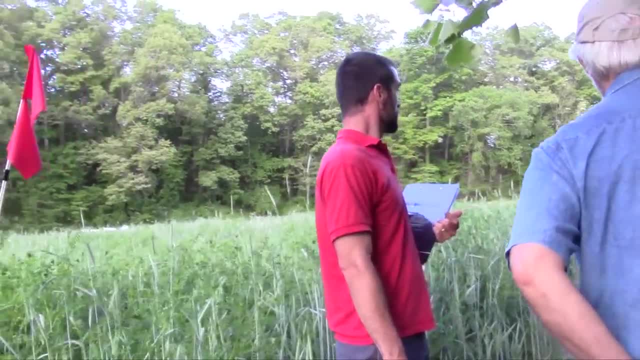 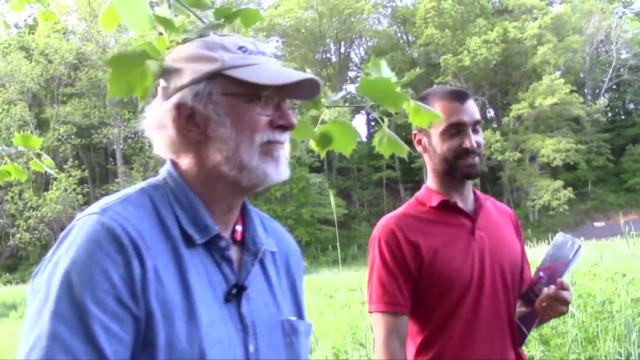 reason to promote diversity. That'd be a fun discussion to have. I don't know if we have time right now, Just throwing it out there for something to keep in mind for the future. That's good. Put that on the pasture. Yeah, put it on your pasture. 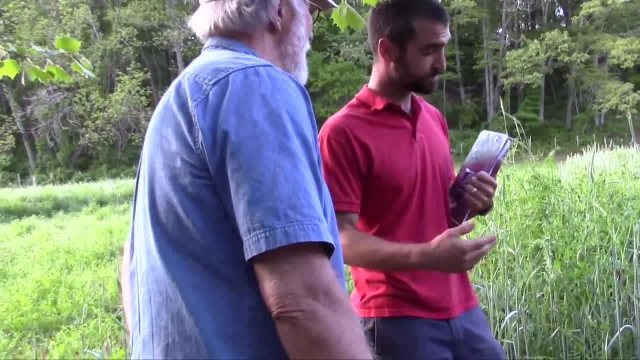 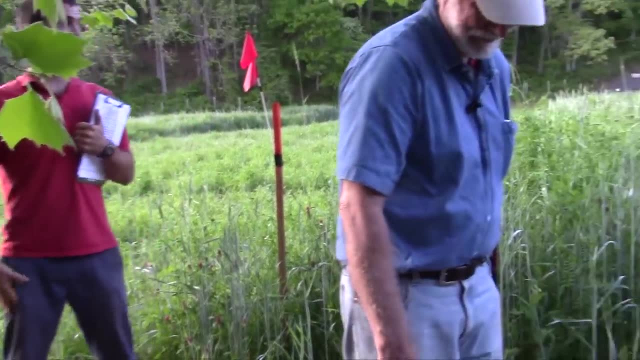 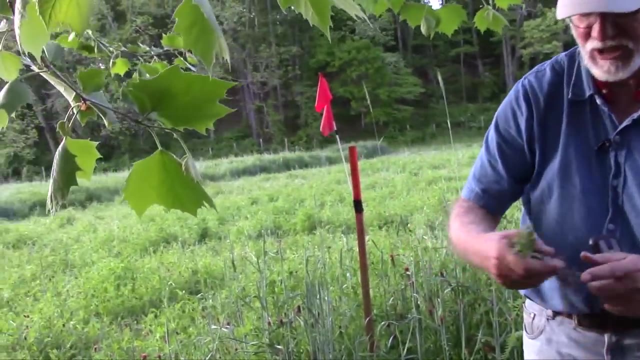 So maybe I'll describe the one gourd problem and then you take over and do the rest of it, okay, Okay, so the reason why we came out here is we're doing a major experiment. Mark Dempsey, here is going to be our. 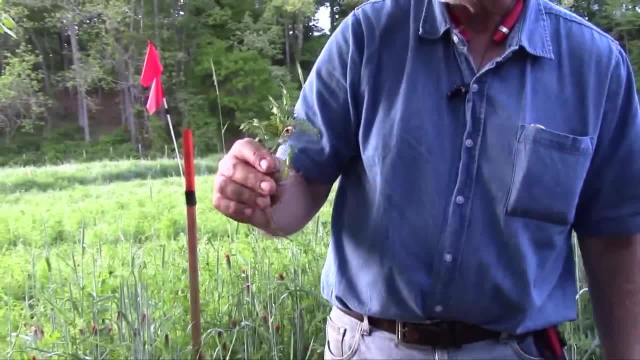 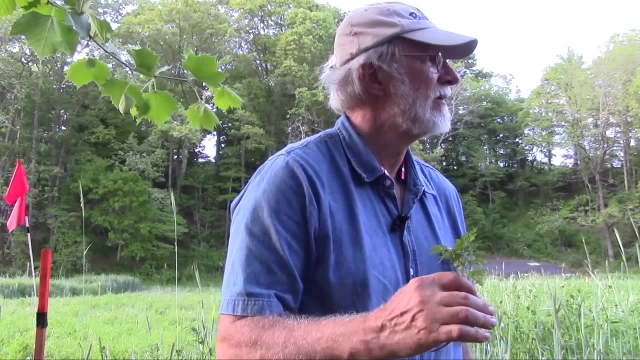 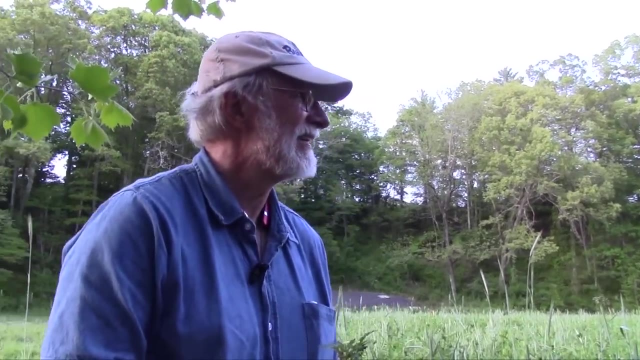 scientist to actually keep all the records and stuff And he was integral in designing it. We've got a question for David Brandt. Is he here, Gone back to Ohio? Any time you get around equipment he's gone. He's good at it too. 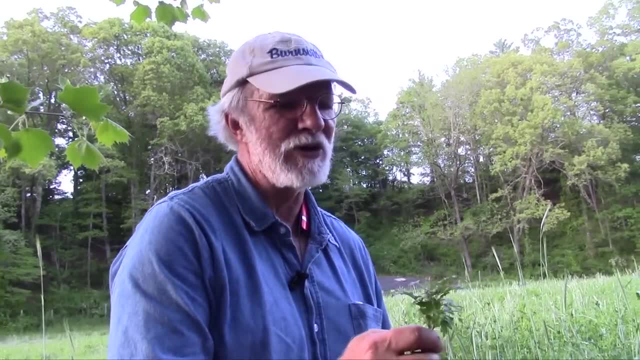 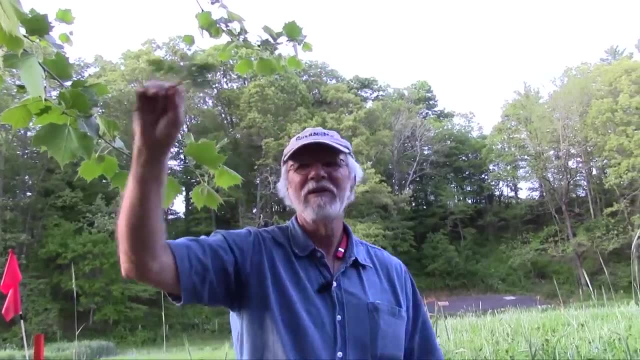 Can you give him a call and ask him, Because I'd like to ask him that question if he's willing to come? Okay, so the reason why we're doing this is: anybody know this plant? This is mugwort. Mugwort is one of the harder perennial. 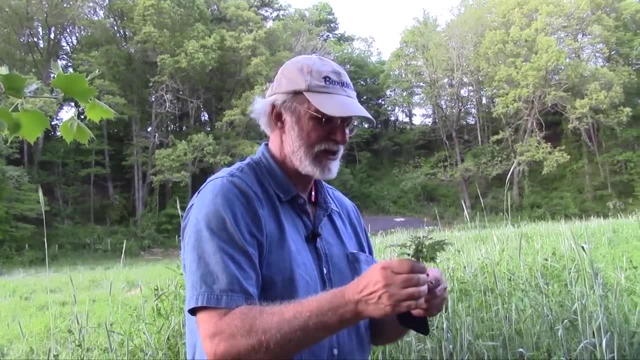 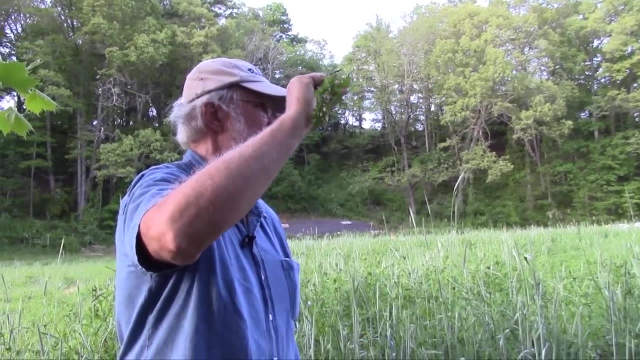 weeds to get rid of. It might be the hardest. A piece of root that big if you don't take care of it could have a whole field infected in not many years at all. You know, every little piece you break off reproduces. 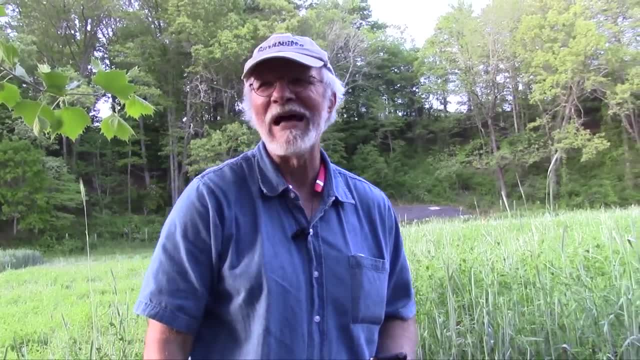 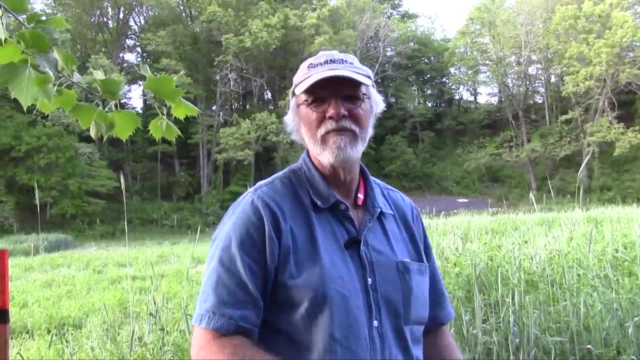 You cannot dig it out. You can't really till it out unless you want to kill your soil. It's incredibly invasive, incredibly persistent. It was higher than a tractor last year And it's all on the road here. We made a huge mistake by not 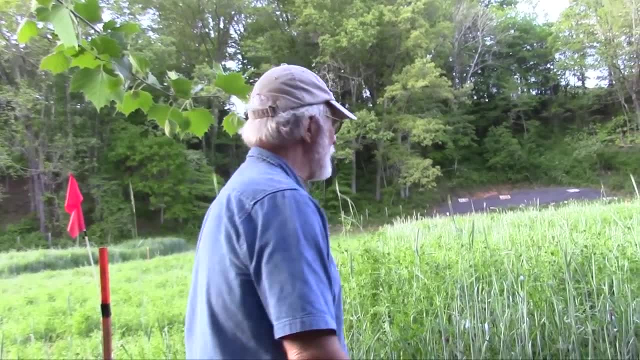 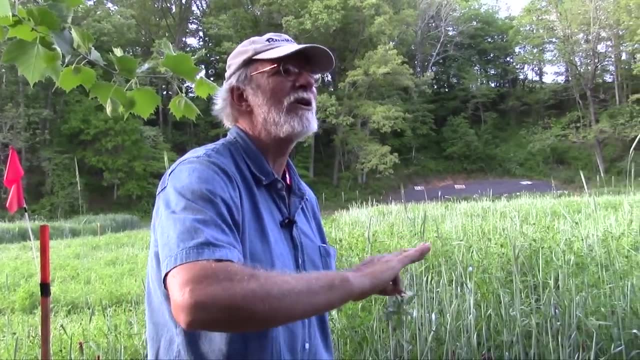 putting the cover crop on the road too. I'm going to let Mark describe the different trials. we're going to try to see organic ways to control it. We're actually going to use some herbicides so we can compare. That's the only time we'll probably ever use herbicides. 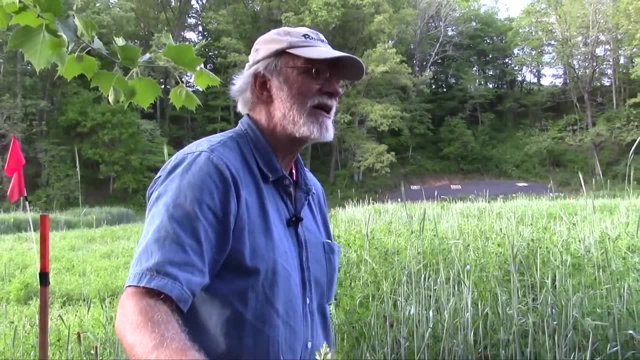 But we want to be able to say, yes, the herbicides did this. maybe they were even the most effective, but what about the soil damage? What about the ecological questions? We can't do that comparison without using them, So that's. 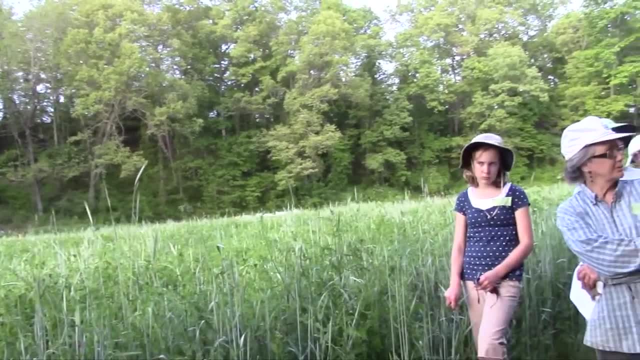 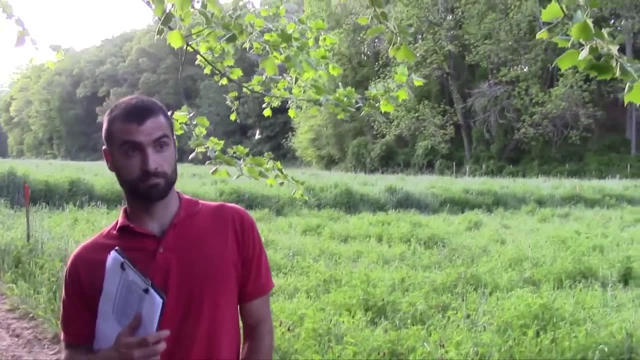 why we're doing it And we're going to use it to see. we're going to do the PLFA, so food web analysis- to see if it suppressed some of the biology. So we want to see all these treatments. I'm hoping. 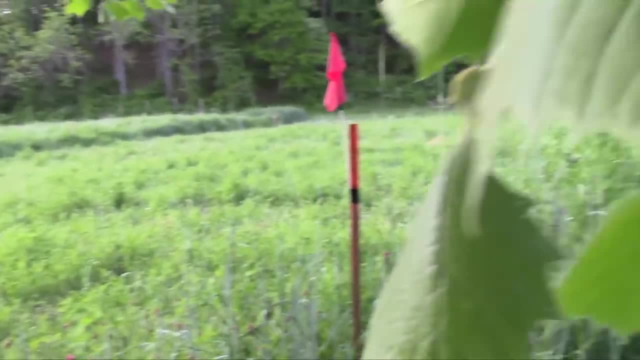 we can just do it with covers like that. Hopefully we can roll and plant through it. That's going to be our ideal. It doesn't even have to be the best way. If it's close to the best way, then the improving of the soil will make. 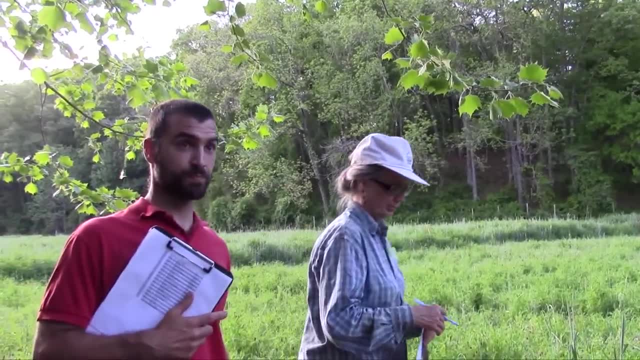 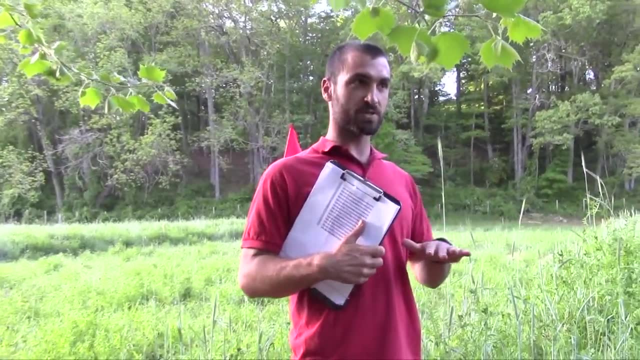 it the most cost-effective way to do it. I'm going to let you take over, Mark. Just go ahead and describe that. Thanks, Pat. So my name's Mark Dempsey. I'm a researcher. I moved here recently from Penn State Up at Penn State. 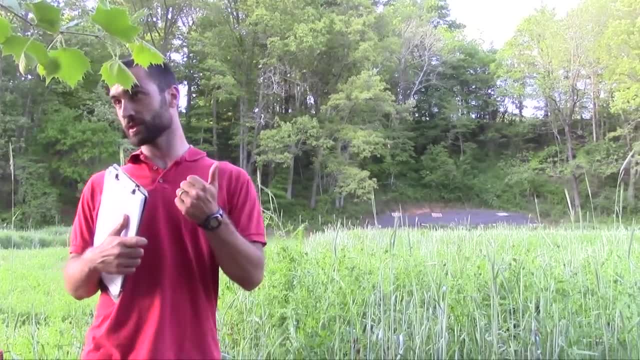 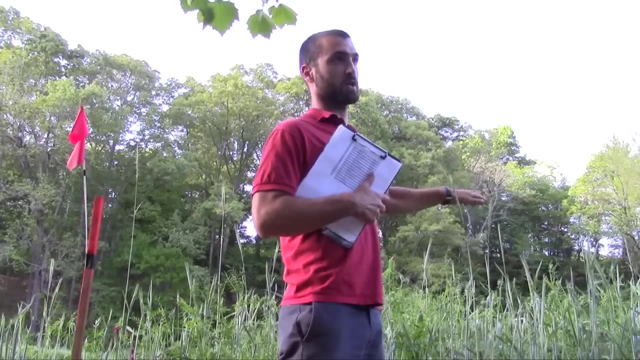 I was working in weed science research and also- I can't see you guys- and also in cover crop research. So the research that we were focusing on is trying to control weeds with cover crops and the whole related field of soil fertility and soil management and so forth. 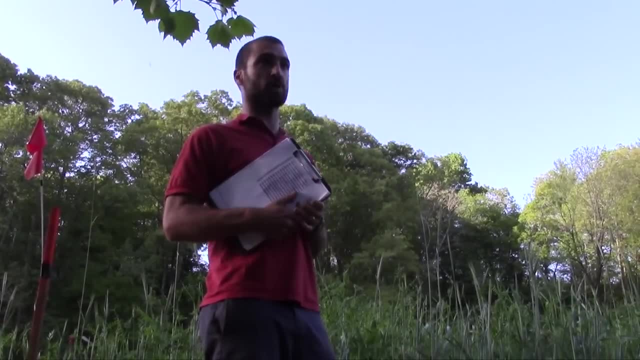 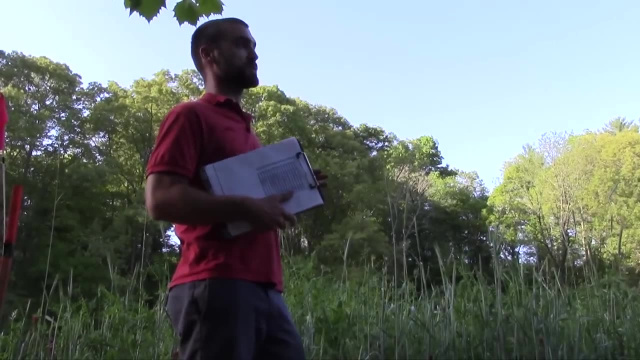 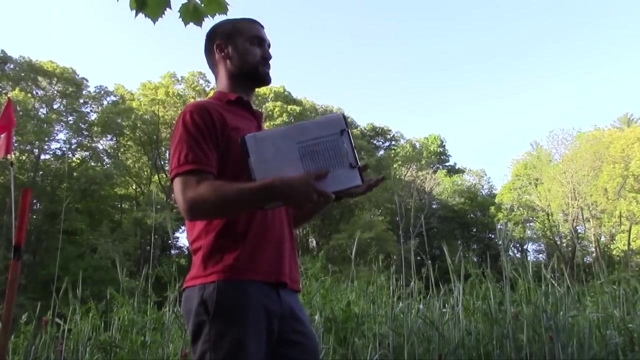 So I was happy to help out with this project and see if we could design an experiment that tackles mugwort control but also tries to address soil health and also maybe like human and environmental health more generally with the concerns about herbicide use and stuff like that. 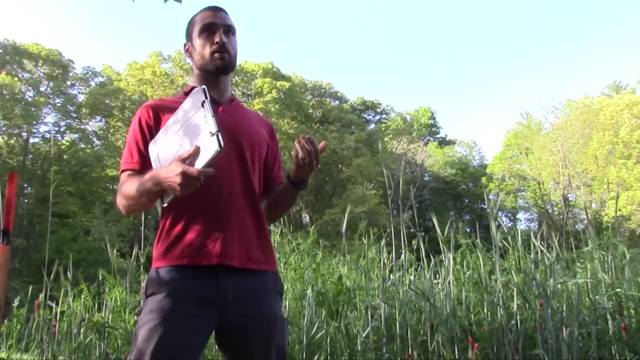 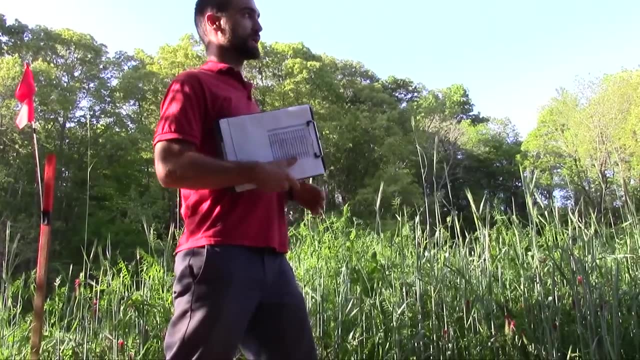 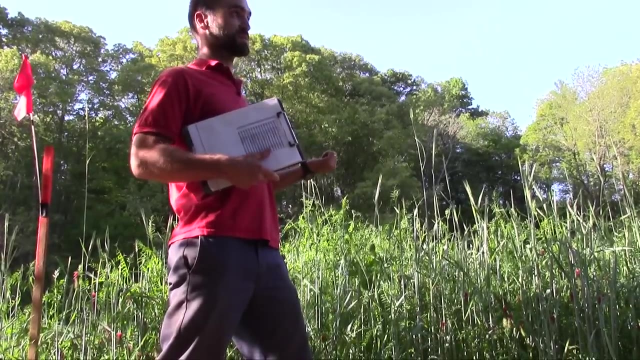 So if you were to take a step back and think about how one and maybe a conventional ag would deal with a persistent weed like mugwort, it would probably be to put down herbicide and or till very aggressively, Because a weed like this requires aggressive treatment. You're not going to be able to. 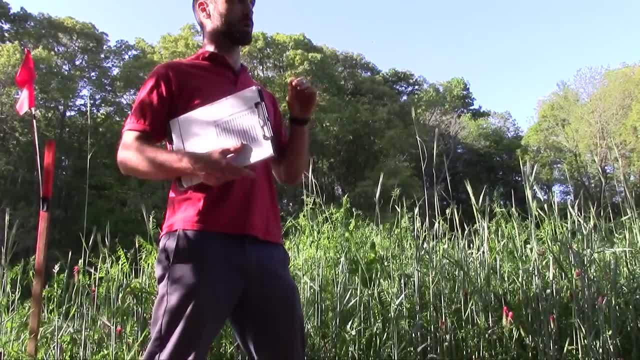 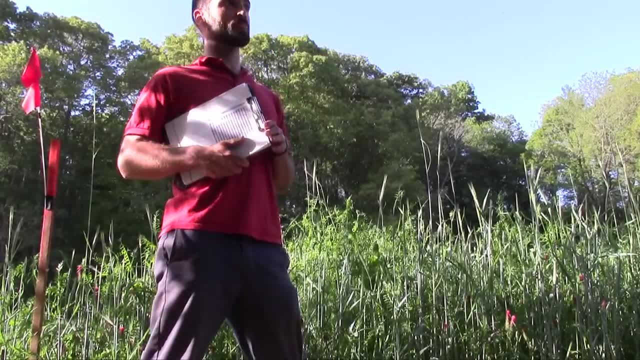 eradicate it. without that, And if you let it go, it just will grow right back within a few years and you're right back where you started. You've wasted that extra money you put in up front. So if those are the conventional approaches, 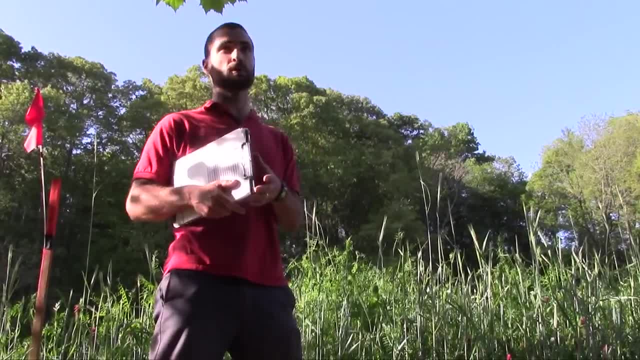 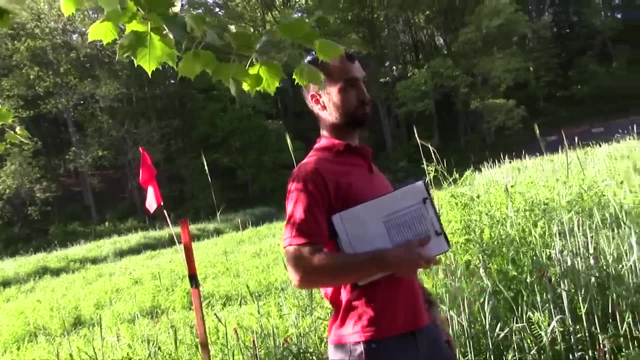 we wanted to kind of plan around that to see what we could do. that would be different. So the basic premise of this whole study is to use cover crops to suppress and out-compete mugwort in combination with herbicide, with tillage, with mowing and with. 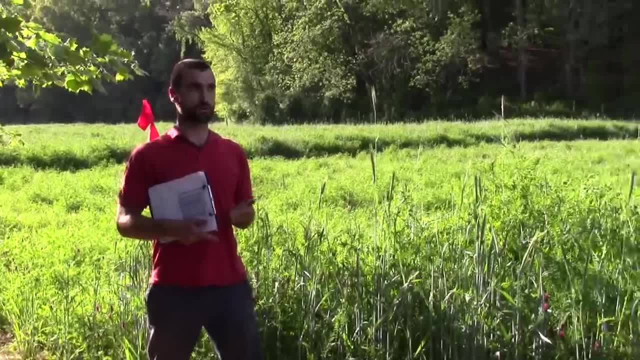 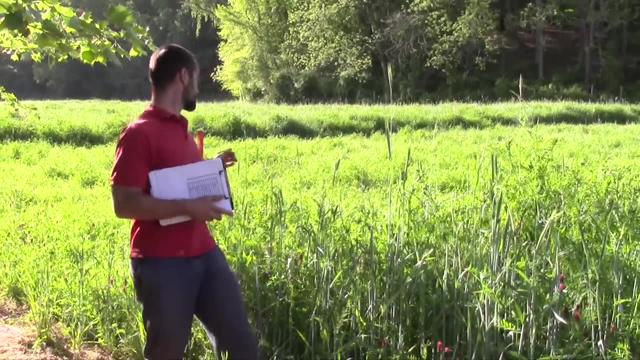 and then just suppression and competition all on its own, And so what we have here is a. so there are ten total treatments, that's replicated three times, and so, starting from here, at this flag stake, down to the next flag stake, are the ten and the first. 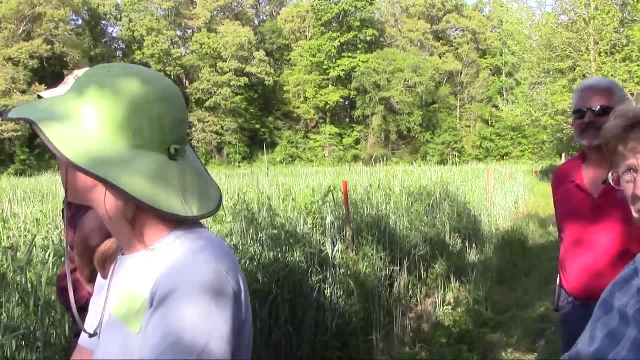 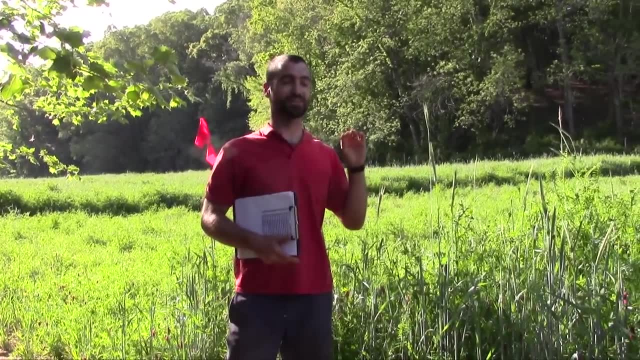 rep. And these first four are all chemical control, And so what we're going to try to do is kill the herbicide, ding the mugwort with an herbicide- sorry, kill the cover crop and ding the mugwort with an herbicide. 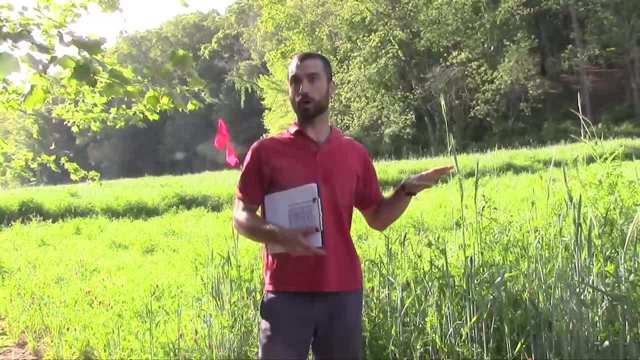 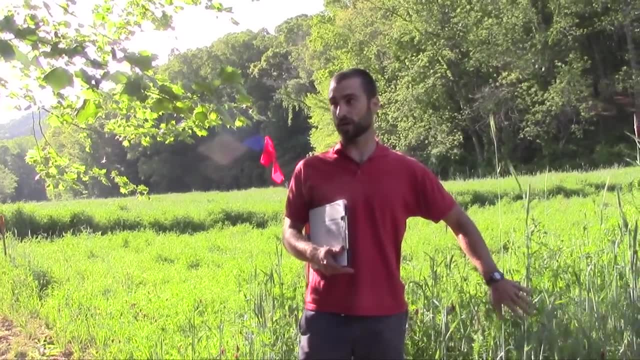 and then plant a summer smother crop into that. The summer smother crop is going to go everywhere here in this field. It's just a matter of how we deal with the cover crop and try to ding the mugwort up front. And so in this first block, 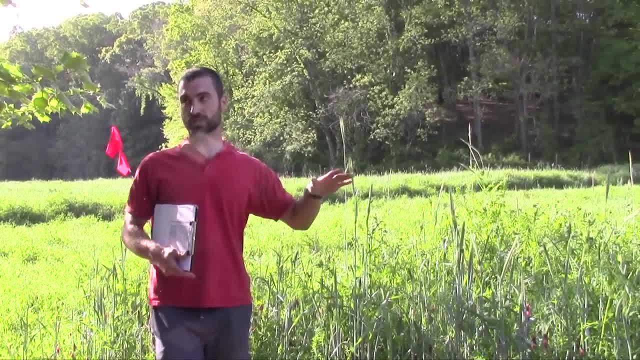 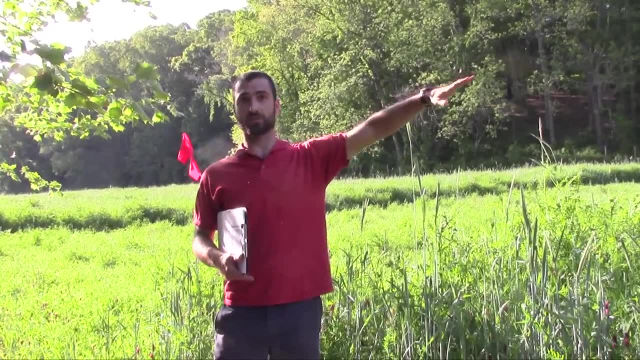 we're going to be doing like a glyphosate and dicamba or 2,4-D combination of herbicides And then in the next one we're going to be doing an organic herbicide, Both full rates. just see how they turn out, see if we can ding the mugwort. 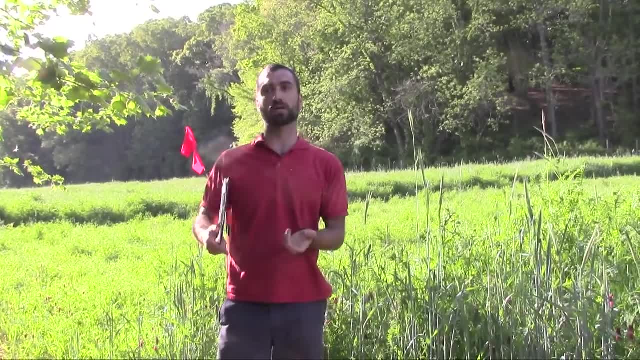 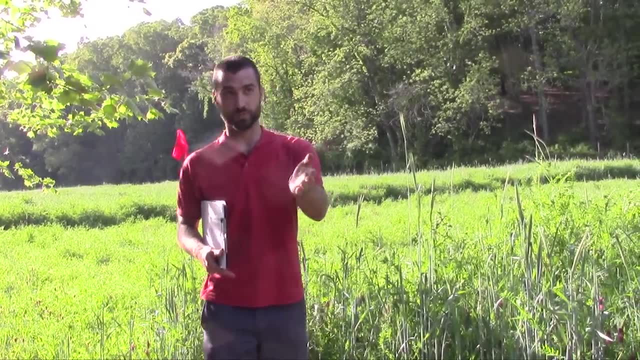 And all these plots. we're going to be evaluating how well we kill the cover crop, how well the mugwort does, and we're also going to be evaluating soil health and some microbiological aspects. PLFA's is a new one to me, but that sounds like a great idea. 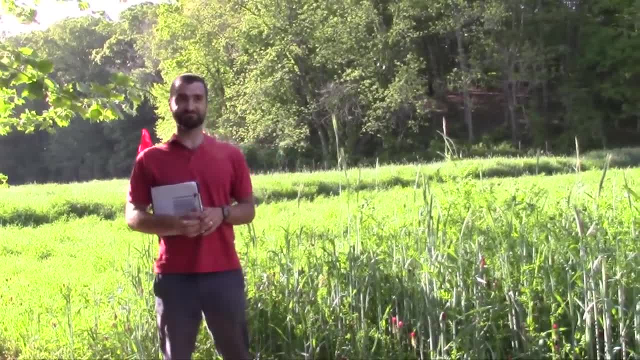 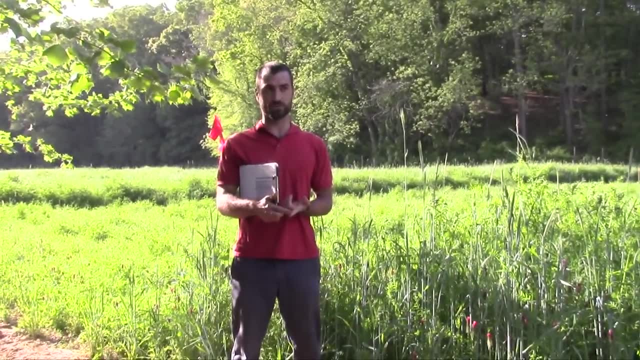 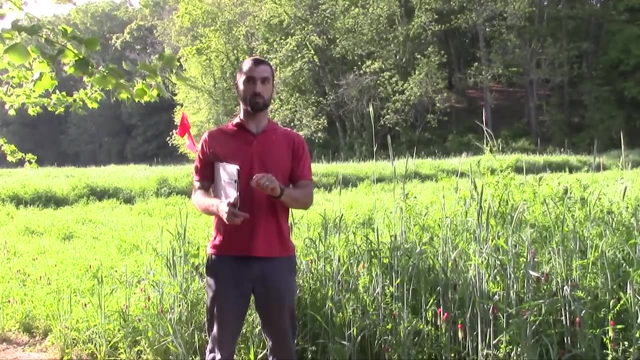 Yeah, yeah, we can do that. That's one of the treatments down there. So the microbial method that we are planning to use up front is just counting fungi under a scope, which is like the most direct way of quantifying them. But there, 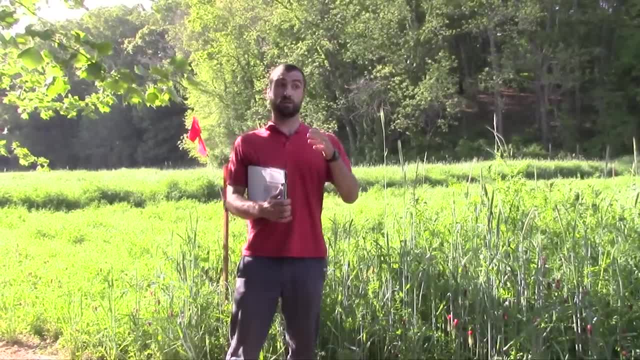 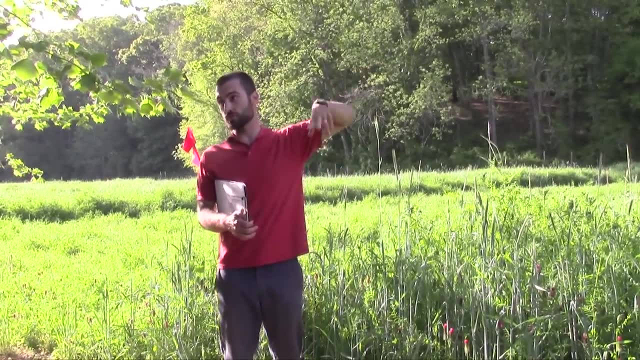 are other ways, basically using biomarkers that you can quantify fungi and a lot of other microbial groups. And so the next two plots, after these two full rate herbicide ones, are going to be a fractional rate herbicide where we're going to try to reduce. 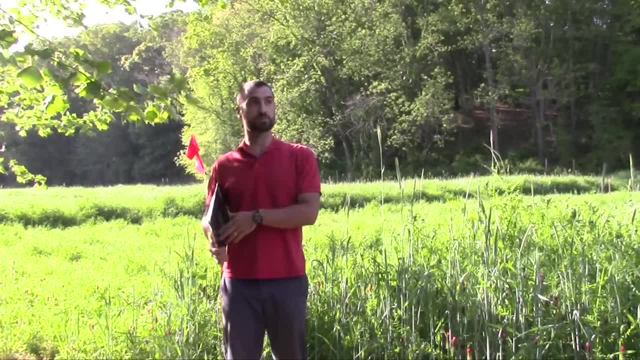 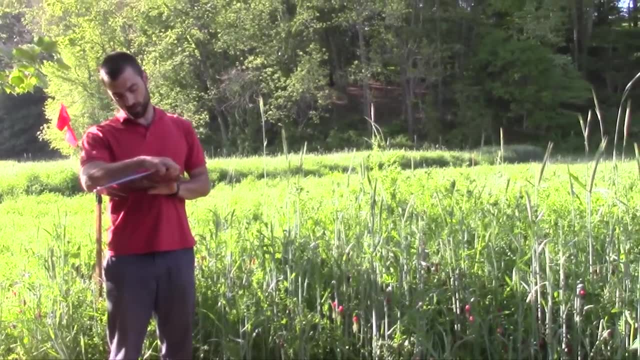 the amount of herbicide that we use by including a proprietary product in the blend with the hope that we can have it be as successful. It's just a test, And then, beyond that is, let's see, tillage, And so we're going to have two plots. 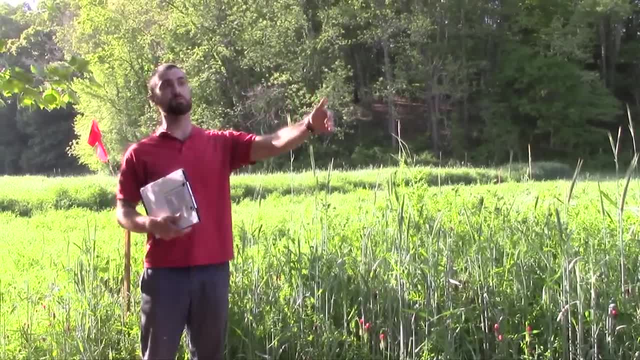 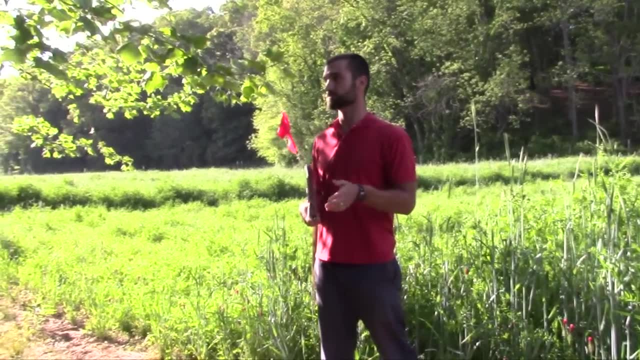 where we till intensively or we till lightly, And then the next ones after that are going to be mowing. So we think that if we continually put down a cover crop and then mow it, we can out compete the mugwort And then the 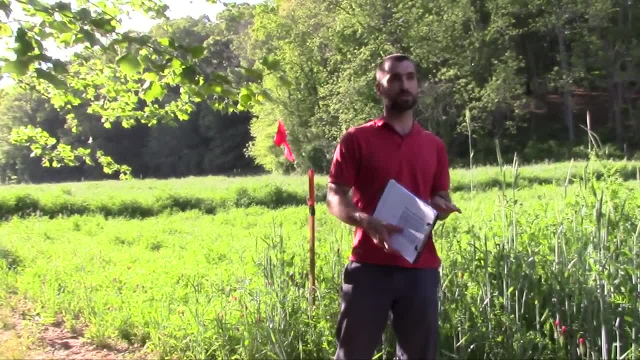 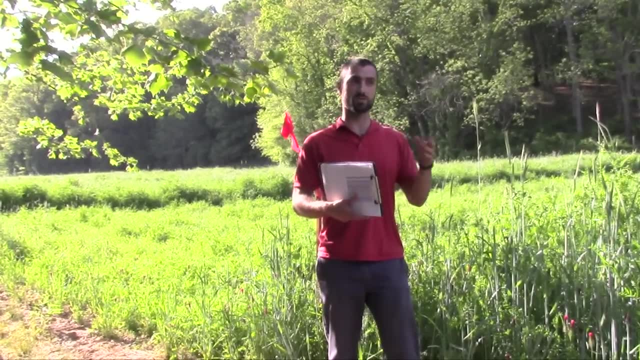 split there is that we're going to have annual cover crops versus a perennial forage, And just because the probably the commonest way an organic farmer would deal with this is by putting it into pasture or, excuse me, into hay where you're pulling out. 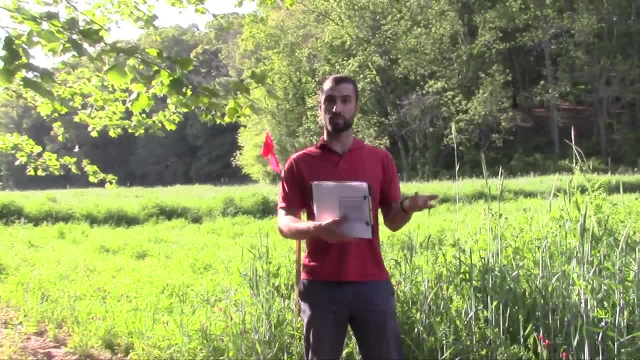 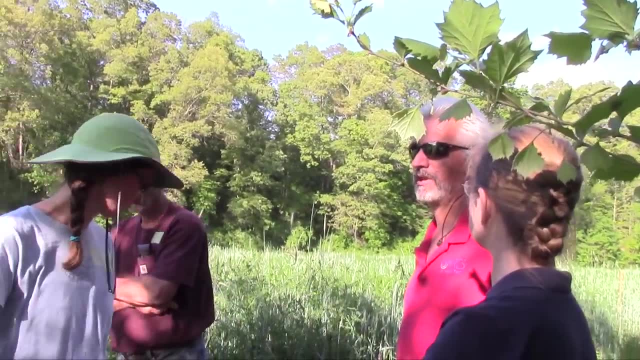 hay every year and you're making frequent cuttings with the hope that you can out compete the mugwort eventually over time. That's a longer process. They would hay it or they would till it in right, Or the combination. over time They might also just feed it right. 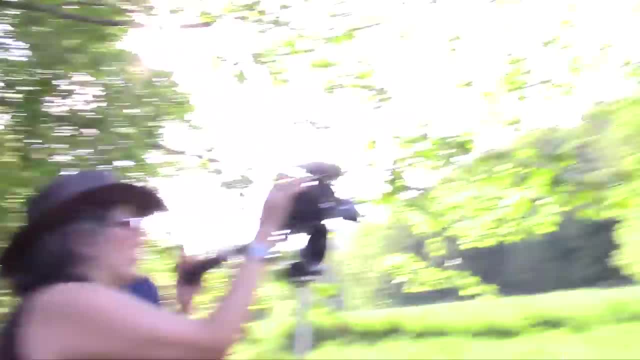 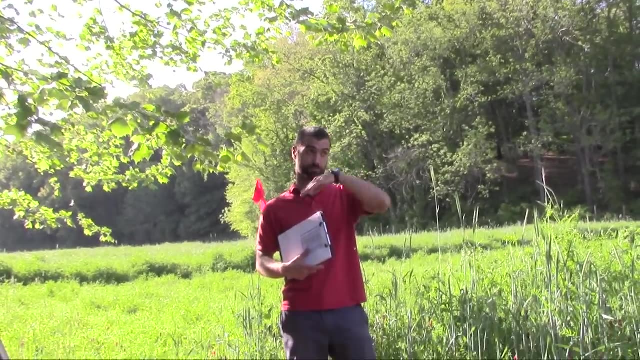 Let cows or something come in and feed on it instead. Sure, people might graze that. Yeah, another way is another way. Sure, It gets more complex. What about the crimping that they were doing over there? The final two treatments are going to be: 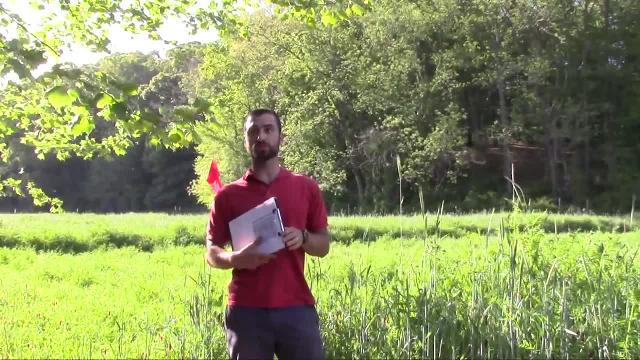 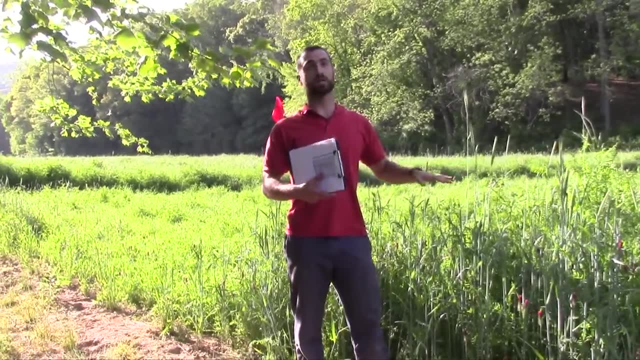 just roller, crimped and then planted into that. And so what we're thinking is that, with a cover crop like this, we might be able to suppress it with just suppression and without chemical or physical control methods. right, We're going to just roll everything down. 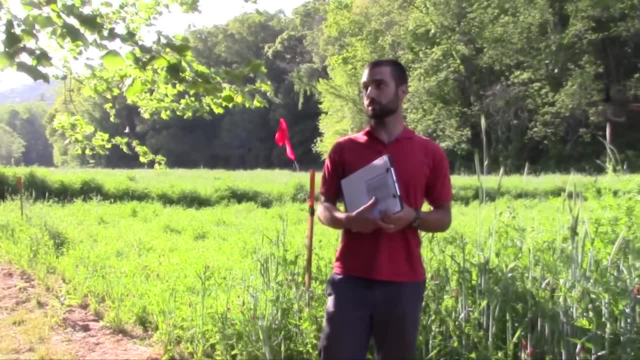 plant into that and then try to out compete it with the next crop. We're definitely pulling for that method. That's the best method environmentally, That's the method we hope is the best, And it's the lowest cost method too over the long term. 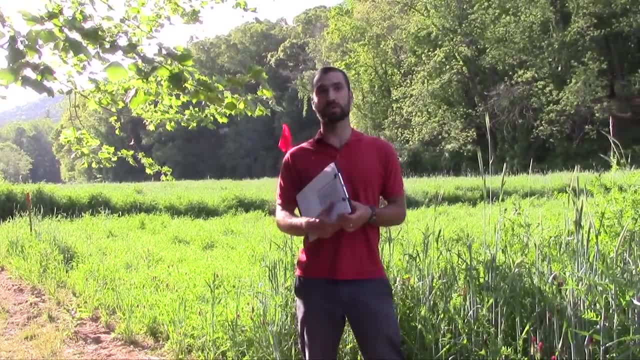 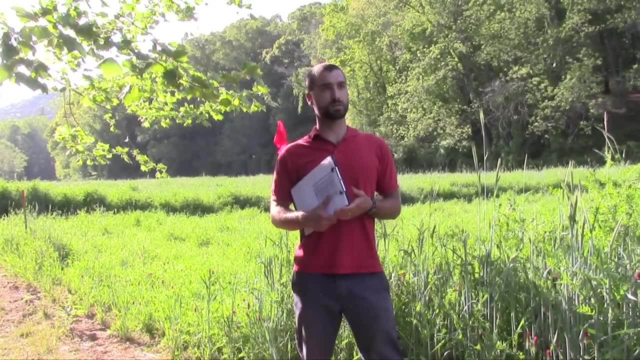 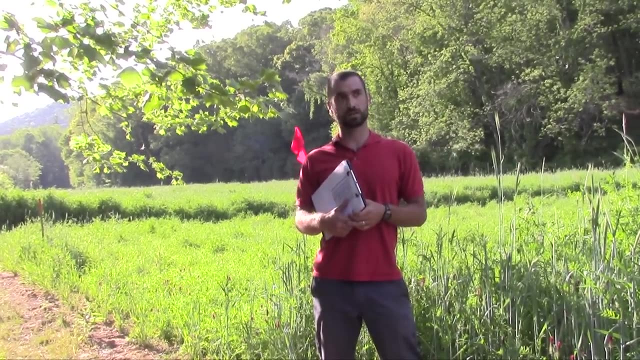 And the roller is a great piece of equipment. It's a great investment. That's the basis of the experiment. I guess we did have a few questions we wanted to ask Ray, and to Dave I guess we'll just say we had thought that we were just going to go. 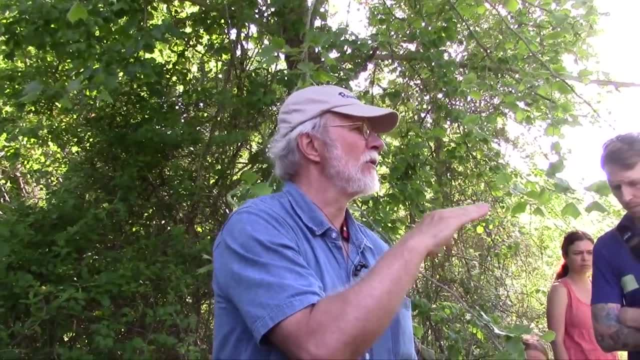 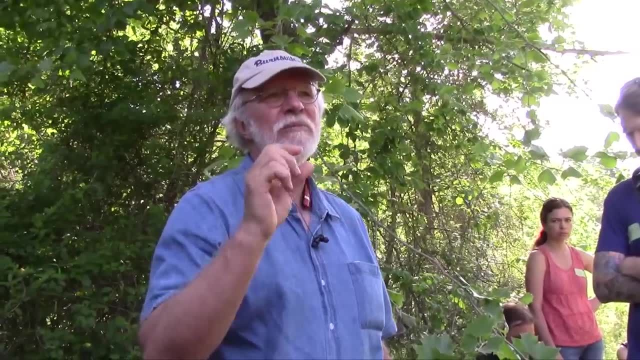 with Nudex and probably we said maybe 25% Crotalaria Sun Hemp. Yeah, that's what we thought we were going to do. We thought maybe less diversity would be denser, would be harder on the mugwort. But then 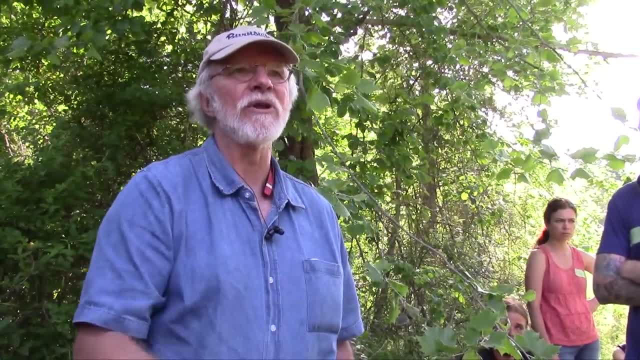 Dave said he thought that the mix that you all just designed would smother it really well, So I just wanted to have him here and then get Mark to ask him the questions. That's why we can do it back at the place, He doesn't have to be looking at it. 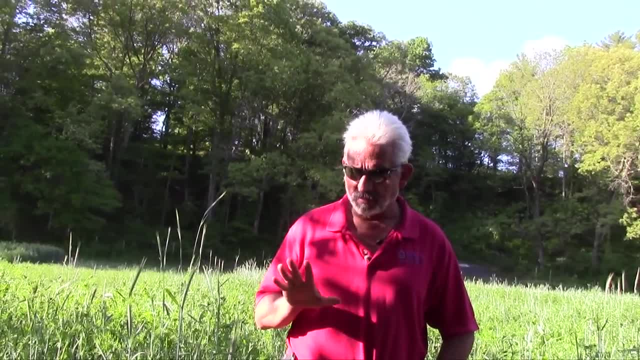 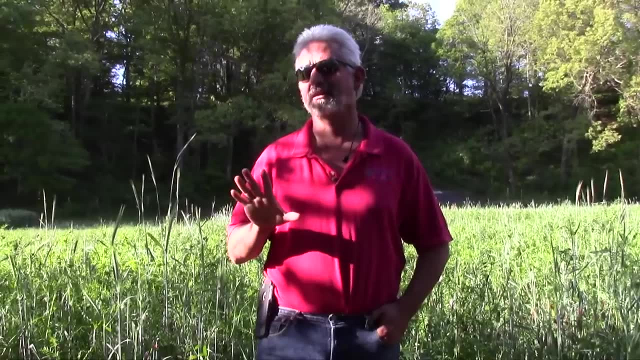 The nice thing about having a mix is that they'll all bring different chemical messengers into the system, But it complicates the. we don't know who's going to do what And I don't know if. I don't even know if our science is. 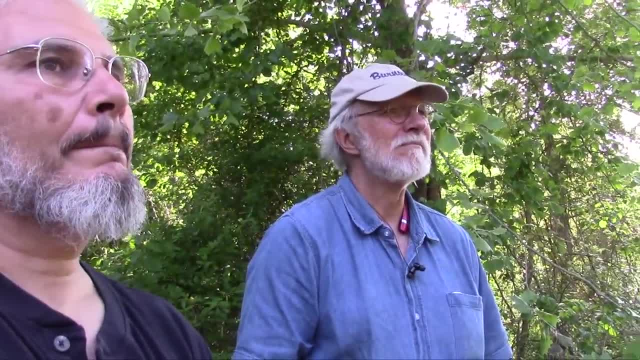 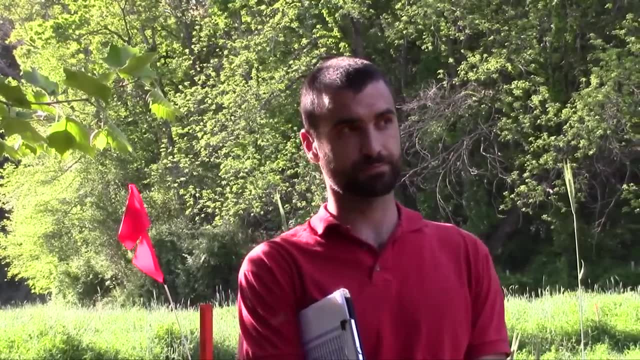 that far ahead. We can just see what the impact that you'll see is, Because you're going to count how many mugwort you have per plot, and that's what you're going to do. I applaud you. Thank you for helping us. 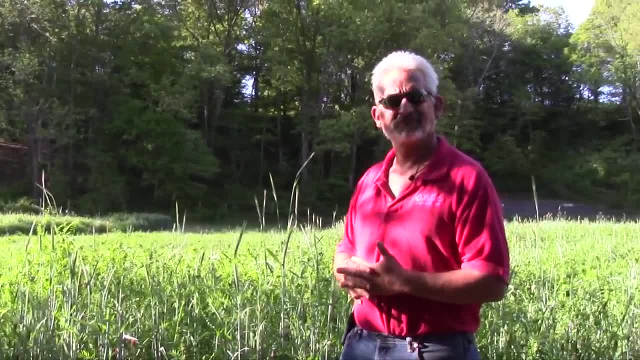 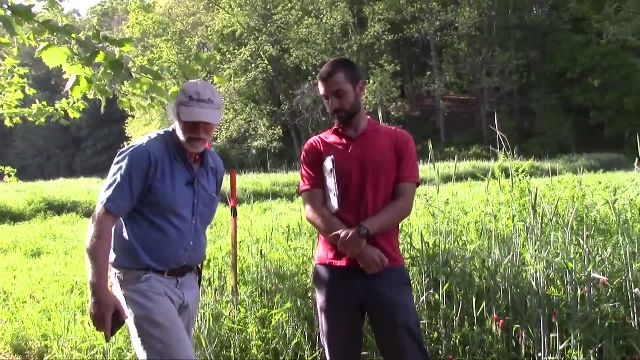 It's going to be a lot of work. It's a several year project. Two year project, Two years- yeah, It's going to go a long way. probably could, When you're leaving, just note that the mugwort by the road is probably the weakest. 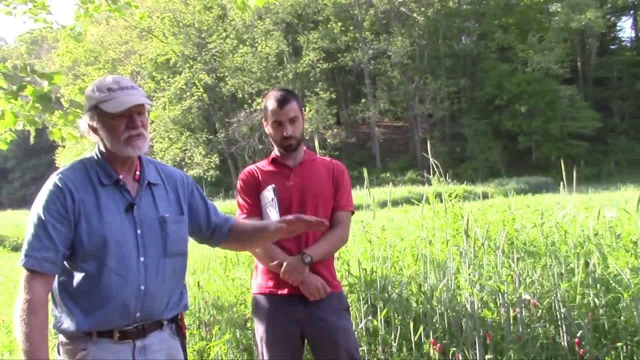 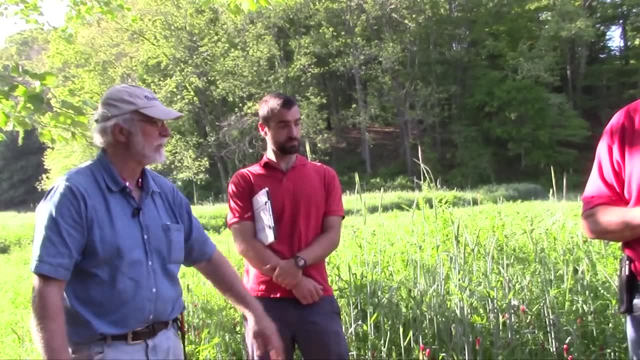 Because it gets driven out and all that. Imagine that it would have been much thicker in there and yet right now it's totally suppressed. It's not dead, It's waiting to pop again, but it's totally suppressed. But one of the things 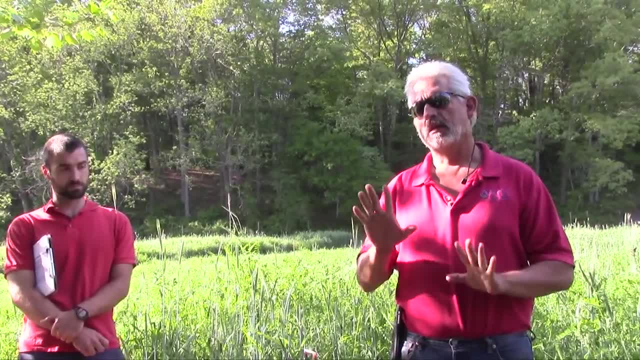 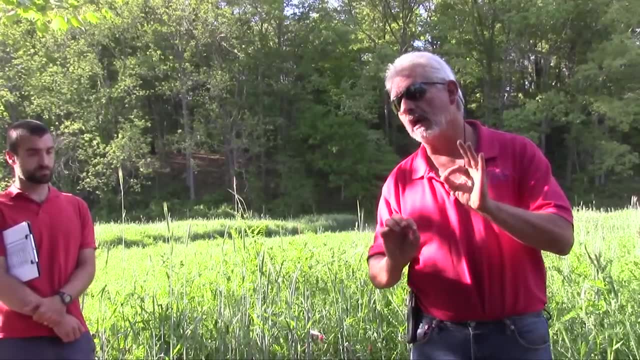 you have to realize about weed species. the seed banks are there. Arthropods and all these little critters that we talked about, millipedes- all that will eat weed seed. The fungus also will degrade weed seed. But once you start bringing a healthy soil ecosystem, 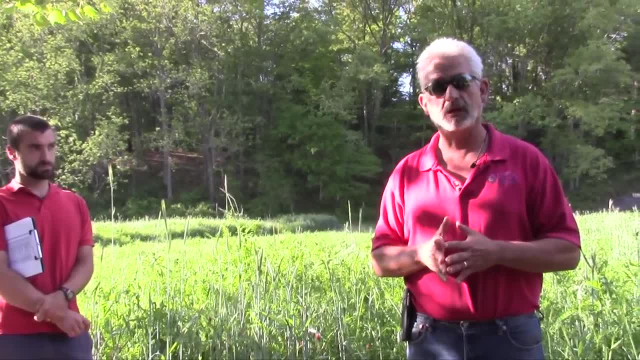 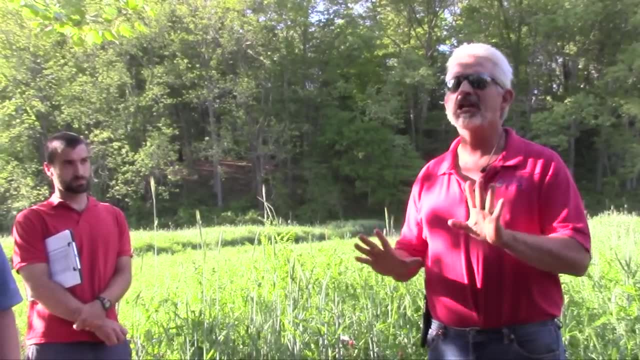 that will reach an equilibrium that will help suppress some of these weeds. will we ever get rid of completely weed seed? No, But the best way is putting living covers. So learning how the ecology of the weed seeds, and that's why we have Mark here to help us out. 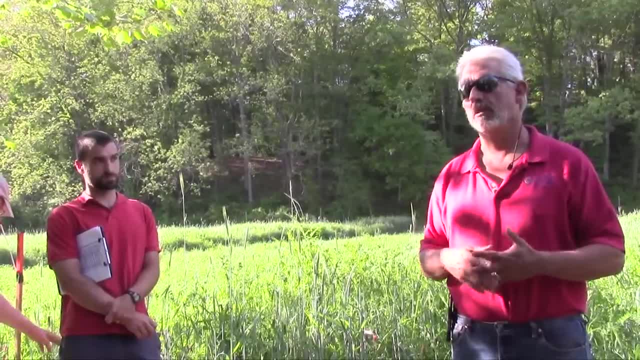 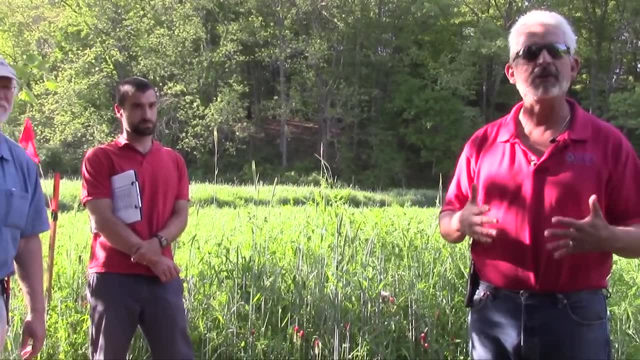 because he understands some of that Using all these tools. but if we can use ecological means before we use physical and chemical, and those means we're better off. We're trying to understand the system better than just trying to force it. So that's our thought process. 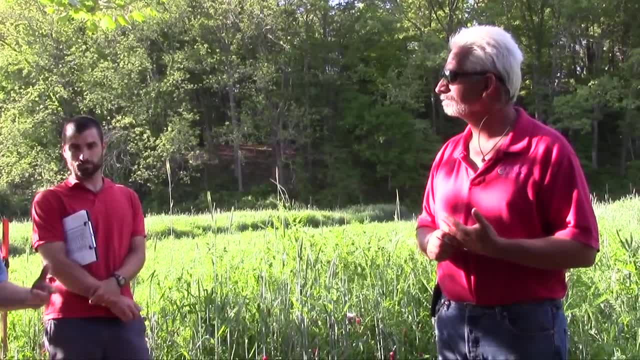 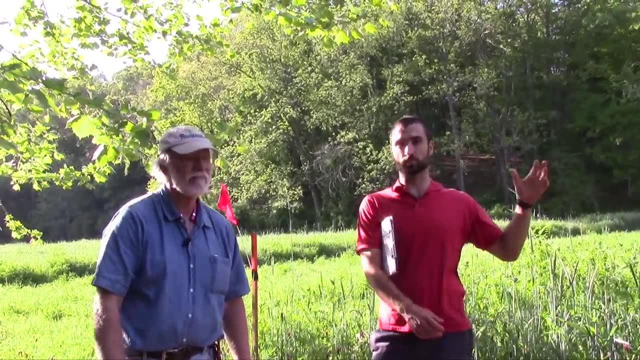 So that's it, And I'm thinking that what we learn here will be not exactly, but pretty broadly applicable to other things like Johnson, grass and things like that too- Same kind of concept. So the goal is to have a high quality educational product that we can put out there for people. 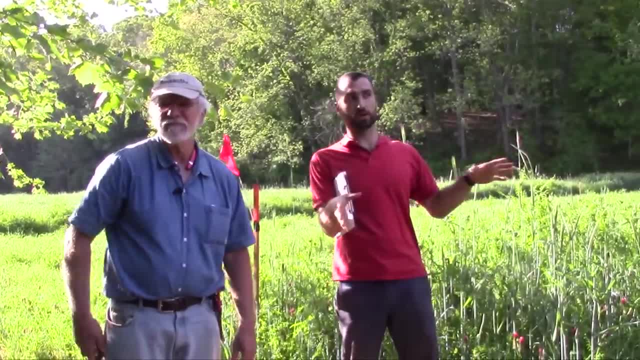 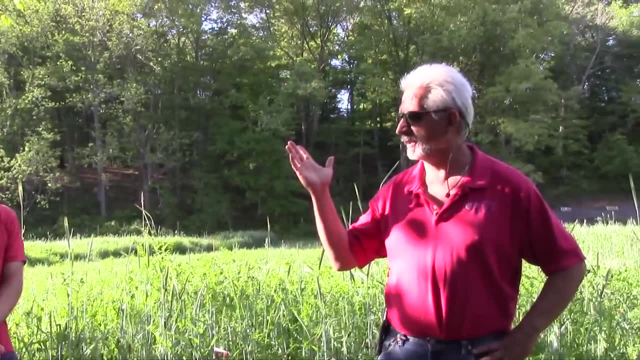 who are struggling with this kind of weed or similar weeds, especially in this area, that might be most applicable. See how to deal with them in the best way. That's a brutal one And it's hard until it just spreads it around. But if you can graze it hard. 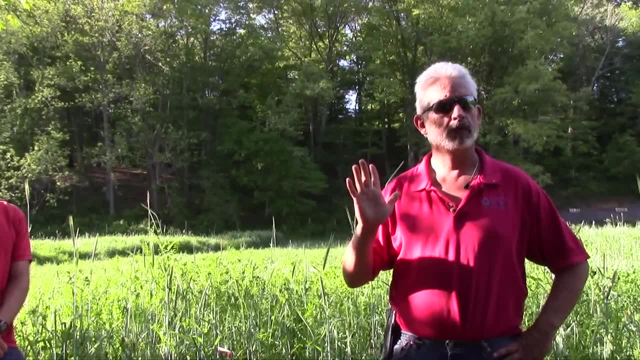 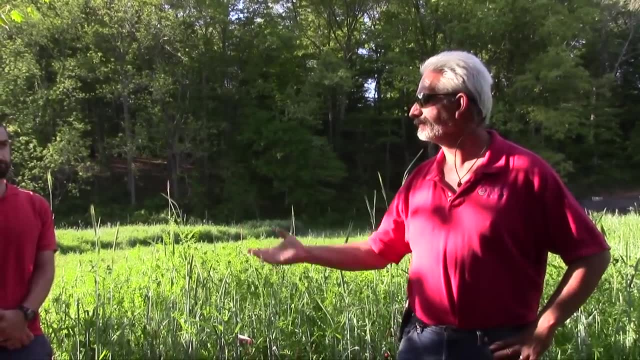 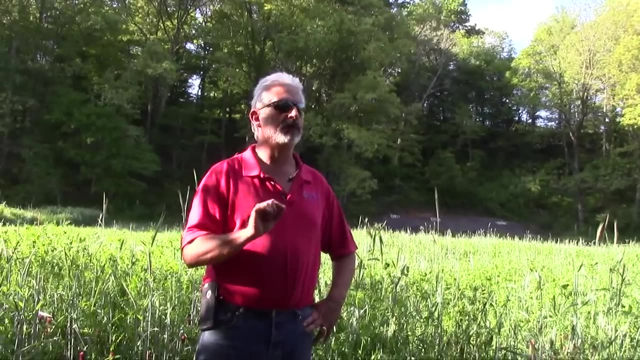 it's a fantastic grazing. it's great grass for grazing. So using the right biological tools to suppress it is always better if we can learn how to use that. What's the difference between weed seed and cover crop seed? The weed seeds a lot of these. 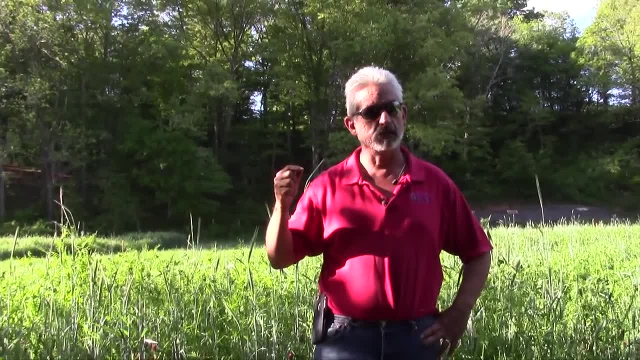 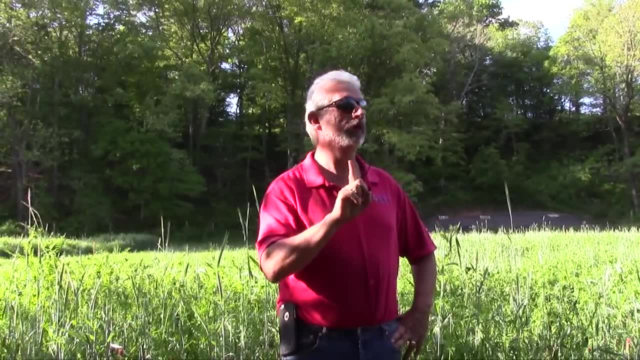 and Mark, you jump in because you're the weed scientist. a lot of the weed seed plants are designed to do. all of them have purpose and design. Remember I was telling you: the majority of these plants will put 40-60% of their energy into root exudates. 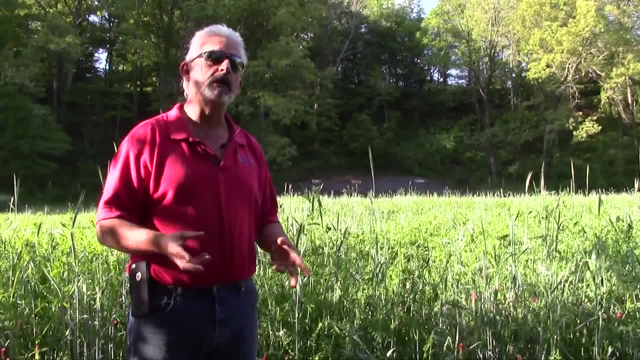 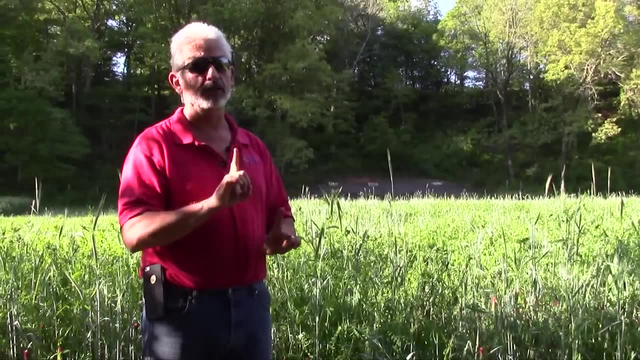 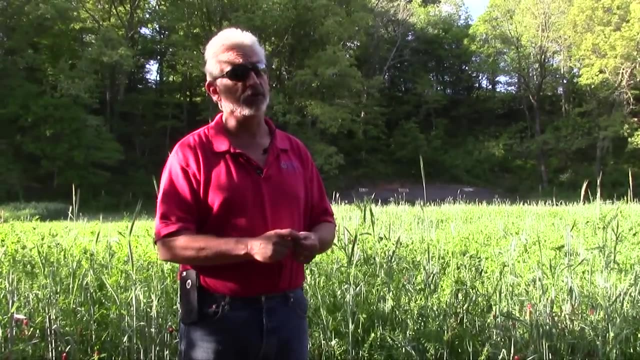 I want to feed biology. Weeds will probably leak about 20 some percent. They put their into seed head. They are secondary, successional plants. Their design is to cover and they also tell us: do you have a deficiency in calcium, Do you have a deficiency in this? 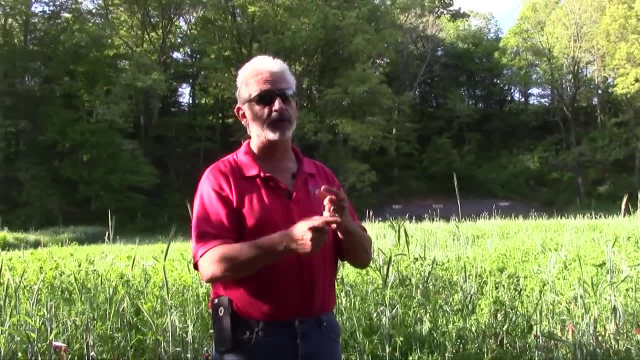 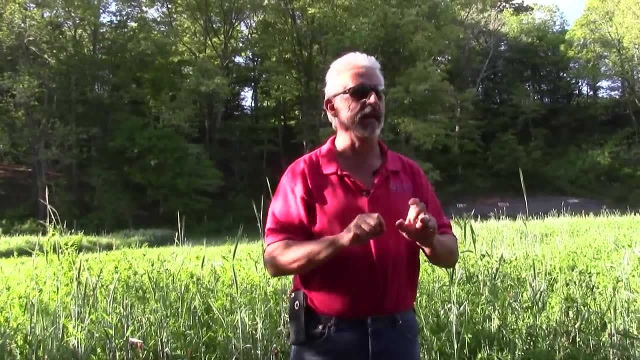 They're indicator species But nature wants to cover itself because you do a lot of disturbance that they don't want. It's a mechanism. They'll put a lot of their end product into seed head- Other things you want to add to that. 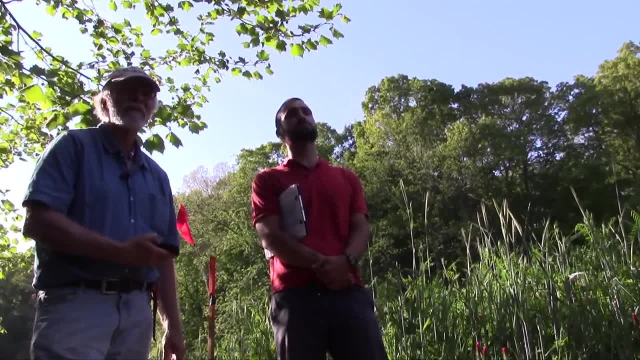 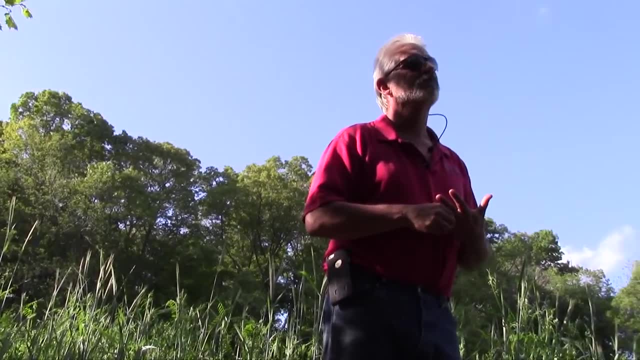 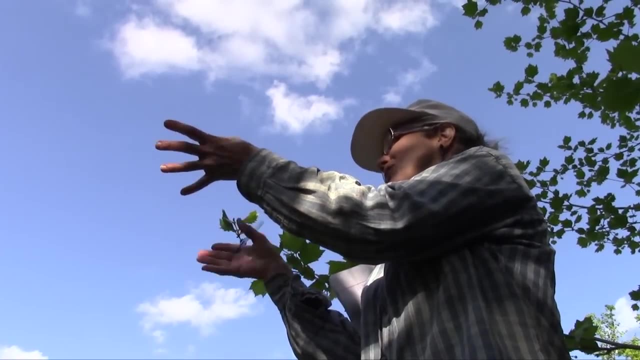 What exactly do you mean by? how are the seeds different? Do you mean the crops? No, You want to get rid of this plant because it's a weed, but you want to keep this plant because it's a cover crop. You were saying there was so much mugwort here. 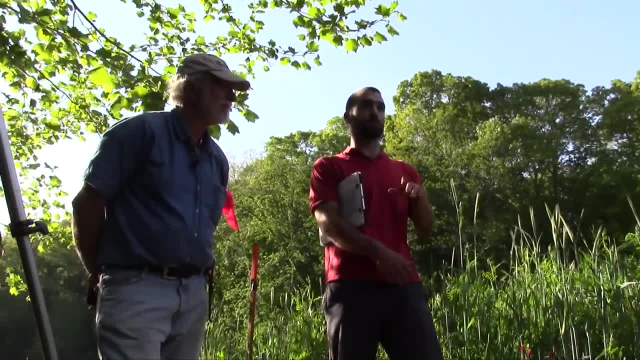 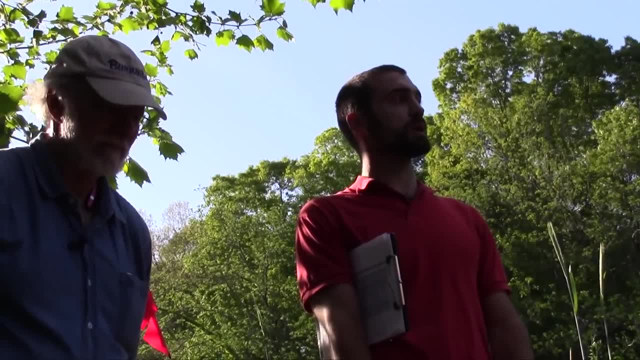 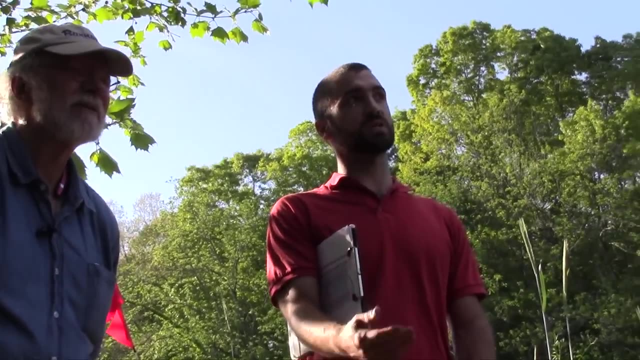 covering things. What we're planning to do is the seed. thing is a little bit different with mugwort. because it spreads by its rhizomes, We can easily control the cover crop. It rarely becomes weedy to affect our cash crops. The mugwort will. 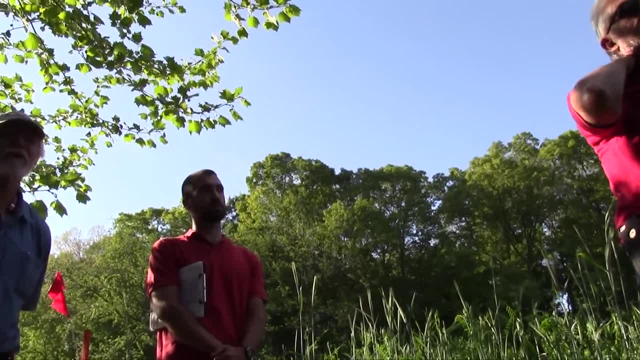 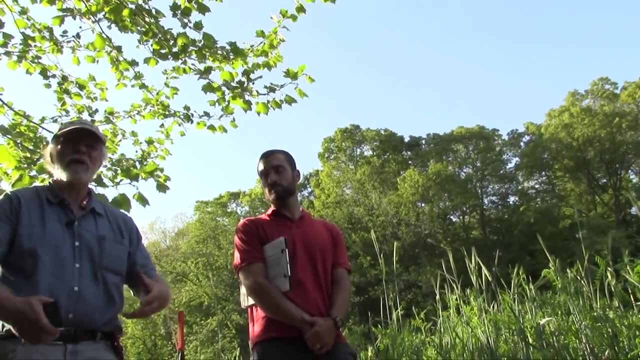 put you out of business. It will overrun your crop and out-compete it. It's interesting because I pulled up some for Ray. We looked at what I pulled up and he said: what a great aggregator. It's not hurting the soil. There's nothing bad about mugwort. It's got tons of great uses. It just doesn't work for how we want to farm here. We're humans, right, We want to control the plants we have here for our purposes. We've got to make a living. 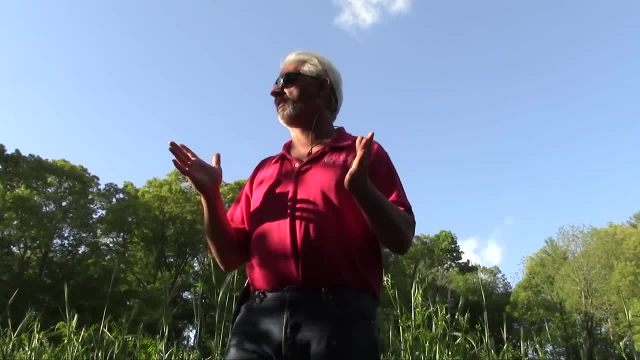 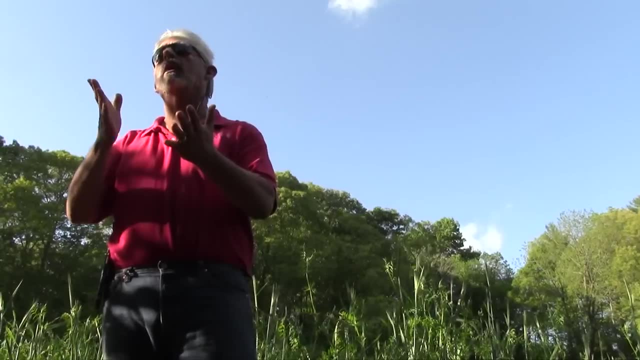 At the end of the day, we've still got to make a living. I tell you, being in the Peace Corps for a couple of years, we've got to be able to. I want you guys to make a lot of money. There's nothing wrong with that. 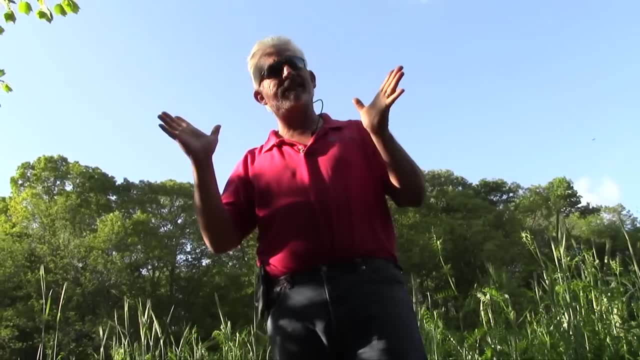 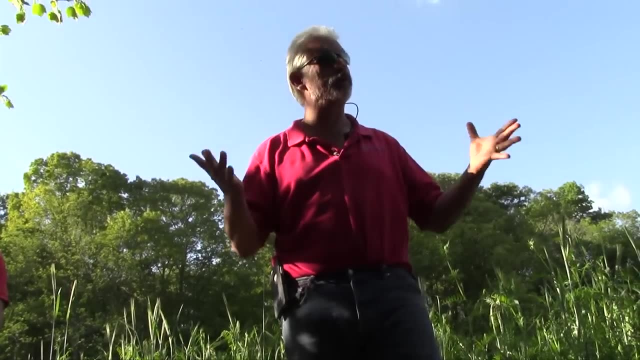 But we've got to do it in a way that's responsible. Another thing about weeds that we've noticed: they're secondary successional plants, A lot of them like bacteria-dominant soils. A lot of disturbance, a lot of tillage. 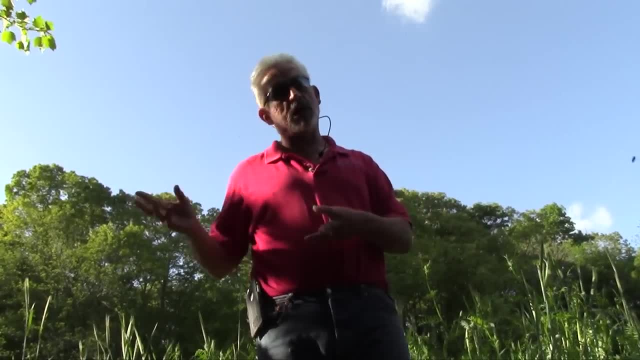 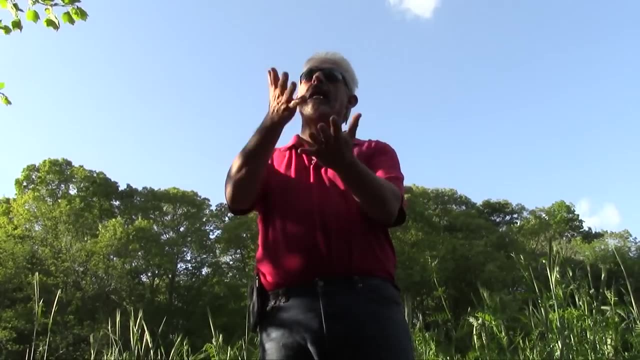 They're the first ones, the first invaders to come in. If you're doing a lot of physical disturbance, what we want to do is lessen the disturbance. then the soil biology changes, because the plant community and the soil biology are very connected. In fact, in the science literature, 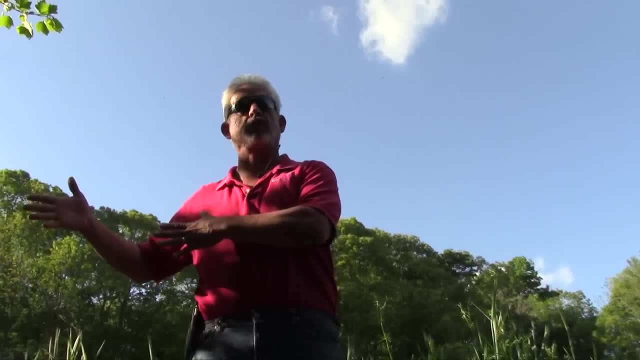 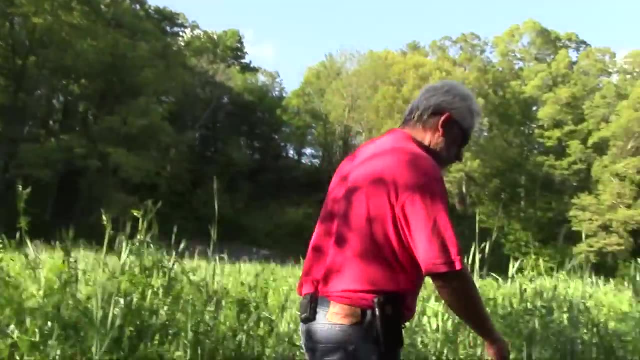 we don't know who controls what. It's that complex. So if we shift the biology to more fungal, the plant community is going to shift. Let's go eat. Let's go eat, absolutely. We've got six minutes to get back there. 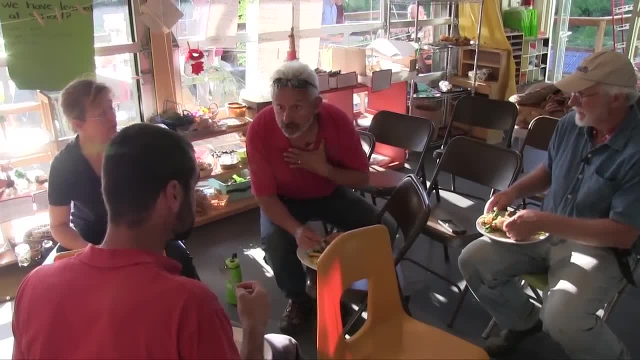 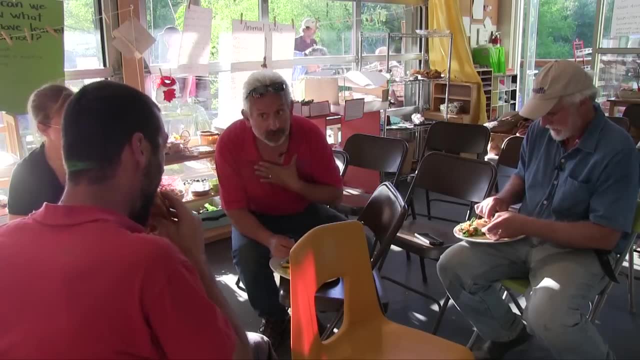 We can do it. But what I don't appreciate: I said: disprove us, Go get your equipment and disprove us. We'll help you get a CIG grant, But don't sit there and diss us and you've done nothing. 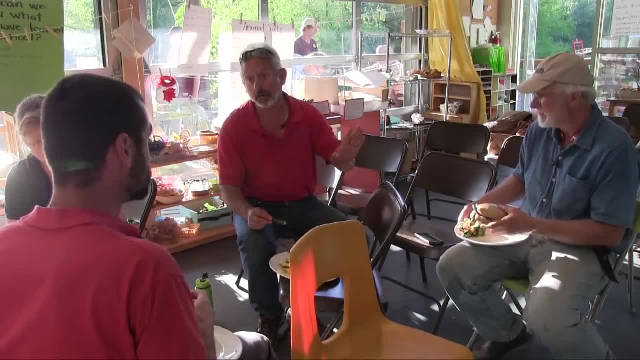 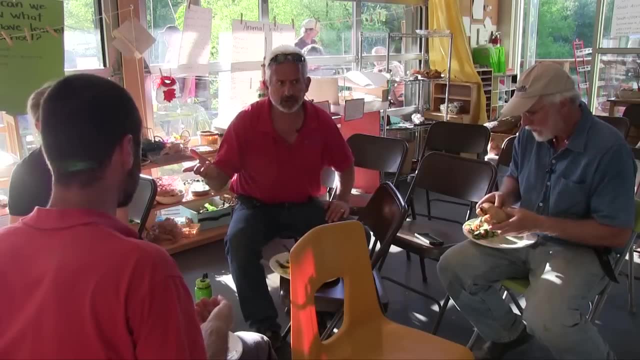 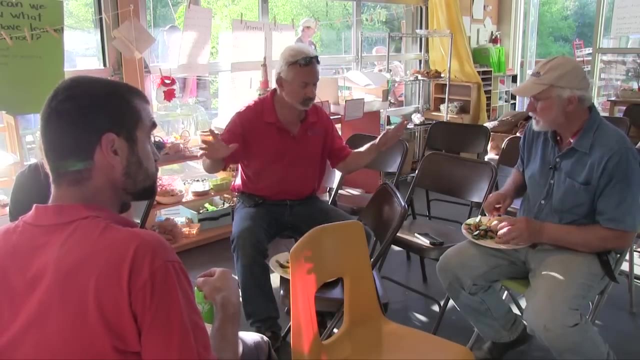 That that's not appreciable at all. That would be really valuable research. Absolutely Just to have somebody try to disprove that. We want you to disprove it. Good science will stand under scrutiny And they should be able to work everywhere. 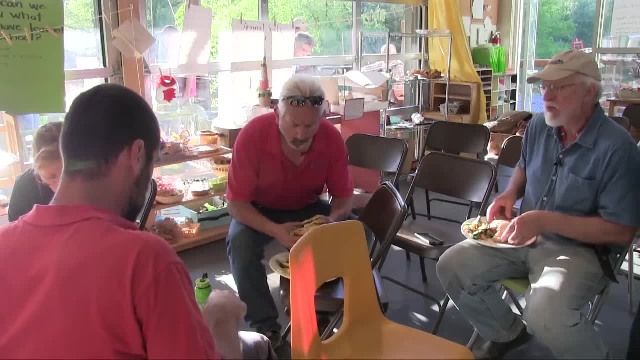 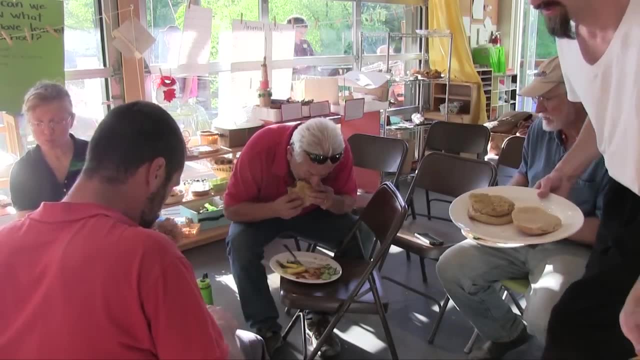 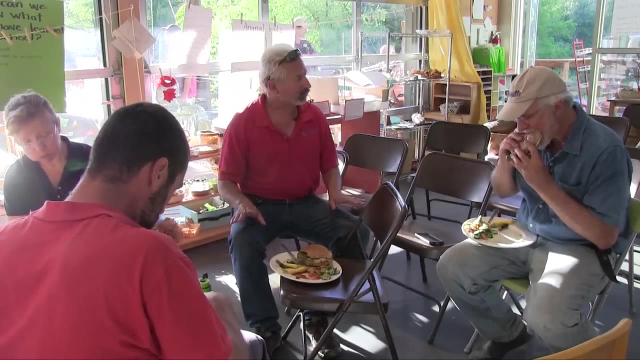 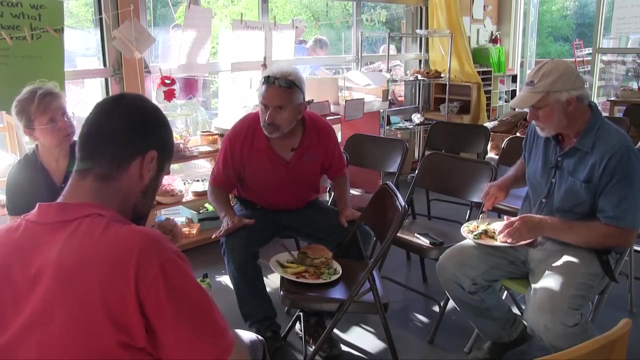 I'm going to just settle the matter. Yeah, yeah, And It's okay. Hey, This is a cucumber. Look, please, Mark. People are arguing. See, in my mind we're almost burning it And we're worried about the violin. 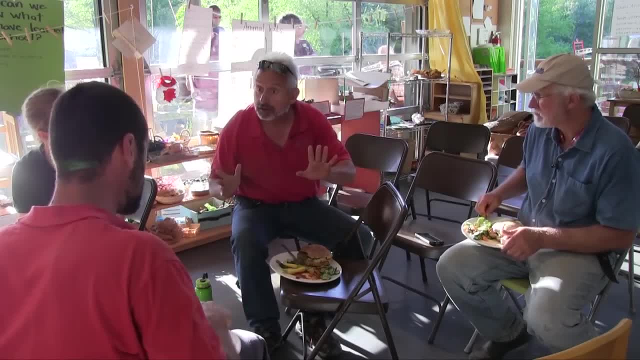 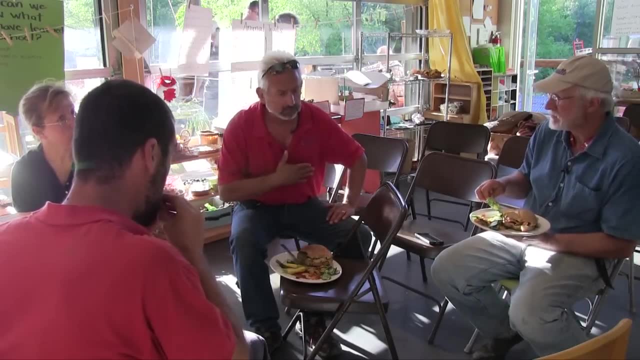 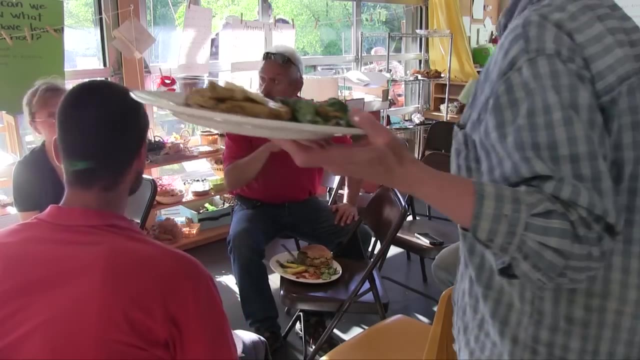 If it has three strings, five strings really. Come on, They haven't driven the hook and track like I have. I drive it, I fly it. It's a mess. Let's be realistic. My very best friend, Huh. 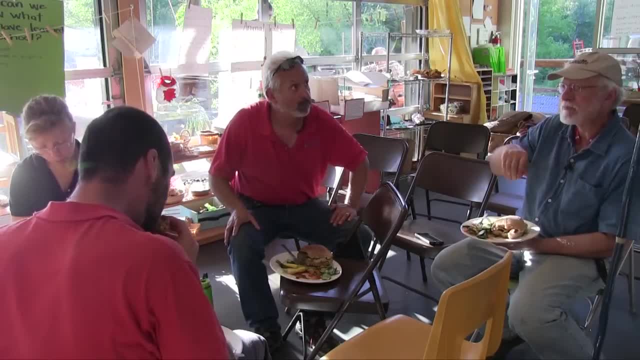 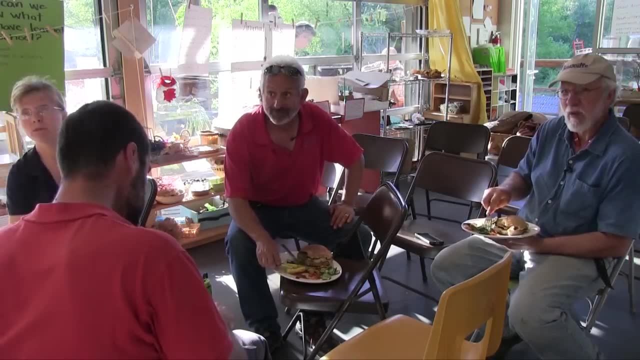 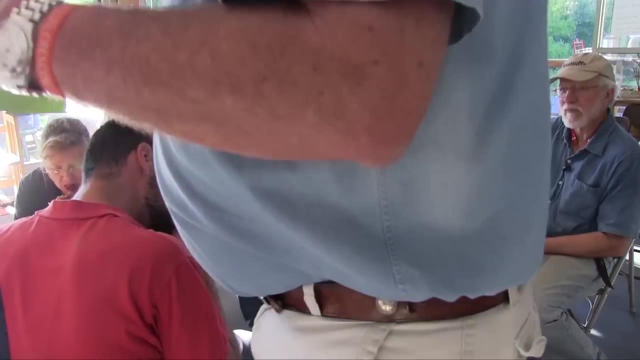 Tony Carlin, Nice to meet you. Tony, You can grow 4,000 acres of hard corn. All right, And he's All right. So Good to have you here. I'm enjoying the meal. You see, Mark, if you go, look at the country where it's at. 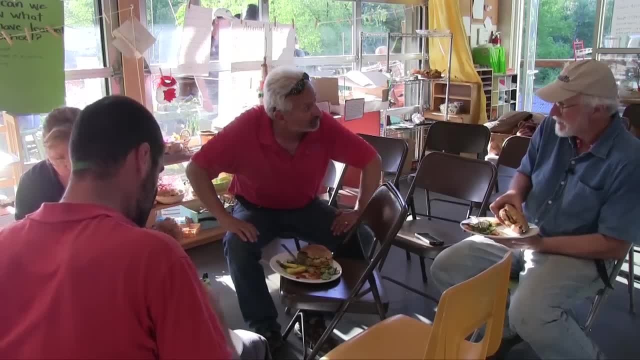 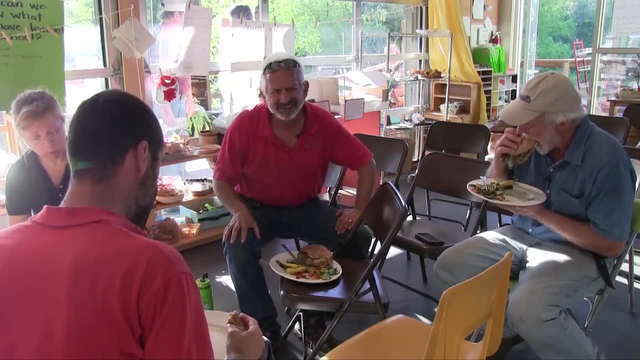 and we've been doing this for 75 years. Our ages have been doing this for 75 years, And we still have conservation. Oh yeah, right, And we're still having Dust Bowl. Come on, I almost want to blow a blood vessel. 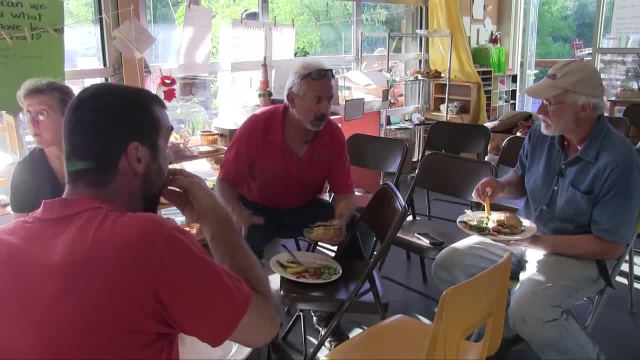 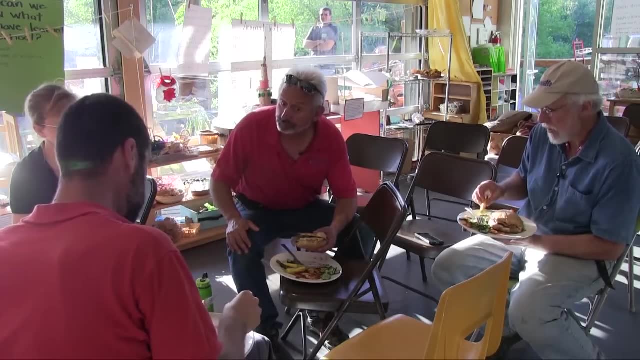 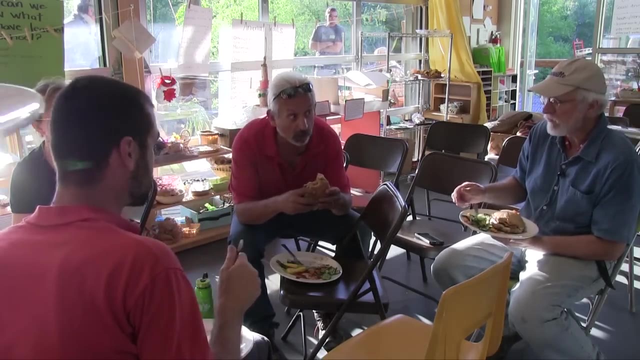 when they say we've got to study it more. Have you ever Googled organic matter? Google it. There's millions of papers that come up. I can't even get people to come up and do it in soil, Really, If I had to do one conservation practice. 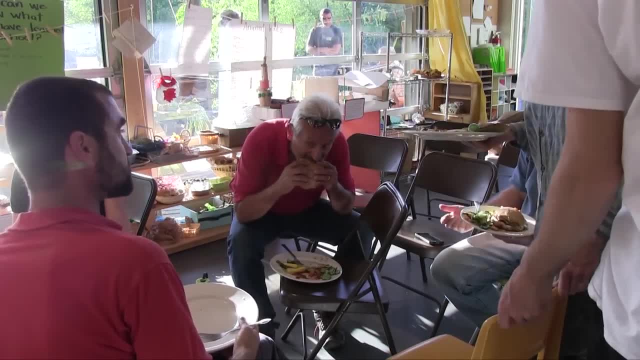 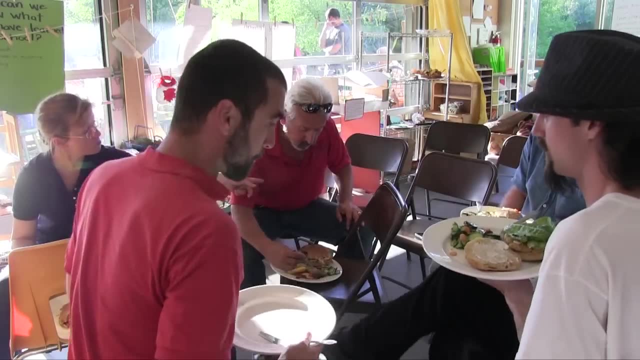 I would do it in soil Here. you can have this one if you'd like. No, I just want to try it. I like when you kid with me, I guarantee it. I've got like two minutes and then I'm going to go. 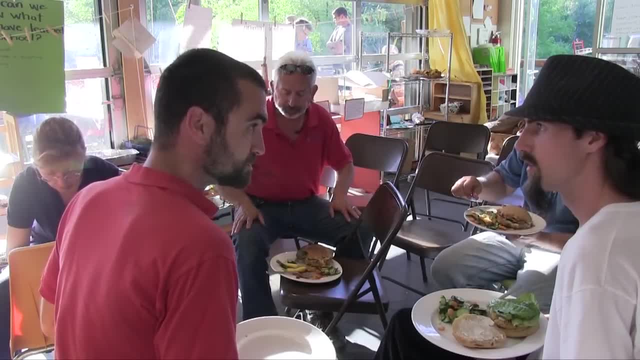 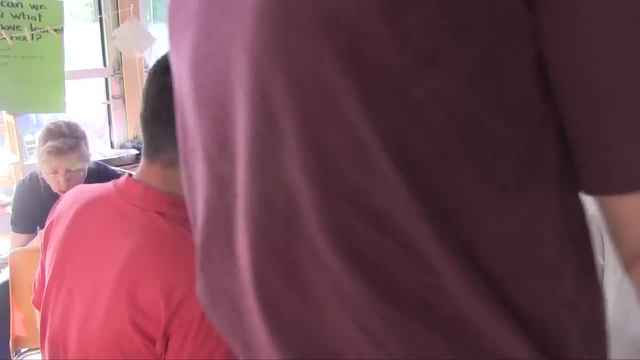 I'm running late. I've got an out of town guest in town. Email me to remind me that I'll connect you with Dr Haney. That would be great. He's a friend of mine. He works for ARS and USDA in Texas. 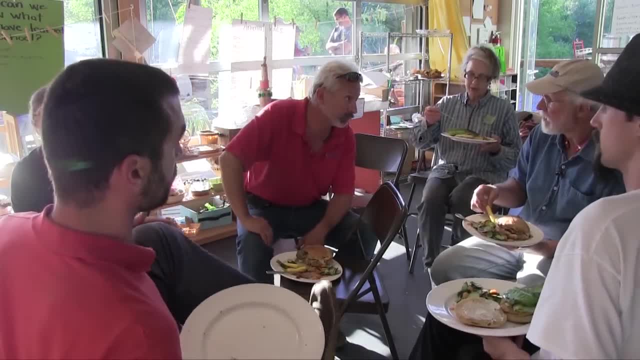 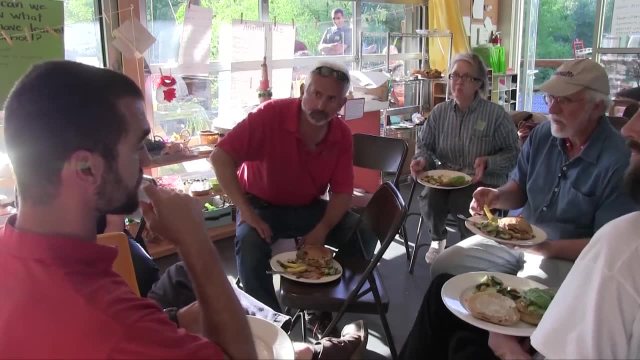 He'll run the soil analysis for you for free. Great. The only ones you're going to have to pay for is the PLFA and the soil wet. Yeah, If we could talk about PLFA, that would be really cool. We could talk more about that. 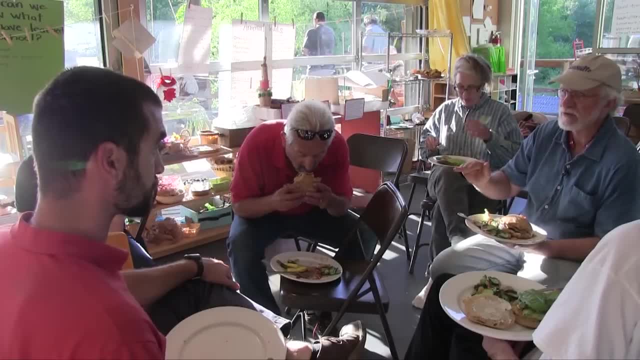 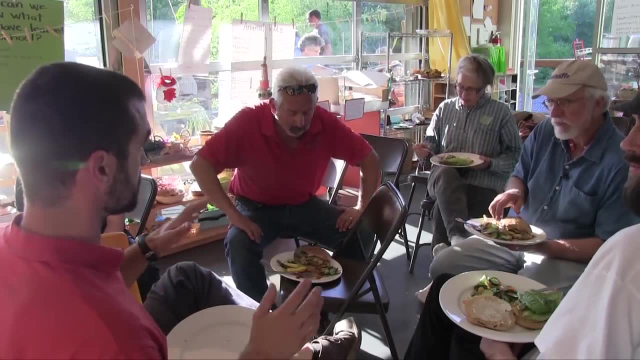 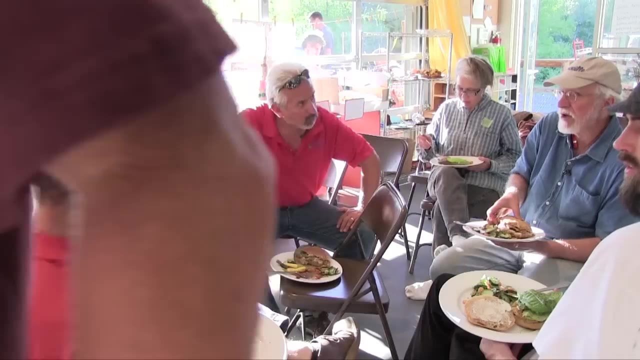 If we're going to bother to use that poison, I want people to see the reasons why we should use it. Yeah, PLFA would pick that up. It's a fairly coarse microbiological test, Probably like 20 variables. No, You don't think that the 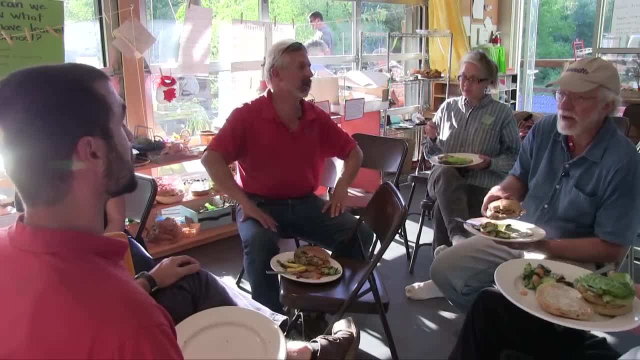 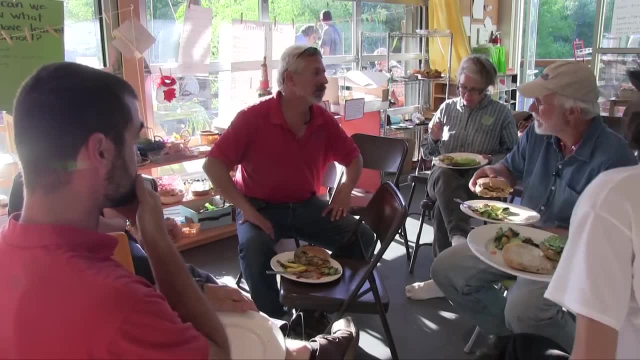 salts from those herbicides. You know where we picked it up. No, I think that it could. You know where we picked it up. I don't know if that would measure it. well, You know where we picked it up. Dr Haney did a test on Rhonda. 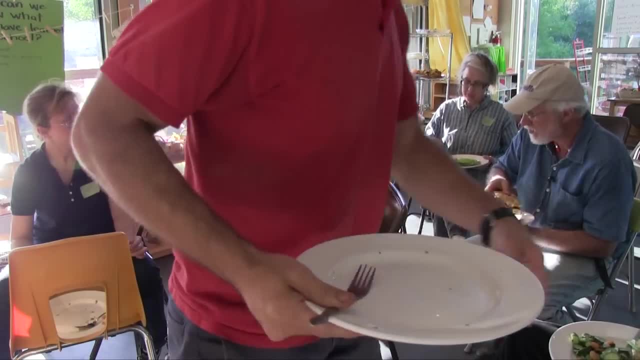 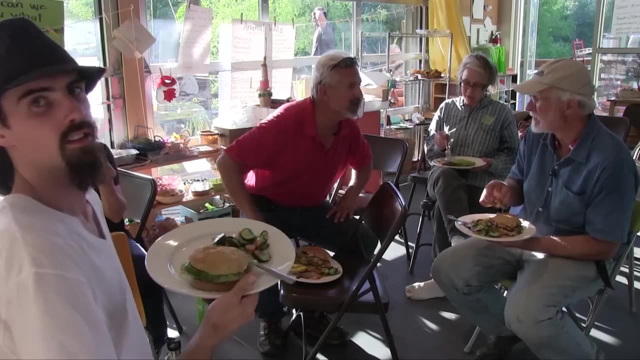 I'm going to go find out Sink and put this in, Then I'll be back. Be right back. And then I've always heard that surfactant, Yeah, and then Bonsanto never wants to say anything about the surfactants either. 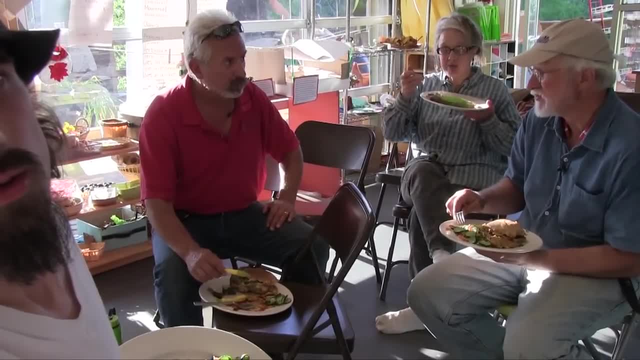 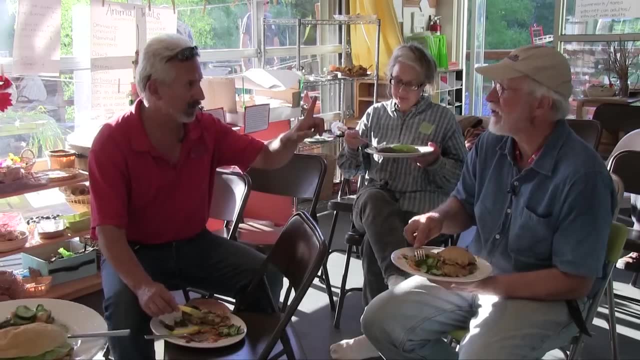 That's probably what's the endocrine disruptor to it. It's probably not the salts. And it's interesting We picked it up. The Haney test did pick up the respiration going down, So if we pick it up we'll be able to pick it up. from there, But the soil samples have to be done at the same time. We'll do them exactly as they tell us how to do them. You might not pick up the results of the herbicide until about 10 days later. You want to do the? 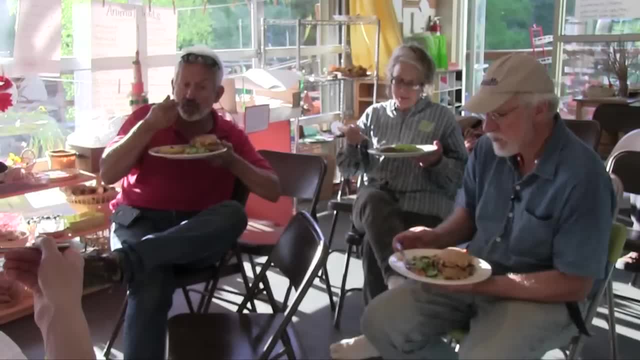 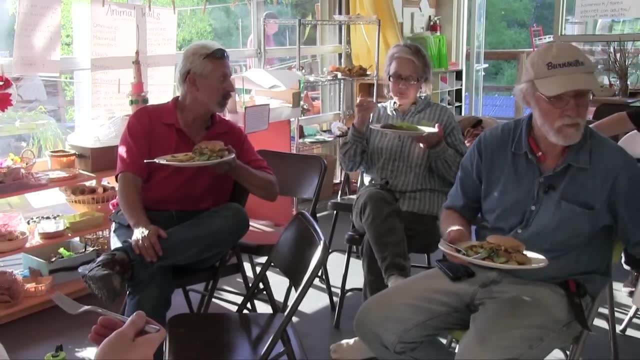 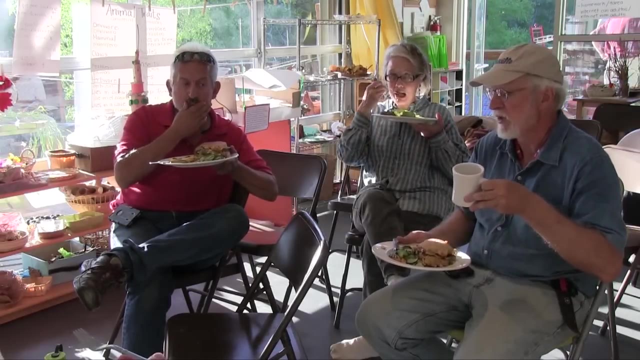 sample right before and after. We'll do it. Do you think the course worked out? It was a great class. You guys did a great job, Really wonderful class. Mark was saying how good it was The pickling. There's a serious critic there. 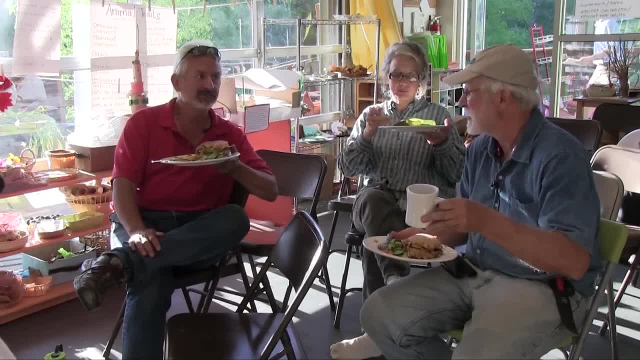 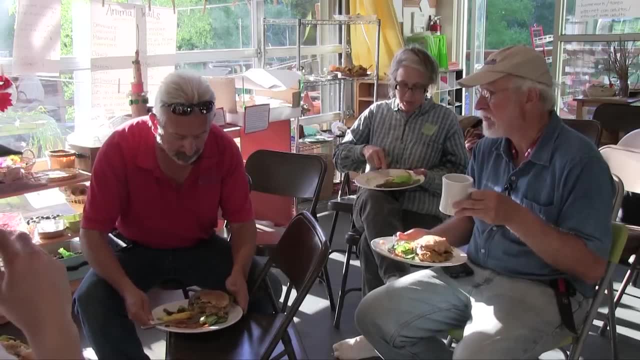 He knows a whole lot of stuff. Mark is the guy we were just talking about. Oh yeah, He just drove back with me and said it was a great course. Well, I think you're very blessed to have somebody to help you here. 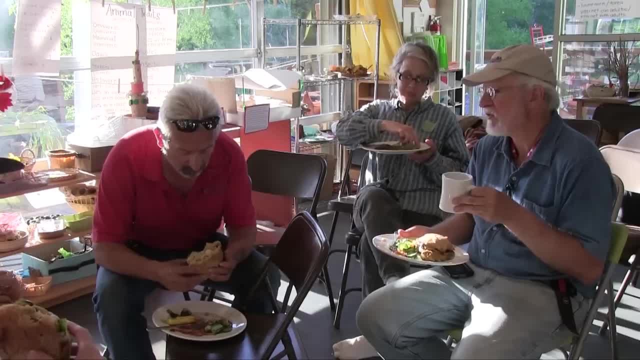 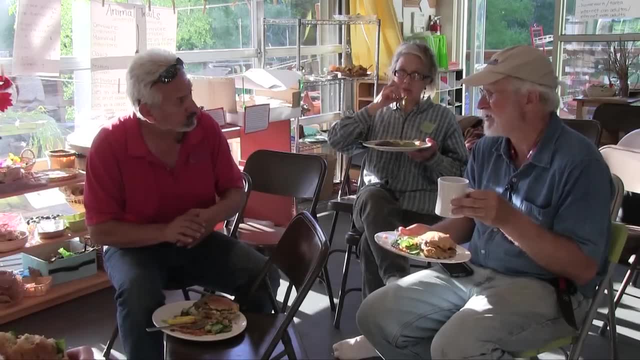 Pickled radish. Like I said, we didn't have a better workshop we've been to in a long time And Dave was in complete agreement with my reductionist science complaint. Totally gets it. you know, It's nice to have a researcher that sees. 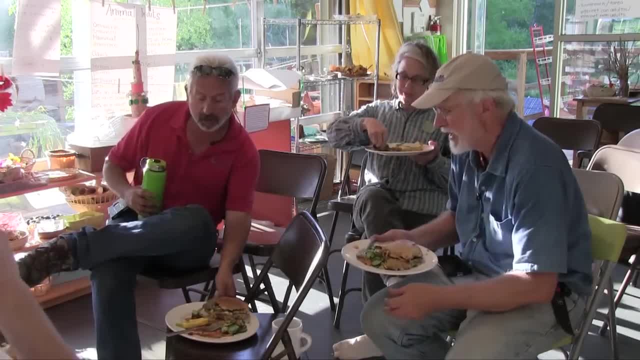 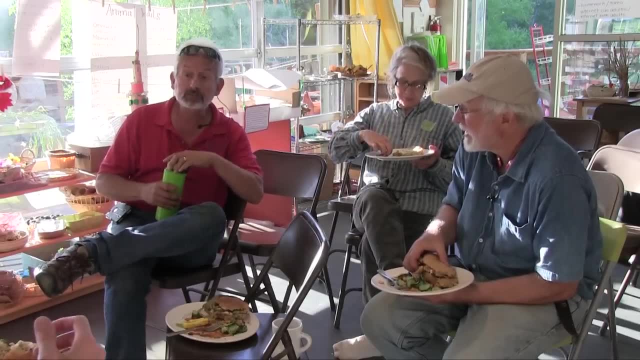 the whole ecology. It's rare. I'm excited about that. I hate to see Dave in the meeting. I think he ate and left. We could have put him up again. He's jumping to go. He's got a farm tomorrow. 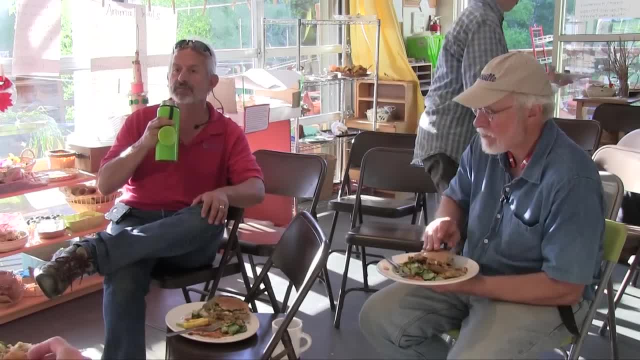 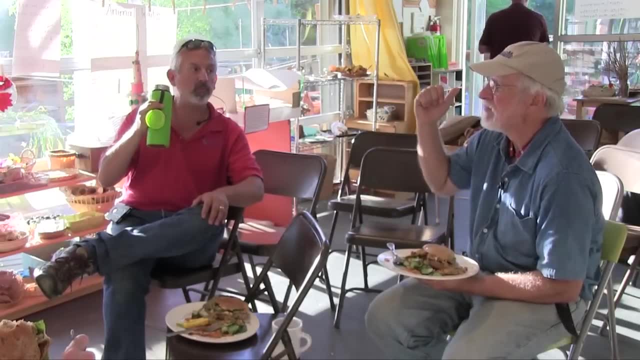 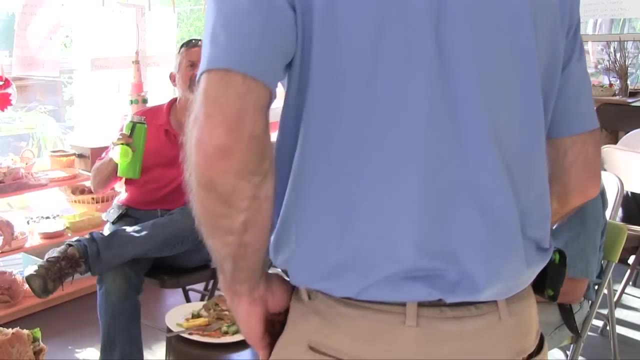 He'll send you the transfer free file. That was great, That was really good. Oh, there he is, Jay, can you? Oh, you need to leave. How come you're not going to send it? It's already done, The bread's done. 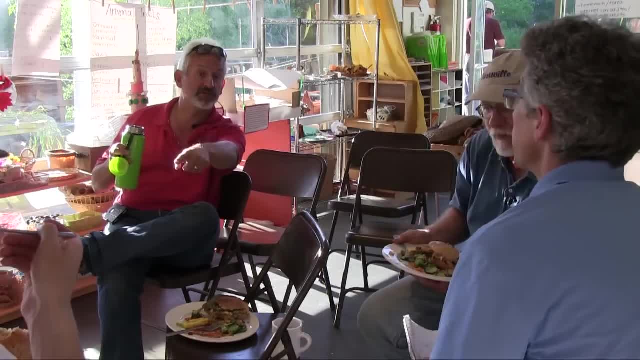 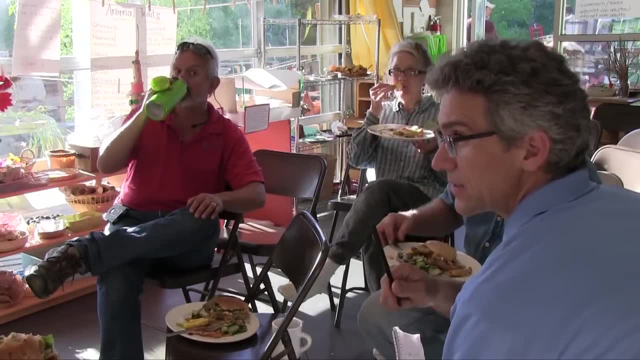 He wants your. Can you send him a transfer file Like your PowerPoint, would you? I'll have a flash drive. We're already packed up. We're hitting the road. I will get it to Pat and he can forward it to you. 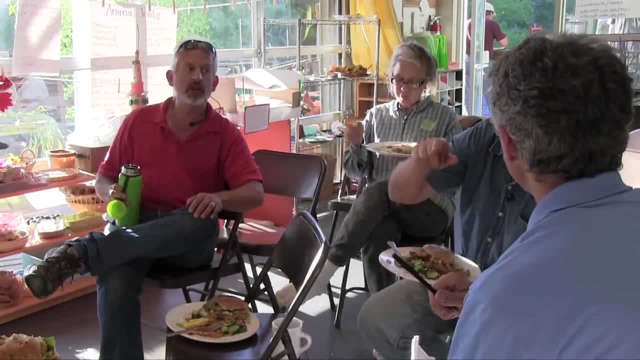 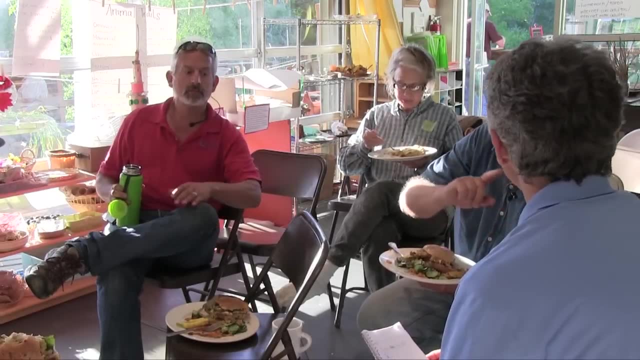 Okay, What I'll do is I'll get the address. You can transfer it right now. Pat's got enough to do. I'm computer trained. I'll be glad to forward the address. So I'm going to leave you a box of the cover crop mixes. 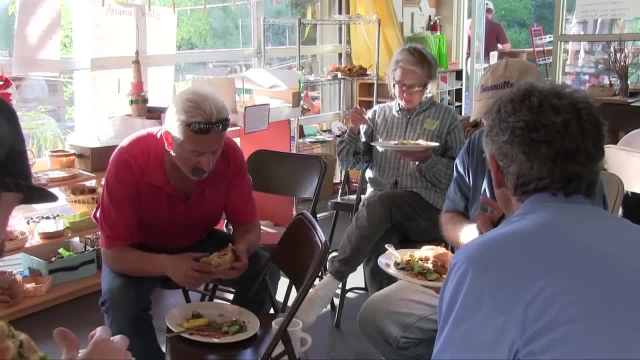 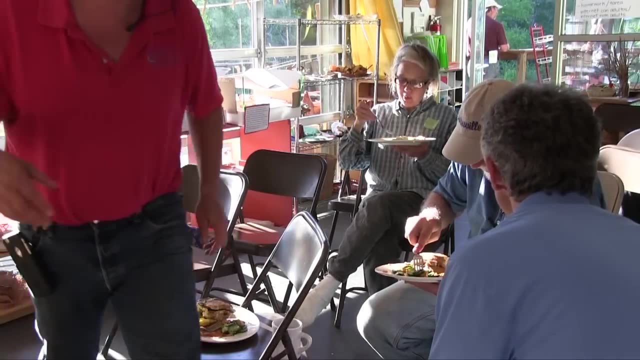 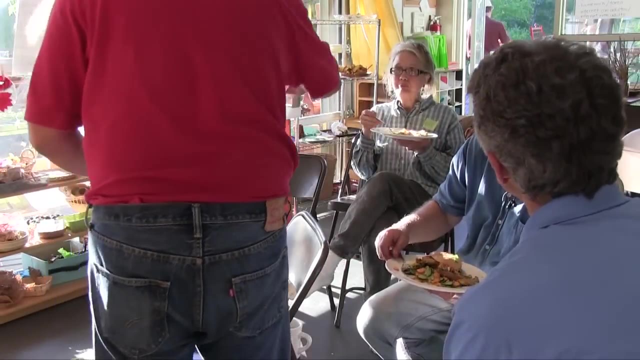 They're $7.. So now all you need to do is let me know what you have sold And I'll send you an interest. So I've got mine. I've got a list of what I left, So I know. So you'll get. because we have a wholesale price. So we'll only charge you wholesale, But our retail price is about $7.. So you're already packed up. I know people are looking for that kind of stuff. It's great to have you here. I'm really glad you made it out. 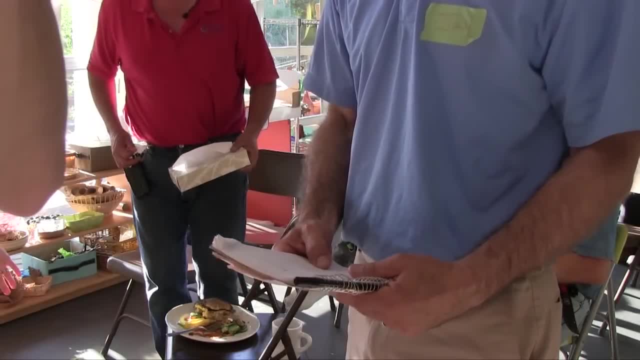 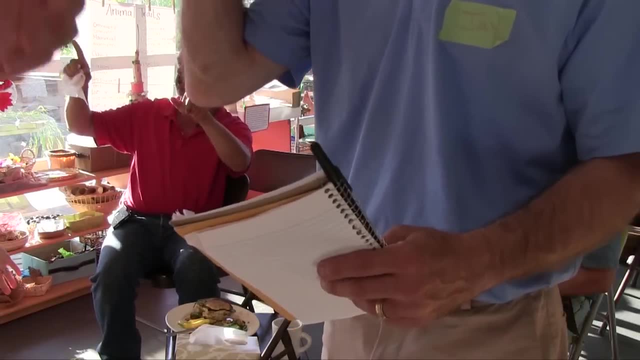 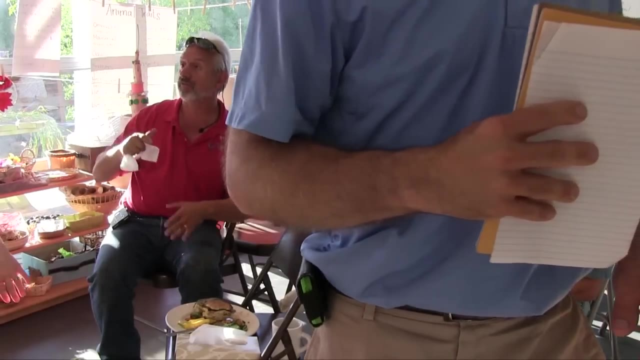 It's good to see you. Thank you for coming. I took it That's Ray's, So my information is on the computer I packed. Okay, I'll get you hooked up with Dr Haney. Okay, And I'll get you information for the PLFA. 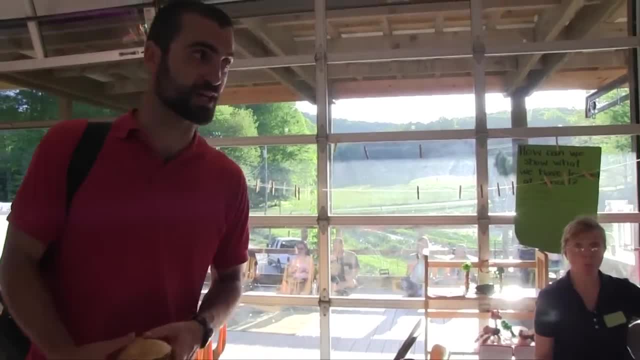 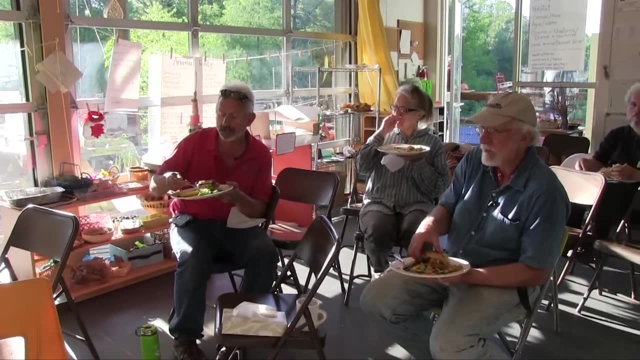 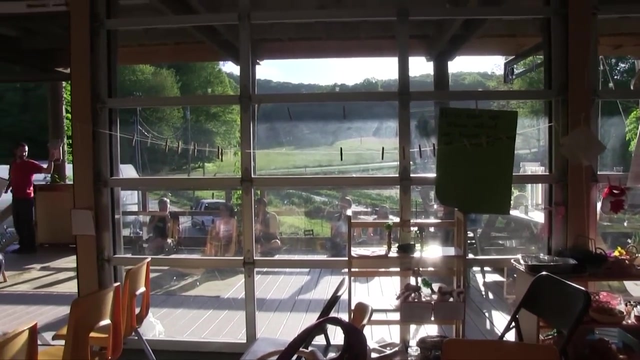 Cool, That would be great. See you guys, See you, Dave, See you man. Thank you, Jay, You were awesome, of course. Thank you very much. I thoroughly enjoyed it all. Hope to see you again soon. 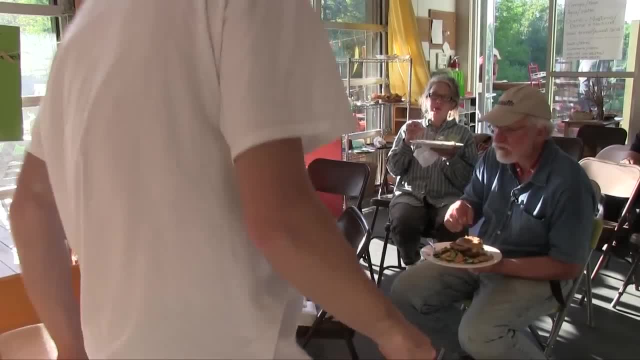 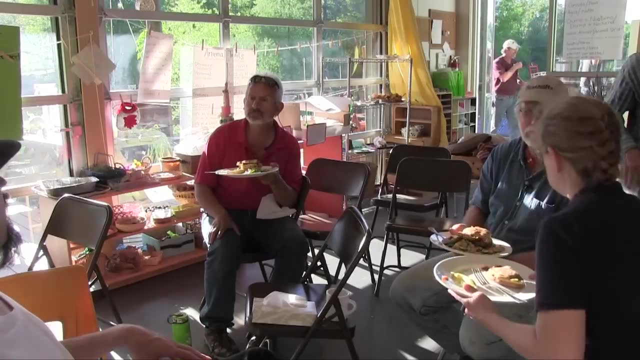 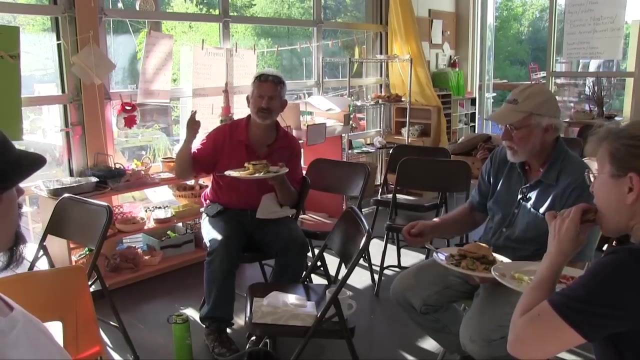 Thanks for filming. So, Dr Haney, if I gathered it correctly, she said that you could plant directly into cover crops. in certain situations, You could plant directly into it. Yeah, that's what I gathered. Absolutely That's what we were talking about. 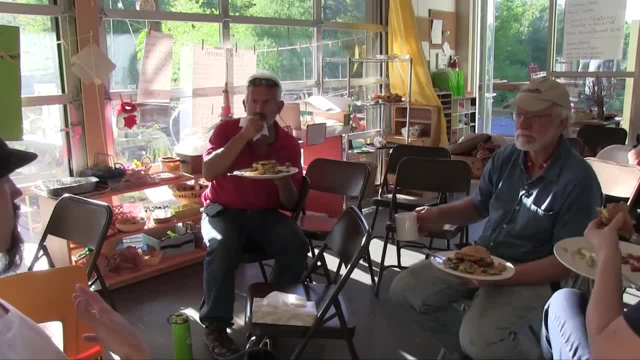 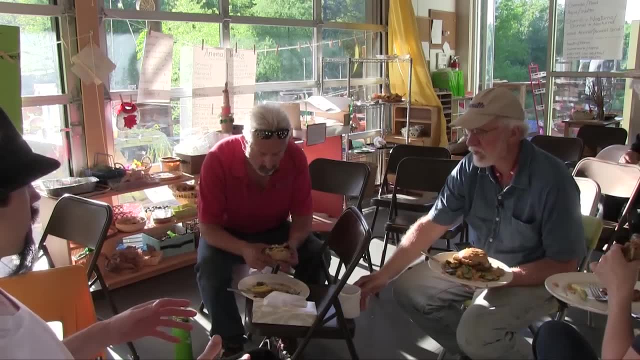 It's called green planting. Let's talk about that, Because that's what I'm doing, That's what I'm really interested in, Because we've got cover and a few other kinds in our garden And we want to plant tomatoes. We want to plant it so that it's not tall. 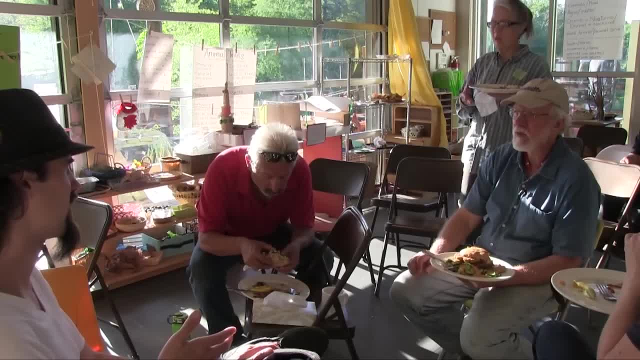 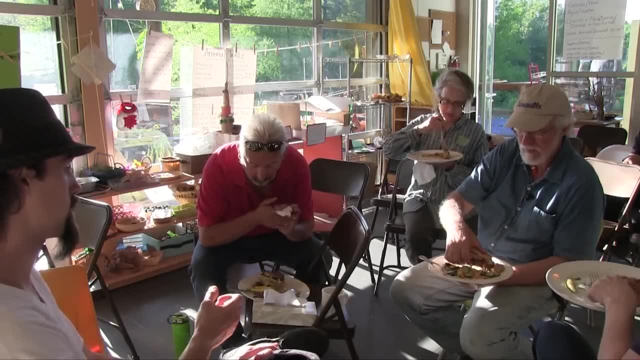 But we don't want to kill it, We want it to come back, We want it to get established And we've got a bunch of these mustard greens that came out of our compost from our last house And we're just going to take those up. 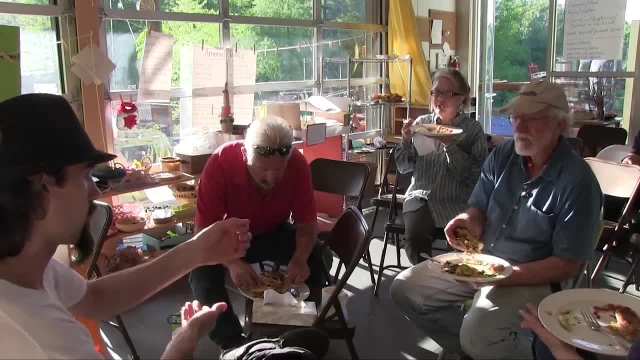 I wouldn't take them up, Just cut them down. Well, you know what I mean. Don't pull them out, though. Leave the roots in, Just let it lay there and plant through it. See, I was thinking, if you pull something up by the root, 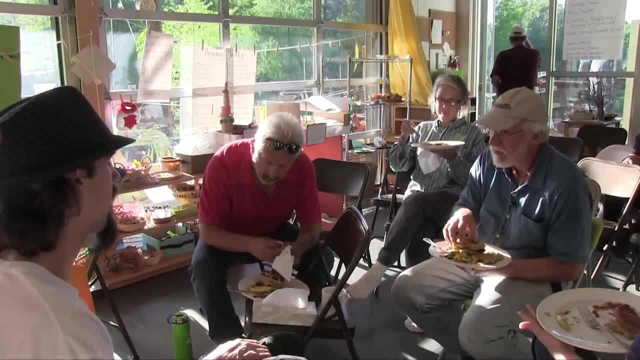 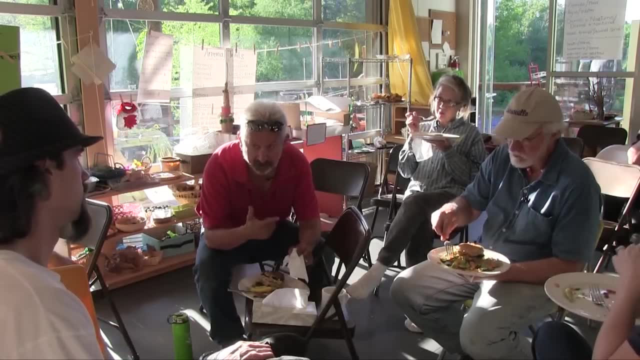 and it leaves this hole. isn't that a good thing? In a different aspect of what you're trying to get out of it, The thing is that it's quite different leaving a hole versus mechanical tillage. Mechanical tillage actually stimulates oxygen into the system in a large amount. 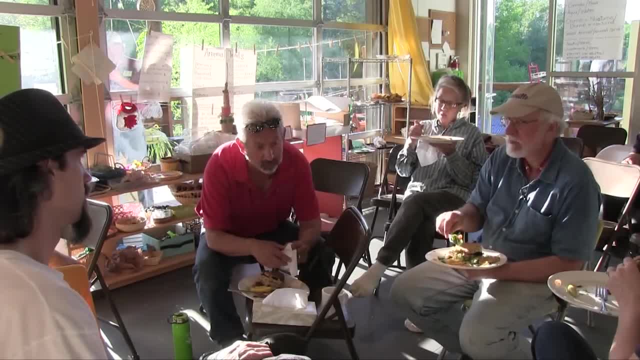 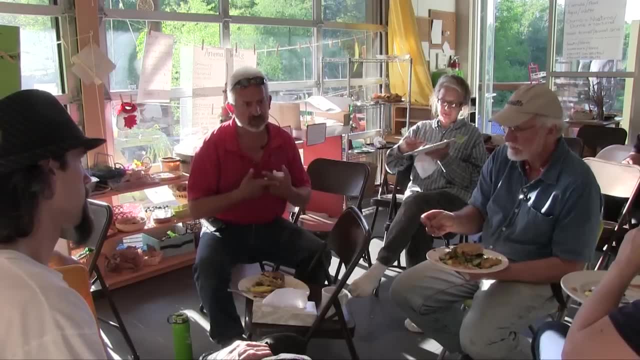 and wakes up these coprotrophic bacteria. These are strategies Very different. When you run the rototiller or a rut disk, you smash aggregates, you server the hyphae, you create a different system. What you're doing? you're doing biological means. It's not an issue, But don't you think it would be? I think it would be less work and, I suspect, even be better for the soil, rather than pulling it up, which is a disturbance, just cutting it off and letting the roots rot in there. 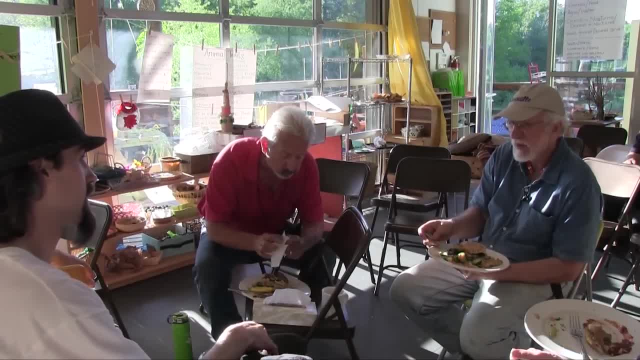 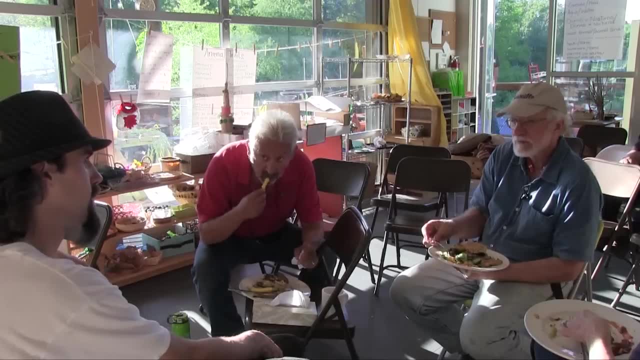 That's what I was thinking. You get the residue down there already. It doesn't have to fall in the hole. The only hole you make is to put your plant in. Don't bother to pull the stuff out. Well say, I plant a tomato and I just 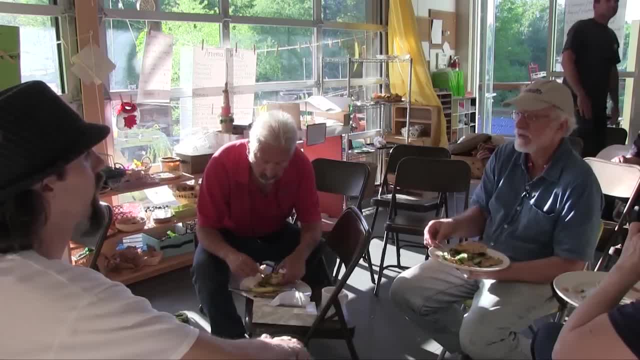 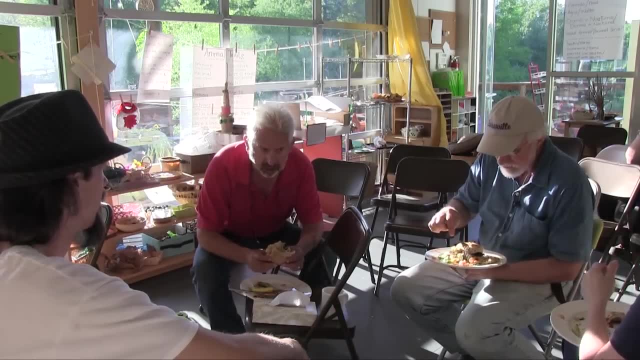 part inside. Yeah, that's right. That's the hole you make. You've got to do that With the planting mix. It's not three-year-old cover crop soil, It's just a yard. I'm considering that with the chickens. 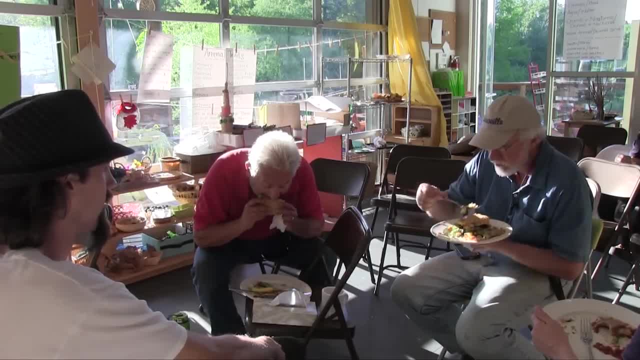 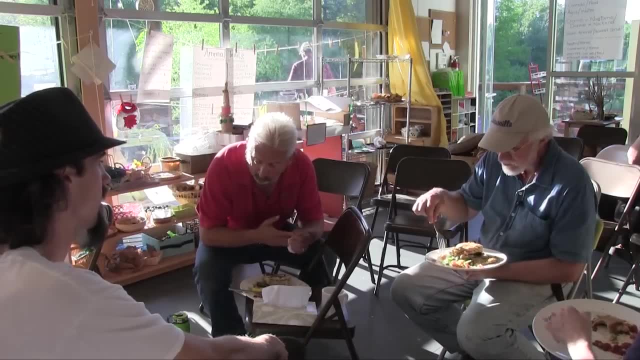 and everything that's been on there. I don't want to put the chickens back because that will be fresh poop and that's only okay if it stays on the surface and it's not near the tomatoes. But as far as cutting the cover crop, I found better results when I have mulched the cover crop around my plant without cutting it, because when you cut your hair it sticks up straight and it sticks up through the mulch, but if it's long it can mat from weight. That's exactly what we're doing. 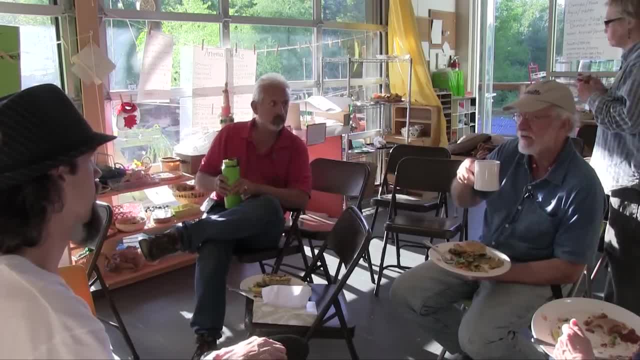 That's why you do the roll. You get a better kill rolling than trying to. even if you till it under at the wrong time of year, you can't kill it. Now, what are worms eating? Do worms eat composting material? Worms eat microbes. 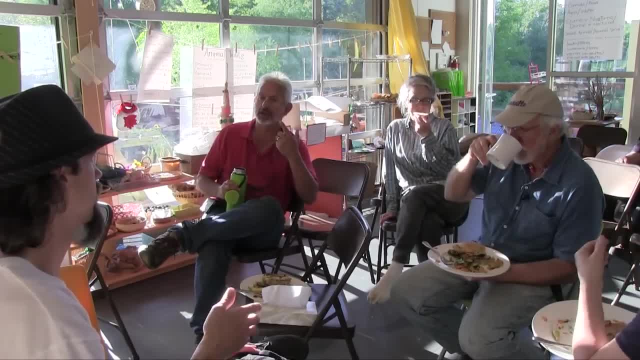 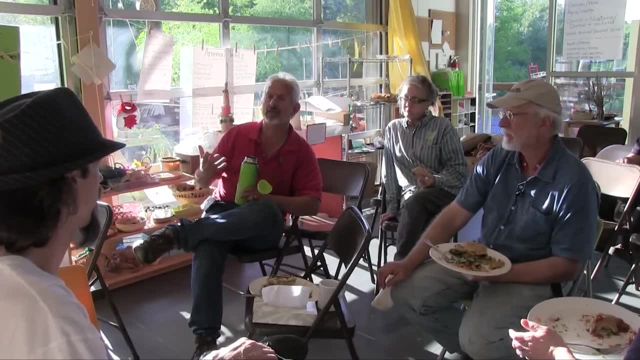 Yeah, they eat the protozoa. They're like little vacuum cleaners. They're way too big to know what they're eating. How can they find a protozoa? Oh, they can. They're like giant vacuum cleaners. They've got protozoa on there and they'll eat it. 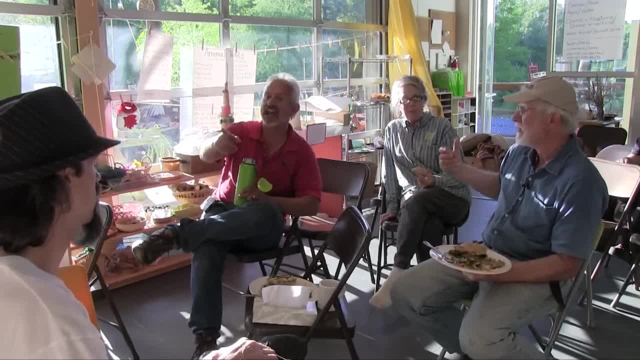 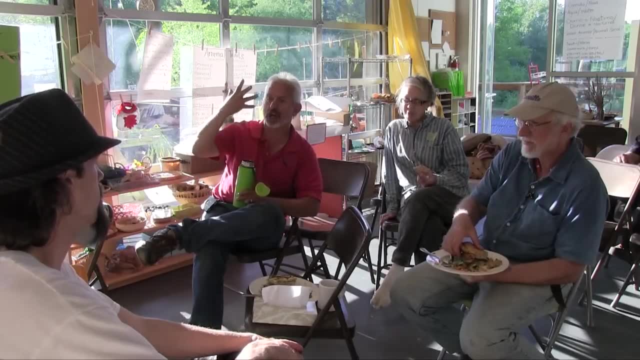 They're like the whales going through the ocean pulling the protozoa. That's a great analogy, excellent analogy. They pick up those crayons- you know how they use, like those fins, and they'll pick up these little tiny fish. They're like whales. Earthworms are very similar. 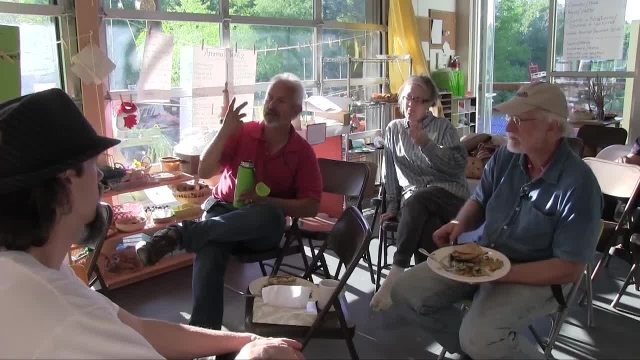 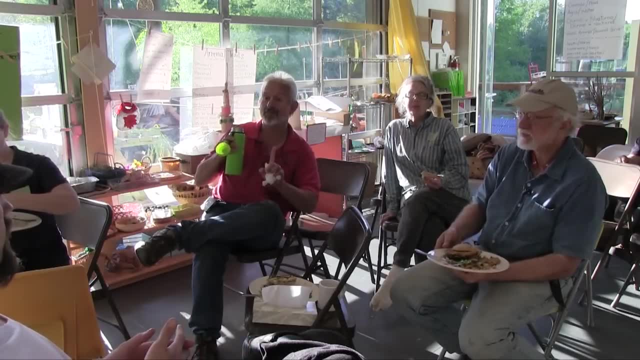 They'll pick up those grains and they'll poop out and they'll pick up the bacteria and the protozoa. Where are you going to find worms? Where are they prolific? Build it, they will come. They're there. Create the conditions. 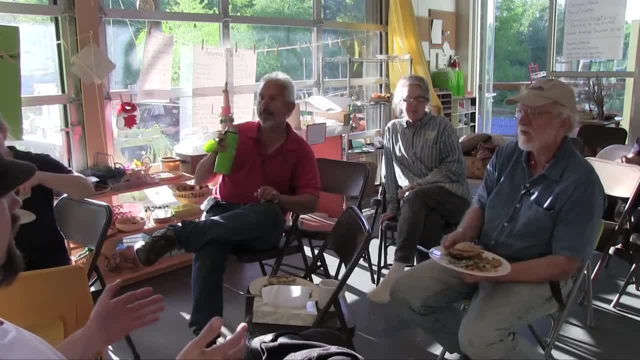 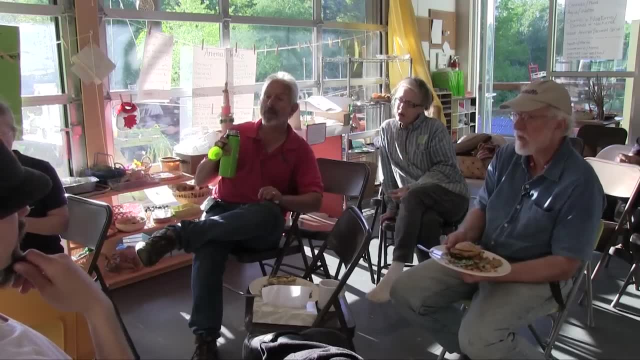 The conditions in the soil, or do you need some kind of compost in this situation? Do they like to be in compost? That's different worms, Different worms, And the thing about it is they're already there. What kind do I want? Well, you'll get. 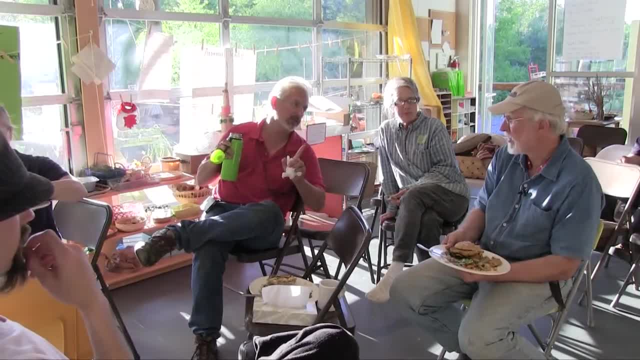 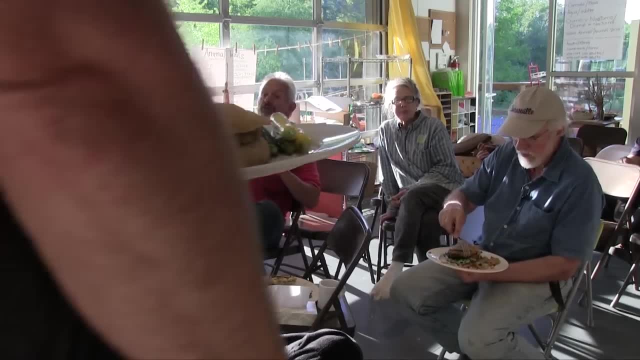 what's it called? What do you call it? The big earthworm? You want them there? Night crawlers will be there. The thing is, all you're going to do is feed them. Right now, a lawn situation is pretty sucky. 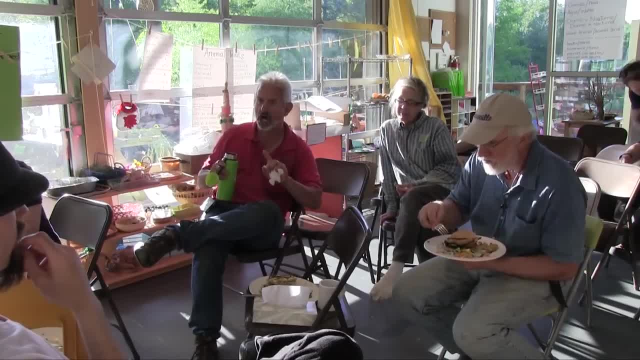 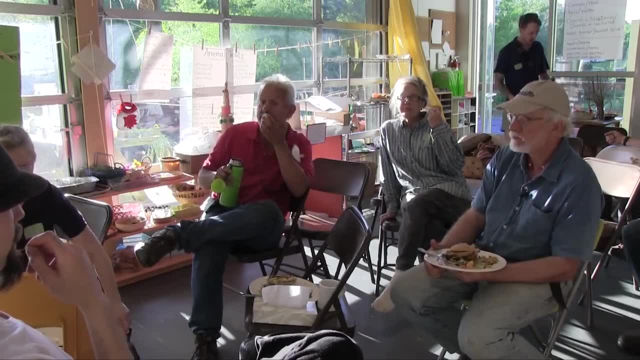 You mow it all the time. It's short, It's hot, It's compacted, Walked on, It's just not much biology, I don't think. I think what he's trying to say is that you don't have to. worry about what kind of worm you want. They'll come on their own. They'll come on their own, But what I'm trying to do is accelerate the process in nature. Do you want to accelerate? This is my biodynamic runner, The fastest way to get the soil. so it is. 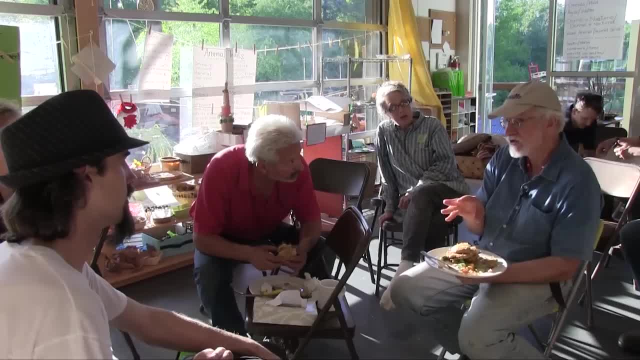 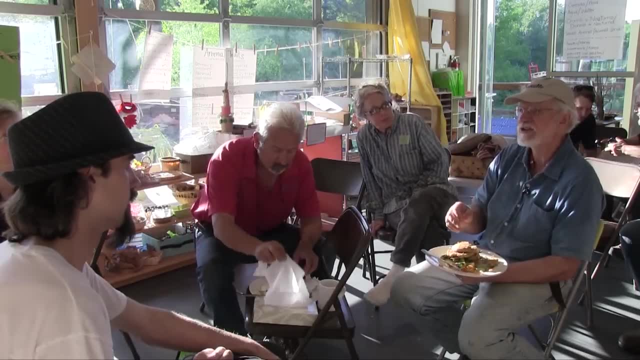 rocking. incredibly is if you know somebody who mows lawns So you can get fresh grass clippings. You take food waste and put down about an inch of food waste. Put four inches of fresh lawn clippings on top of it. 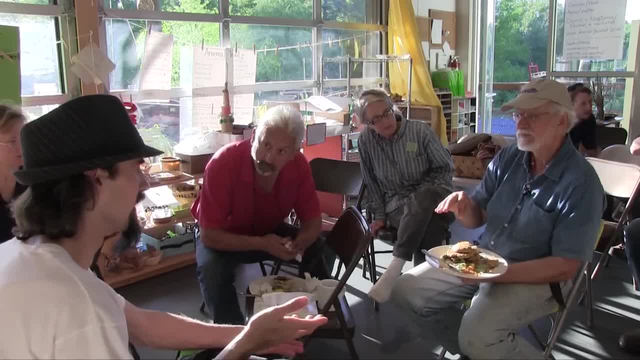 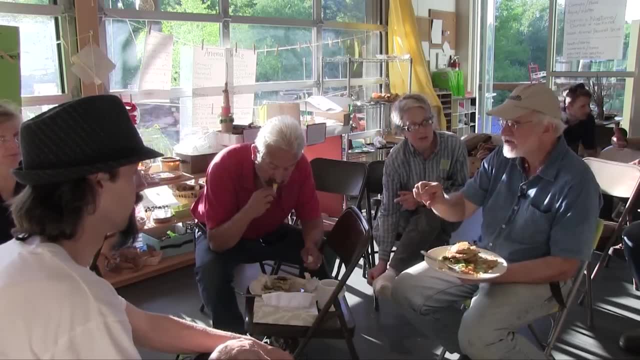 And then four inches of dry brown on top of it. Lasagna bag: No, but it's got to be that formula, That specific formula. I've got lots of grass, That's what I'm mainly using. Put about an inch or two of food waste down. 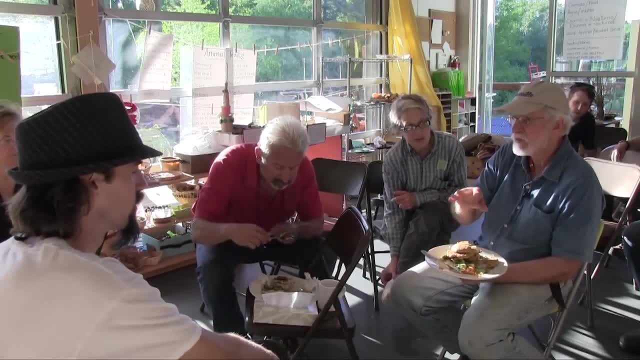 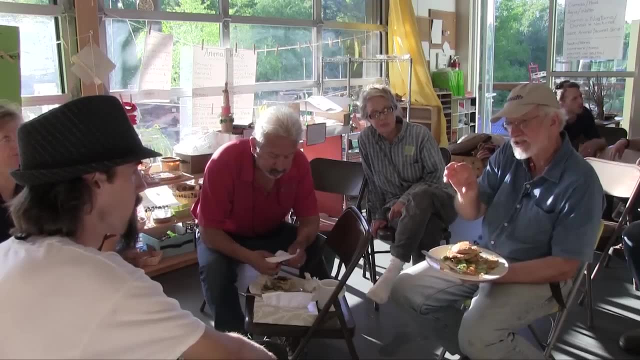 Not anaerobic food waste, but just fresh food waste. Put that down: Four inches of green grass and then four inches of dry brown, So you create this thermal because of the grass. It heats up. That stuff breaks down fast. The light comes. to the soil so fast, you wouldn't believe it. So once I've got the worms in there, they're going to go down and they're going to start aerating underneath. Yeah, but you don't worry about the worms coming in, You just create these conditions. 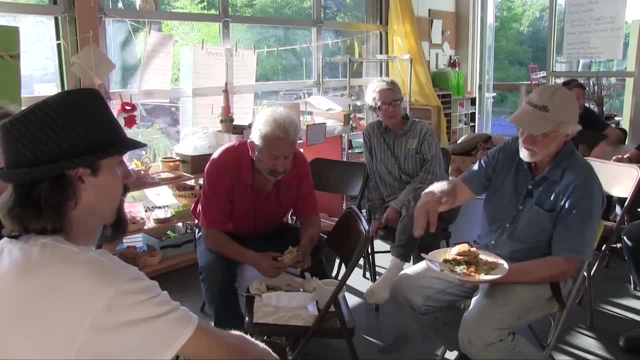 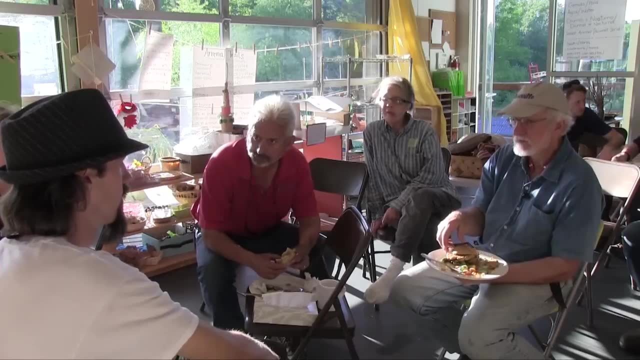 You're going to create incredible microbial diversity doing that, And then the worms will come in and follow. There's little cocoons there, They go into excavation and they're waiting for the right conditions. They'll come. I taught this to Mike and 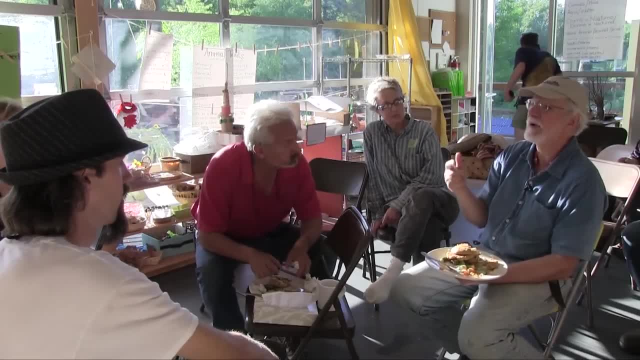 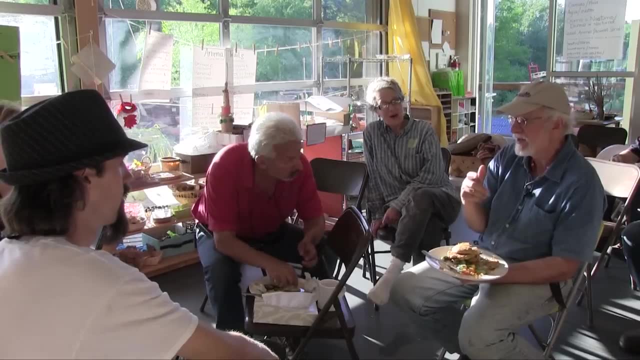 what's her name? Myla Lakers. What's her name? Mike and Lori. And they put one bean plant in that their daughter had started digging with us. That bean plant was enough to literally. Mike finally was willing to let Lori just temper what he was saying, but they both agreed. 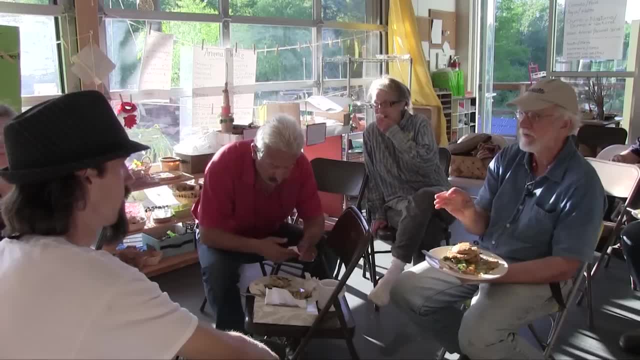 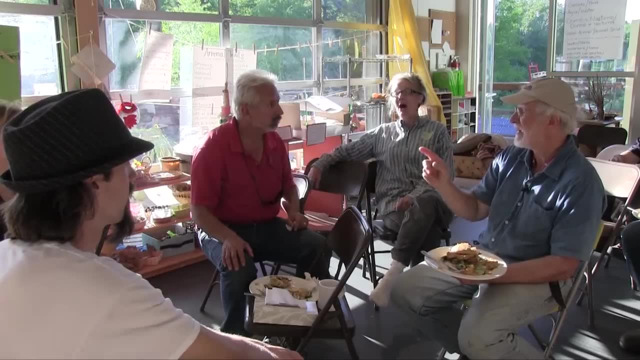 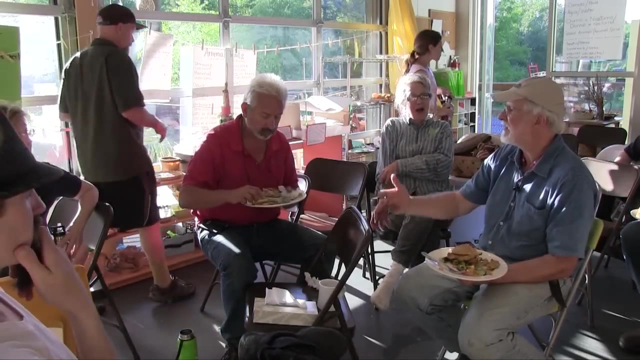 15 pounds of beans from that bean plant, Not counting what they ate. One bean plant Eat what They got. 15 pounds of beans from one bean plant, not counting what they ate. Using this fertility system Because it just makes it so diverse. It's like it's putting everything. 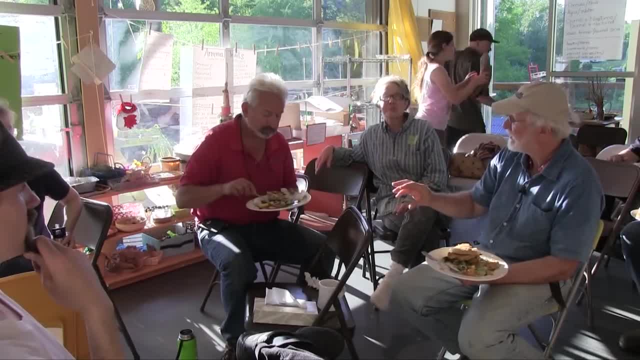 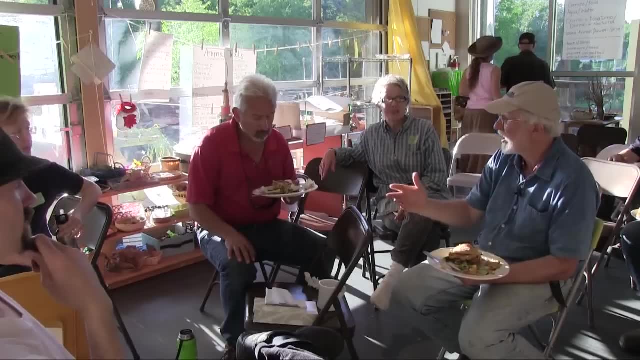 we're doing on high speed. You got the readily available nutrients from that food waste And then you have this thermal situation where it heats up. There's nothing you can do on a big scale. This is, for small scale, What you're doing. you will ramp things up faster doing that. 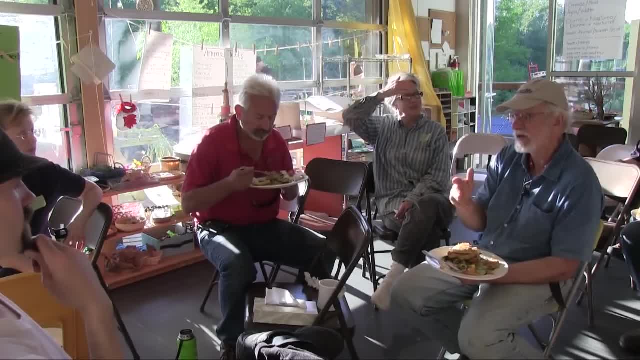 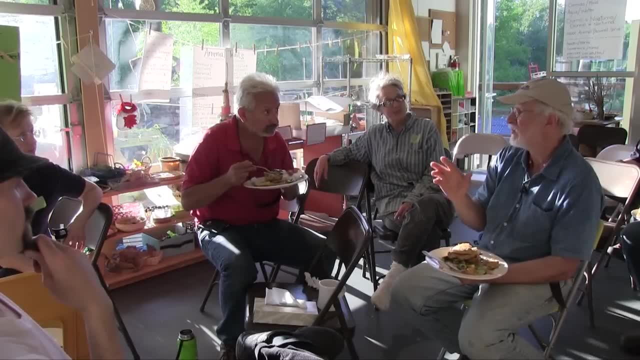 I've never seen The first time I did it. I got taught it by Bob Carnegie, this biodynamic grower. My kale, my collards, all those hardy crops, died from the frost because they were way too lush. They grew way too fast. 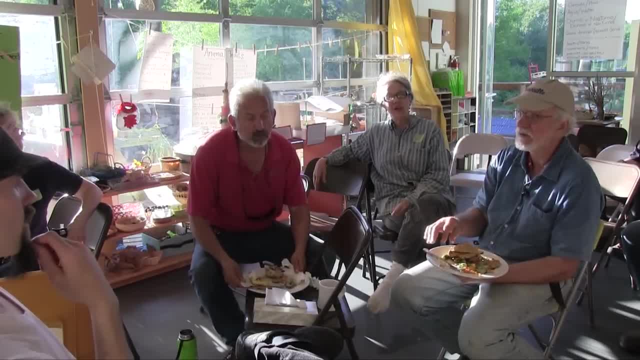 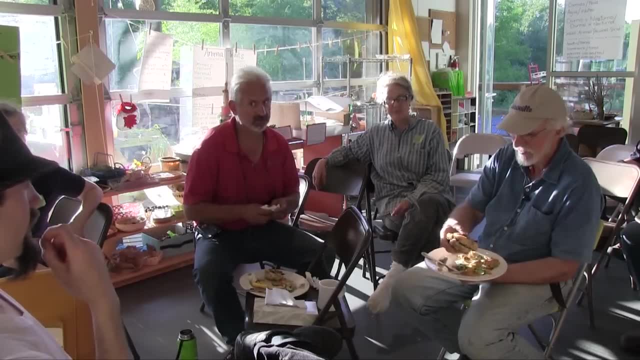 It is the fastest way to pick the soil into high gear. So what Pat is telling you is: we underestimate way the power of the biology and what they can do. They do everything. I was just asking Marshall's dad what he thinks about steaks versus strings. 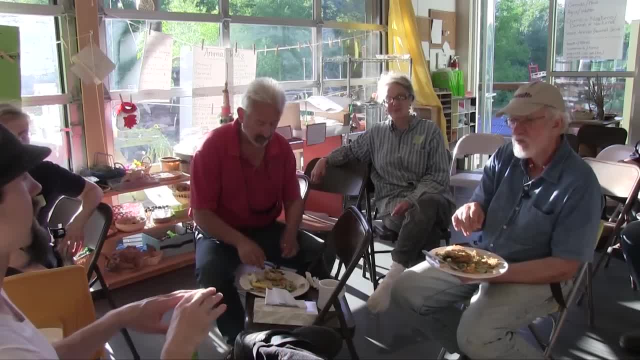 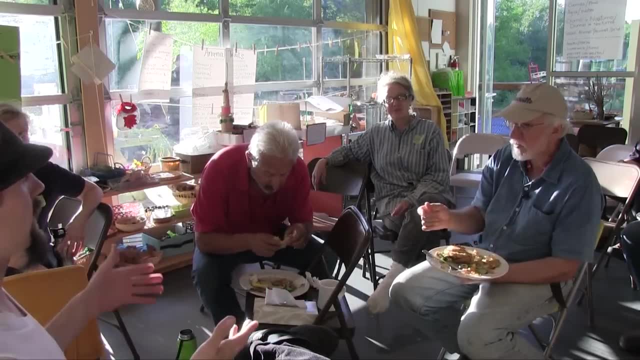 versus burying the tomatoes. What do you think about burying the tomatoes as they grow and picking off the bottom leaves and burying those nodes as they grow, so they don't get taller, they just get more root mass. and the bottom leaves are what blight first? 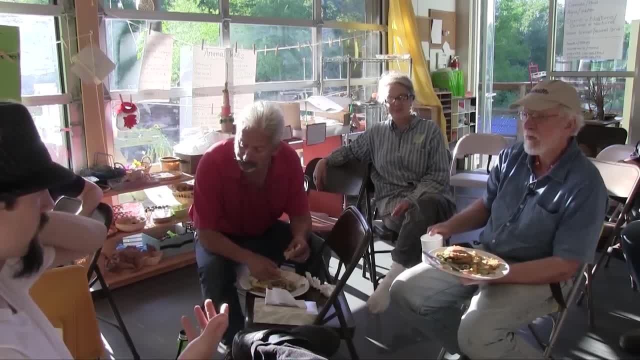 so that's also preventing the blight, because they get blighted first and the fresh growth is the blight. Yeah, we do that. If you're going to do that, you're going to have to suspend it, though You're not going to be able to bury it because it's out of state. But if it's suspended and being buried, I've got to move the whole suspension system down as they all run right. That's work. It's work. but you get a lot of production. You do that in greenhouses. That's what you do. 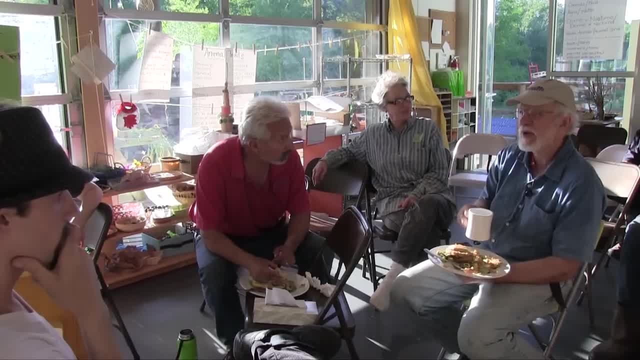 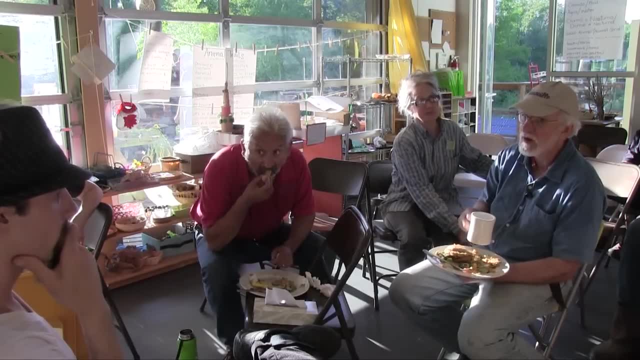 That's how you get the maximum production out of a greenhouse. The same plant will be in there for eight months and that's why I said we bury the pukes. like that You get massive production that way. I'll tell you this When you're. 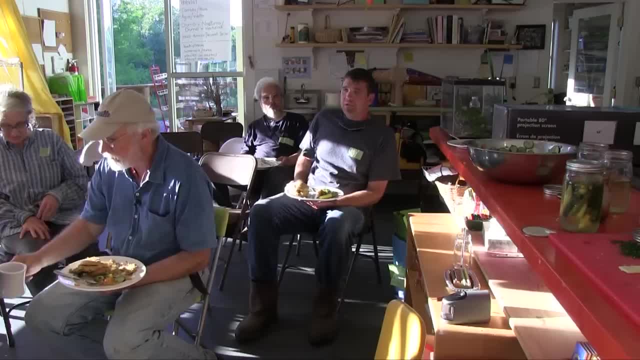 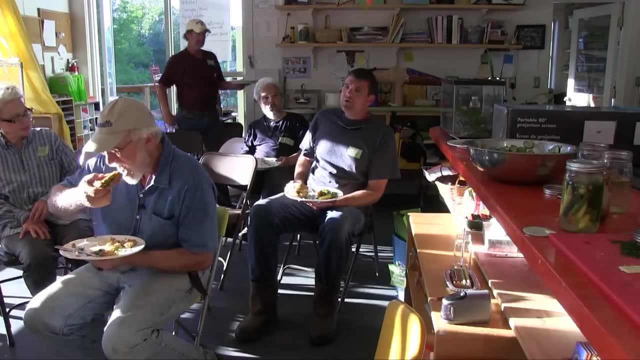 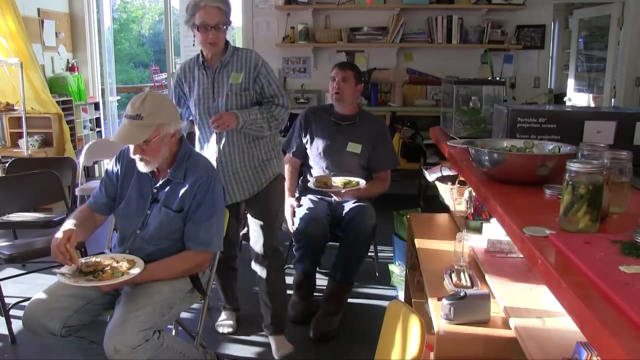 talking about tomatoes, late blight. early blight is easy to take care of. Late blight it doesn't matter what you bury, it doesn't matter what you do. If there are spores, live spores in the air of late blight. they're getting on that new growth While you're pushing those along. any of that new growth, even if you're harvesting that tomato, is still putting on new growth. That new growth is the most to getting those spores. The new growth. It often starts low. 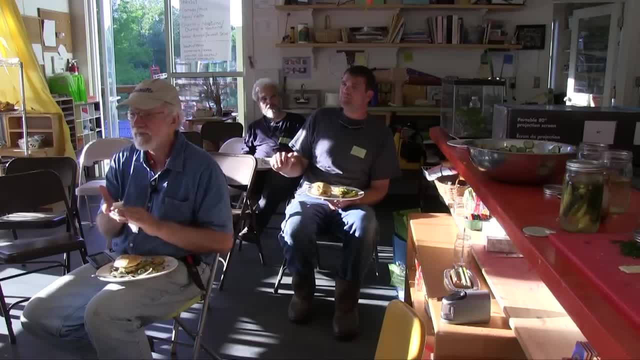 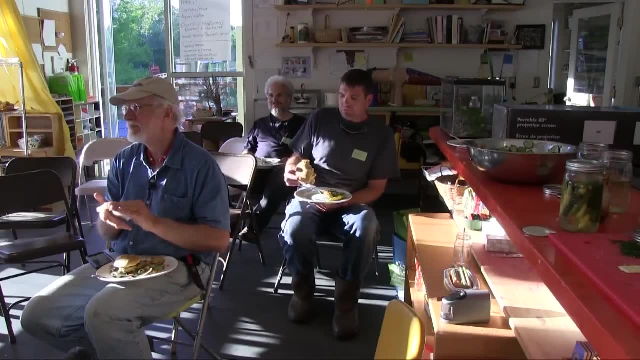 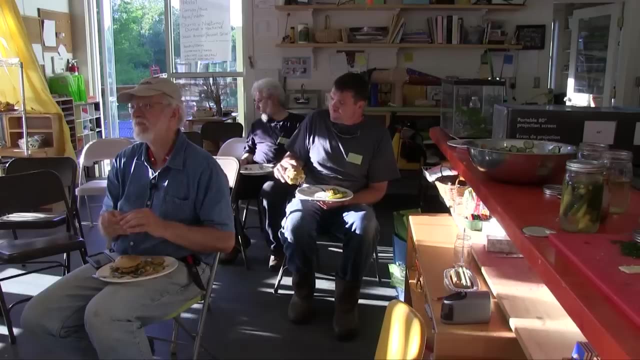 Early blight starts low. Late blight doesn't discriminate, It starts wherever it can. Thank you for coming. Bye, Redmond. Thank you for coming. They're for sale. They're for sale. They're $7 a bag. He kind of explained it to me. 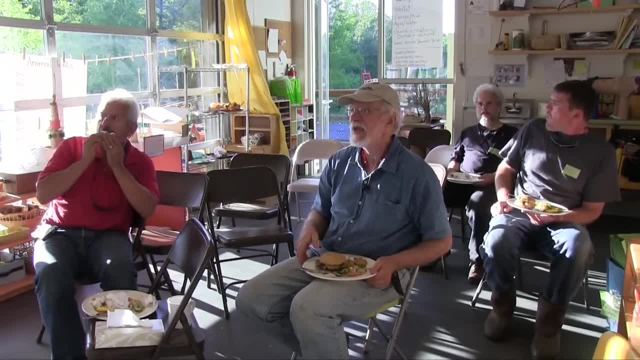 I offered to leave them here and I'll sell them because I know people want them. He had to go, but I know people are going to wish they had an opportunity. I'll have them. If you don't get them tonight, I'll have them until they sell out. 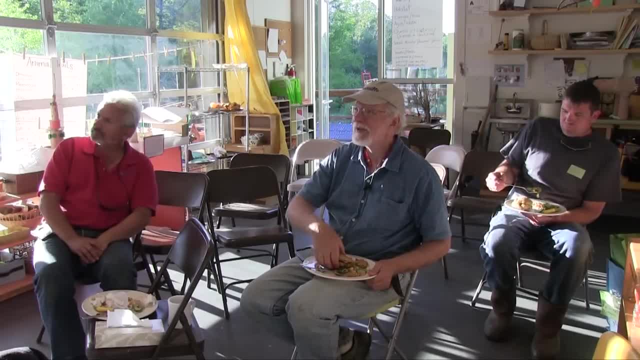 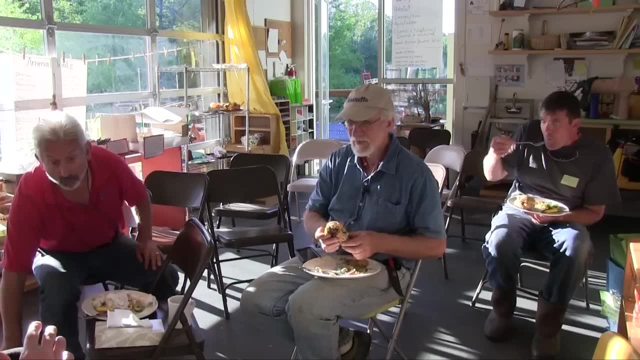 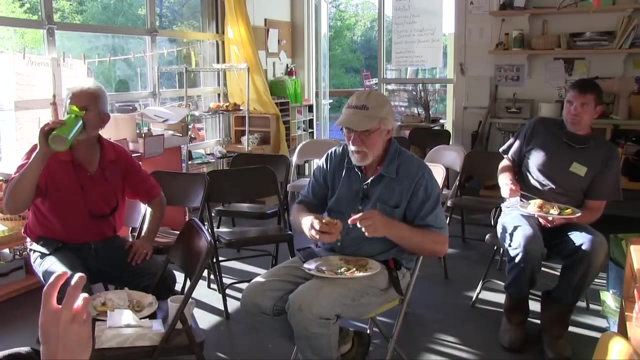 Thanks for coming. Thank you Absolutely. Thank you, guys. Quick observation: I noticed that all around the table people like Pat- they always wear blue. for some reason, Orchard specialists wear yellow, Michael Phillips and Andrew Goodheart, they all wear yellow. Cover crop guys seem to wear red. 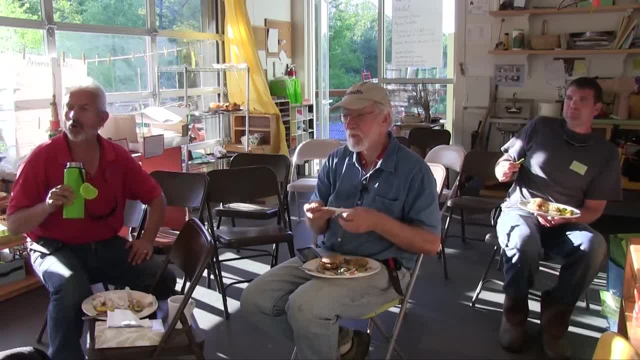 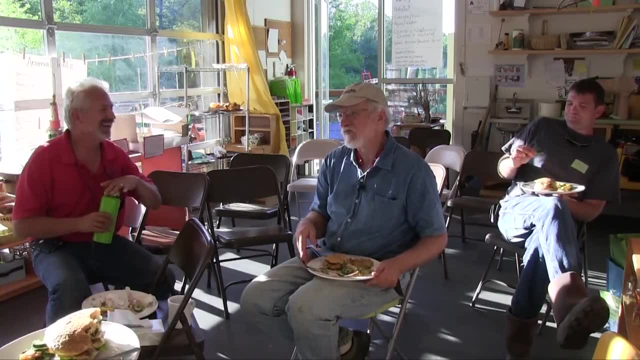 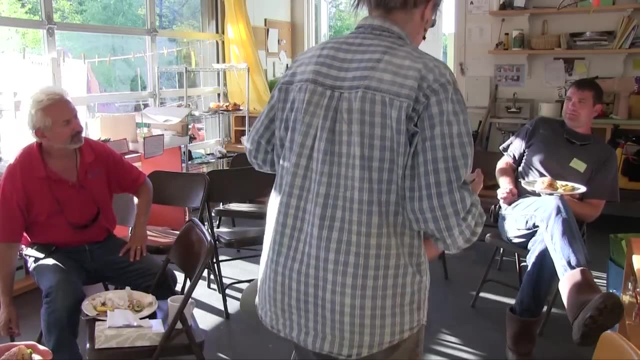 Including Mark Mark was wearing red. Wasn't that amazing? I think that was a coincidence. The truth is, I had a choice between We're supposed to wear black, A blue shirt and a gray and white striped shirt. I just happened to grab a blue shirt. 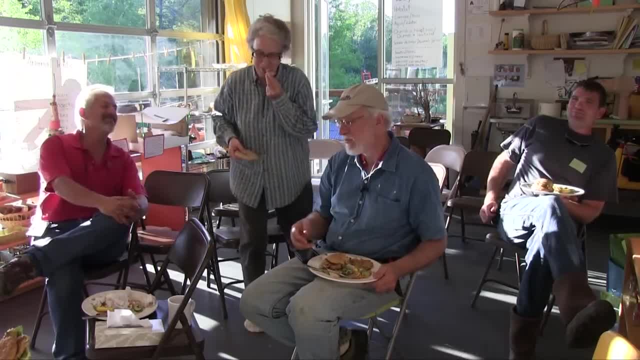 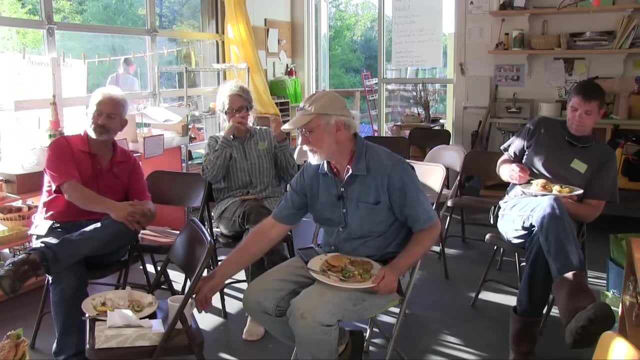 And I had something that was baggy, 50% chance I would have readily gone for the other one. My thing was baggy. I just don't like tight clothes, so I want baggy as possible And one that was clean. Clean is a major piece. 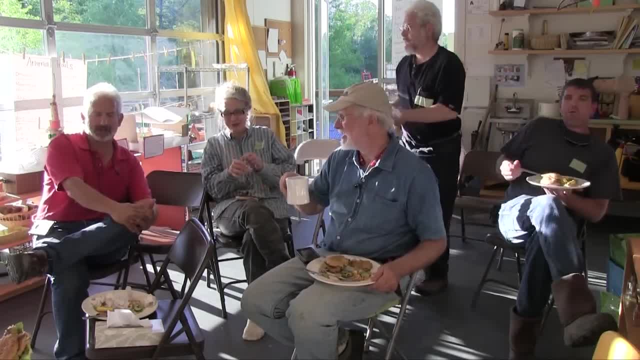 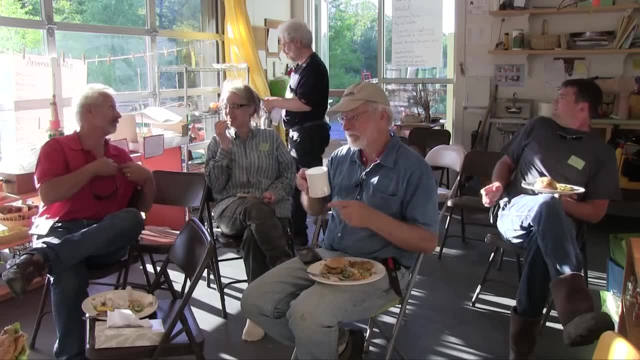 And not wrinkled as far as I am, because I can get very wrinkled. My wife tries to make sure I don't go wrinkled. You've got to look professional. I even wore my little government shirt. Thank you, sir. Thank you for coming. 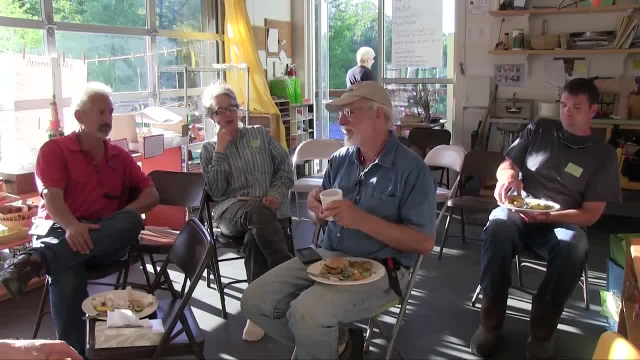 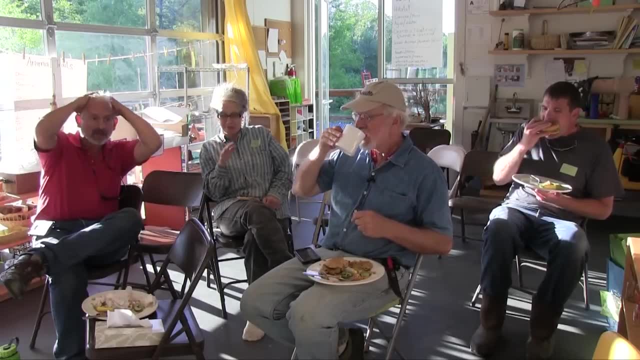 To which Meredith said: when I told her, Diane said: tell her, it's way too late. I saw Diane, She's here somewhere. She just stopped by for a minute. I tried to get her to stay but she set it back up north away. 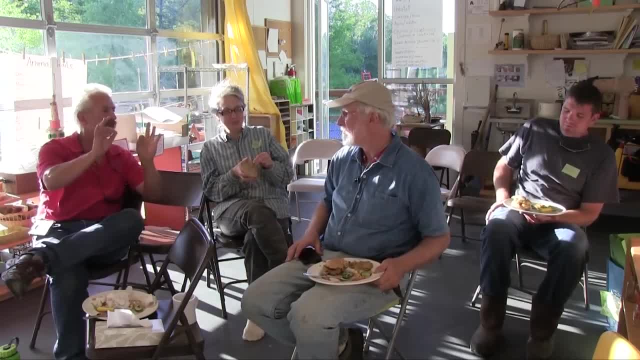 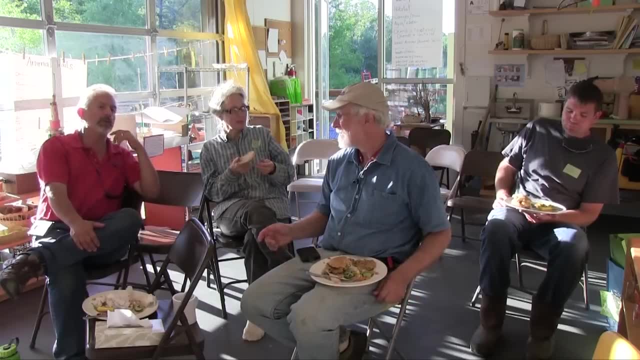 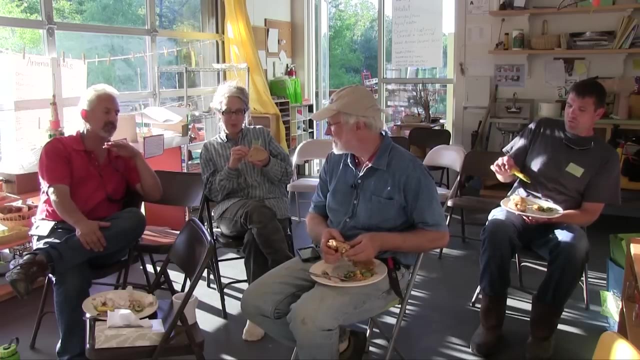 The bread was amazing. I'm glad you like it. You are a professional bread maker. I was a professional bread maker. I actually teach it too. Love bread, A lot of our bread. I can't believe that wheat in itself is bad. It's not. 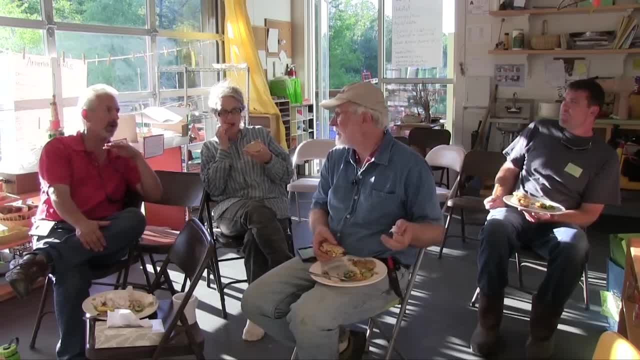 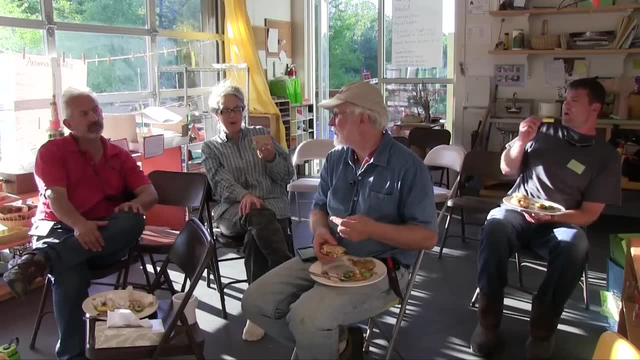 It's just how we process it. Now they're all realizing that if you're not getting organic, it's all got Roundup in it. They're hitting it with Roundup so it dries faster and of course it's systemic: You're eating Roundup.